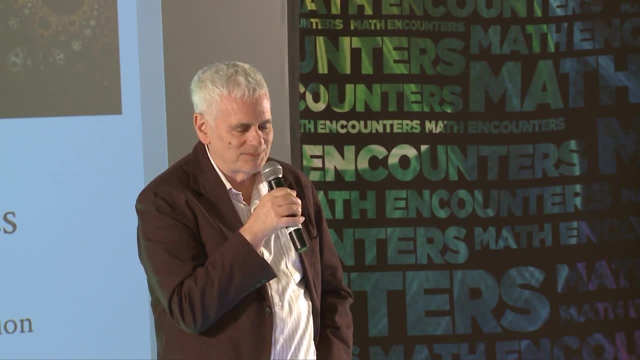 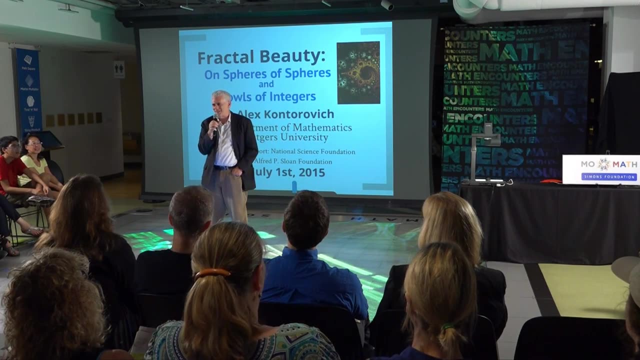 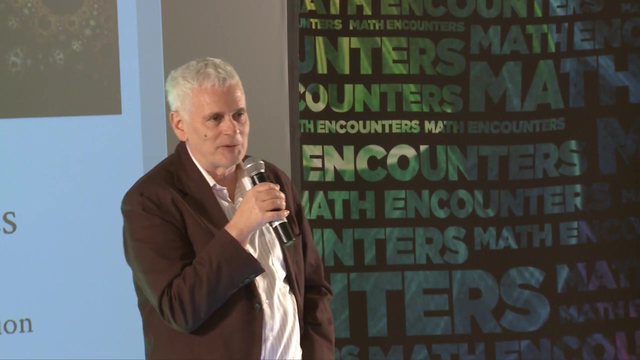 don't you talk about infinite volume quotients? So it wasn't so easy to talk about this topic, but it's actually what makes all his new math, his new ideas work. It's based on these infinite volume quotients. So let me just try to give you a flavor or an idea of what it is. And 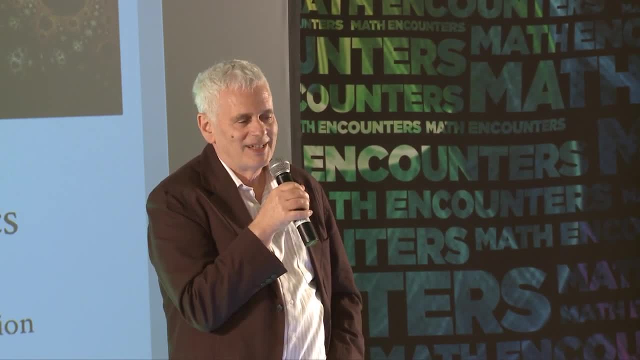 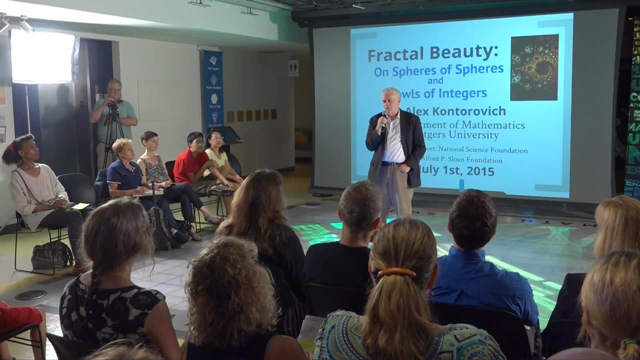 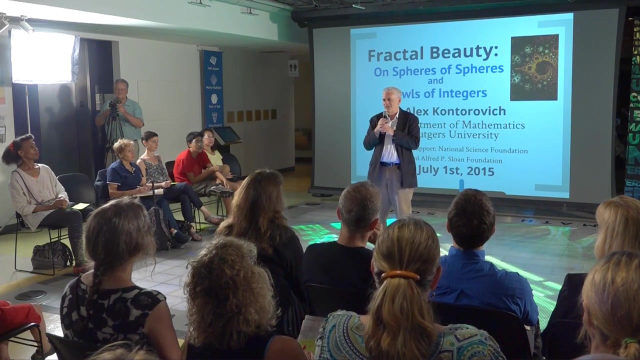 I'll just talk about the finite volume quotient. So imagine I'm on this ship and I get shipped, wrecked, and I'm on this island and I want to count time. So I'm living in this cave and every day, when the sun rises, I put a mark on the cave And I get a straight line. 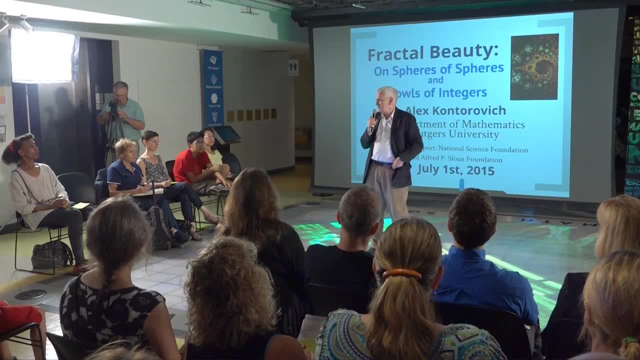 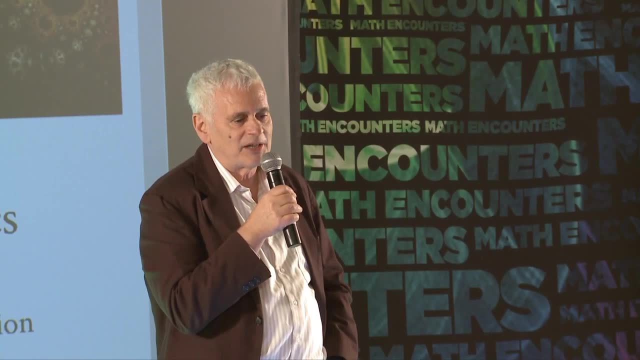 with these markings and I can look and see. By counting the markings, I know what day it is, how many days I've been here. So this is what's called a timeline, And time is actually a one-dimensional line and it's. 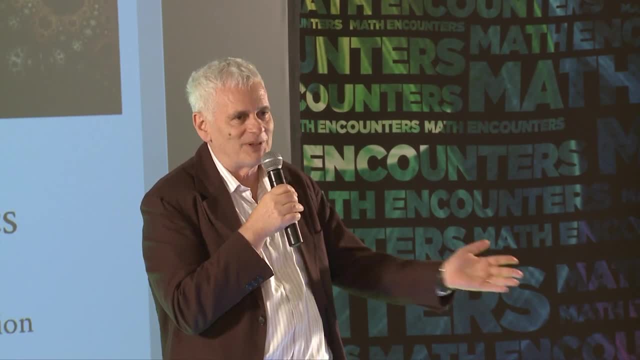 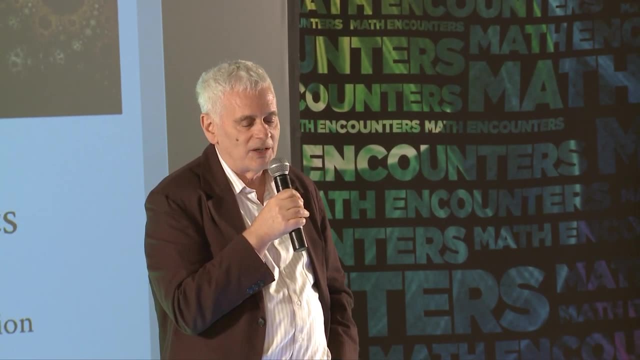 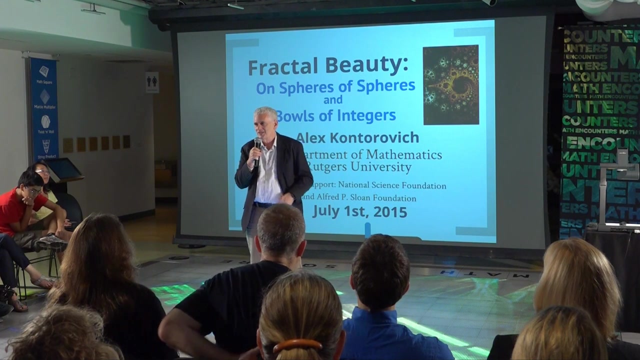 infinite. Of course I'm not going to live forever, so I'm not going to have infinitely many markings, But it does go on and on and on. Now what you can do is take a quotient. What is a quotient? It's like when you divide two numbers. You divide 15 by 3, you get 5.. That's a quotient. 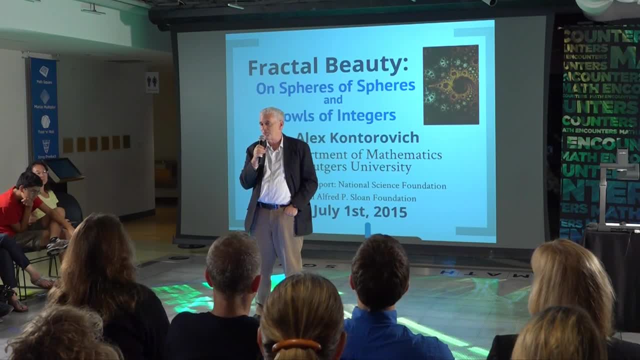 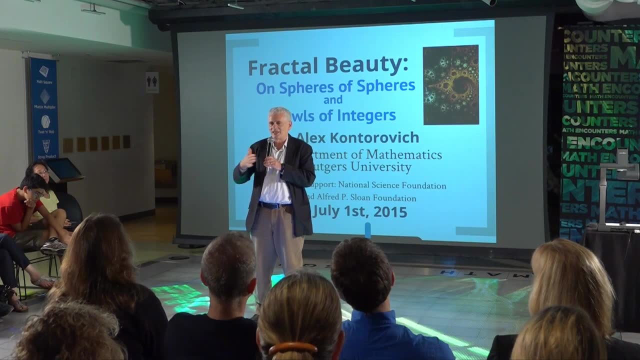 But the type of quotient that Alex wants me to talk about is a geometric quotient. So I take this infinite line and I divide it by all the infinite days, And when I'm on this ship, I'm going to have infinite days And I'm going to have infinite days. 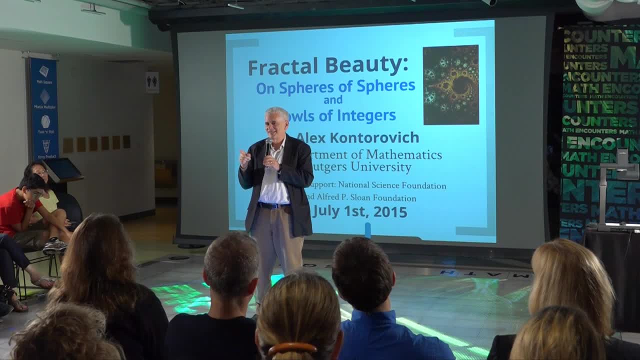 And when I'm on this ship, I'm going to have infinite days. And when I'm on this ship, I'm going to have infinite days And what I'm left with is a circle. It's like a clock. If you look at the clock, you 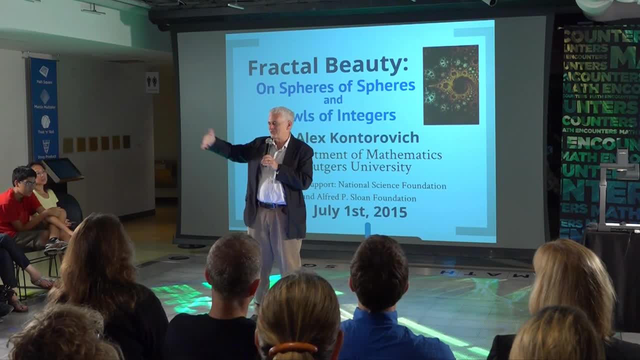 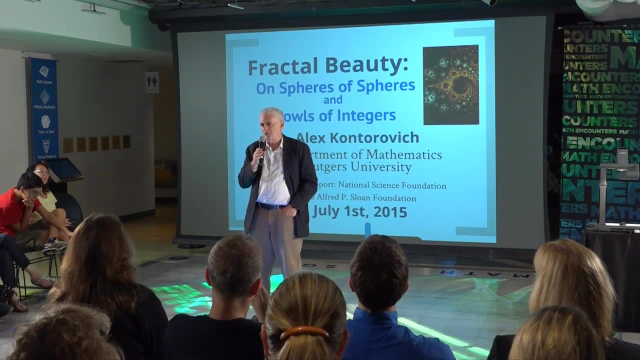 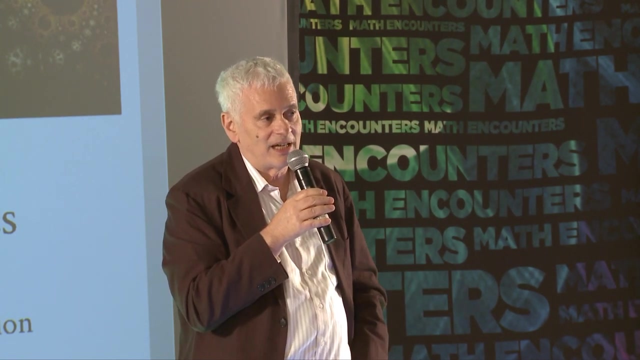 can see what time it is And the clock sort of treats all days as the same. You're quotienting by all the possible days. So this is an example of a finite quotient, because the circle has a perimeter of length 2 pi times the radius, so it's a finite By volume or area I mean. 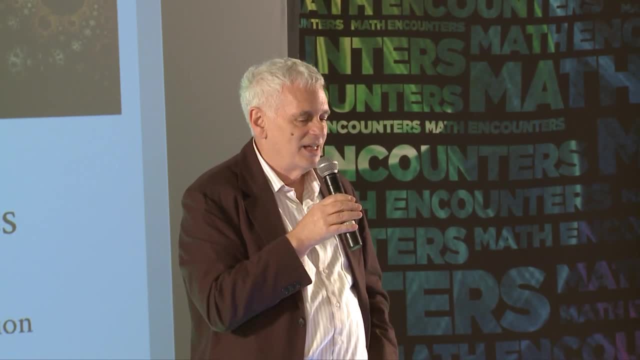 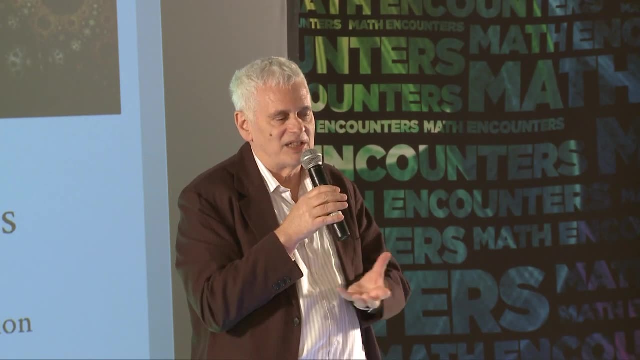 That's what I'm talking about: finite area or finite volume. Let me give you a more complicated example in two dimensions. If I take a two-dimensional plane, think of it like a piece of paper, except the paper has thickness- A two-dimensional 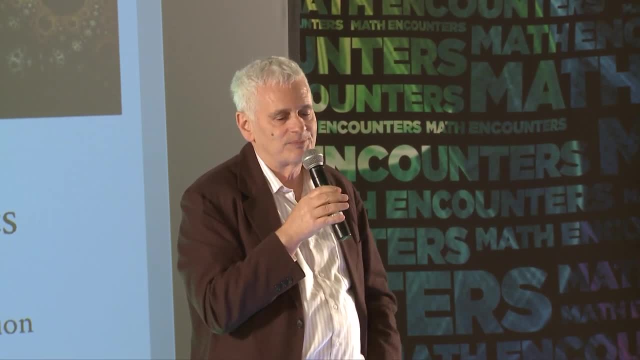 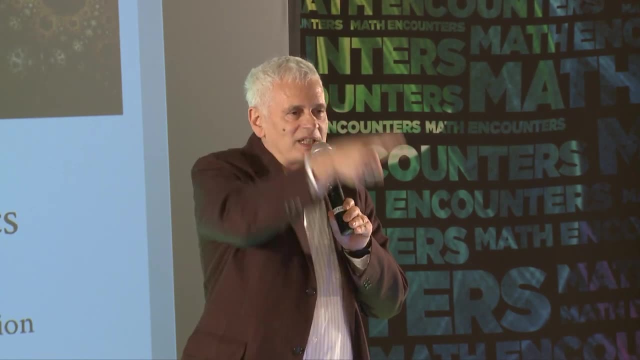 plane would have no thickness and it would be infinite in all directions. What I can do is I can take a quotient in one dimension and that's like wrapping the paper around itself and you get this infinite tube. Then, if you take a quotient in one dimension and you take the quotient in the other dimension, the tube would wrap around itself and you'd be left with something finite. It would be like a tire, just like a tire on a car which is mathematically called a torus, And it's again finite volume, finite area. 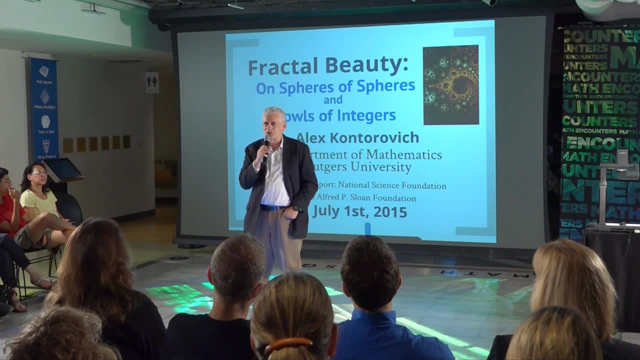 The type of quotients that Alex is using in his work is something much more complicated. First of all, the geometric space is a hyperbolic space And it's in many dimensions. It's not just one or two dimensions, It's higher dimensional. 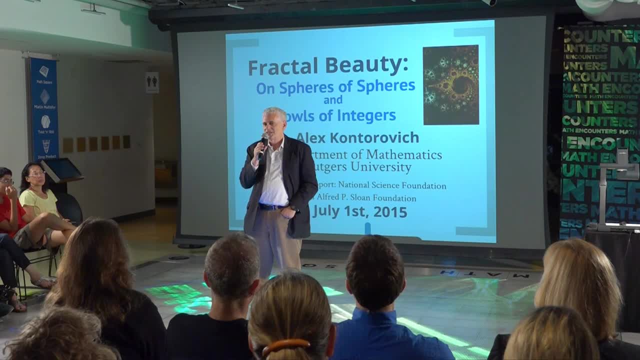 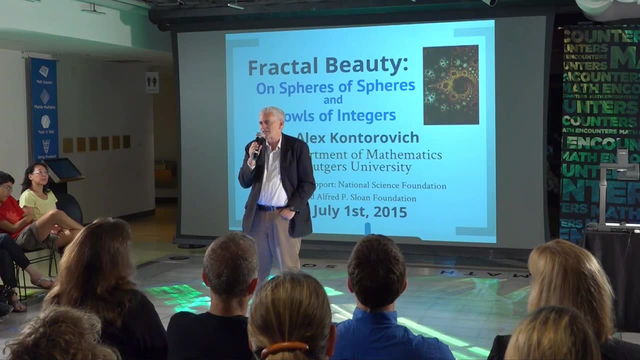 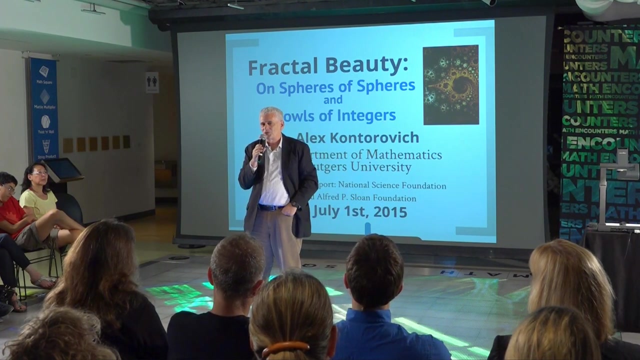 And it's a hyperbolic space. That means everything is weird. The Euclidean axioms all break down. If you draw a triangle, the sum of the angles could be more or less than 180 degrees. If you have a line and a point, they could be infinitely many lines tangent. So everything. 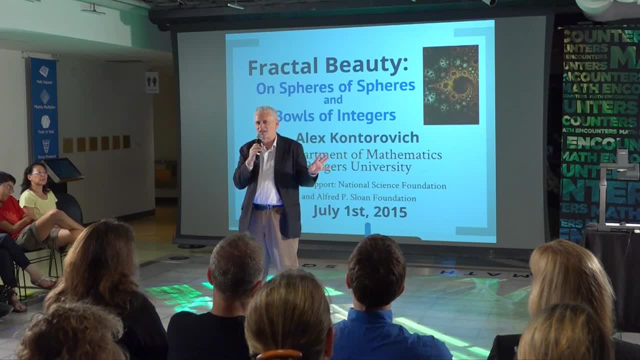 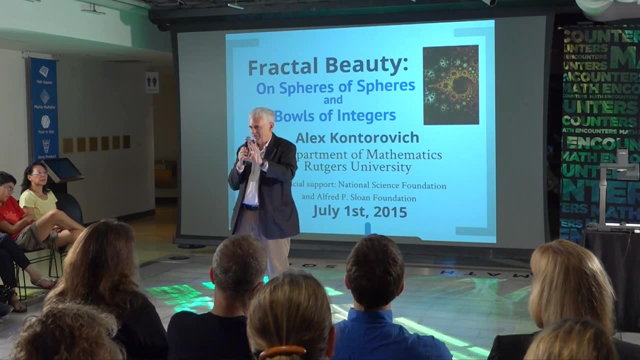 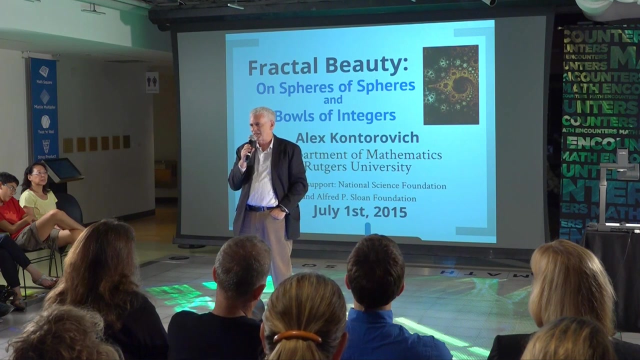 that we consider Euclidean and normal breaks down. So that's the first thing. Then he's taking a quotient by infinitely many things that are acting on this space and he's ending up with something of infinite volume, not finite volume. So it's a very 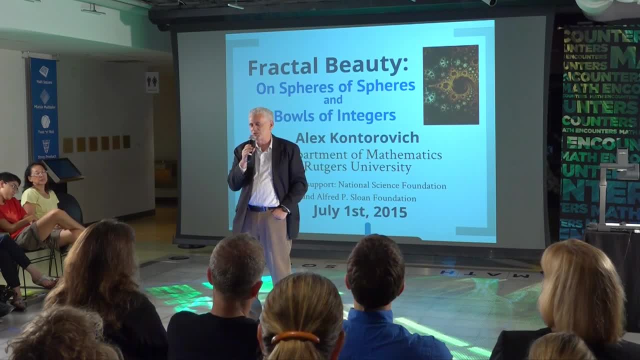 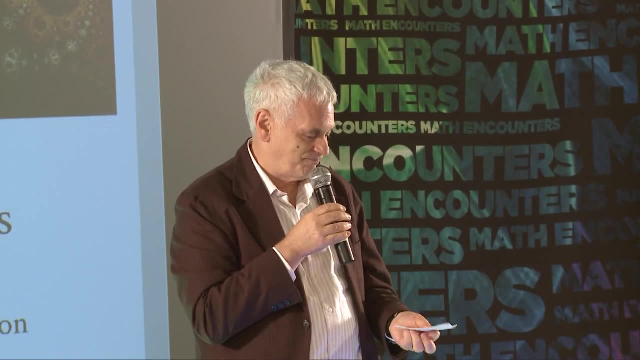 complicated thing, And the way to study it is using something called fractals. I don't want to say any more about fractals, because he's going to tell you all about that. Let me just end my brief introduction by telling you a little bit more about Alex. 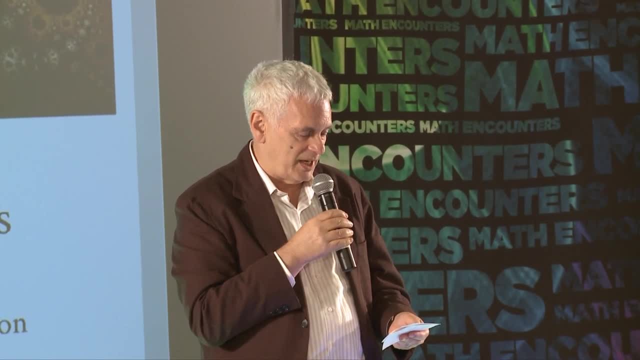 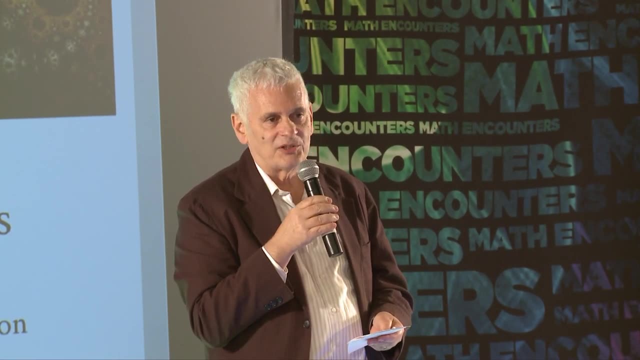 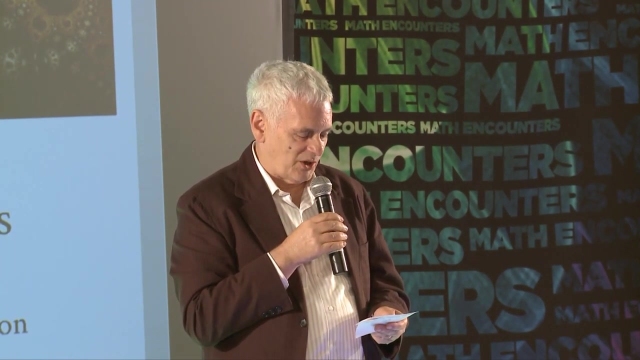 So he graduated in 2007,, and then he got a job at Brown for three years. After that he went to the Institute for Advanced Study for one year, Then he was at Yale for three years, Then he was at Stony Brook for a year and then back to the Institute for Advanced. 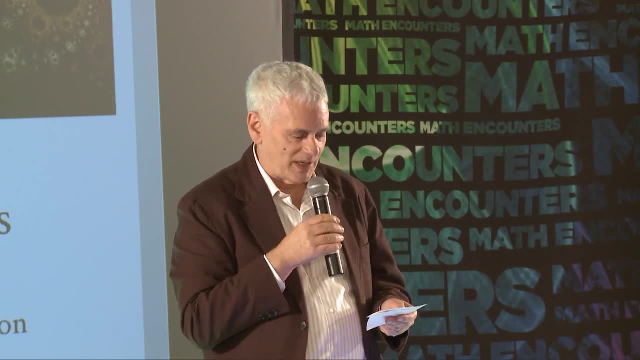 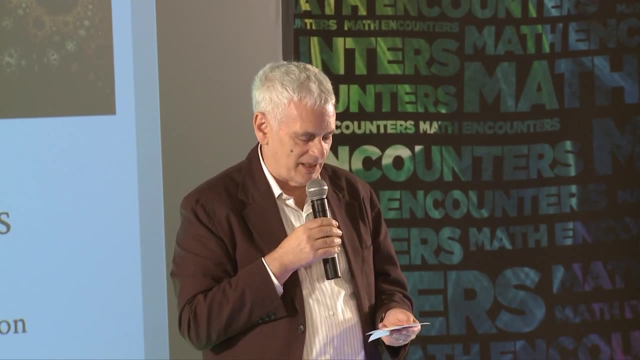 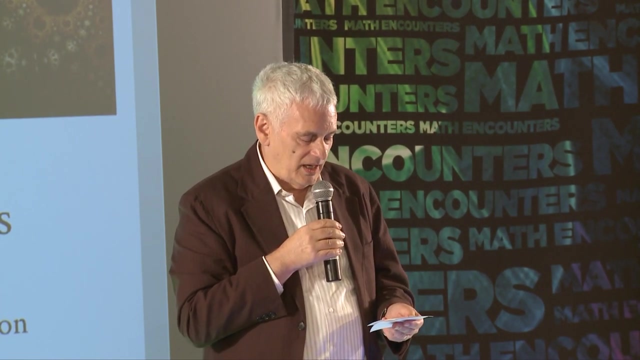 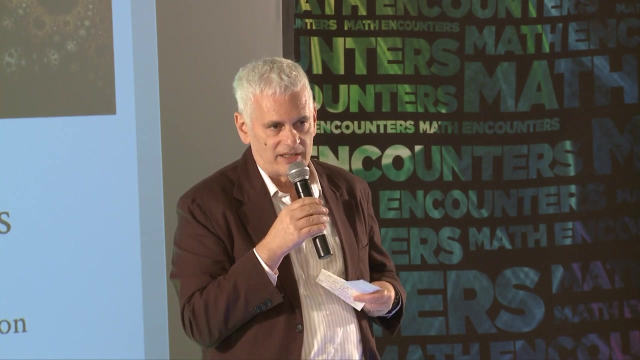 Studies And now he's a tenured associate professor at Rutgers. He's had visiting positions at that time At Columbia, AT Howe in Zurich and Harvard University. He won the Levi-Conan Prize, which is given by the American Mathematical Society for the 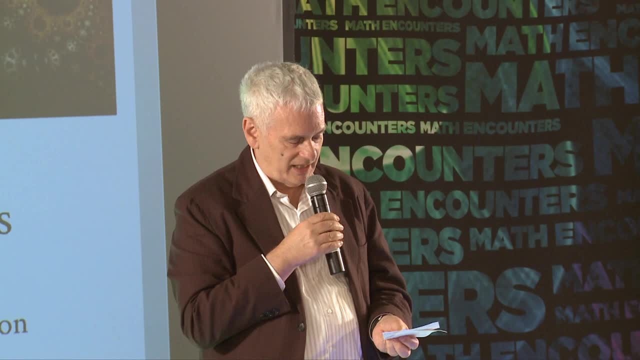 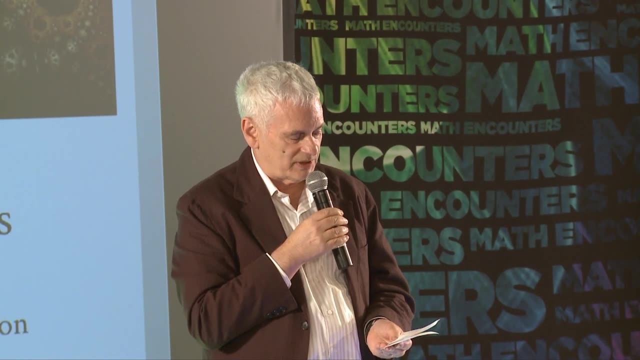 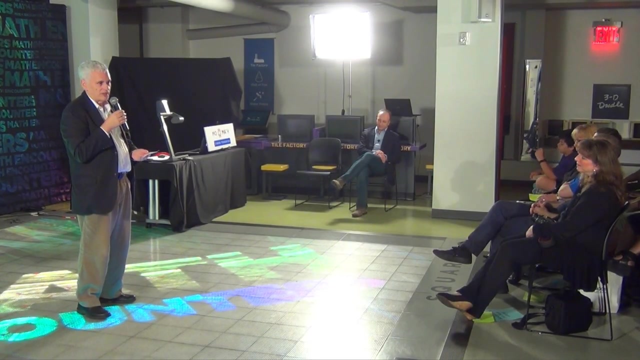 best expository paper, And the title of the paper is From Apollonius to Zaremba: Local Global Phenomenon in Thin Orbits, published in the Bulletin of the AMS 2014.. Let me just tell you what they wrote, why they gave him this prize. 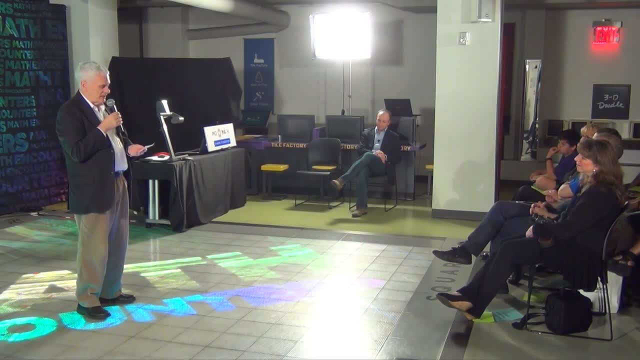 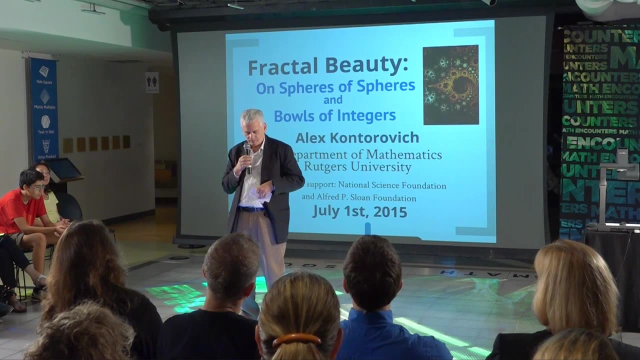 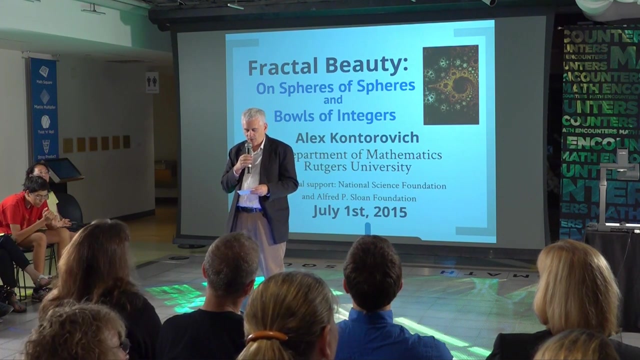 This paper introduces a new field of number theory that has proven to be extremely fruitful, even in shedding light on ancient problems. Let me conclude by telling you some non-mathematical things about Alex. So he is actually well-known in the music field. He plays the piano. He's playing the piano too, So he is in the music. 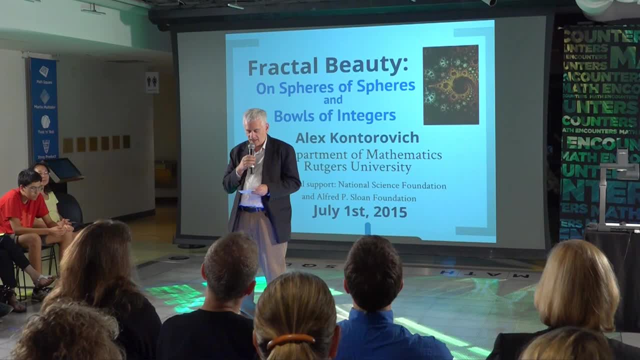 and he's a great pianist. He's a very good soloist and he's going to give you a few. He plays saxophone and clarinet and he was a member of two bands- Deep Minor and Klez Dispensers- for many years. In 2008,, Deep Minor was considered by Downbeat Magazine as Best of 2008.. Deep Minor was featured on Continental Airlines flights from 2008 to 2010.. It was on an off-Broadway production in 2011.. 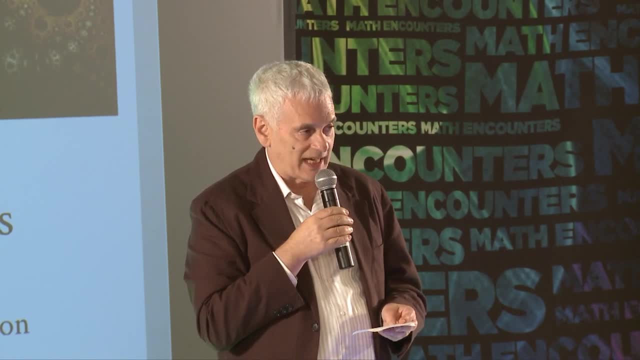 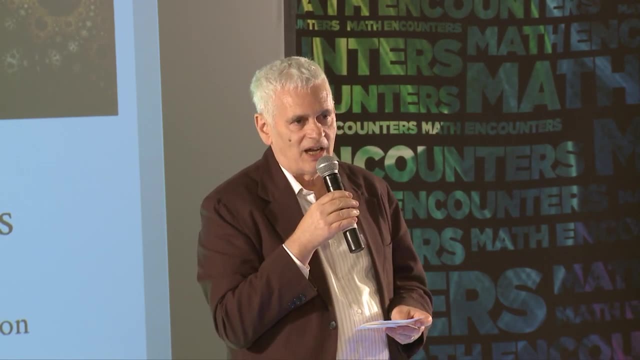 Alex was on the cover of Saxophone Journal in 2009, and he was interviewed in the journal. He told me once that he was going to give a concert and there would be 10,000 people in the audience and he was nervous. 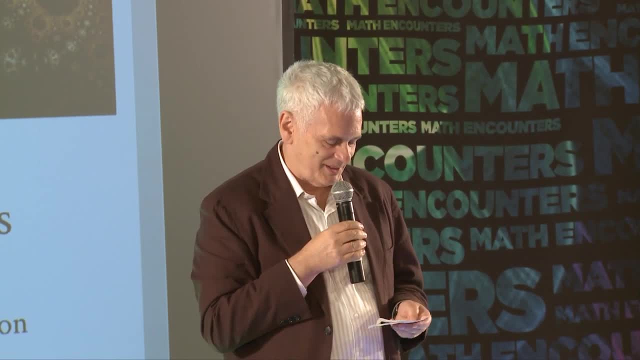 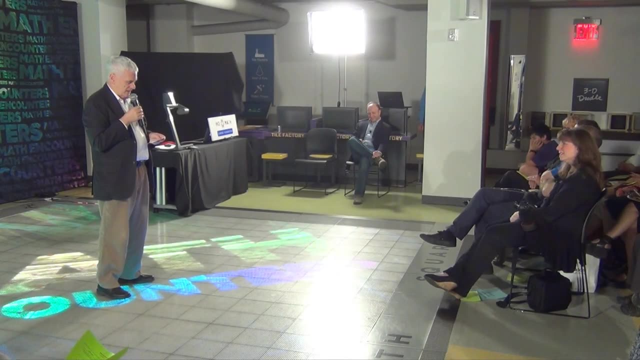 Let me just finish by one other non-mathematical ability that Alex has. He has a third-degree black belt in Kung Fu. He's the founder and instructor of Soft Tiger Kung Fu School in Princeton in 2002.. He started a similar Kung Fu school in Columbia in 2004 to 2007, and when he was at Yale he also started the same Kung Fu school. 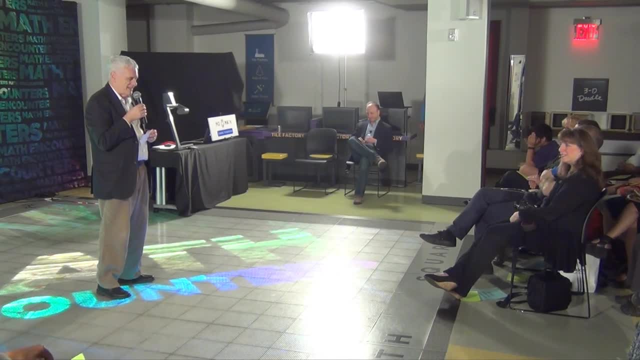 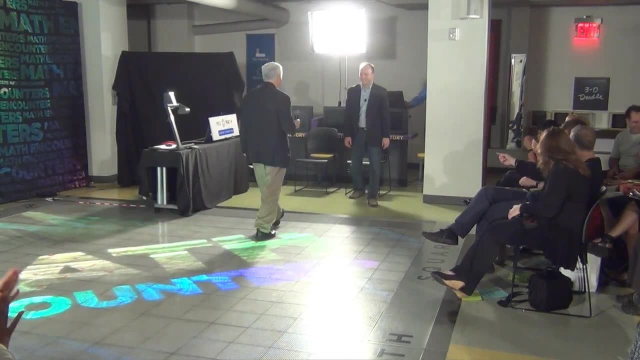 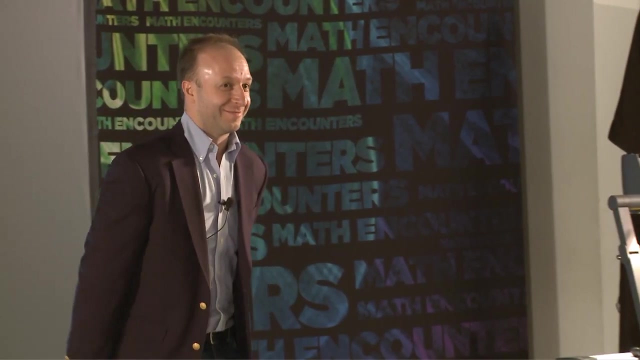 Anyway, I'm very proud of him and he's a great mathematician and you're in for a real treat. Thank you so much, Dorian. It's an honor to be introduced by you. I learned so much from you, and thank you all for coming. 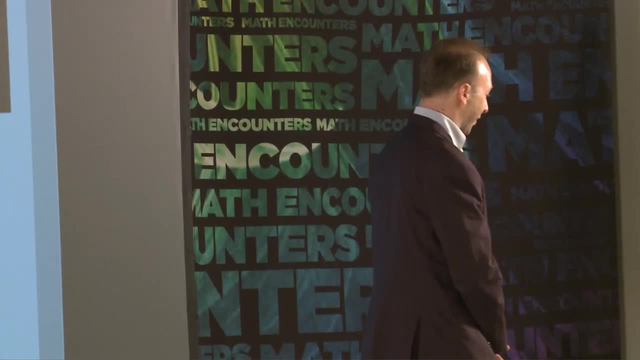 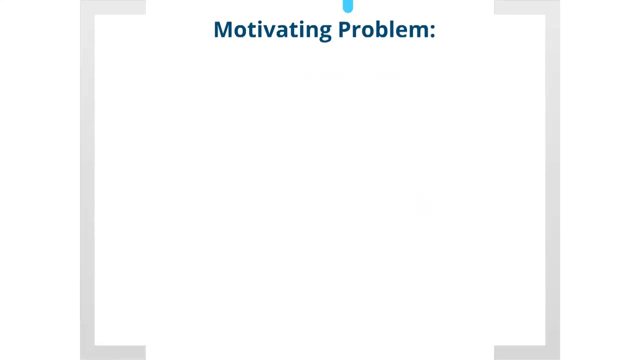 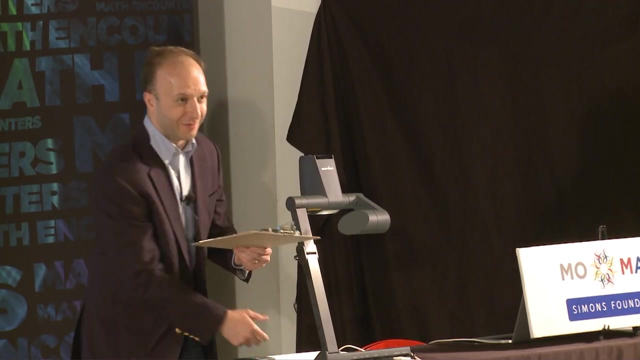 Thank you to Cindy Lawrence and Glenn Whitney for having me here, the opportunity to be here in front of all of you. So let's get started. You all have—let's motivate what we're talking about by pulling out—most of you have this, not everybody. 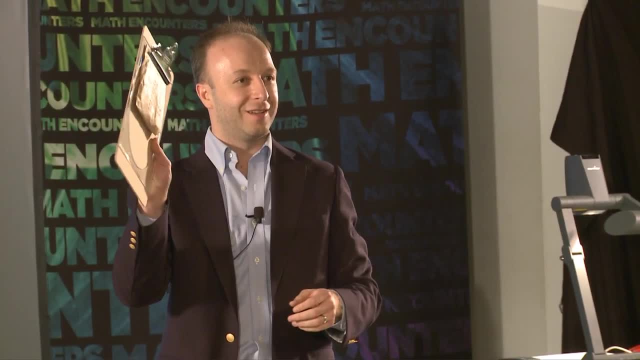 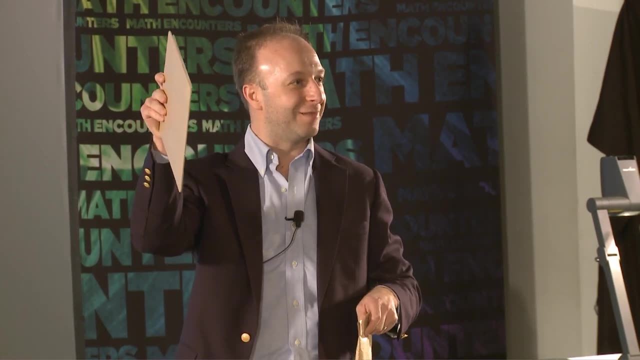 If you don't have one. someone nearby Has a little packet like this with a bag and a clip-on. Does everybody see something like that? Introduce yourself to your neighbor. if you don't have one yourself, You'll need their help. 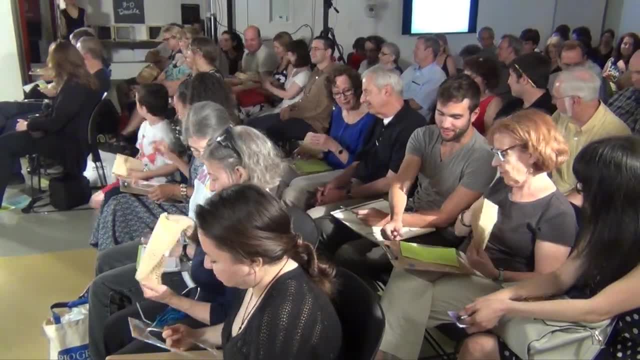 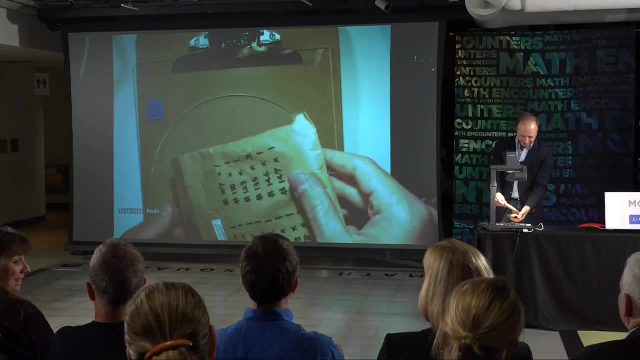 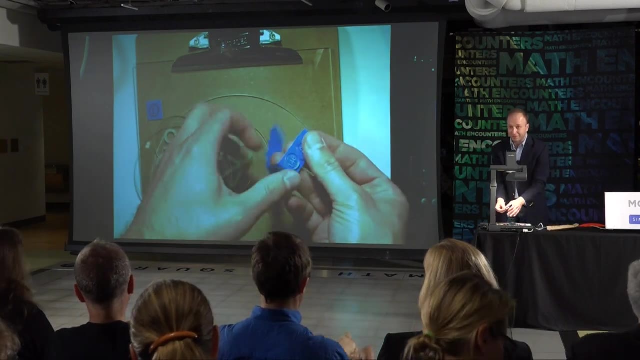 They'll need your help. Okay, so you take out this baggie, Let's see. So you take your baggie and you'll see. when you look inside a bunch of circles, Discs, There's some really little ones, so that you don't lose them. 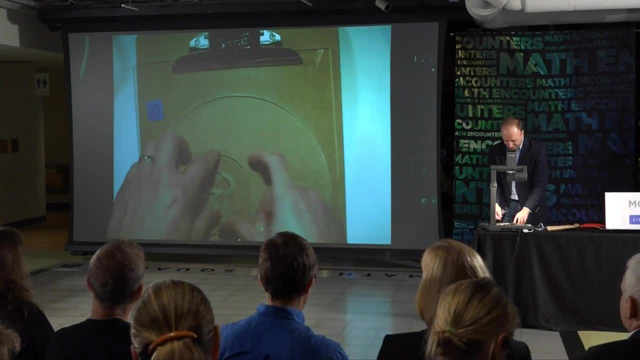 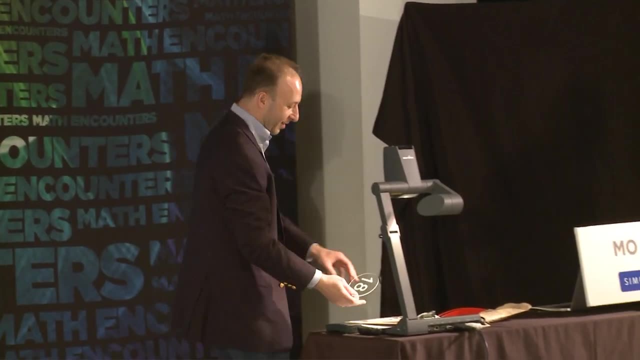 They're taped together but you can just take off the tape. So first you find the disc that looks like this: It's got a number 18 on it. Okay, Everybody got their number 18 disc, So put that one somewhere over here near the bottom. 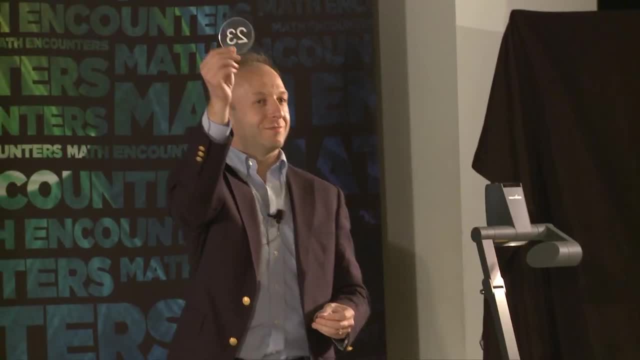 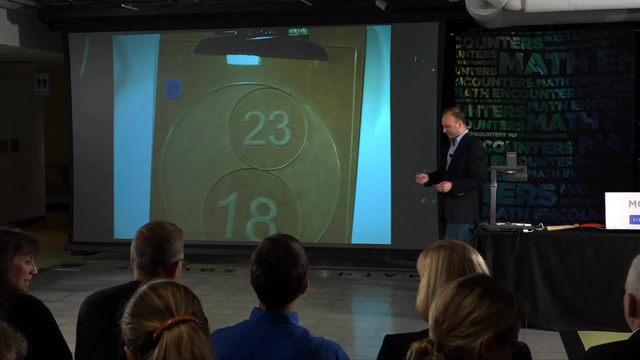 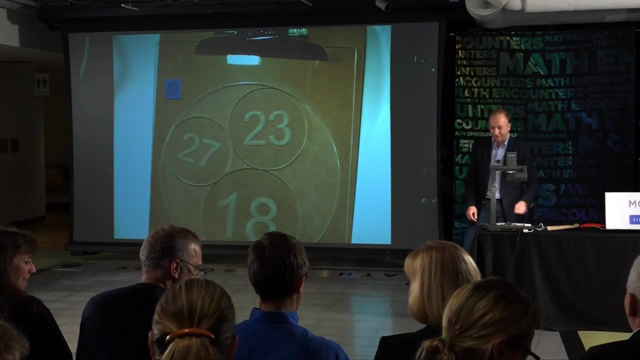 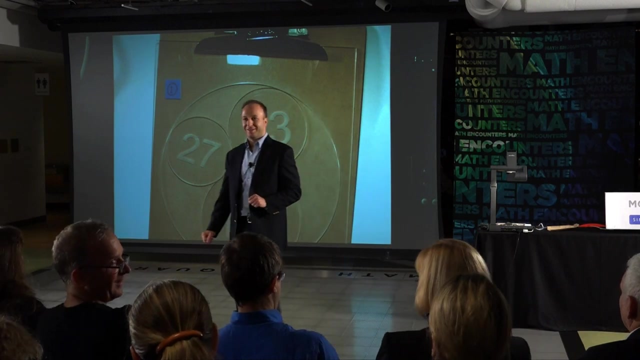 Okay, Then you have this number 23 labeled disc. Put that one somewhere next to it. They should just click together in the right place- And then put this 27 disc, which should perfectly fit inside the other three. Okay, Everybody there so far. 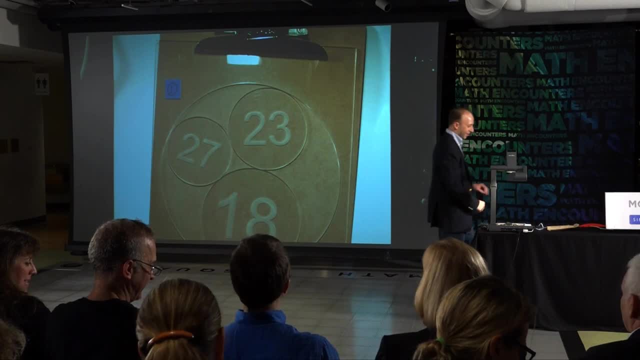 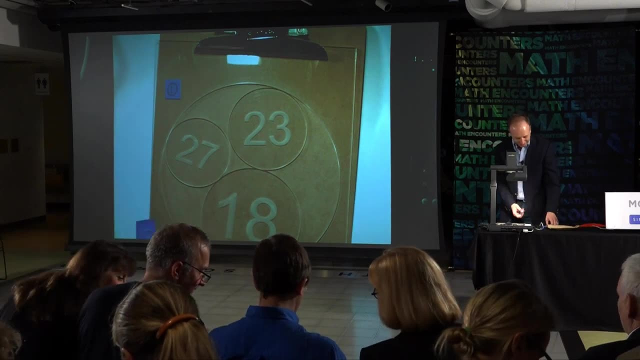 So here's your task: Find a disc that fits perfectly into that little triangle out of these- So it's not going to be these big guys, It's going to be one of these smaller ones- And see if you can figure out which one fits. 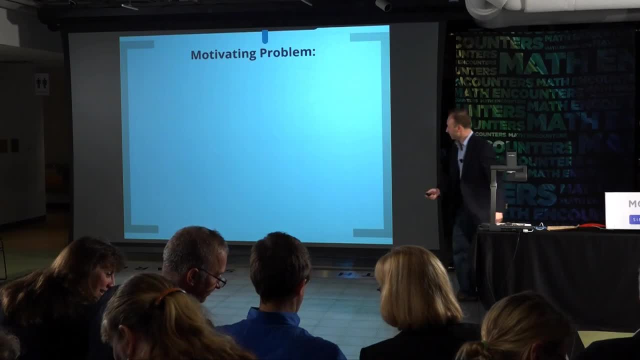 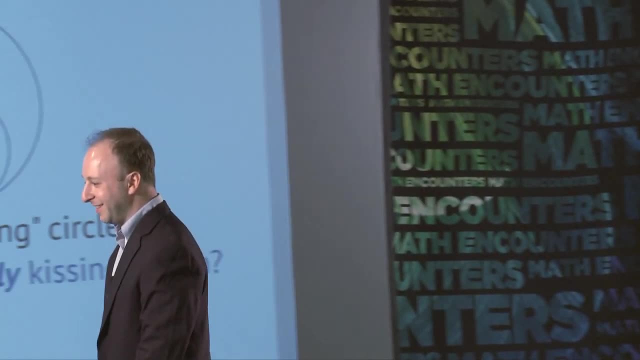 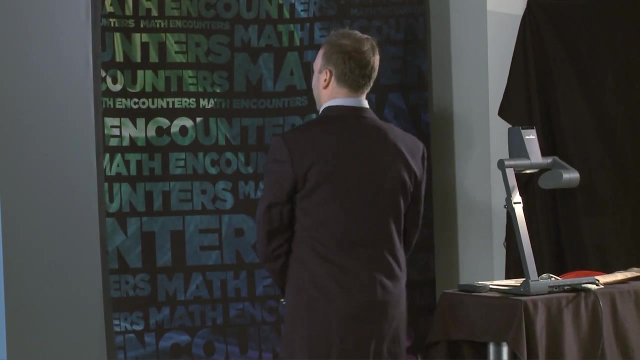 See which one it is, And I won't show you what I'm doing. You got one, Okay, All right, Good job. Okay, Let's see. So what's the motivating problem? We have our three discs, one labeled 18,, 23, and 27.. 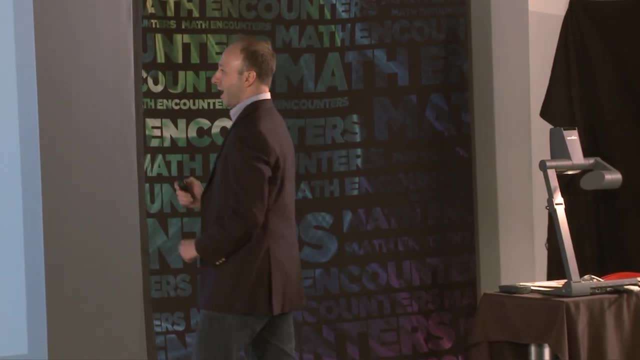 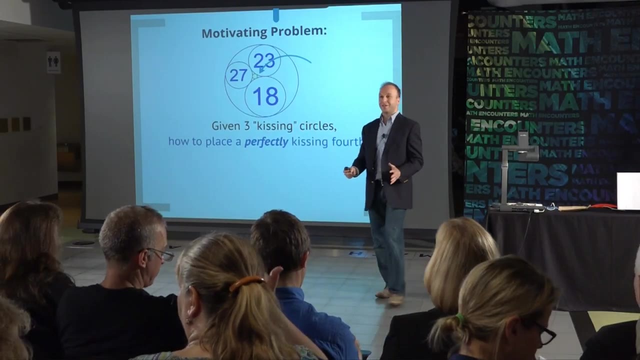 Those are three kissing circles, if you like. They're exactly tangent And our goal was to place a perfect one, So we're basically kissing fourth disc And most of you have done it now. Everyone's done it Okay. So let's see. 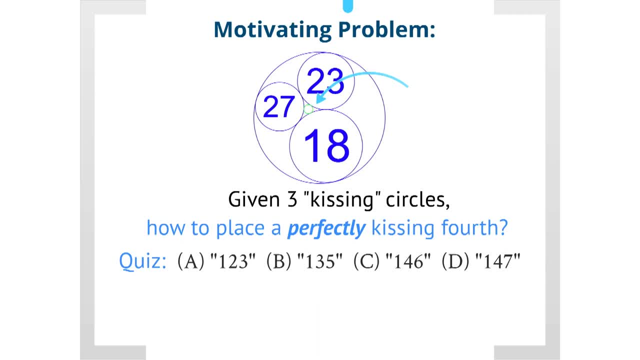 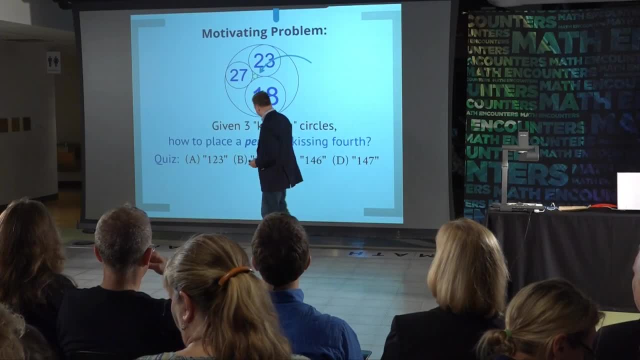 How about a quiz? You didn't know there was a quiz, So which disc did you end up placing? So how many people got the disc labeled 123 to fit in there? Interesting Nobody. Okay. How about 135?? One, two, three, four. 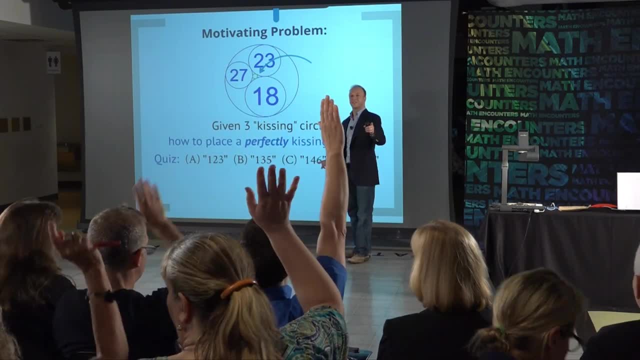 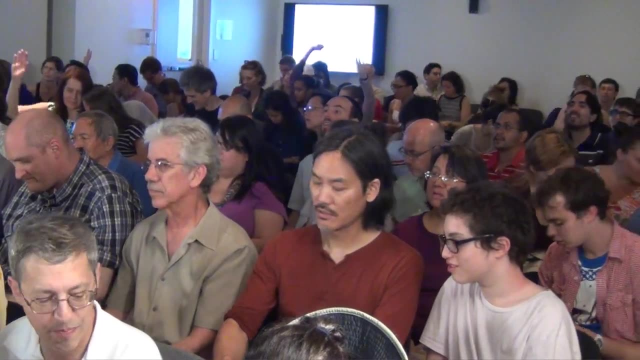 A handful, All right. How about 146?? One, two, Okay, Quite a number of you. How about 147?? Yeah, Another handful. One, two, three, four, Okay. So quite a number of you Interesting. 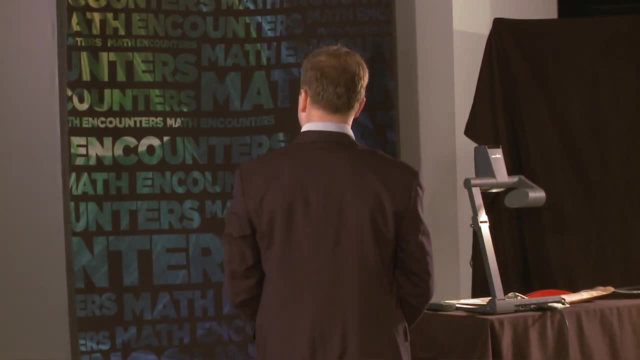 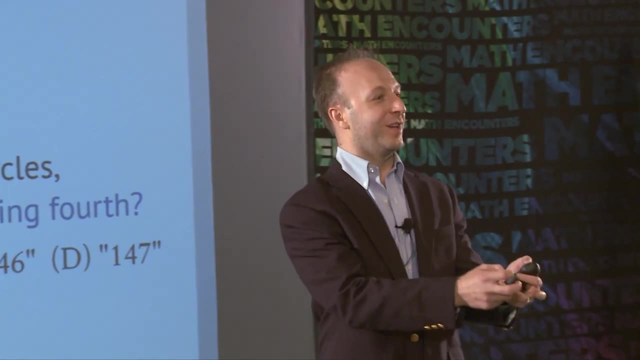 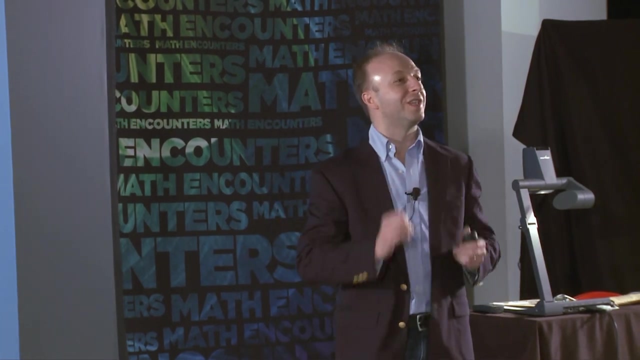 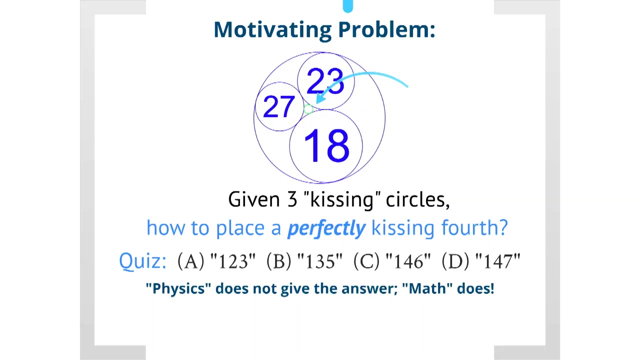 Interesting. You see, what's going on is. what you're doing is physics. You have a physical disc in your hands. Each one has some small rounding error And there's some ambiguity about what's the perfect disc that fits just right. What the question is asking about is about perfect circles, perfect discs. 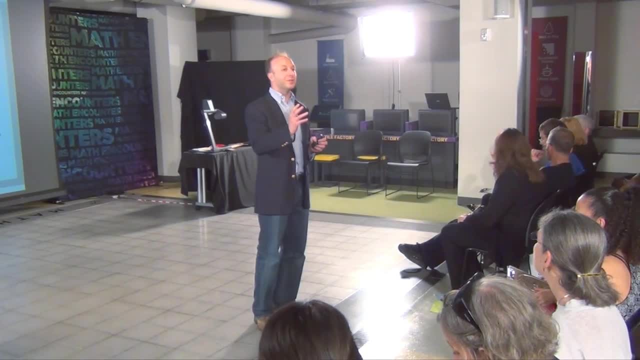 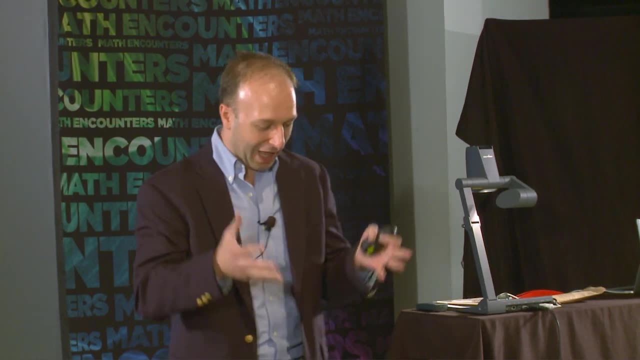 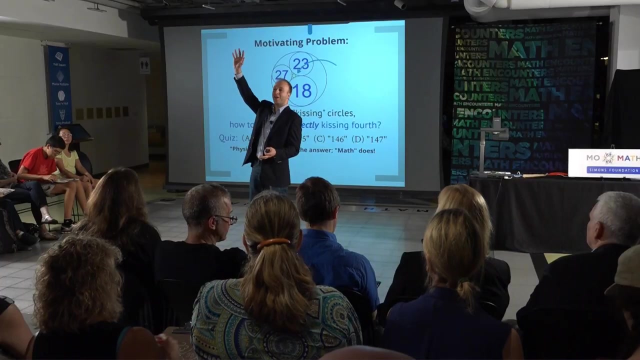 And this is something that does not exist in this world. So the difference between physics, one difference between physics, science in general, which tries to describe the world, and mathematics. Plato liked to say: any object that we, as human beings, experience on this earth is an object which is the shadow of an ideal object in 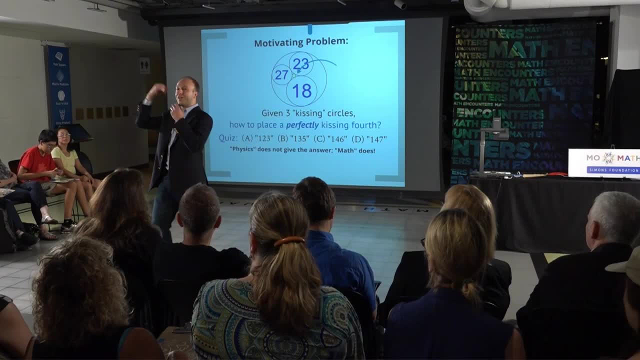 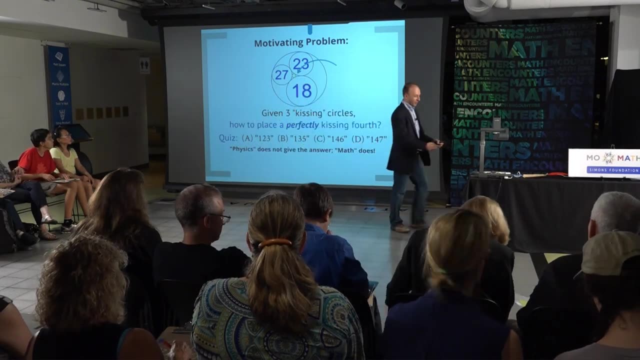 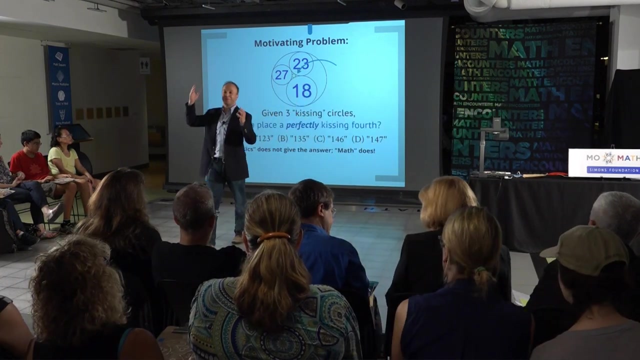 heaven that we can't see, But we just get glimmers of through our life experiences. So what we have is the glimmer of a life experience. We have our life experience, which is what discs we saw, And there's an ideal which only exists in our mind or in heaven, if you're Plato. 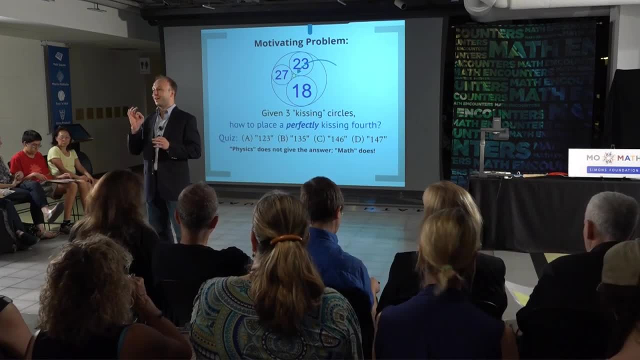 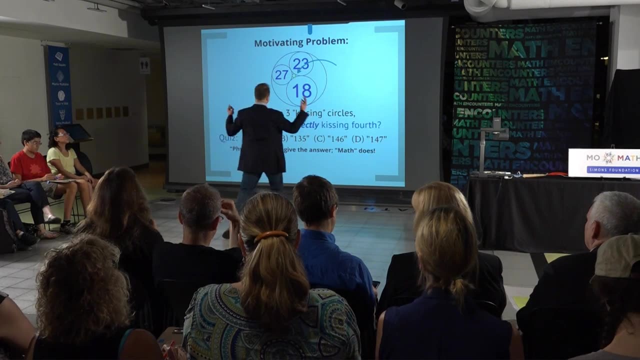 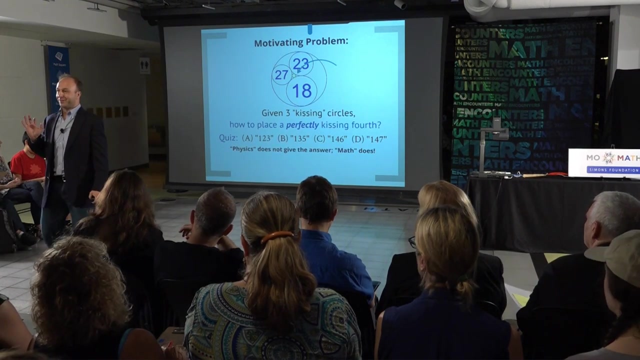 But there's nowhere else that this perfect disc that just fits there exists, except in the ideal world of mathematics. So, mathematics, you try to study this. it's not a religion or something, but you know, you have this idealized version of life and that is all you're interested in. 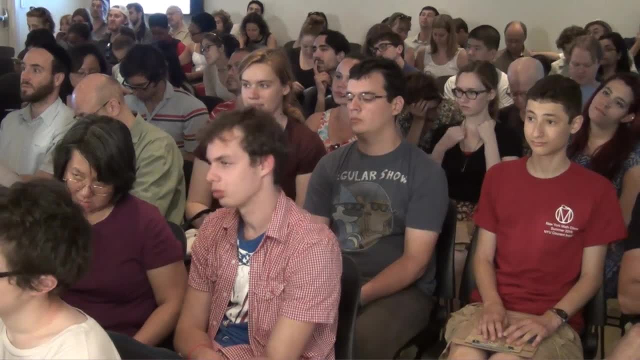 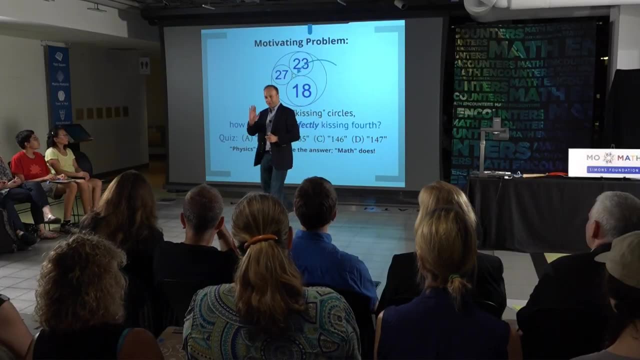 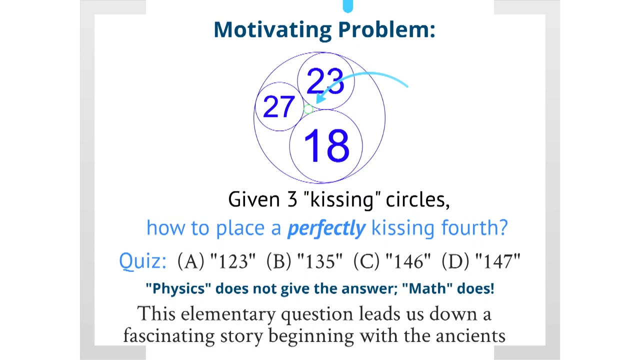 Because anything beyond that is science, physics, engineering and so on. So we couldn't get a straight answer experimentally. We'll get one mathematically And in fact this very simple elementary question will lead us down what I hope you will find. 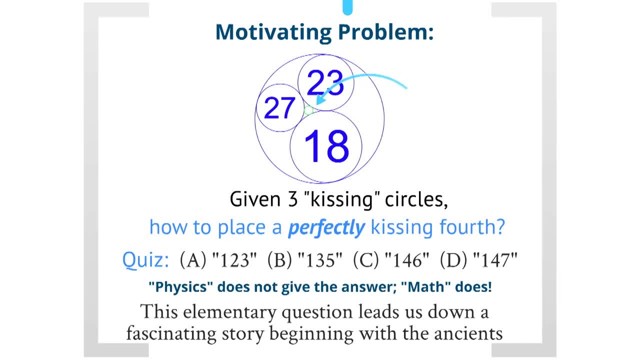 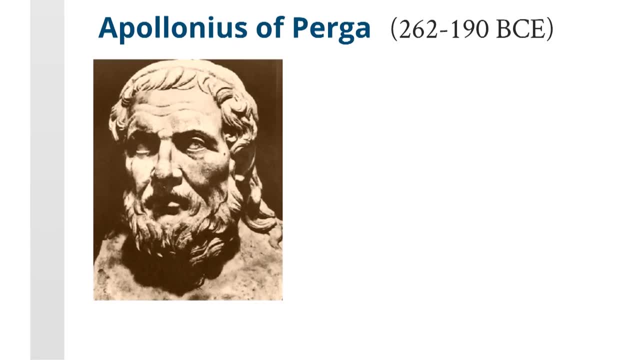 is a fascinating story that begins all the way with the ancients, So let's go back about 2,000 and something years To this gentleman. How many of you have seen this guy walking around? That's, I'm sure, nothing. Wikipedia says that's what he looks like. 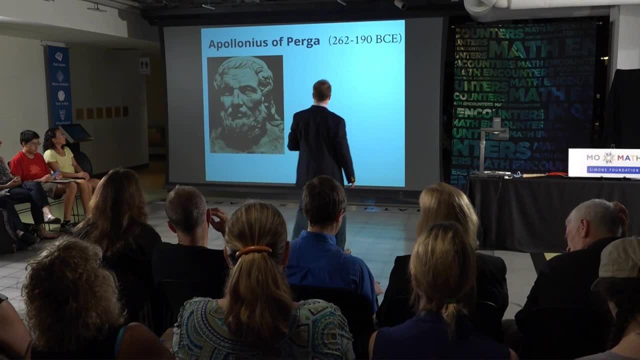 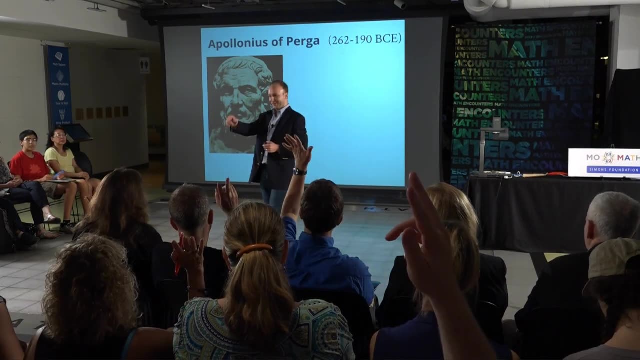 Nobody knows what he looked like. So this is Apollonius. the ancient Apollonius of Perga lived about 250 BC And have people heard of him before A handful. Really, You've heard him before. 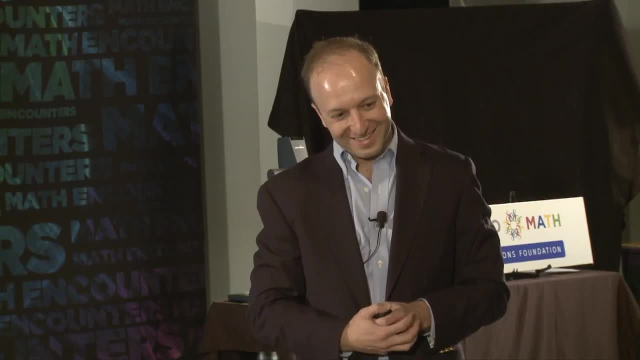 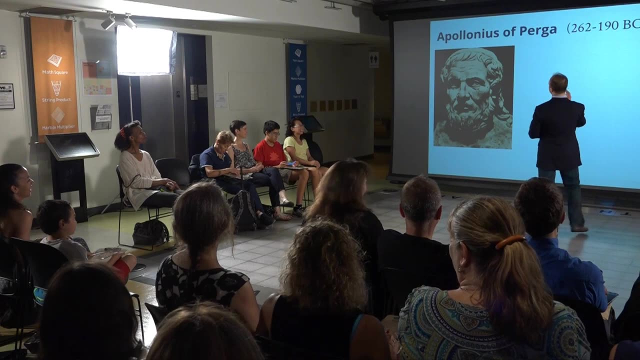 Yeah, What do you know about him? Okay, Yeah, That's what I asked. Did you hear about him? Yeah, Okay. Well, the thing that he's probably best known for is a work of his called conics, where he treats conic sections. 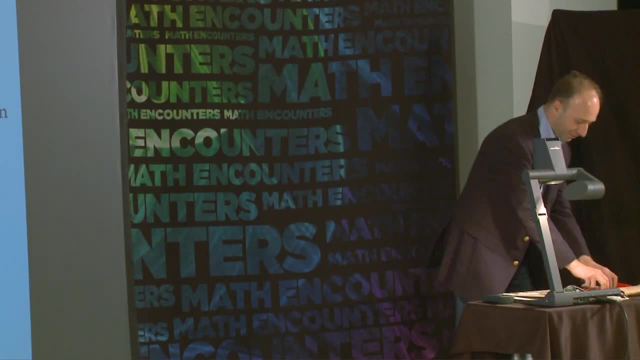 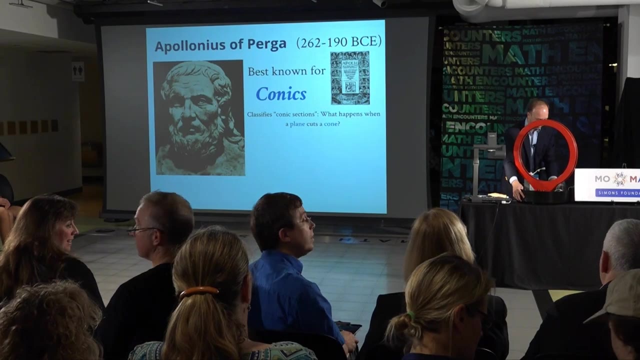 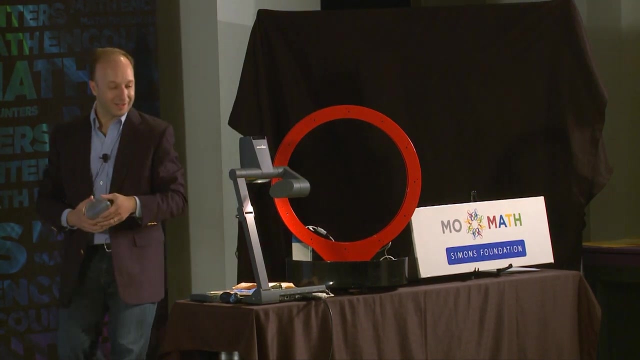 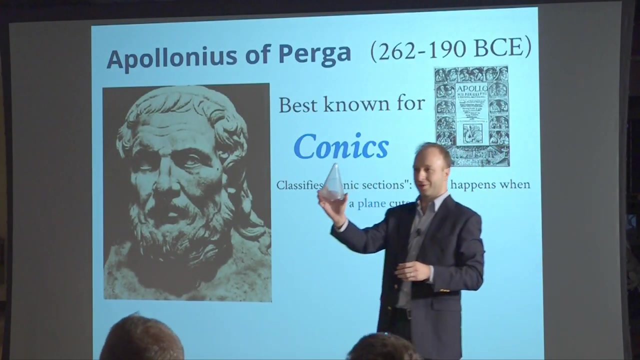 So let me explain to you what I mean by a conic section. So this is called the ring of fire. You'll see why in a second. Can I lower this a little bit? Okay, This is a cone, It's a cone. 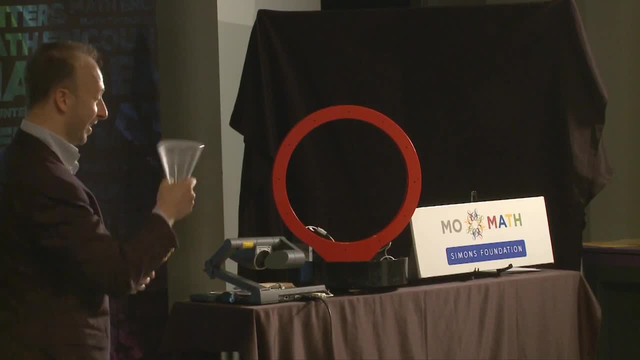 You know what an ice cream cone? right, You've had an ice cream cone. Okay, This is a cone Again, it's a physical cone. It should be perfect. tip at the end: Okay, We can all live with that. 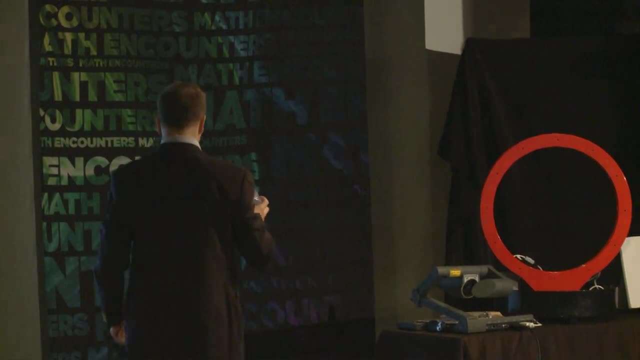 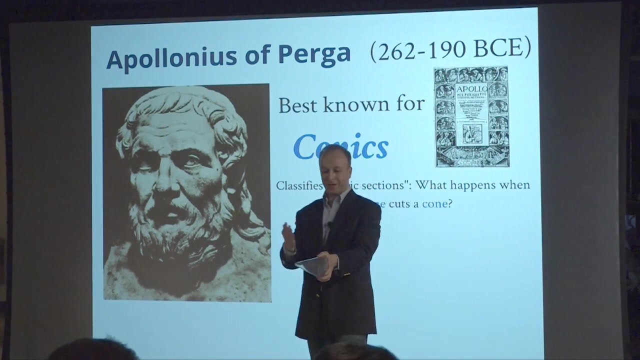 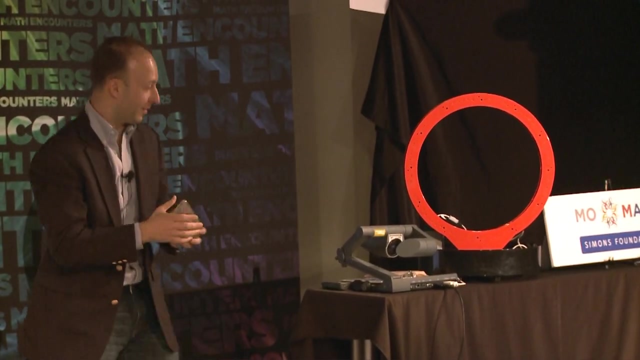 And this cone. what the? the problem that Apollonius was interested in is what happens if you take this cone and you take a samurai blade and you chop it at some angle. what do you get in the cross section of this cone? 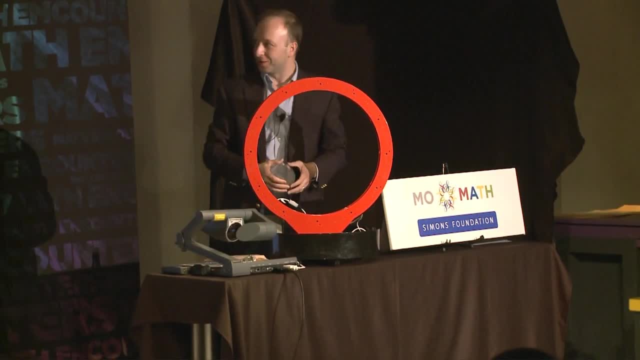 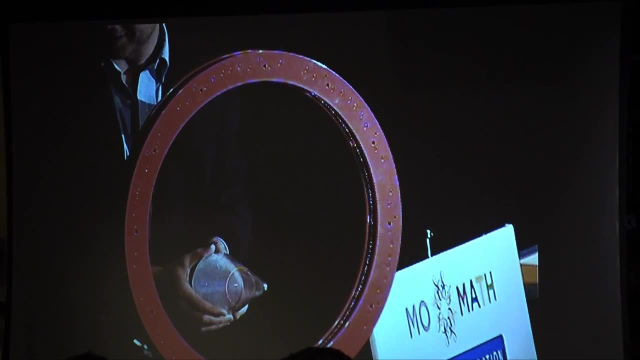 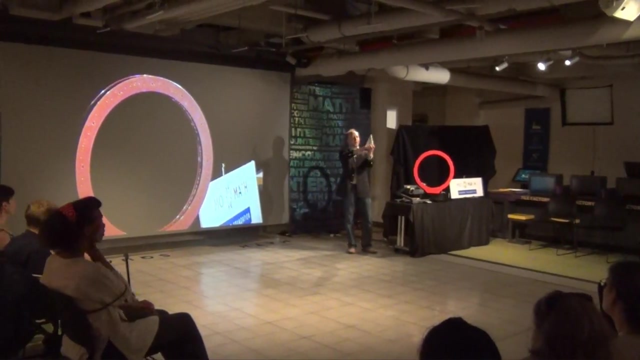 Okay, And so the So he gets. so he builds himself a laser and 3d prints a cone and he sees what the various cross sections are. I hope you can see. So if I, it's pretty clear. if I cut exactly a parallel to the base of the cone, I'll get. 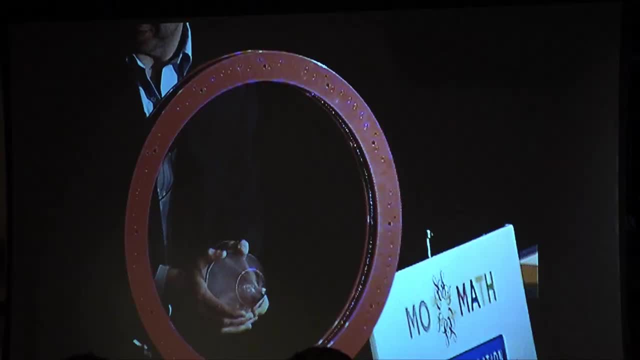 a circle, right? No surprise there. What if I twist just a little bit? Yes, So you guys know you get an ellipse. and if I twist so much that eventually I'm parallel, parallel to the edge of the cone, can you see that? you get a parabola. and if I twist, 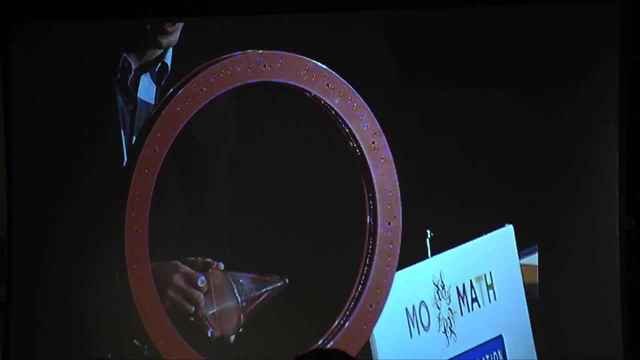 even a little bit more than that. that shape is called a hyperbola- a hyperbola exactly. So these are the conic sections, the sections of a cone, the cross sections. When a cone is sliced by a plane, what figures do you get at that slice, at that intersection? 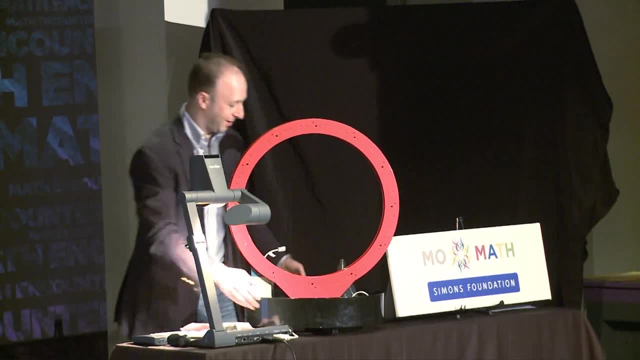 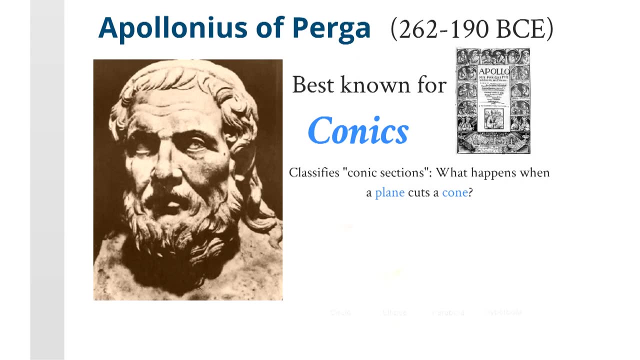 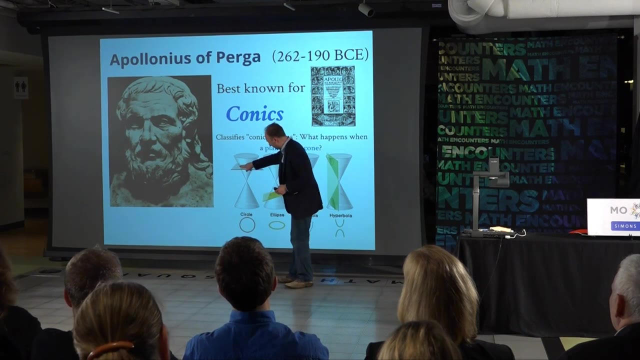 Okay, Now what do you get? Okay, This cross section. That's the problem. that's solved by Apollonius. So again we have our cone, and if you cut exactly this way, you see a circle. If you cut at an angle, you see an ellipse. 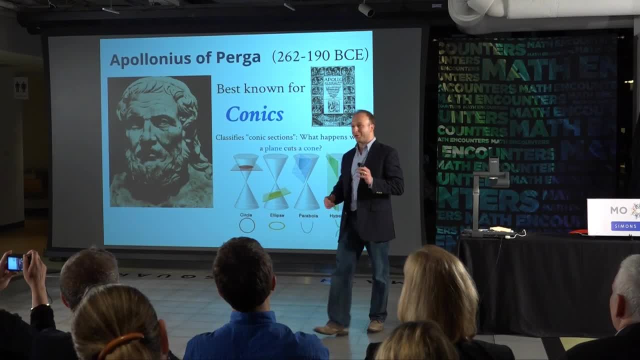 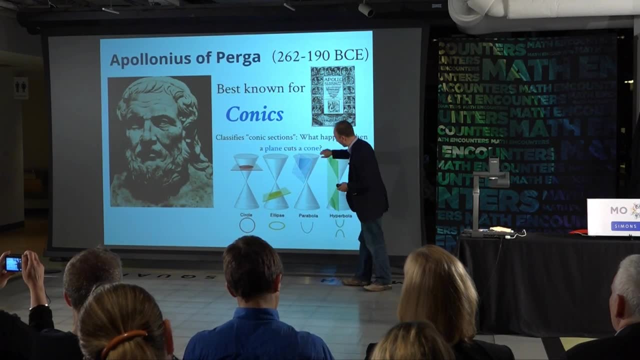 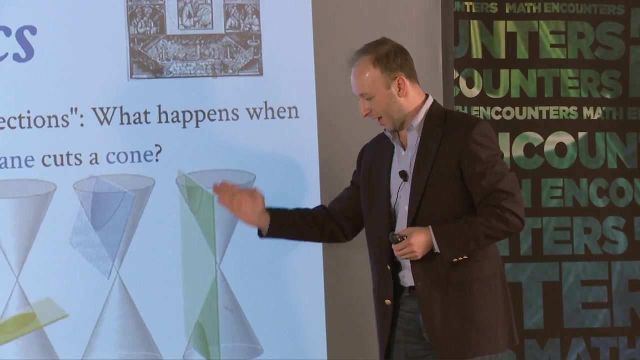 It's very hard, even even using our picture there, it's very hard a priori to distinguish between a parabola, the exact parabolic where you have, where the cut is parallel to the edge of the cone. Okay, So that's the conic section- versus hyper hyperbolic cross section. 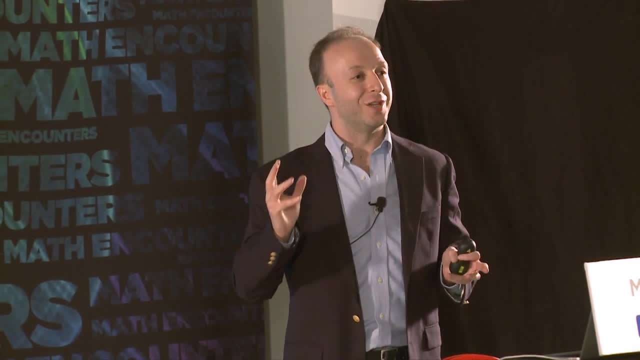 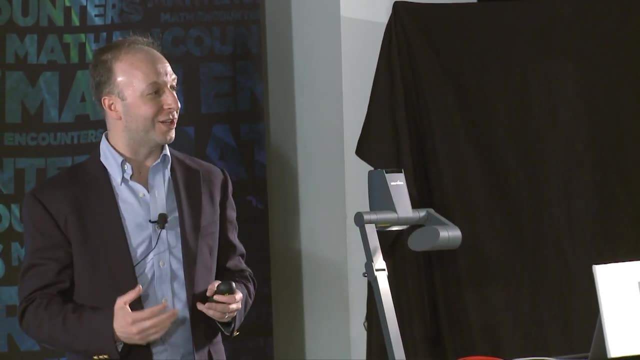 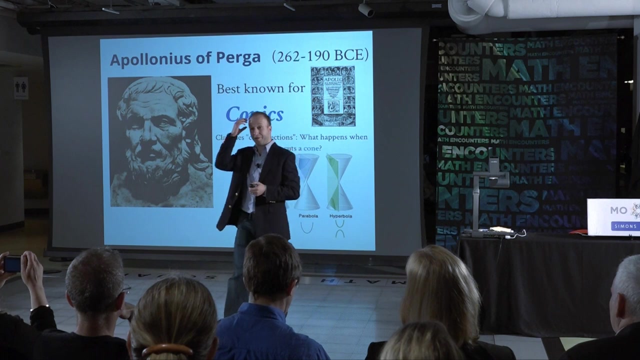 But anyway, using only his mind, Apollonius was able to work out exactly what these shapes are. In fact, he gave these names- ellipse, parabola, hyperbola- come from this classification, And this was an amazing feat of technical mastery of the mind and the ideal objects. 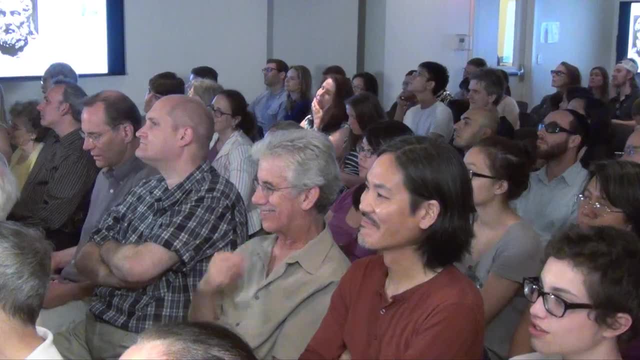 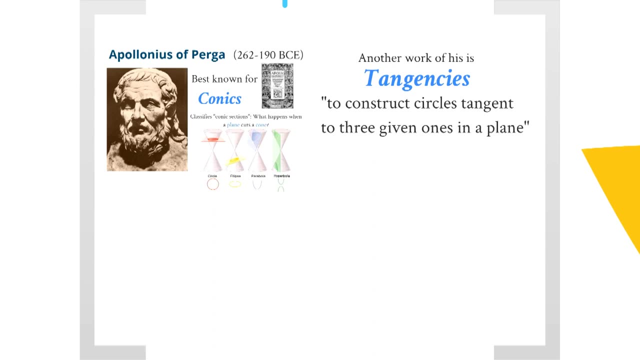 because obviously he didn't have the ring of fire and a laser beam. All right, Let's talk about tangencies, Something that is less well, this is kind of his most famous work, but another very famous work of his is called tangencies. 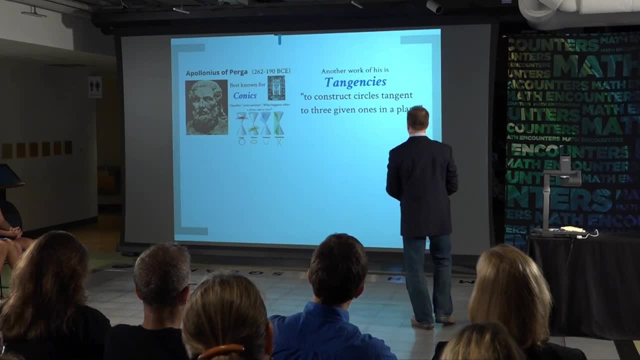 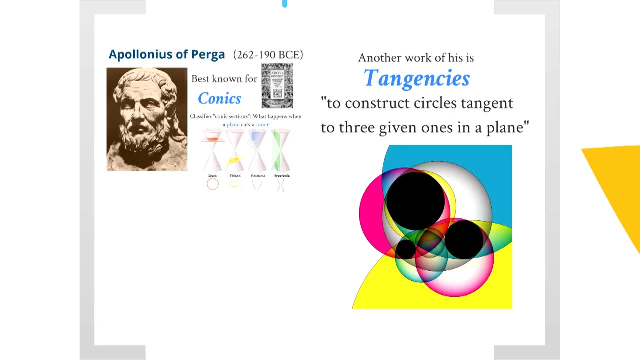 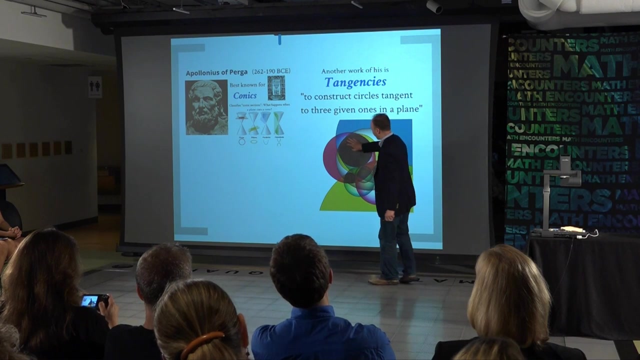 And in tangencies he solves the following problem: to construct circles tangent to three given ones in a plane. Okay, So what does that mean? You're given somebody- God, or your math teacher or me- somebody gives you three. maybe the devil gives you three. 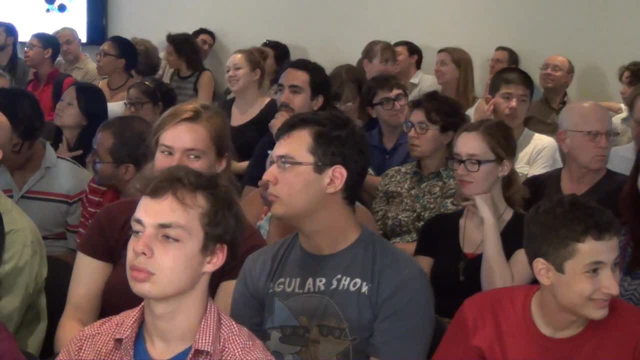 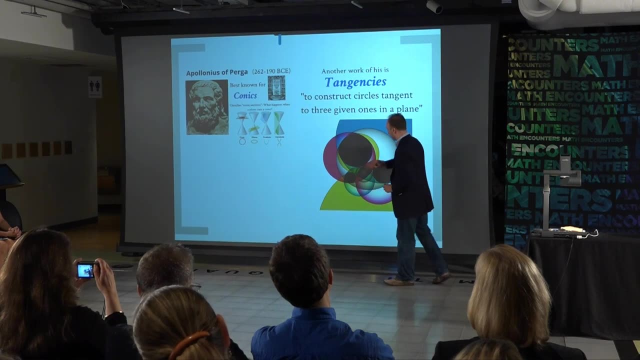 So the black circles are the ones that are forced on you, Okay, And you can find all the circles you can that are exactly, kissing, exactly tangent to the three given ones. So, for example, this is one solution to the Apollonian problem. 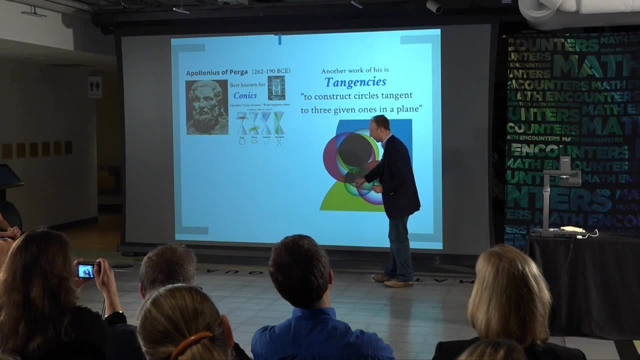 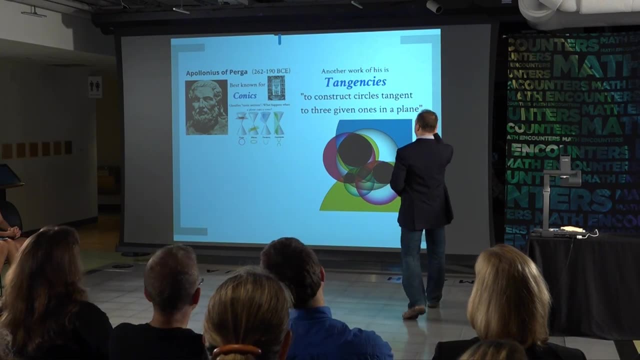 Here's another, and here's another, and so on, and you can trace around all the various solutions to the Apollonian problem. Okay, Now, what do I mean by construct? Obviously, you can just take your hand and doodle it, right. 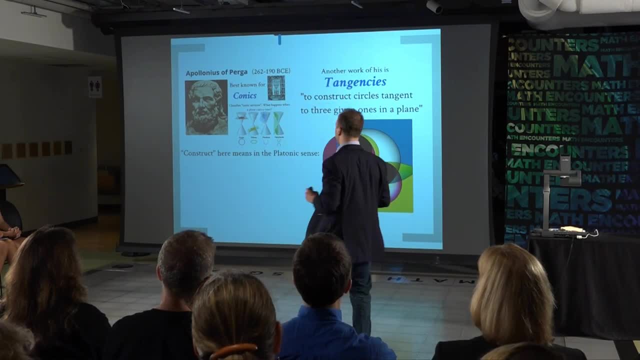 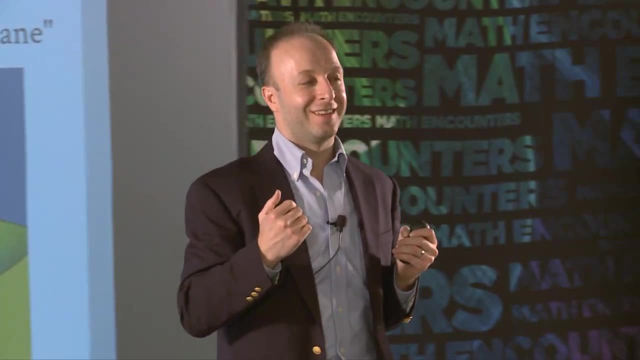 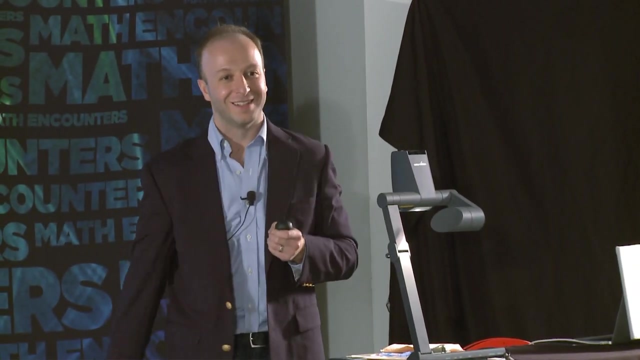 No construct is in the sense of Plato, in the sense of idealized world. Okay, So what does Plato believe exists in heaven as the tools of construction? Straight edge and compass right, The two things that are beaten over the heads of ninth graders in this right. 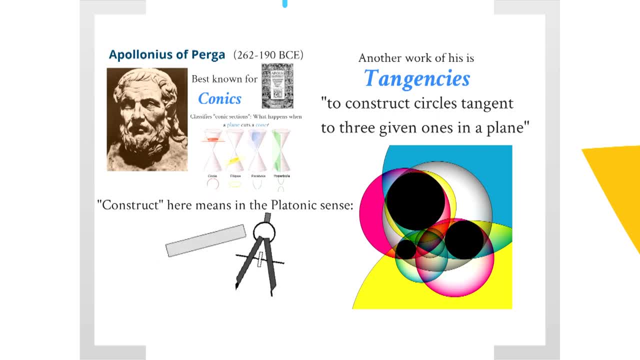 It's supposed to be something very beautiful and very. you're glimpsing God when you study straight edge and compass. I'm not sure that's how it's taught. So he gives this straight edge and compass construction. You have the ideal objects that you can create out of the ideal circles. 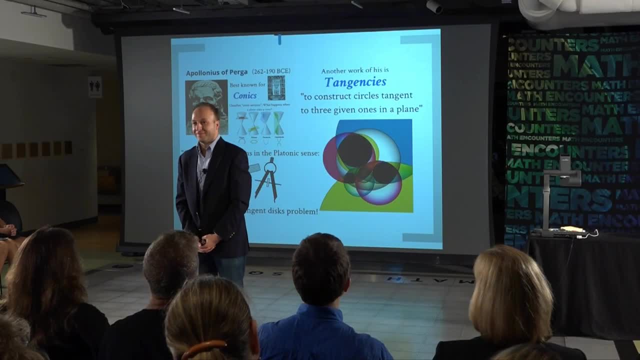 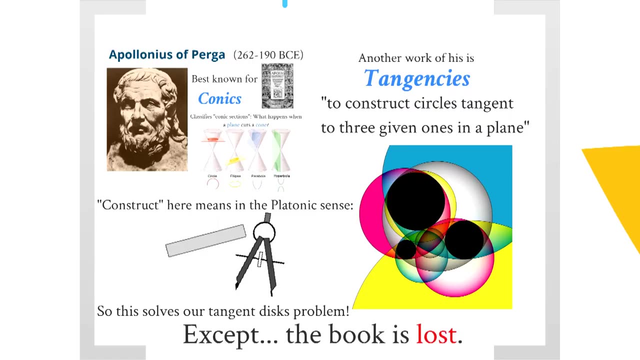 And so that solves our tangent disc problem. Thank you very much for your time. That's the catch. The catch is that the book is lost. So what do I mean by lost? How can a book be lost? We can imagine a book being lost. 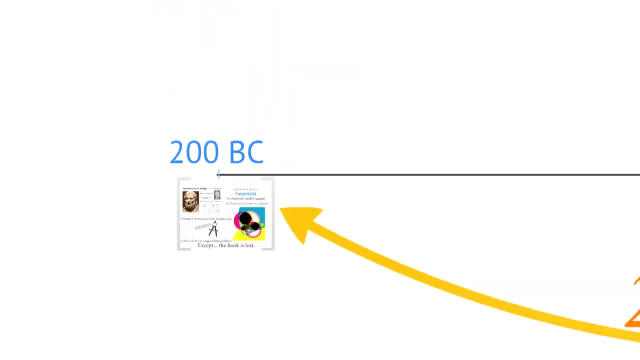 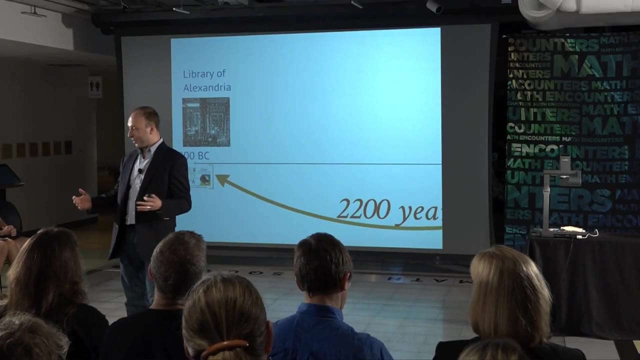 Why do we know about it if it was lost? So let's do a little cartoon history. Alexander the Great- maybe you've heard of him- conquers all kinds of lands, including North Africa. In Egypt He builds up a town. 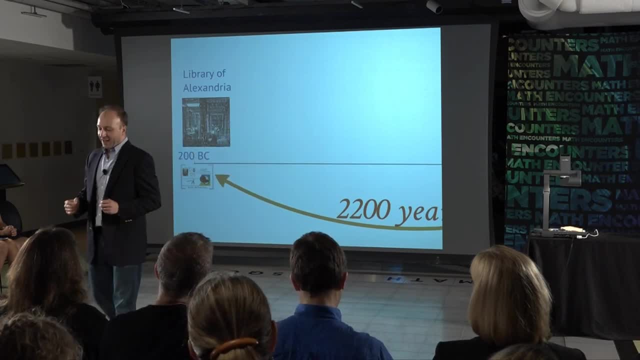 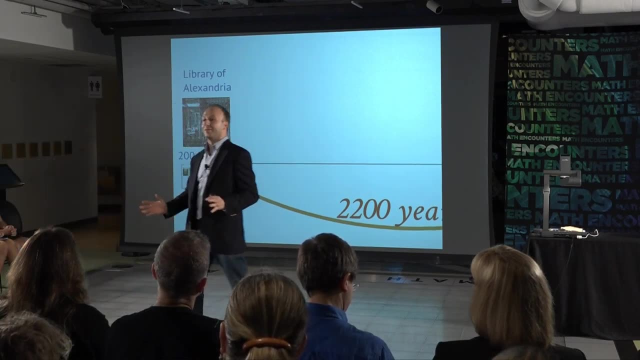 For some reason it's called Alexandria And in that town, he says, there will be a magnificent library which collects every single book known to mankind, And he creates it there, And for hundreds of years, like the Library of Congress, right. 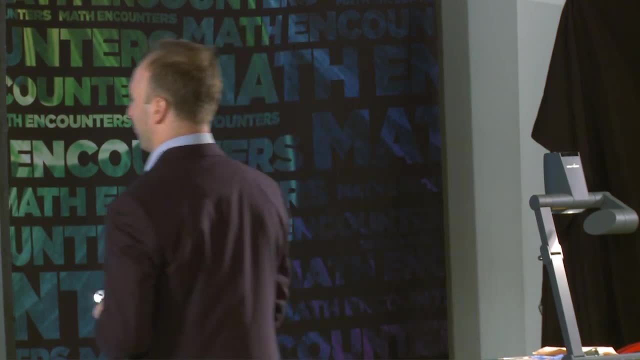 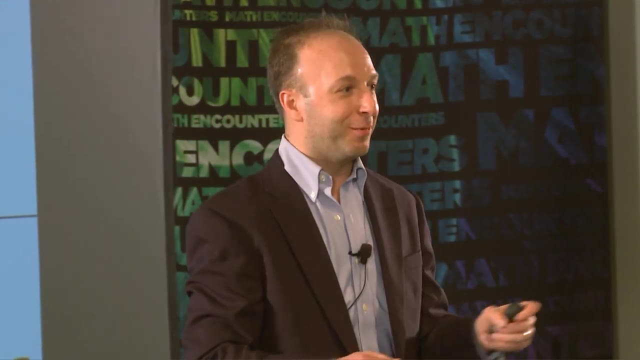 Collects everything that's published, everything worthwhile. So this is a port town. So anytime a ship comes in their minions, run onto the ship and find every book that they can. They say: we're going to borrow this, We're going to use this for a second. 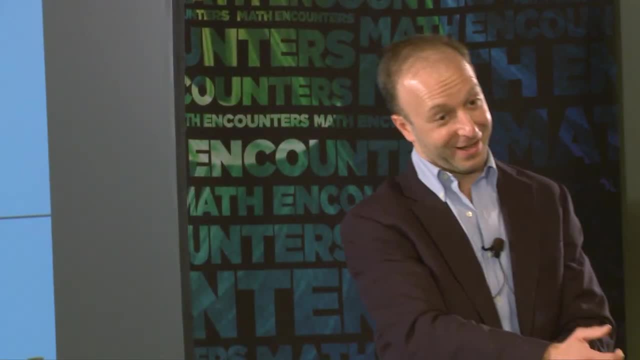 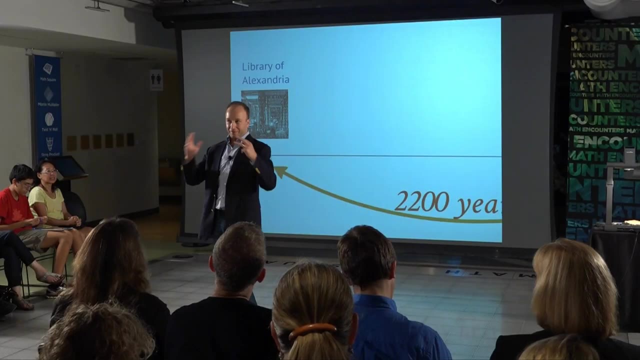 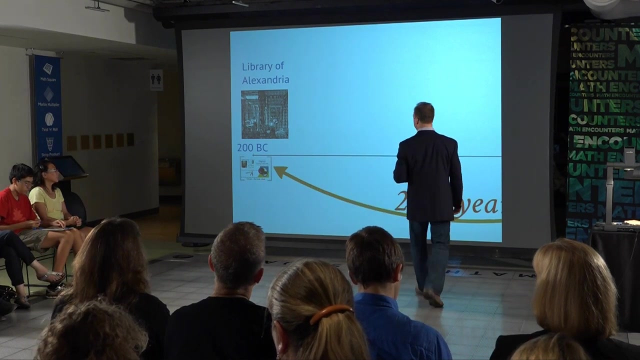 They run off into the library, transcribe it. They bring them back what they say is the original, Never mind. And so they have this amazing, unbelievable collection of every piece of philosophy, mathematics, science, everything that exists writing is collected in this Library of Alexandria. That's just a reference point. It's not just a reference point actually. So the first couple of hundred years of Christianity, Christians are persecuted. They're treated like a cult right The doomsday. The world is coming to an end. 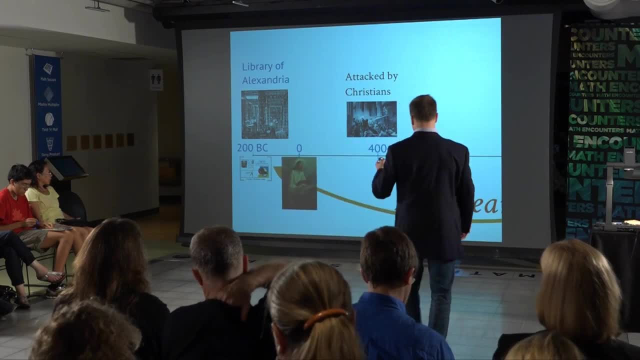 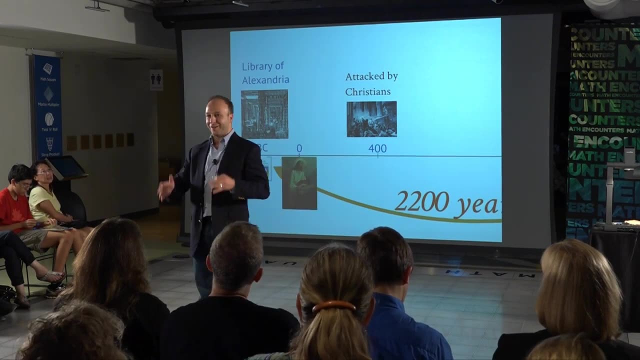 Jesus is coming again Sounds crazy, And they're persecuted. Around the year 300, Constantine converts to Christianity, And by the year 400, the entire Holy Roman Empire is Christian. And so what are you supposed to do with a book full of pagan books? With a building full of pagan books. Burn them. Burn them So they don't. They attack it in the year 400.. It suffers a similar fate At the hands of the Arabs shortly after Muhammad dies, 250 years later. Now it's burned to the ground. 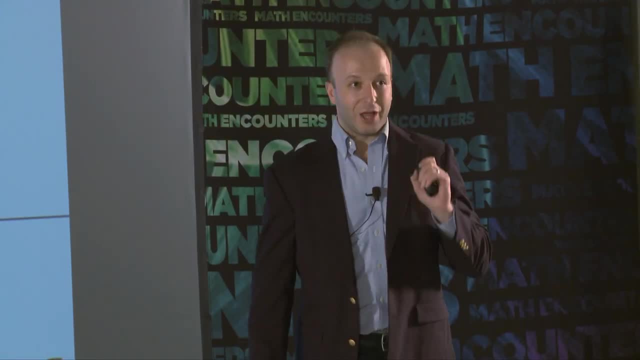 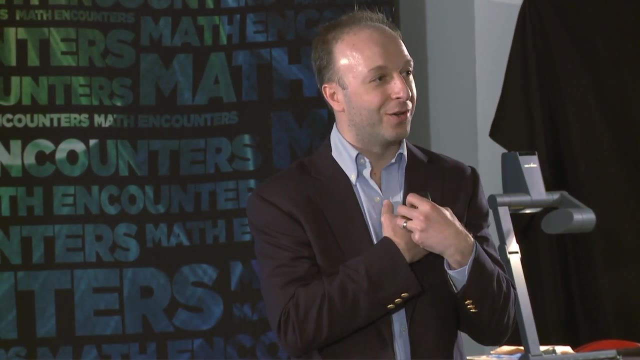 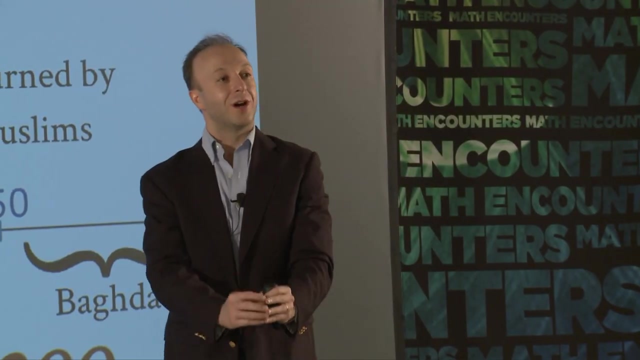 The library is gone. But following the Arab armies come the Arab scientists, And whatever is left they treat as precious gold. They grab those books and they bring them back to Baghdad And for 600 years Baghdad becomes the cultural capital of the universe. 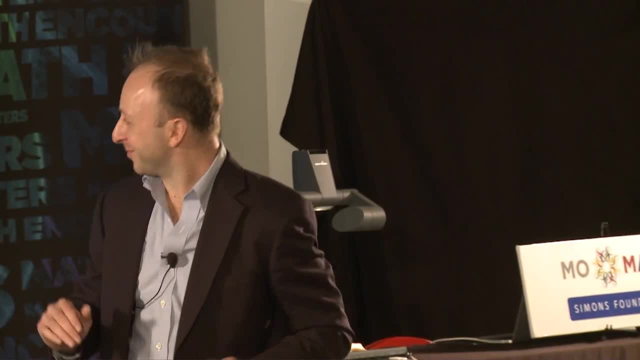 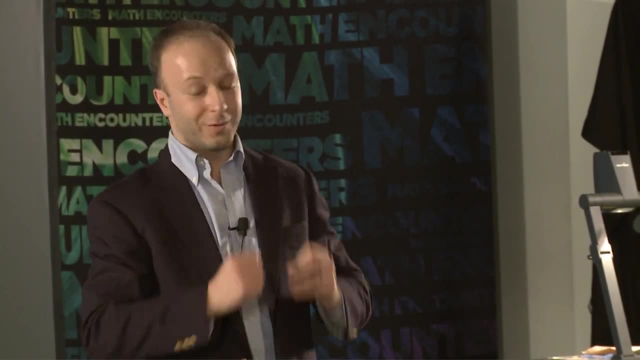 Well, at least Earth. Maybe there's aliens there, I don't know. So they're in contact with mathematicians and scientists in India, in China, And they've taken all the learnings from the West, And that's where these things are housed. 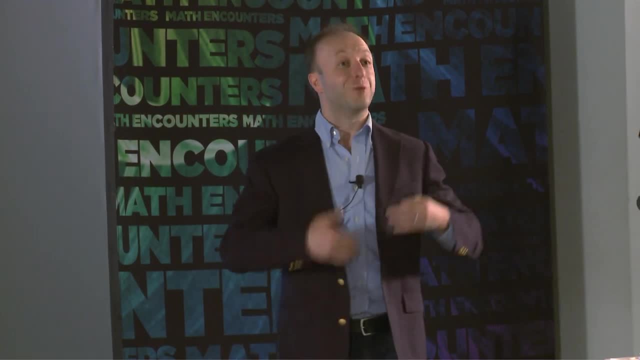 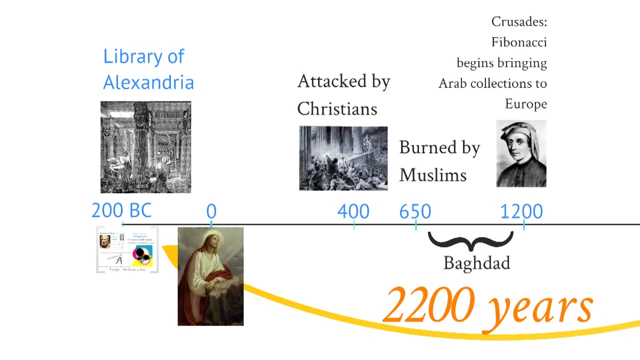 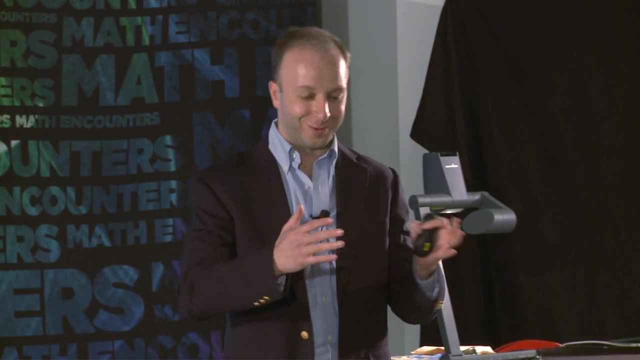 Around 1100, 1200, the Crusades happen. Another happy time in humanity Where, among many others, Fibonacci comes to these new world or old world, whatever Middle Eastern places And he discovers this amazing science that they have there, that the Europeans are completely. 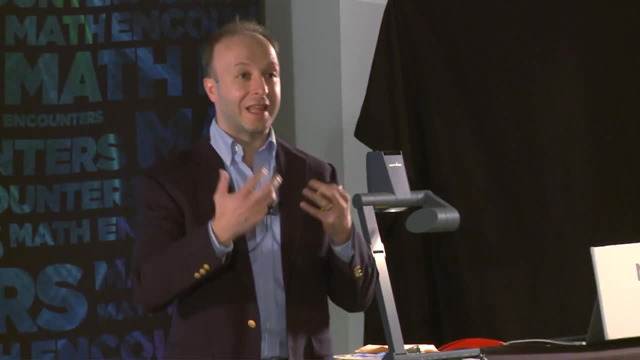 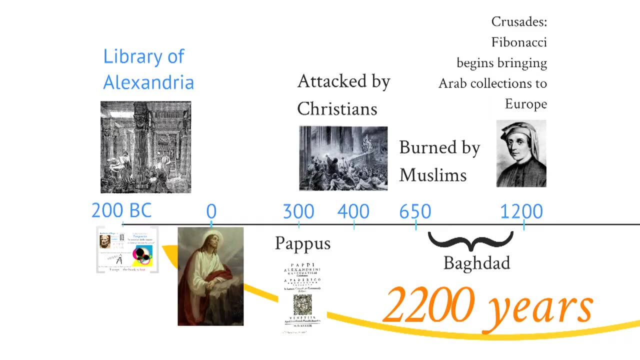 oblivious to, brings this knowledge back, And that's the beginning of the Renaissance. This is very cartoon history. Among the things that he brings back is wonderful work by Pappus, who is 500 years, half a millennium later than Apollonius. 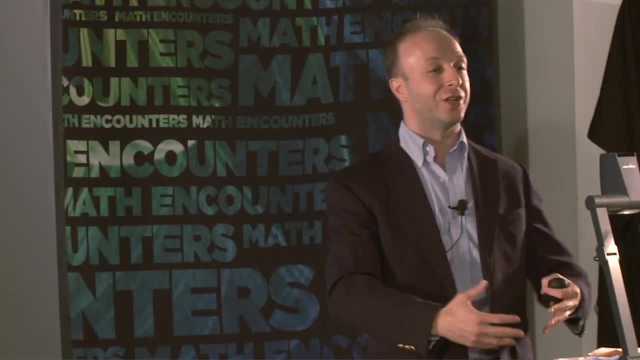 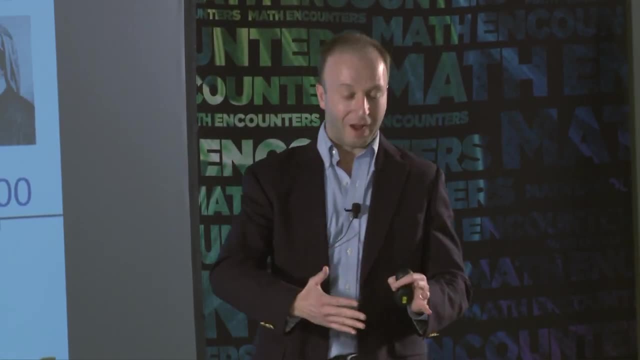 And what does Pappus? So Pappus has a compendium, a collection of all of the mathematical scientific knowledge to that day, So it's like a big encyclopedia. And there he writes about Apollonius' conics. 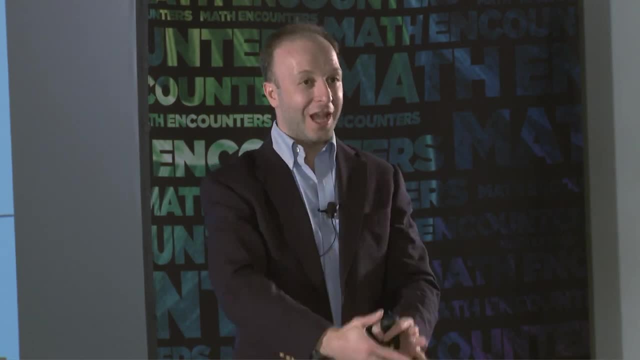 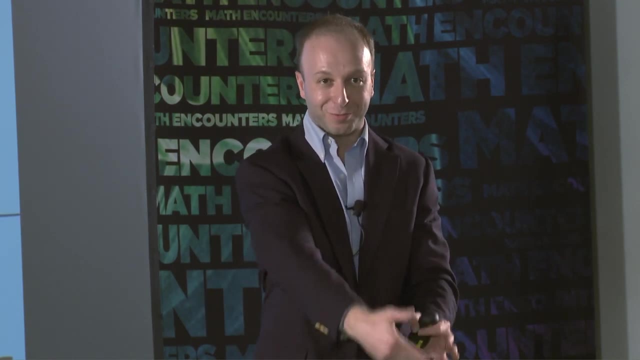 And that book does survive. And he writes about Apollonius' tangencies, He explains what's in the work, but he doesn't bother explaining how, the proof, how this theorem is proved. He doesn't say how to do it, because you can go to the next aisle in the Library of Alexandria. 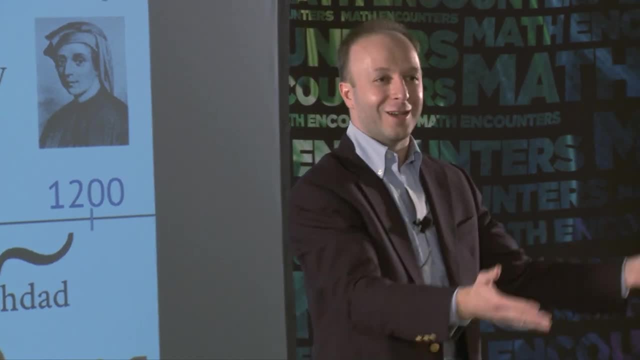 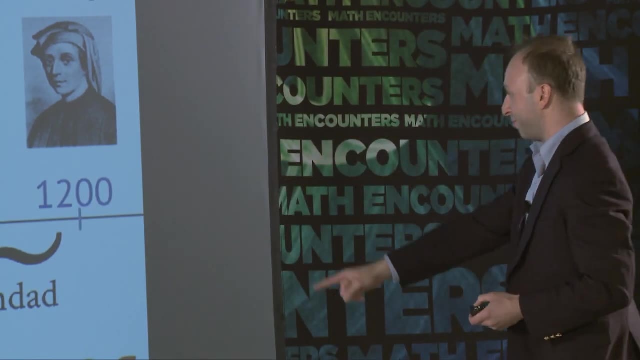 and go and open Apollonius' book. He is not going to waste time in his compendium proving every single theorem, He just tells you what the theorems are. So Pappus' book survives and tells us about the existence of tangencies. 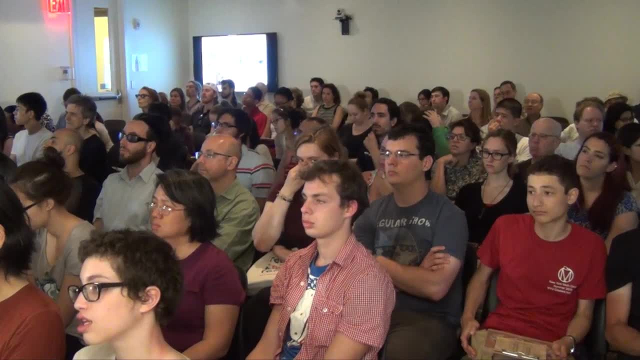 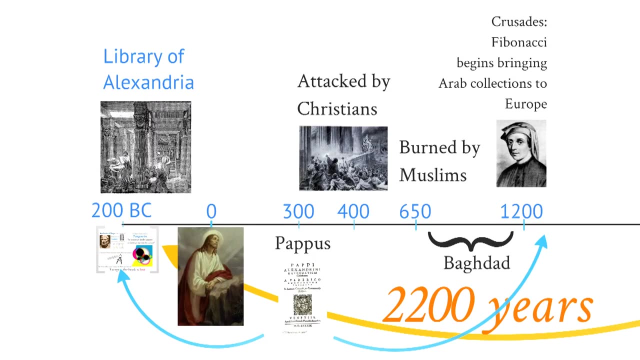 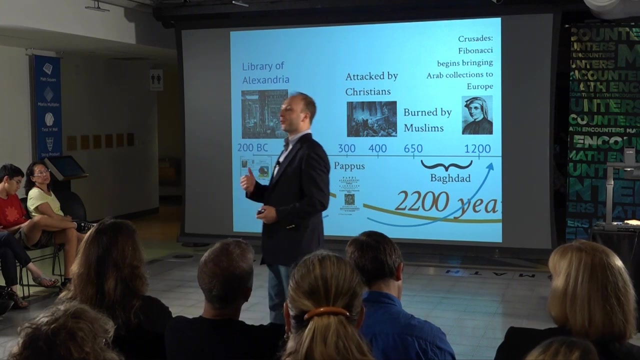 And that's what makes its way to the Renaissance, But Apollonius' tangencies does not. And OK, if Apollonius said he could do this, how did he do it? People spend the next 350 years trying to figure out how Apollonius did it, to the point. 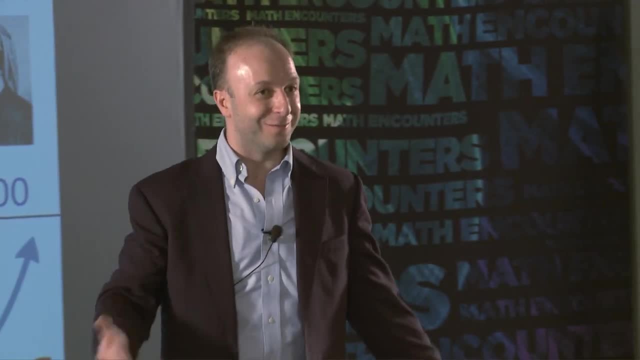 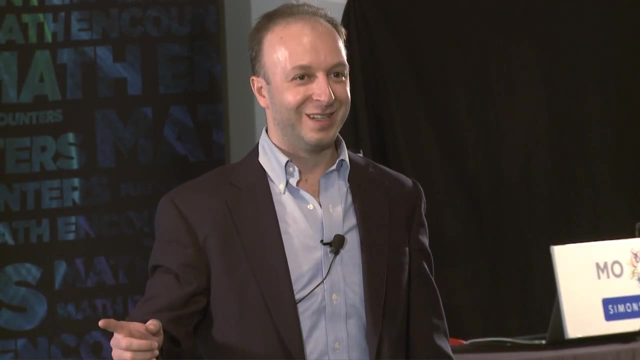 that people think. maybe he didn't do it, Maybe he had a mistake Right, Fermat's little theorem or last theorem. the little theorem is fine. The last theorem also took quite a long time for people to find a proof of. 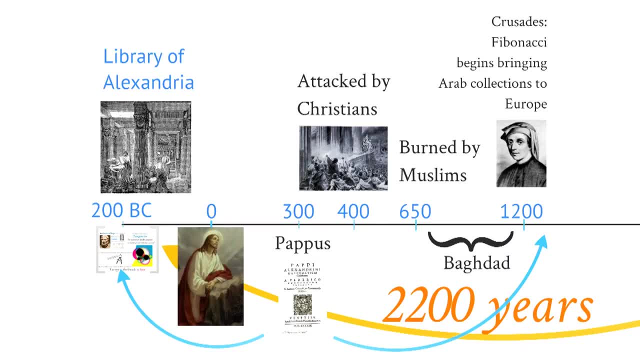 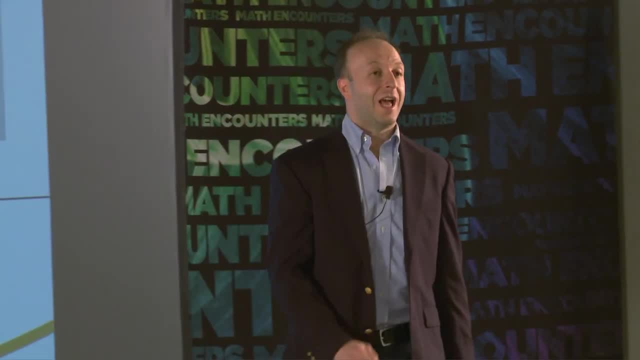 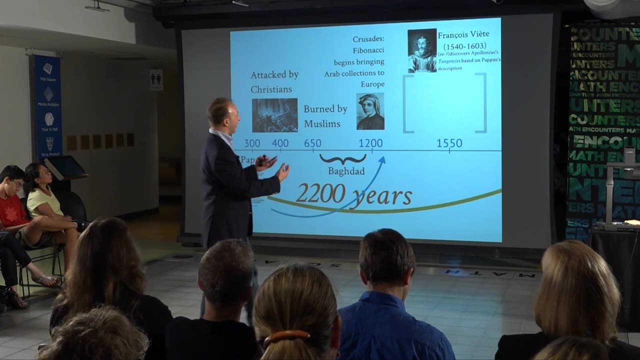 But we do not believe Fermat really knew how to do it In this case, as you'll see in a second. so 350 years later, we meet Francois Viette, And Viette rediscovers, or discovers on his own, what is plausibly a method that Apollonius 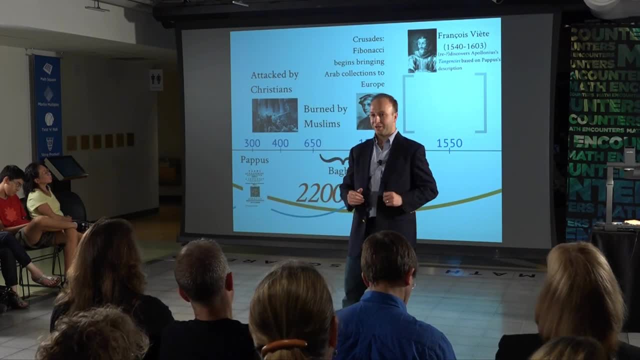 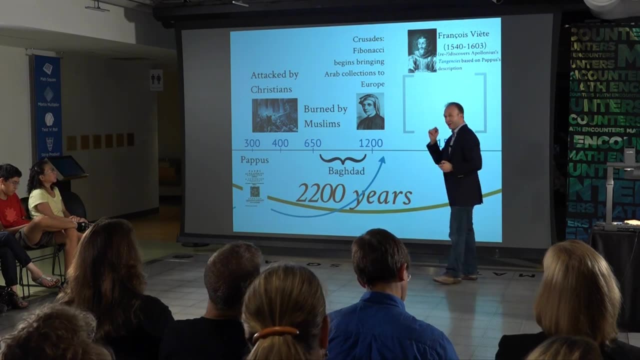 could have used to prove his theorem based on the description in Pappus' book, Pappus' Compendium. OK, So let's see how he did it. So for 350 years, it's not clear that there exists a straight edge and compass. 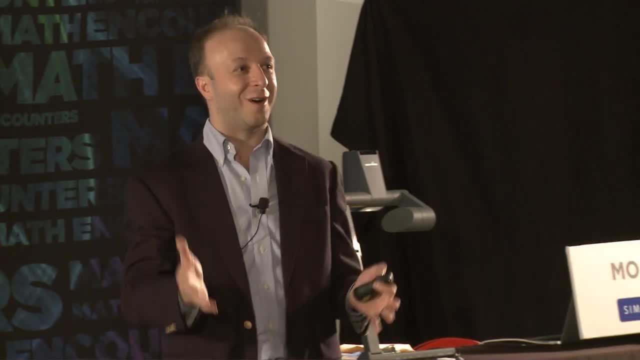 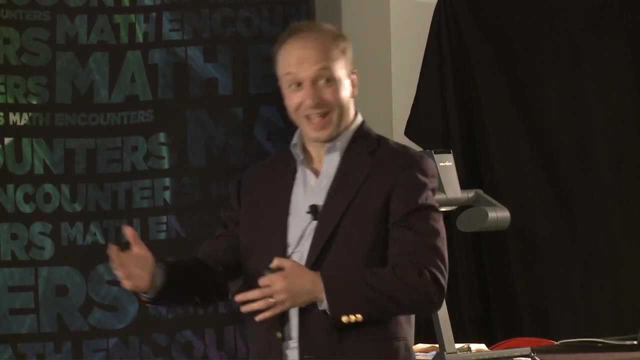 Circles are tricky with straight edge and compass. right Squaring a circle is one of the fundamental problems in Greek geometry that was not settled until 1800s in the negative. So you can't square a circle using straight edge and compass. 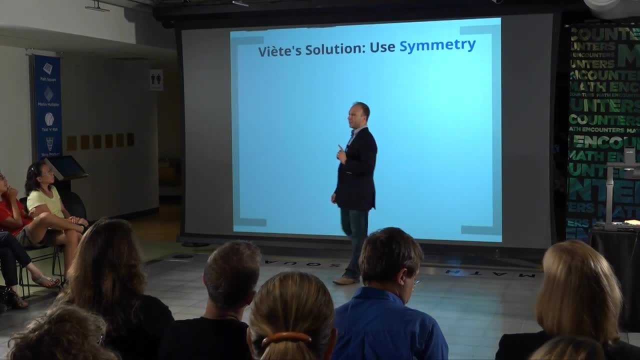 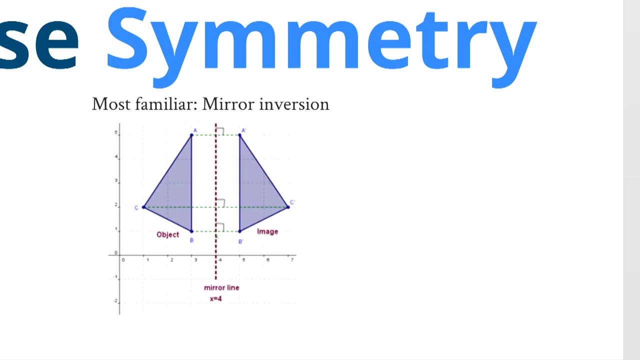 It turns out, you can solve this problem, And his solution requires an understanding of symmetry. So what do I mean by symmetry? You're probably very familiar- OK, I'm sure you're very familiar- with mirror inversion. You look in the mirror. you see an image of yourself. 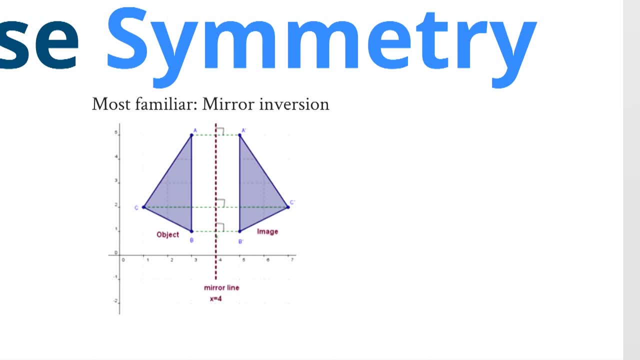 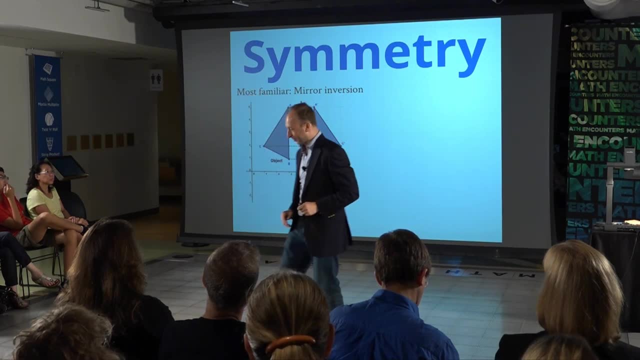 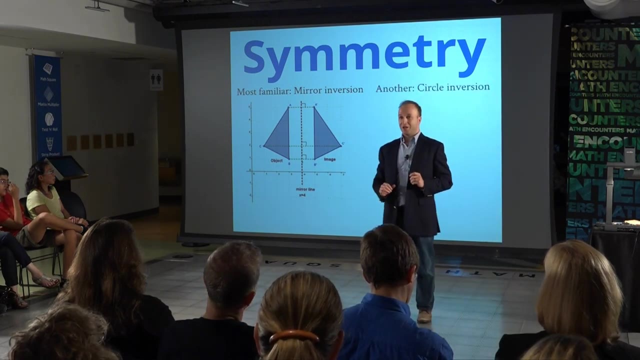 You're not really there. on the other side of the mirror, You just see the image. Or, if you take an imaginary line, everything on this side reflects to that side And human beings have this reflection symmetry Very familiar To mathematicians. another symmetry is also very familiar, which is called circle inversion. 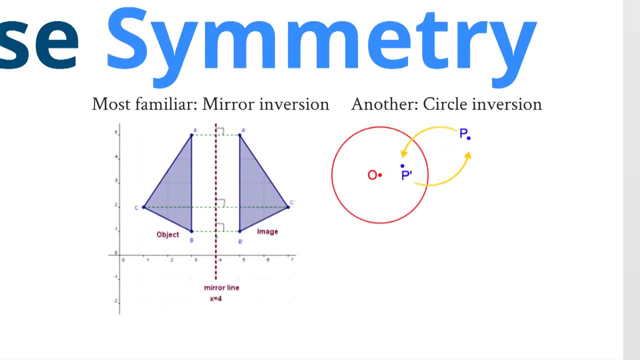 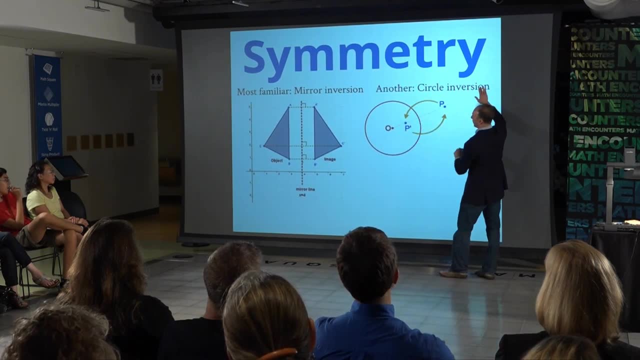 So how does circle inversion work? You give me a circle And then any point. What I want to do is, if the point is three times as far from the origin as the radius, I want to reflect it to a point that's a third as far as the origin, to the origin, as the. 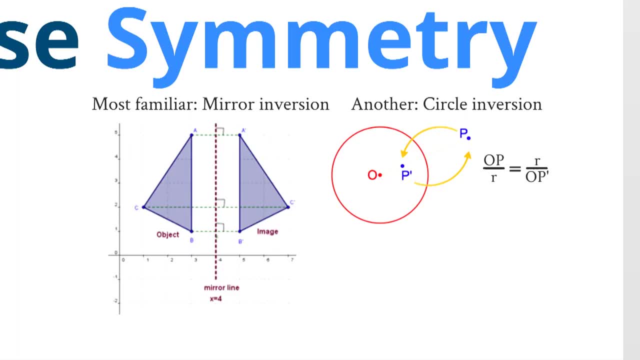 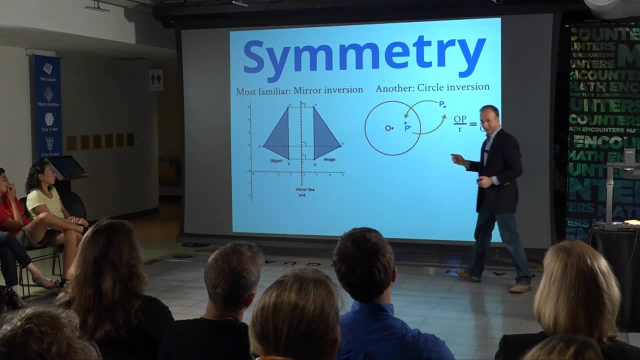 radius. OK, So you just want this relationship to be satisfied. So the distance from the origin to p versus the radius is 1 over the distance from the origin to p, prime versus the radius. OK, So objects. So if something is 10 times as far away, it'll appear 1 tenth as far away. 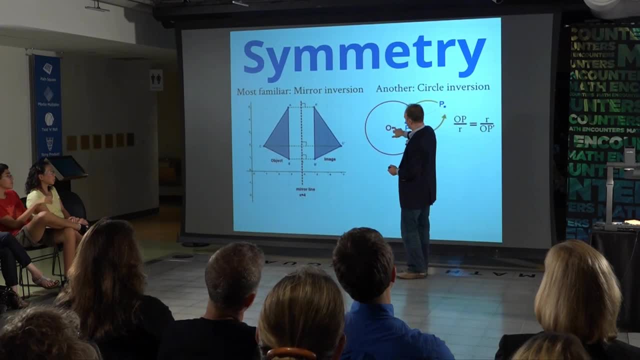 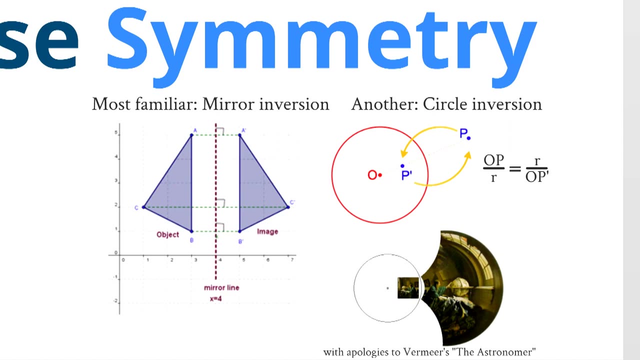 So objects that are very, very far away from the origin Turn into objects that are very close to their origin, and vice versa. OK, So just to see that in action. So this is Vermeer as the astronomer You can see here. 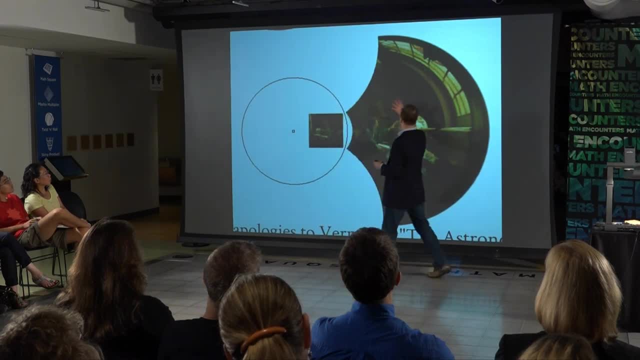 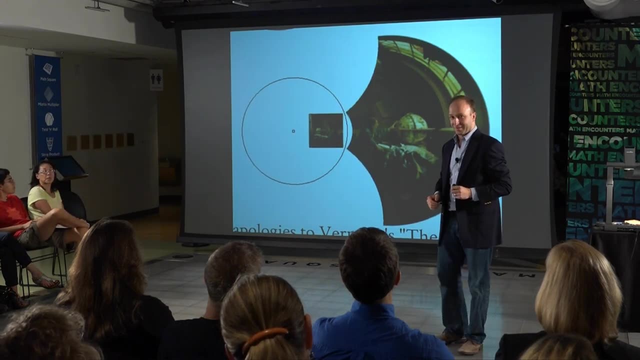 Well, I hope you can see- Maybe you've seen this picture- And what happens to it when it's reflected through the circle. it gets distorted in this way And that's circle inversion. OK, Any questions on this picture? So I'm just moving each pixel. 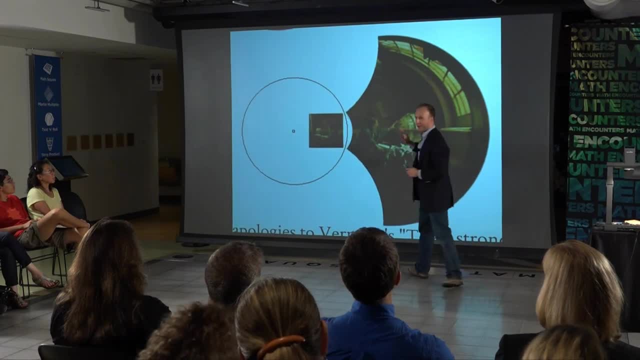 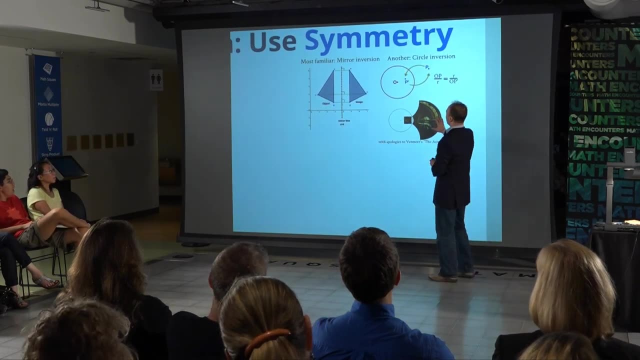 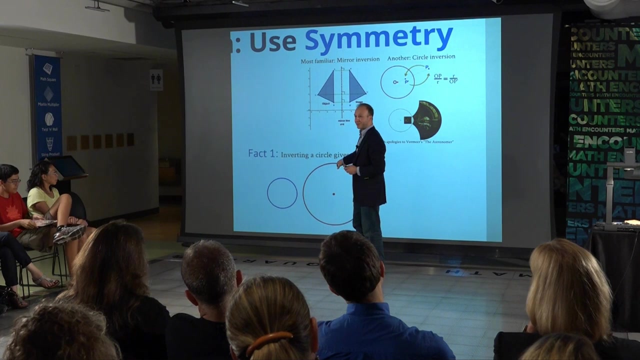 So, pixel by pixel gets reflected to wherever it's supposed to go, According to that rule. All right, So you need to know some facts about this kind of inversion. Fact one: If I'm going to invert through this circle pixel by pixel, but the pixels themselves, 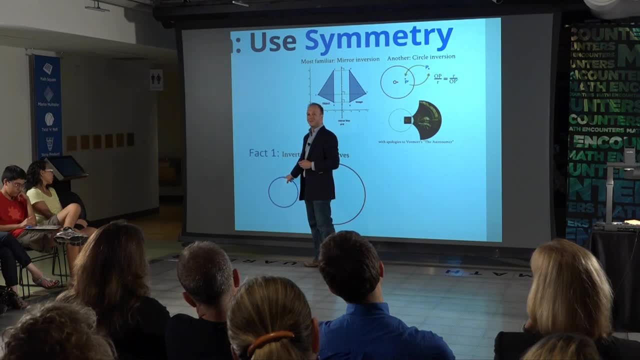 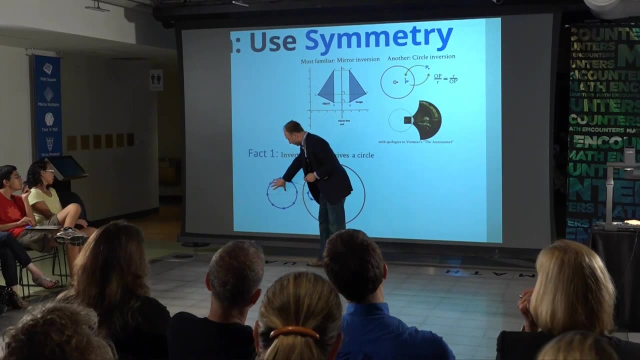 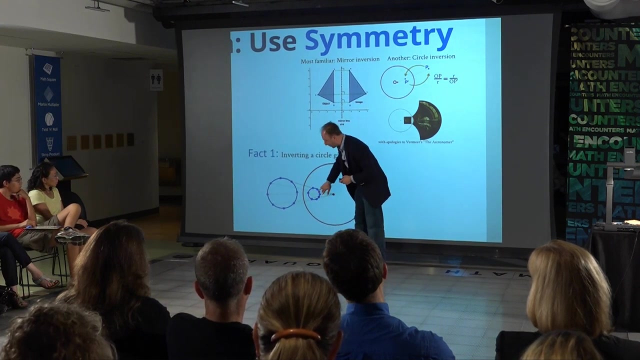 form a circle. what will I get? A circle, Yes, You guys know. OK, Good, So you don't get a circle, You don't get the same circle. So here I've taken equally spaced points around the circle. When I reflect those points, you see the spacing has been completely squashed in some places. 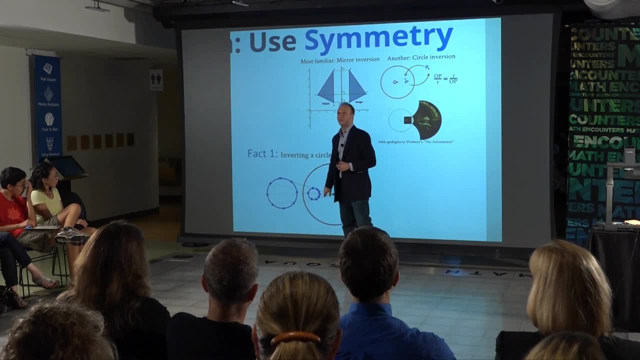 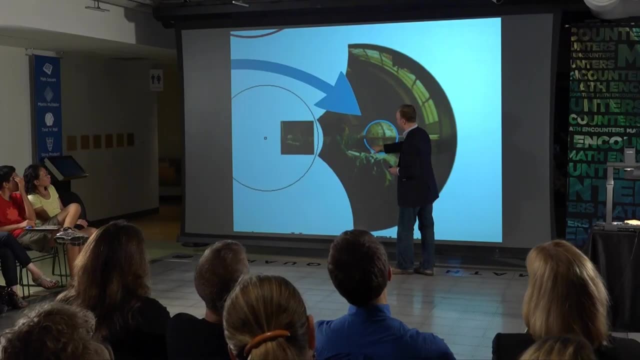 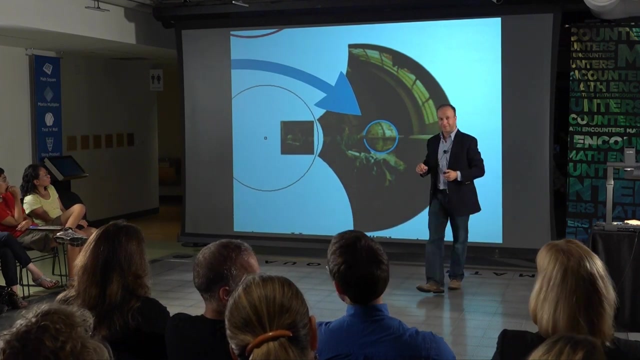 and stretched in other places, But the collection of all points remains a circle And in fact we should have seen that back here. when the globe, you see, it's deformed. Here is the straight line, So it got deformed, But the globe itself remains a circular globe. 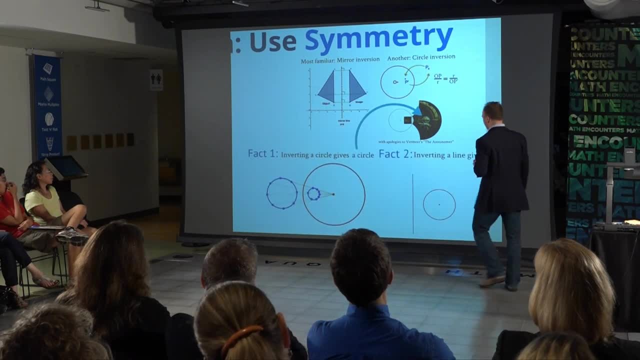 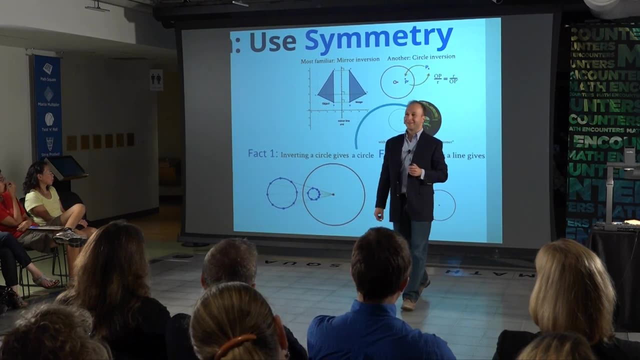 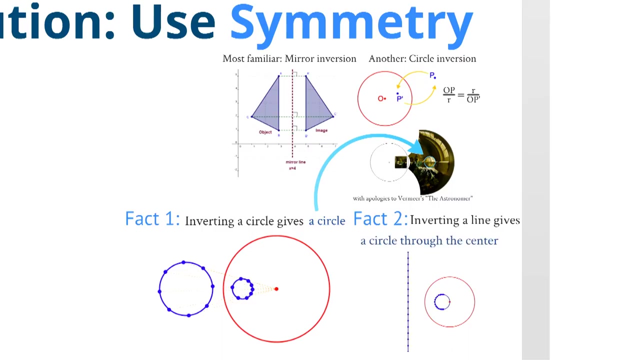 OK, Another fact that we need: What happens if you're reflecting through a circle, inverting through a circle, and the thing you're inverting is a straight line? Then what do you get? You get a circle. You get a circle. 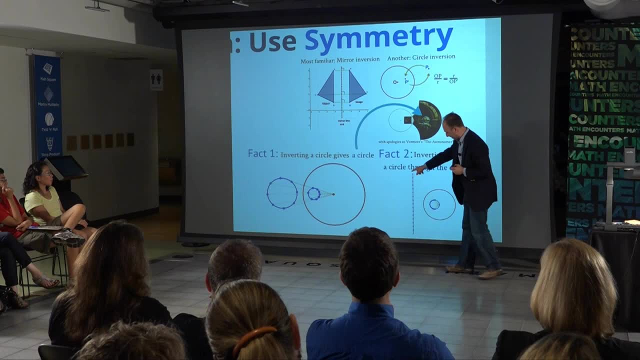 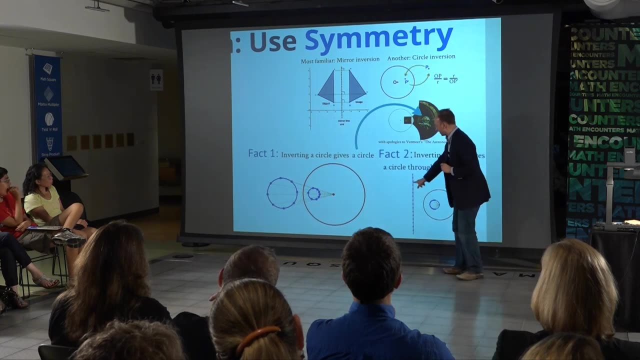 It's again distorted. So here's equally spaced points on this line that are turning into not equally spaced points on the circle. And there's a special thing about that circle: The line gets infinitely far away from the circle. So when it's inverted, 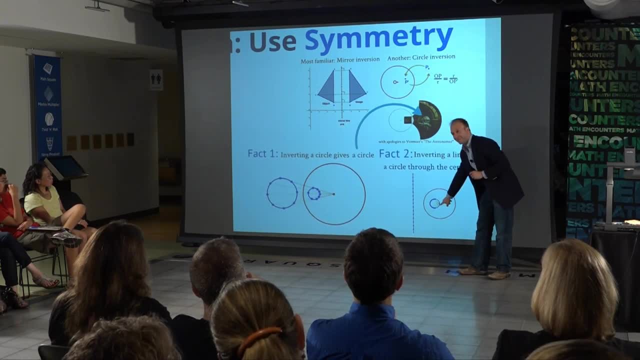 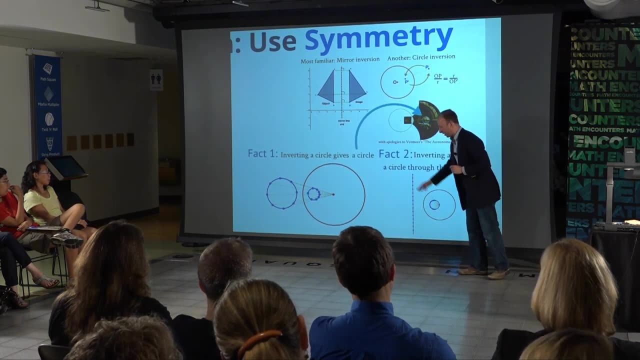 OK, It goes through the origin. The circle gets infinitely close to the origin just means it goes through the origin, OK. So lines go to circles through the origin And circles go to circles under inversion, And in fact we can see that here as well. 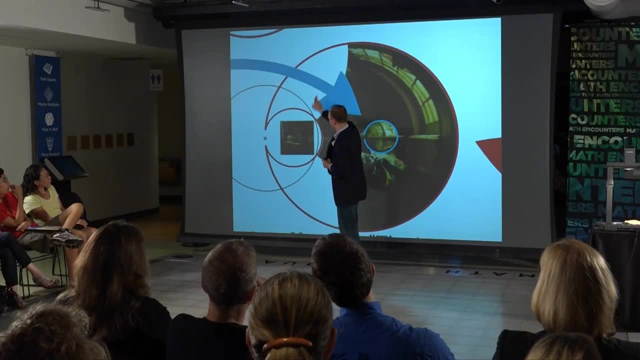 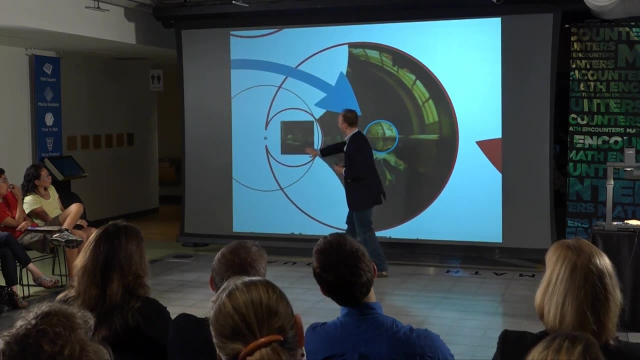 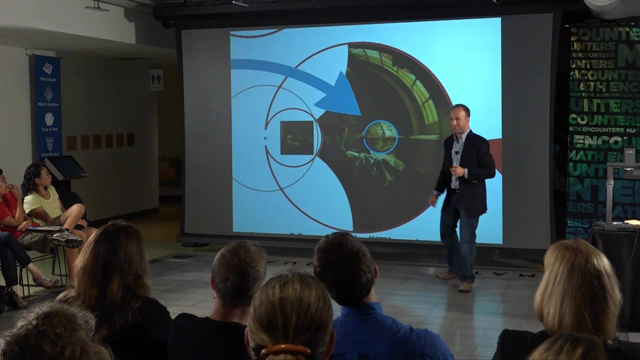 So if you look at this edge, which is a segment of a straight line, that edge turns into this edge which, if we follow forever, goes into the origin. And this edge, this straight edge, turns into that Circular segment which again goes to the origin. 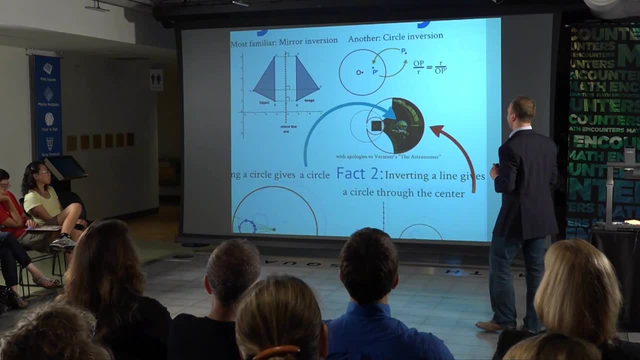 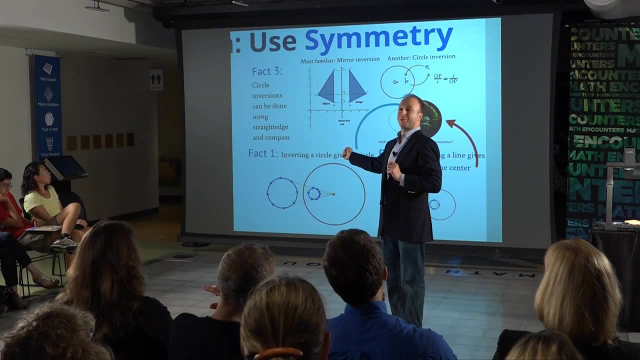 OK, So these are the only two pieces of information you need to know. These are two facts. Actually, there's a third fact that you need to know, which was known to the ancients, is that you can do these operations- circle, inversions of lines and circles- using only straight. 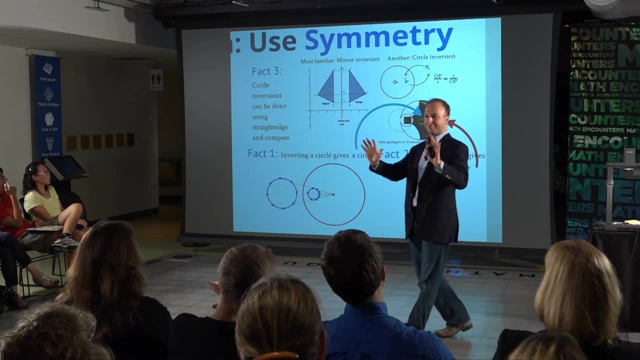 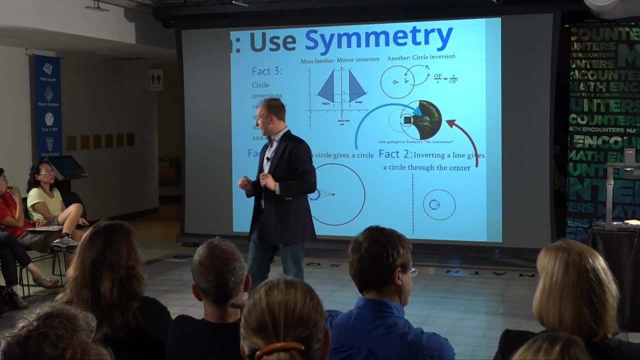 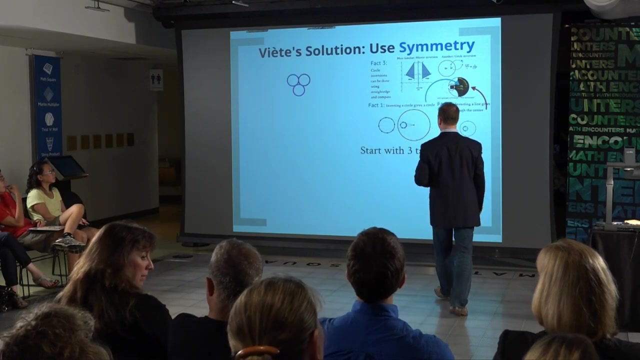 edge and compass. I haven't proved that for you, but you can look at a Wikipedia page if you like. This is very standard stuff. So You're armed with these two facts, three facts, And you want to solve the Apollonian problem. 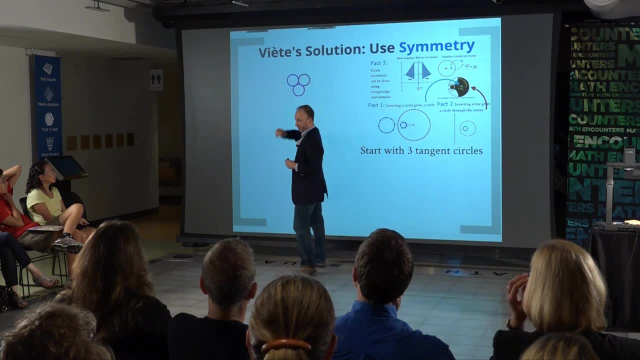 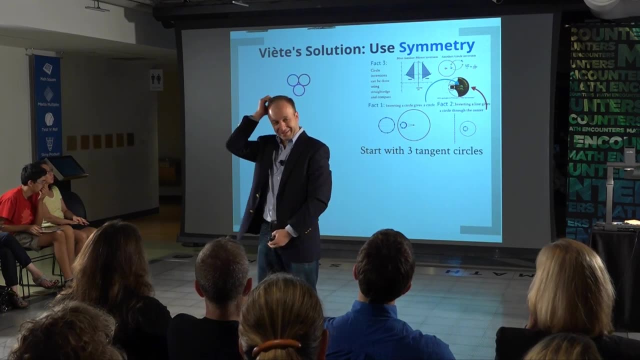 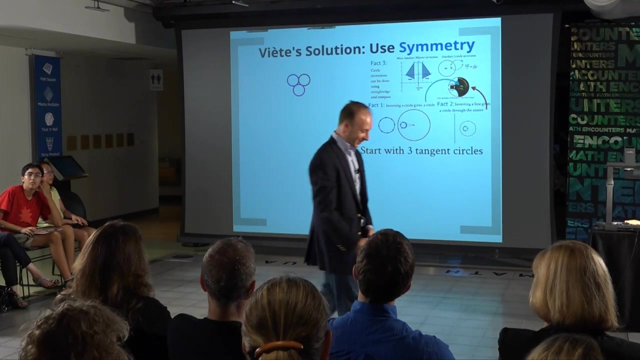 Let's do the case we're actually interested in where the three circles are already mutually tangent. What are you going to do? Scratch your head, Take a walk, Get a coffee, Hear Paul Erdős Something stronger. What do you do? 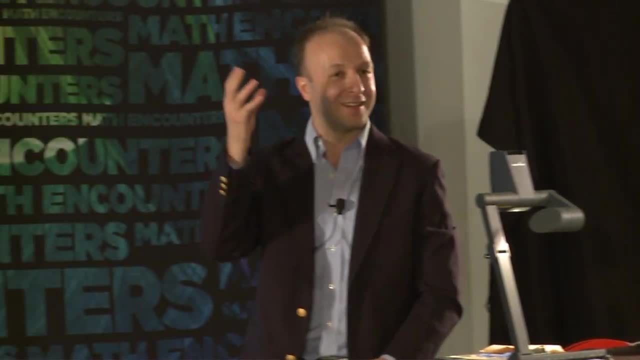 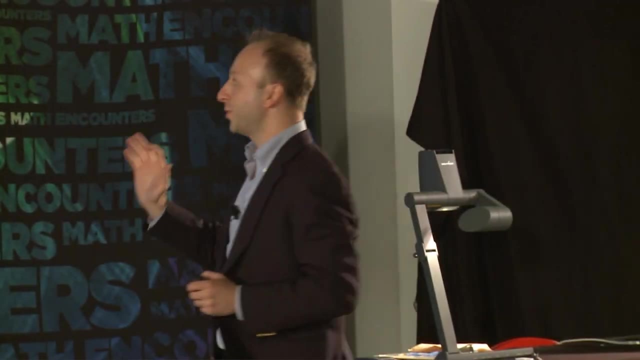 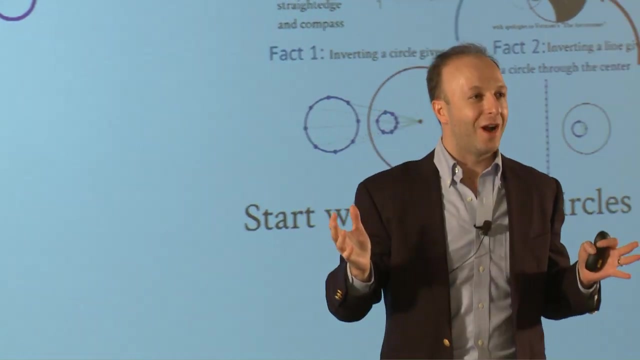 At some point You need a stroke, an inspiration, an idea. I have no idea where this has come down from- heaven or outer space, or what- But Viet has the following absolutely gorgeous idea: What you're going to do is add an object to this picture, which is a totally arbitrary. 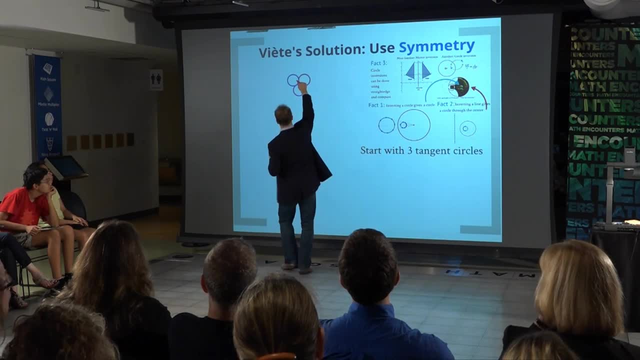 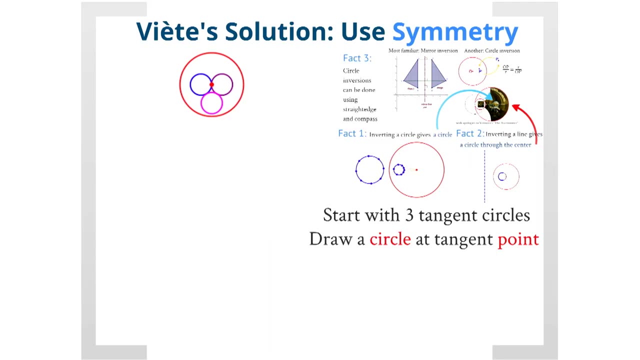 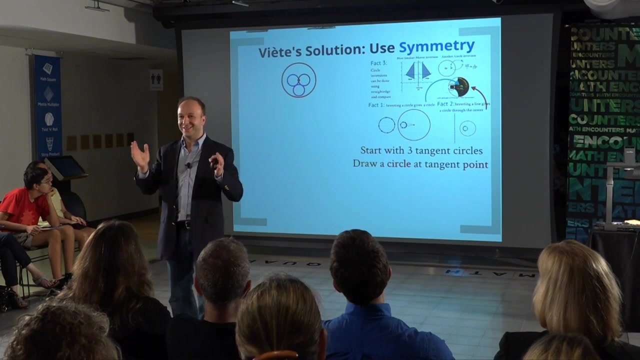 object. What you do is you fix one point where two of the circles touch and you draw an arbitrary circle centered at that one point. Why would you do that? Why would you get that crazy idea? I have no idea why that would occur to you. 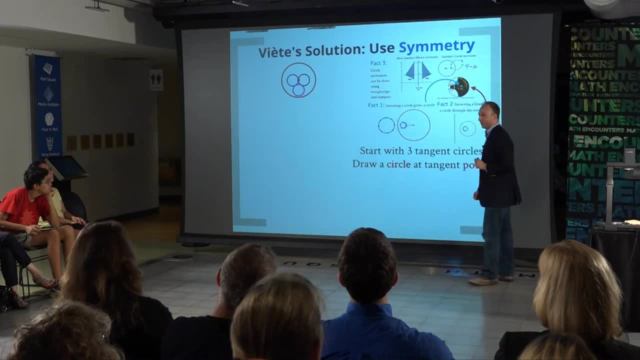 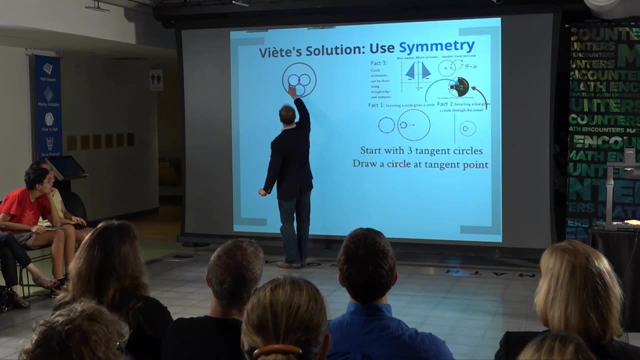 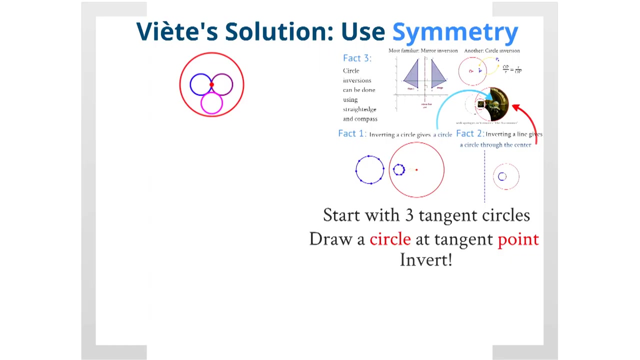 But it occurs to Viet. So, once you've drawn this circle, what do you do? Invert. Now what's going to happen to this blue circle? when we invert through this auxiliary circle, We get a line. It goes through the origin. 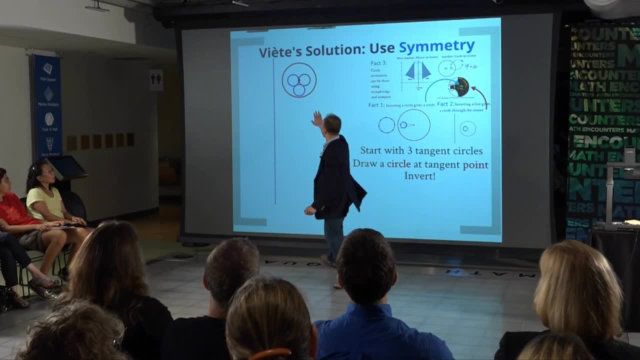 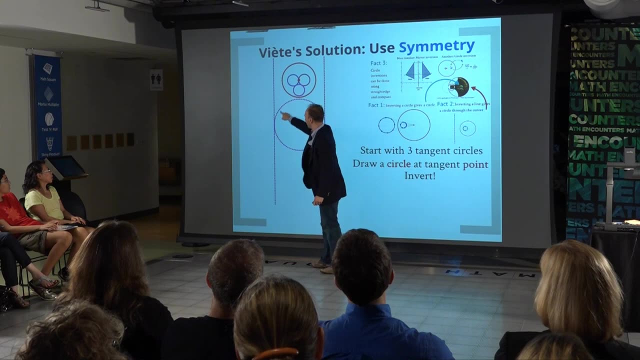 So we get the inversion is a line. How about this circle? It's a line, It's a circle? Another line- And this one, It's a circle- Will be a circle that's tangent to the two lines, So there's only one place where it can go. 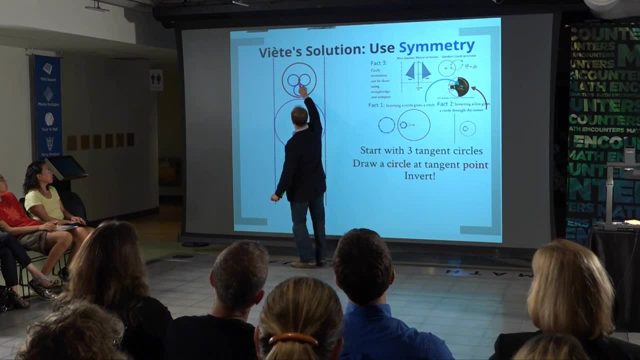 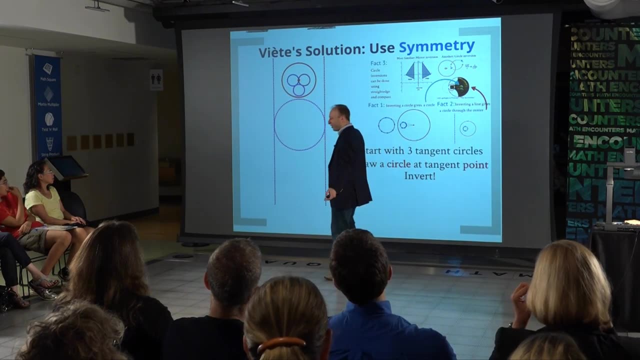 Now again, what are we trying to do? We're trying to find a circle that we can put exactly in here. But we could try to find a circle that we could put exactly in here, But now the solution is utterly trivial, right? 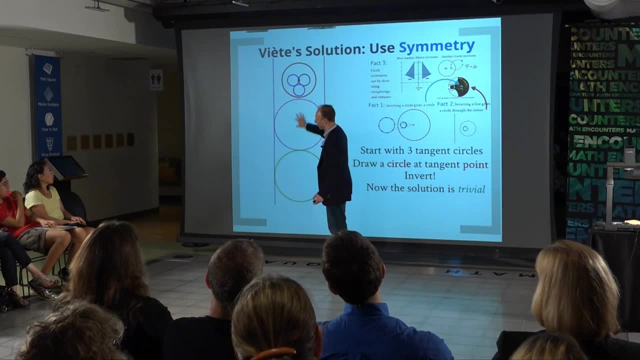 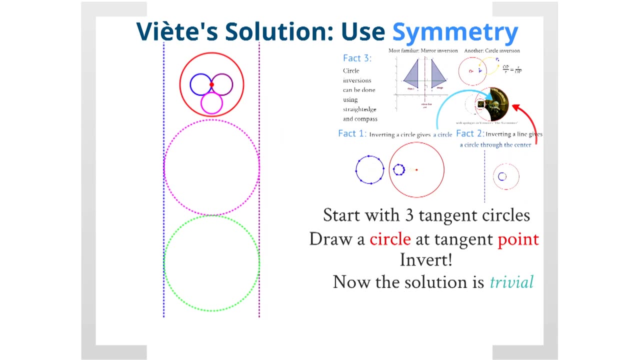 That's the circle. I think we all can agree that this is not a hard thing to do with straight edge and compass. We can use this circle to draw this one. And now what? Invert back, Invert back, So again, reflect through this circle. 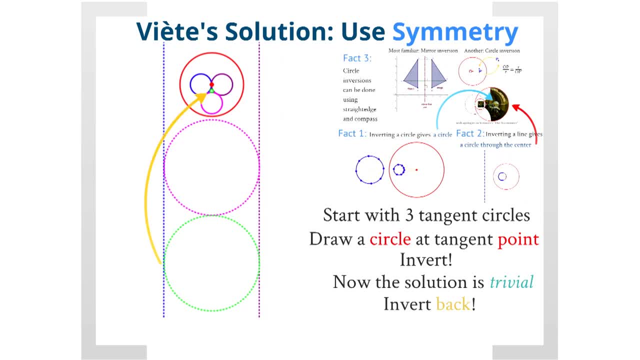 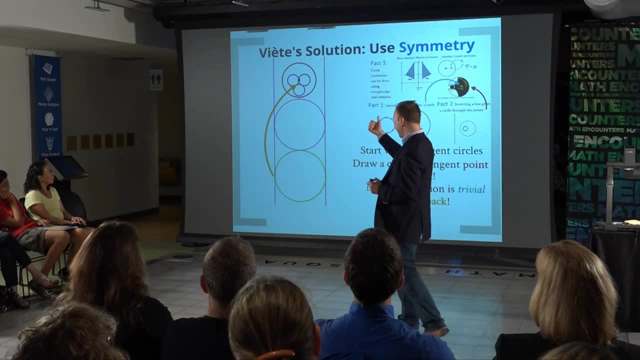 And when you invert back, there's your perfect straight edge and compass construction, And it uses all tools available to Apollonius. You need this stroke of genius. Apollonius has more than convinced us. he's capable of strokes of genius from his conic. 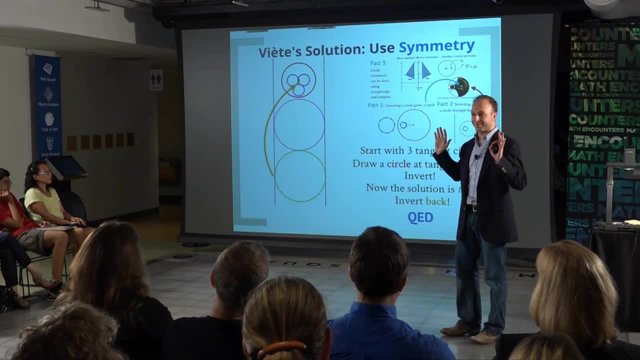 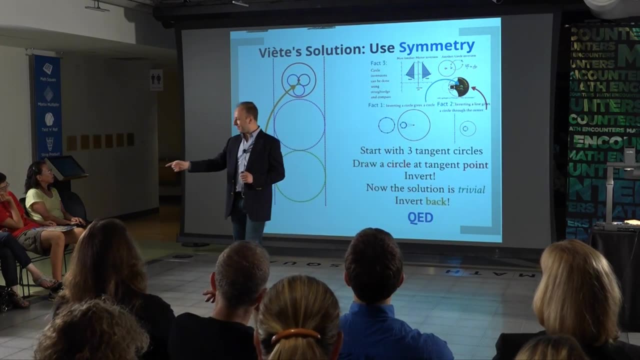 sections. There's no reason to believe he didn't have this proof, QED. OK, Now that's the ideal construction of that circle. It hasn't answered our question: What's the middle guy? Let's keep going, See who else we meet. 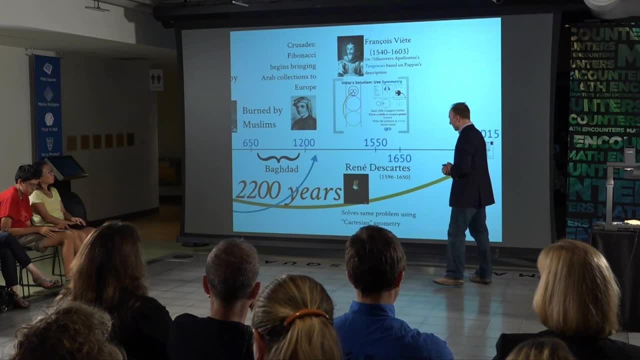 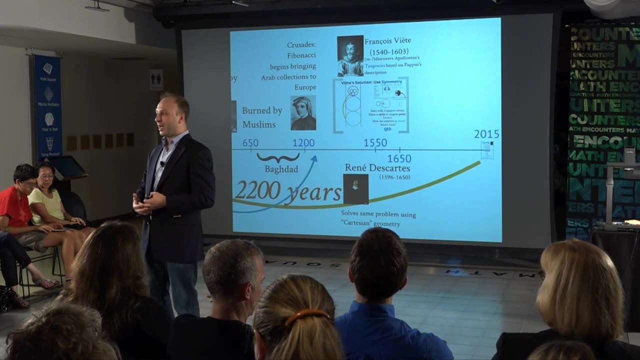 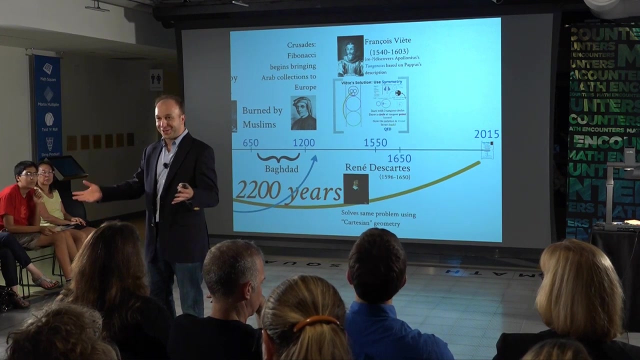 So this gentleman, about 100 years later, Rene Descartes, he solves exactly the same problems. He goes through all of geometry as known to mankind before that time, And he solves it in coordinates using Cartesian geometry. Why? Because he invented Cartesian geometry. 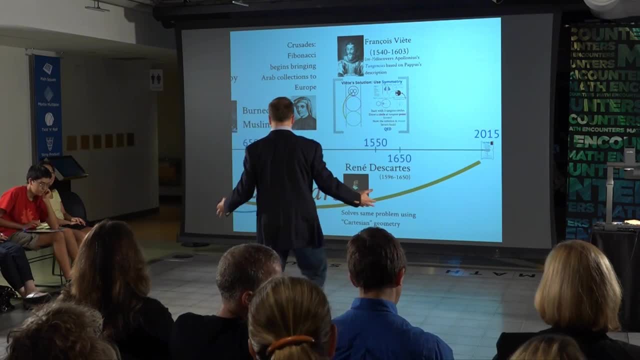 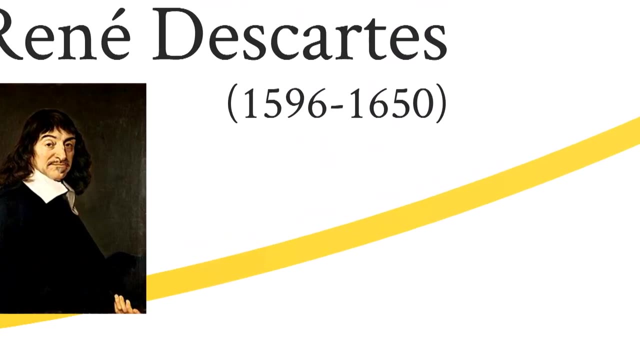 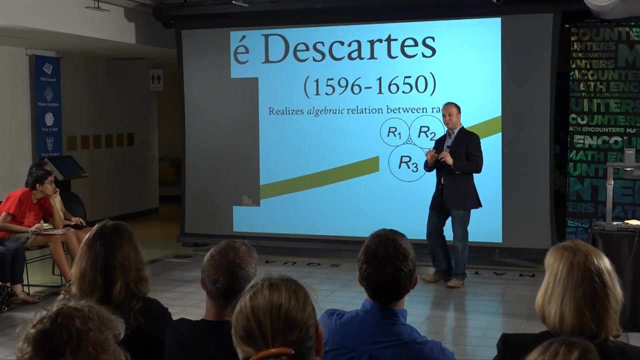 Descartes Right: If you invent something new, you say what does it do to every problem that's ever come, And how does it look? And he discovers something absolutely fantastic. He realizes that there's an algebraic relation between the radii of four mutually tangent 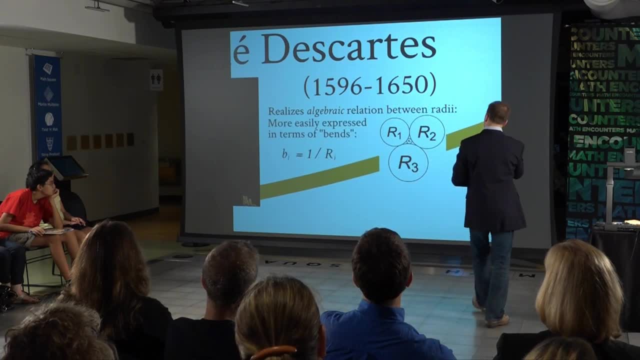 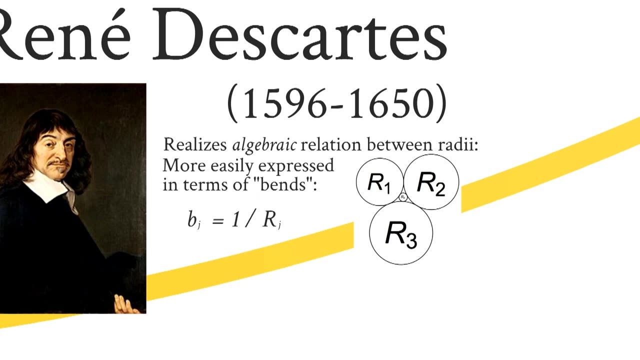 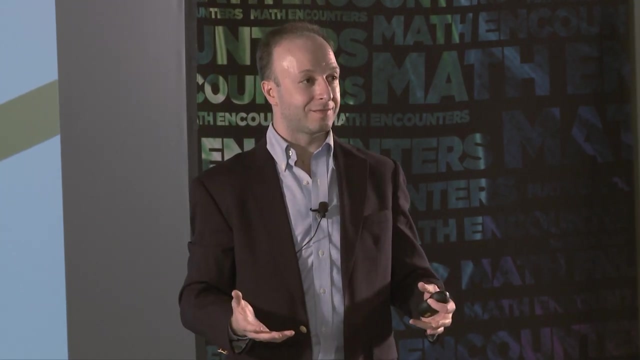 circles. What's the relation? Well, it's actually more easily expressed in terms of what's so-called bends or curvatures. The curvature of a circle is 1 over its radius, The reciprocal of its radius. OK, So if a circle has radius 1 over 100, its curvature, its bend, is 100.. 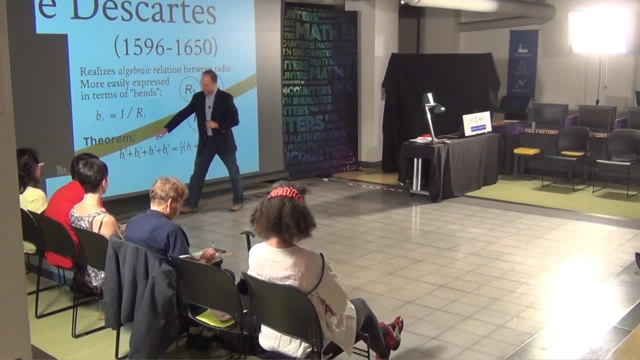 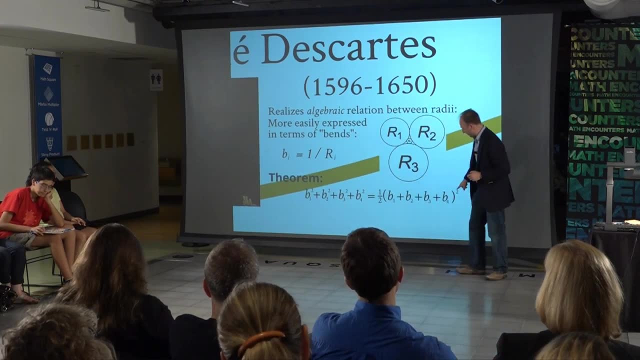 And what's the relationship? Here's his theorem. You take the four bends, You square each one and you add them, Or you first add them and then square And you almost get the same thing. You're off by a factor of 2 or 1 half. 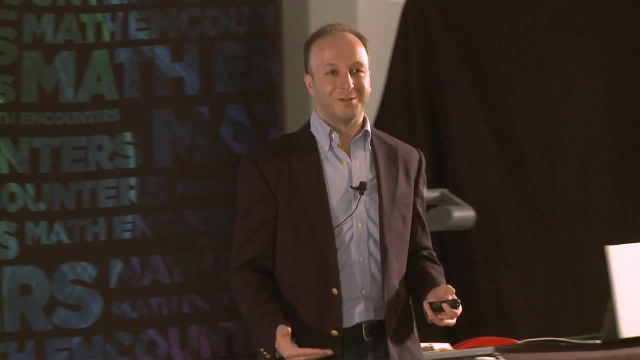 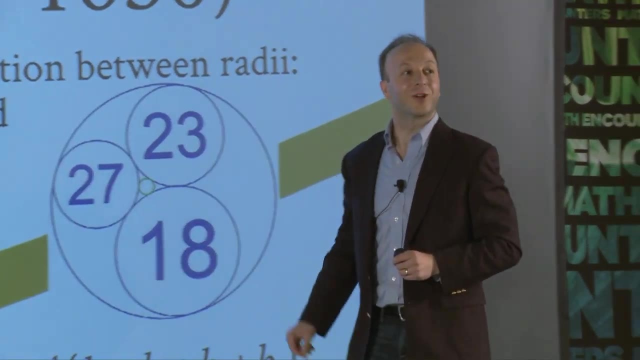 That's the theorem. So what should we do? We have? ah now, what I didn't tell you is that these labels aren't just arbitrary labels, They're actual curvatures. So let's see if I can convince you of that. 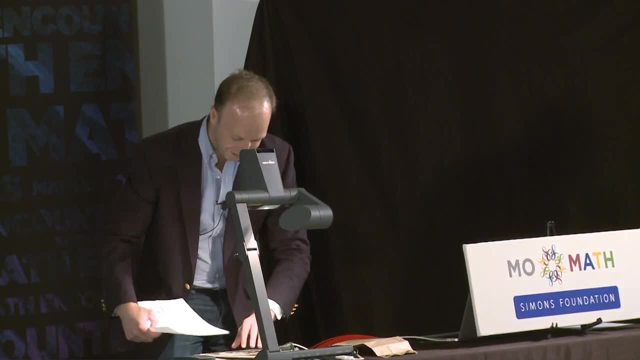 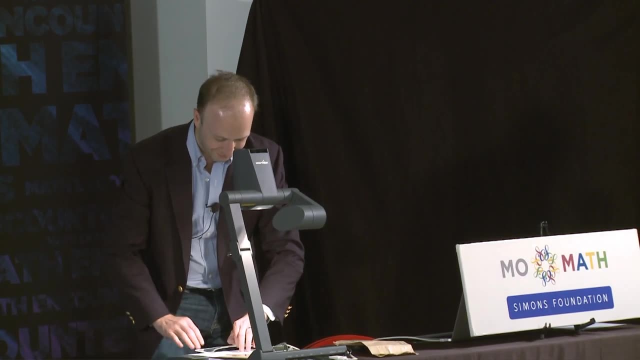 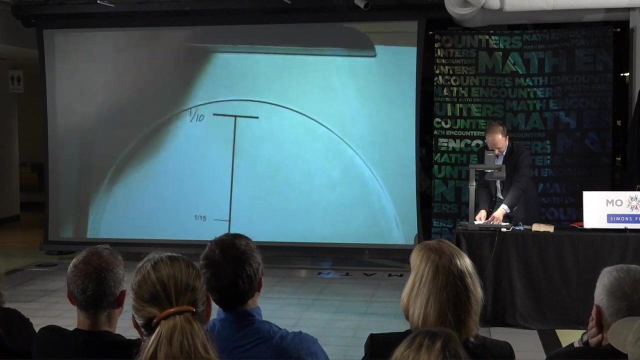 Here's my MoMath ruler. This is a very special ruler. There are not very many rulers with inverse coordinates, So if you can see the outermost circle, Ah, It killed the zoom. OK, Thanks, Here we go. OK. 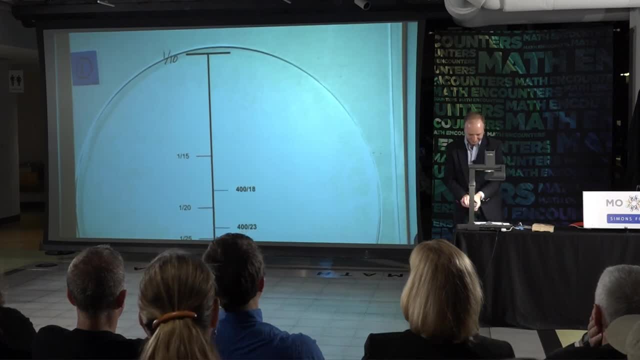 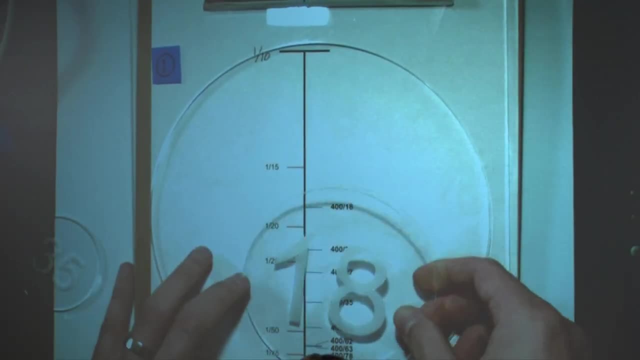 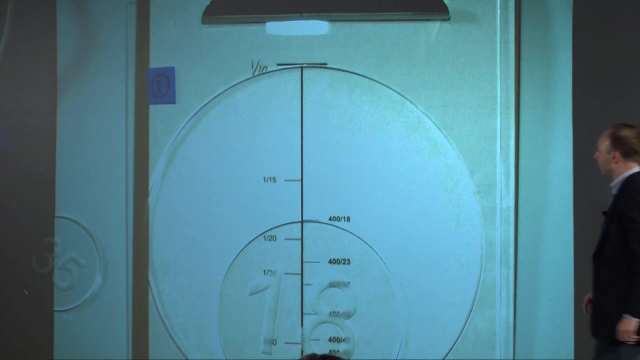 Now you can see. So let's see. This 18 disk is actually. the reason it's called 18 is because, if I measure it OK. so what you have to know is that one MoMath it's not a universal, it should be a universal. 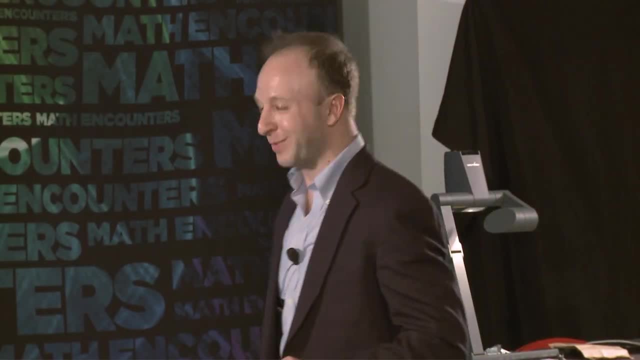 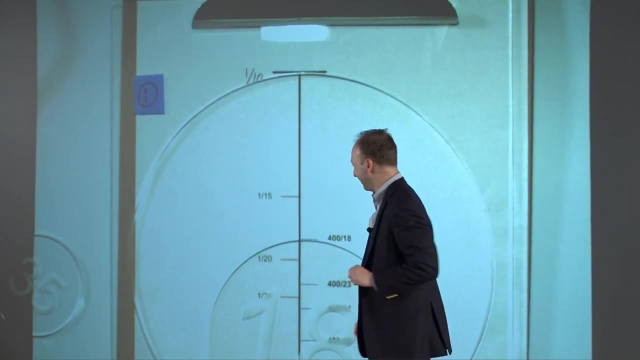 unit of measurement. It'll become a universal unit of measurement by next month's encounters. But one MoMath is 400 millimeters, OK, So 400 over 18 millimeters is 1 over 18 MoMaths, And that's the diameter of that disk labeled 18.. 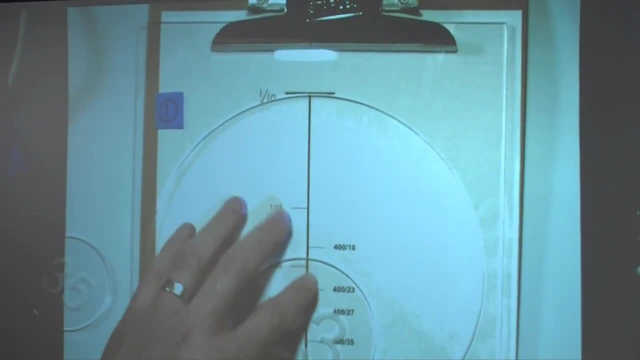 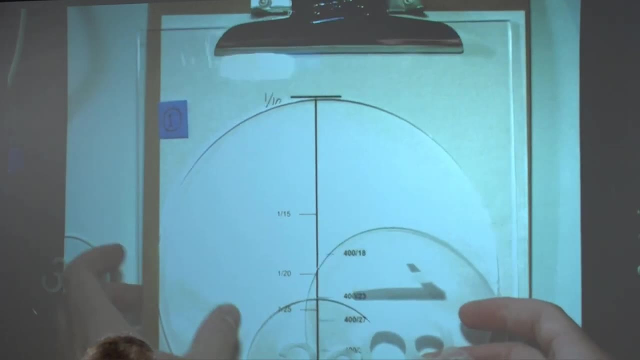 OK, And you can check the same thing for the 23 is 1, 23rd MoMaths, and so on. OK, So these numbers B that you've been seeing are the curvatures. Let's go back to the Descartes relation. 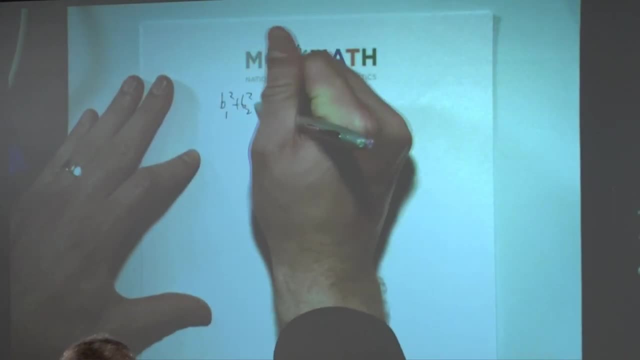 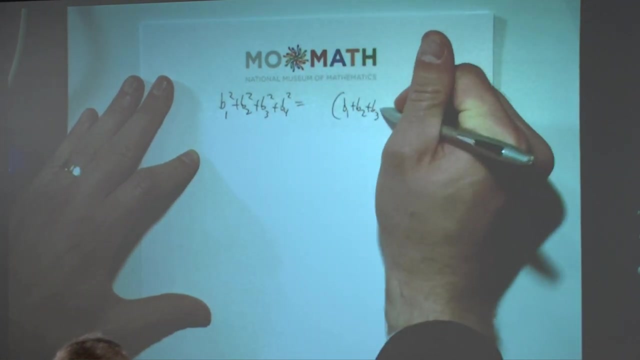 So what did Descartes say? That if you take the curvatures, the bends, and you square them, you almost get the same thing as when you add the bends and square, except you're off by a factor of a half. 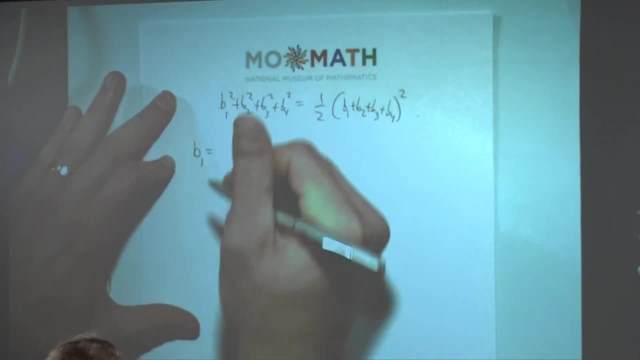 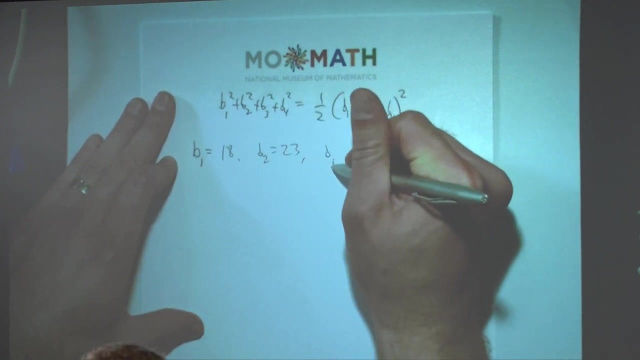 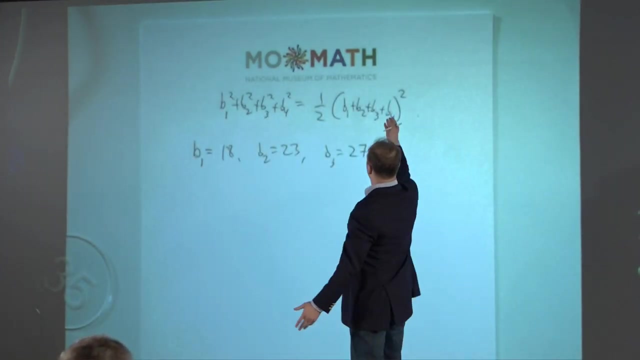 Right. And what were our three bends? So the first one was 18. And then 3. 23. Thanks, And 26? 27. 27. OK, Those are our three bends. So look, we have a quadratic equation with one unknown. 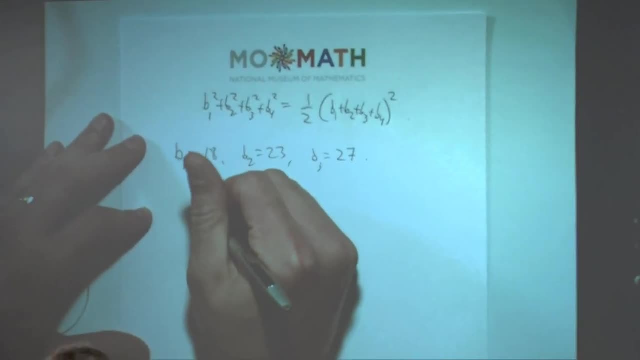 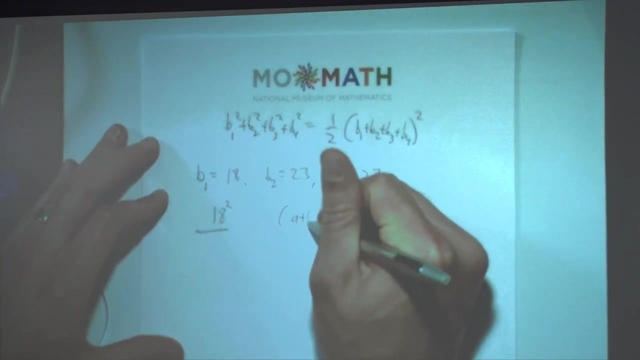 Let's solve it OK. So we need to square. So you know how to square two-digit numbers. You don't do it by digit, by digit, right? You do it by this formula: a plus b quantity squared is a squared plus b squared. 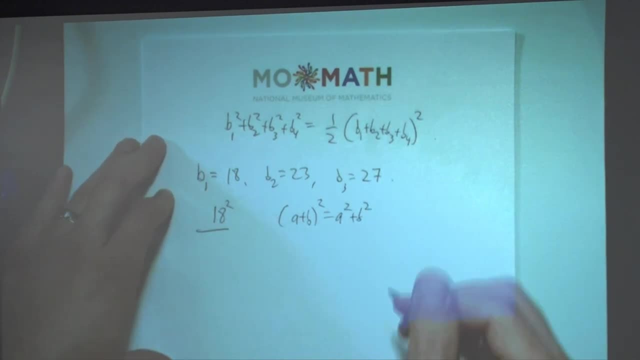 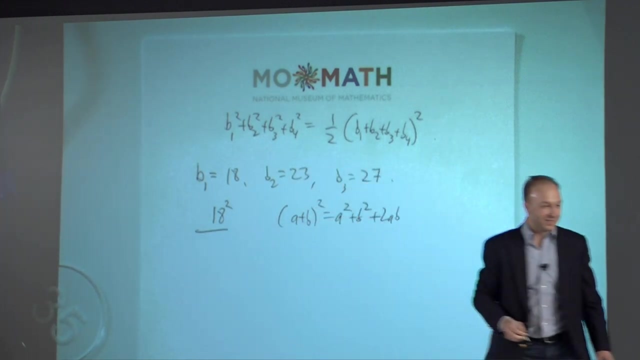 Everybody knows that. Just checking, Just checking, OK. Everybody knows that Your mom will help you, OK. So what are we going to do? Well, a is 10 and b is 8, right, So we just square 10.. 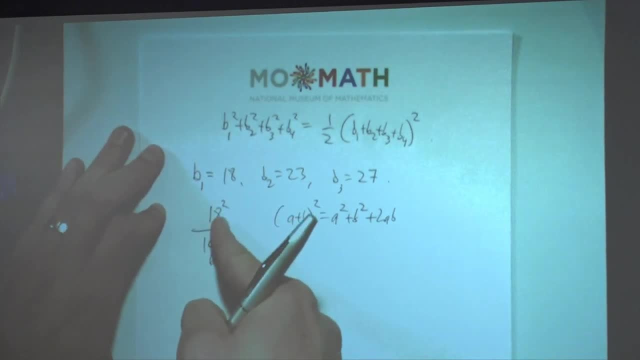 That's easy. That's 100.. If we square 8, that's 64.. 8 times 10 is 80, which we need to double, So 160.. And that gives us 324.. OK, So that's the square of 18.. 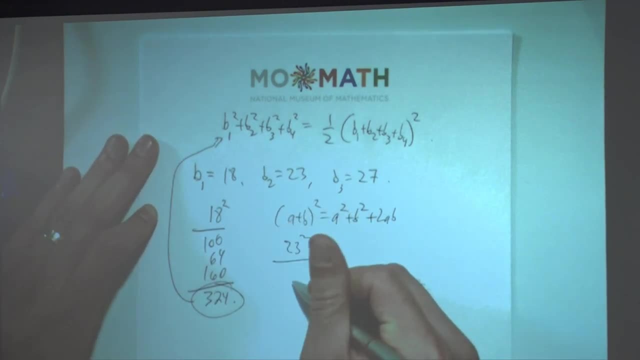 So far, so good. Let's square 23.. OK, So 23,. 20 squared is 400.. 3 squared is 9.. That's 60.. I want to double it, so 120.. So I get 529.. 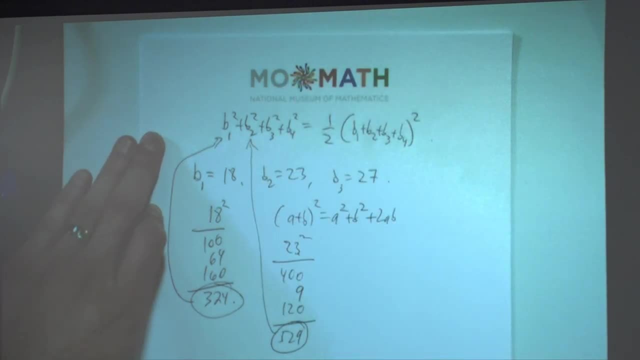 So 529 is that square? I hope you're checking me. There's no guarantee that any of these things are correct 27.. Now there's a little something you might observe if you're looking at 27.. 27 plus 23 is 50.. 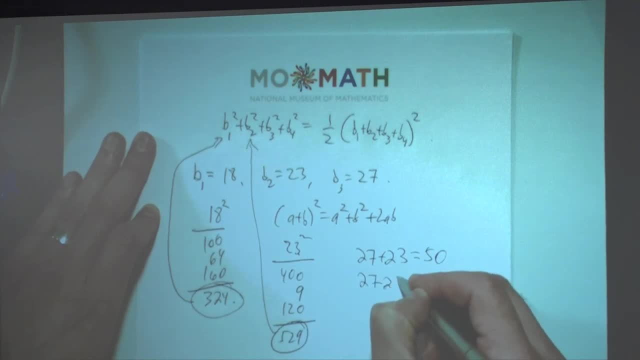 So that's nice and easy, Whereas 27 minus 23 is also an easy thing. It's 4.. And if I multiply these two, I get 27 squared minus 23 squared, And 50 times 4,, 200.. 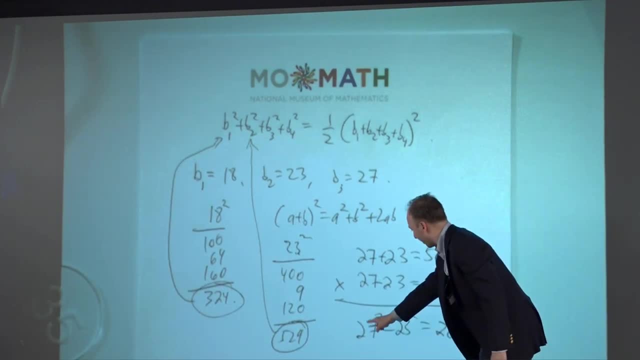 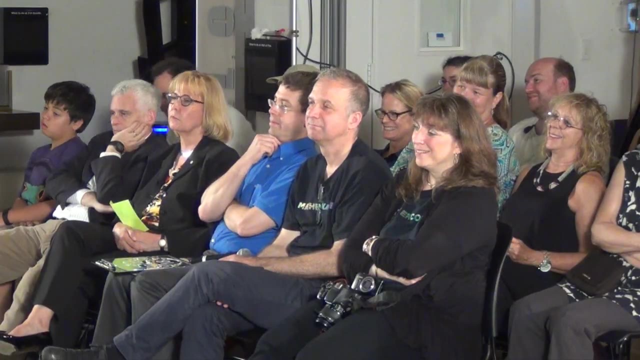 So that's pretty easy. So what that tells us is: 27 squared is just 23 squared plus 200. So it's just 729.. So 27 squared is 729. And that's what's going to go there. So now we need the sum of all three. 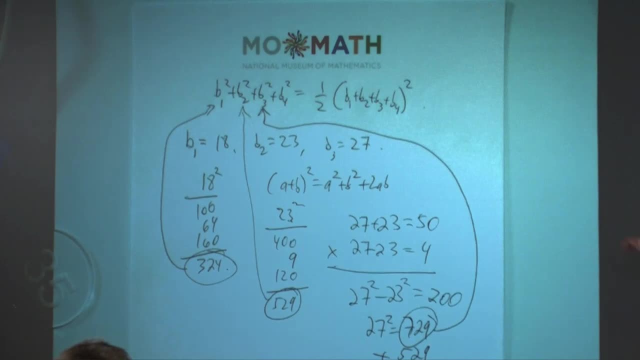 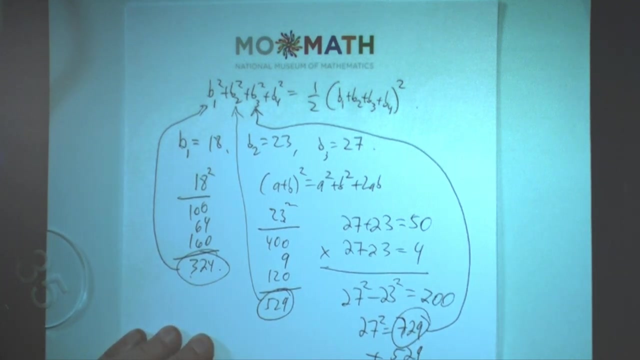 So 529 added to 729.. Well, 29 is like 30. So two 30s is 60. And there's a rounding error, And then that's a 12. And then I need a 324 added on top of that. 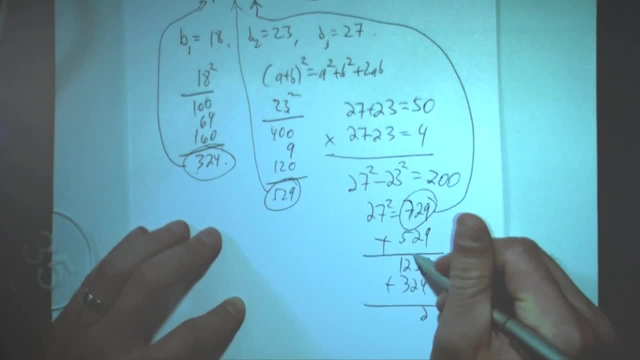 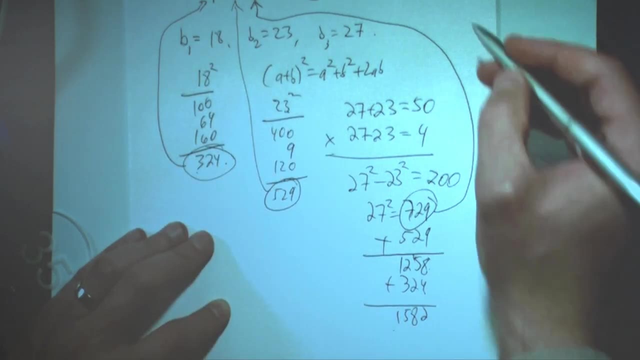 Thank you. Thank you. 8 and 4,. OK, This is embarrassing to do in public. I hope I didn't make a mistake. OK, So that's what we get on the right side. On the other hand, the sum of these three: 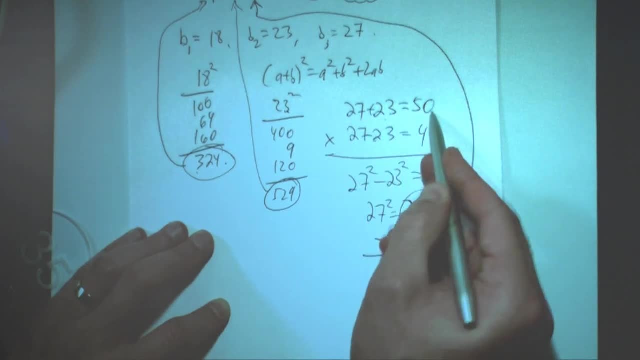 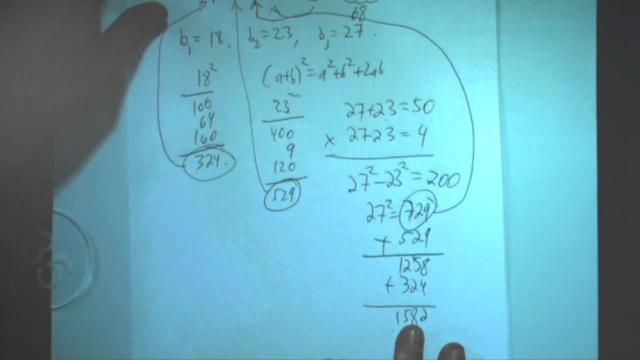 so b1 plus b2 plus b3, where we already know two of them add to 50. So that's 68. So far, so good. I don't like that one half. Let's move it to the other side. Can I do it like this? 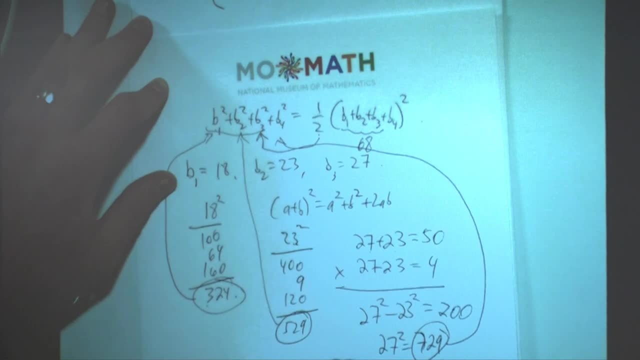 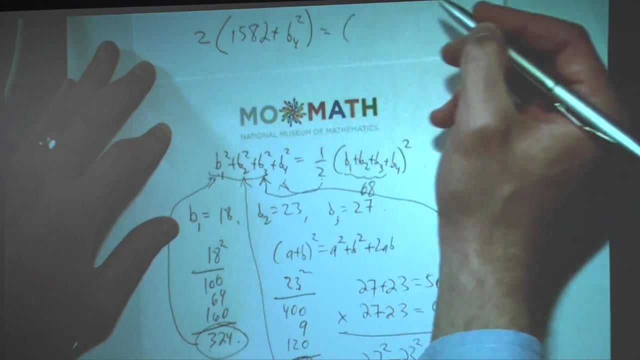 So if I move it to the other side I get two times Now the sum of these three. we already computed It was 1582 plus b4 squared, And on the other side I just get b4 plus 68 squared. 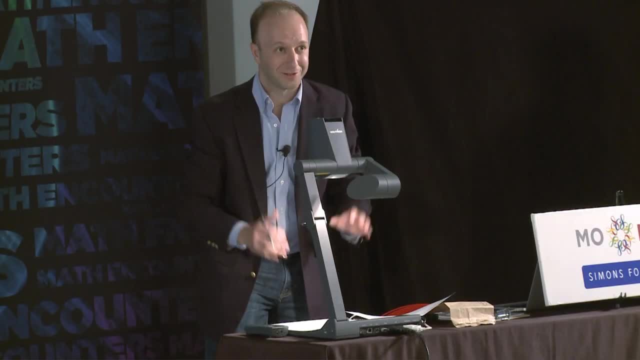 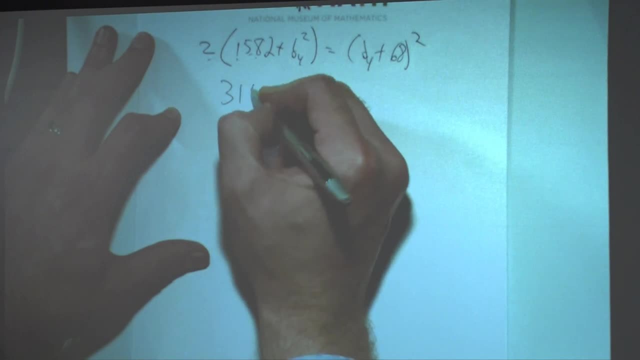 Everybody with me so far. If I'm going a little fast, just check it out when you get home. That's too hard. What? When I double this? 15 doubled is 30.. 8 doubled is 16.. 2 doubled is 4 plus 2b4 squared. 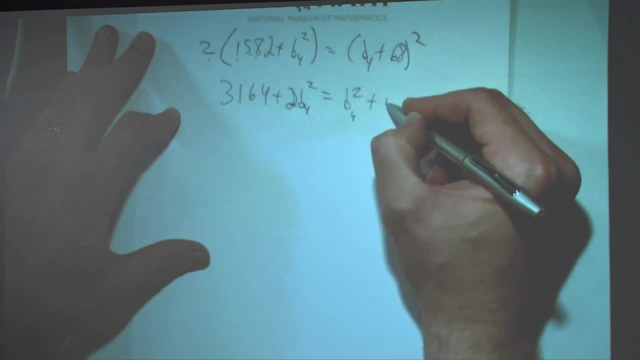 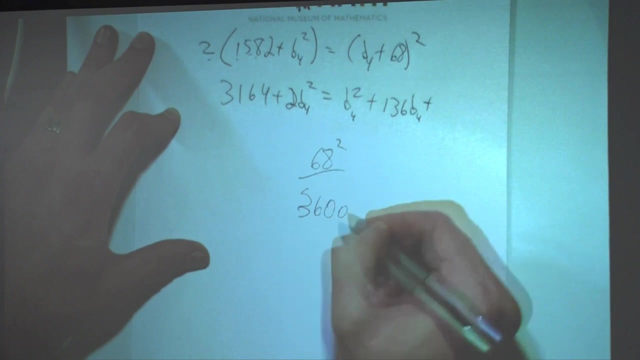 On the other hand, I get a b4 squared Double 68 is 136.. Is that right? And then I have to square 68.. So again, square 60 is 3,600.. Square 8 is 64.. 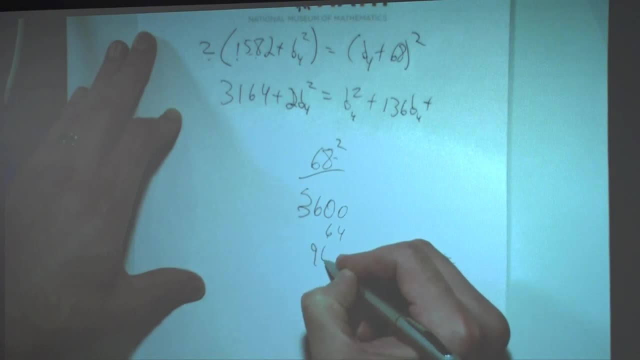 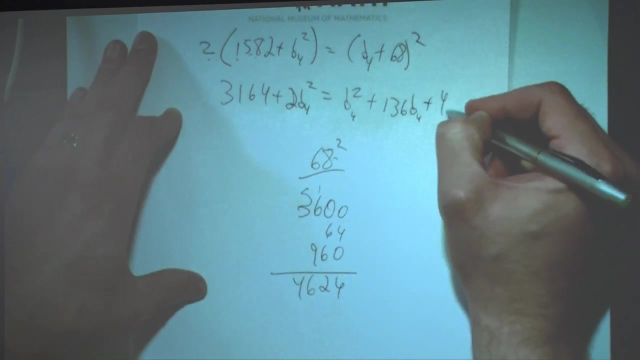 This is 4,896 if I double 48.. And that's a 4, 2, 1,, 6,, 4.. OK, So something like that: 46.2.. 46.24.. OK, Now I want to collect terms. 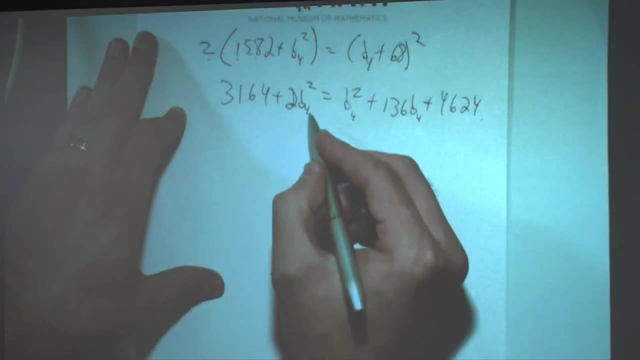 Algebra: we're OK so far. There's a 2b4, so I'll bring everything to that side. So I'll kill one of these and one of these. So I get a b4 squared minus 136b4.. OK, what's this difference? 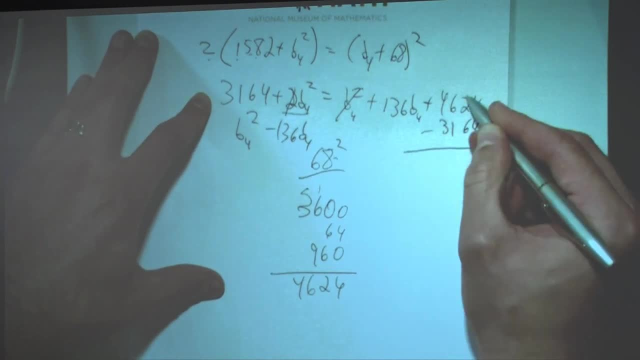 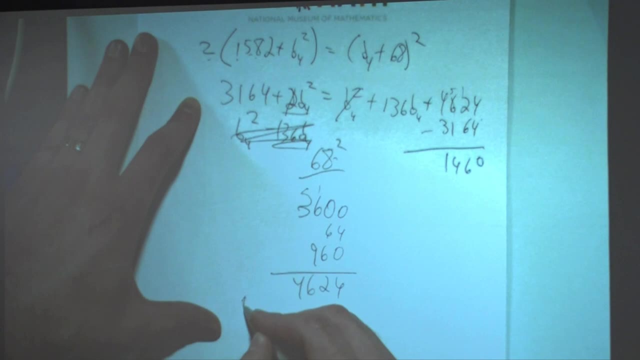 So 31,, 64.. The 4's cancel. I need to borrow a 5, 4, and a 1.. So 1460.. Let me write this somewhere. So I have b4 squared minus 136b4 minus 1460, because I 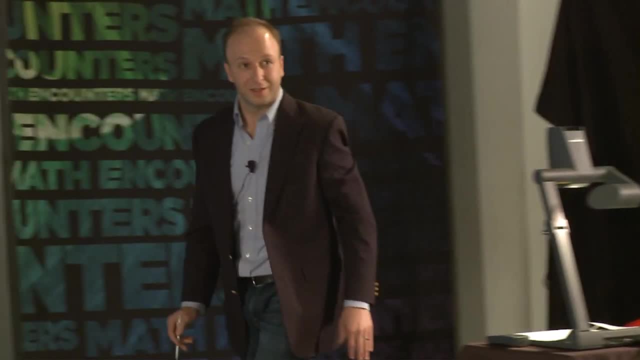 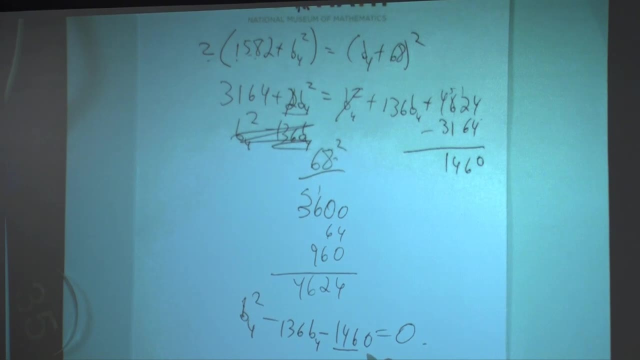 brought it to the other side, equals 0.. So far, so good. OK, Now we need the quadratic equation. Actually, this one's a little easier than that. Here's a 146 and a 10. And this is a 136. 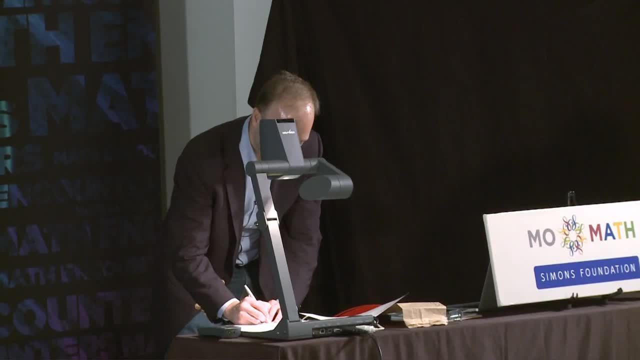 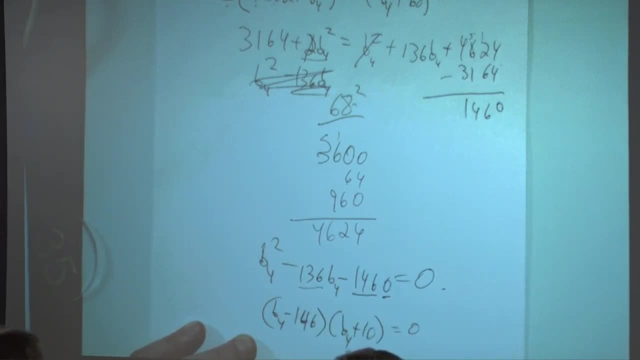 So that tells us it's going to factor. nicely, I think we can do minus 146 and b4 plus 10, and that should do it. So that gives us our answer. b4 is indeed 146.. So answer C was correct. 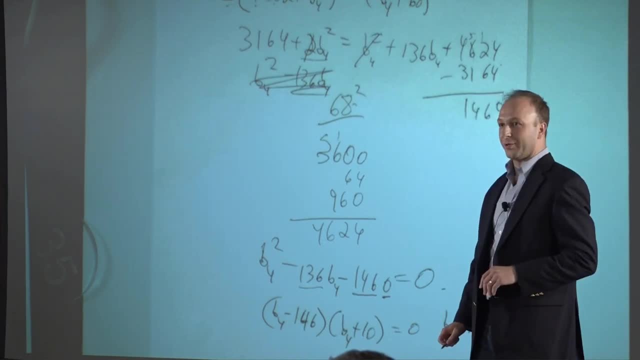 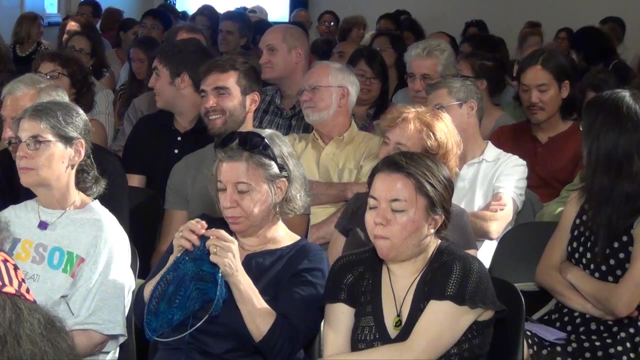 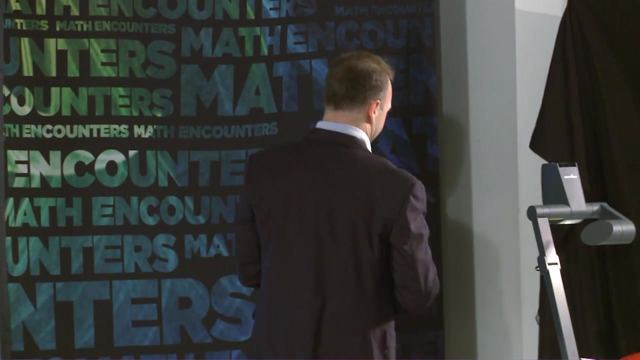 Most of you got it. Any questions? How did? Question? I just found from the. So the question was: if we go back to Descartes, let's do it right here. What did Descartes do? He was given three tangents. 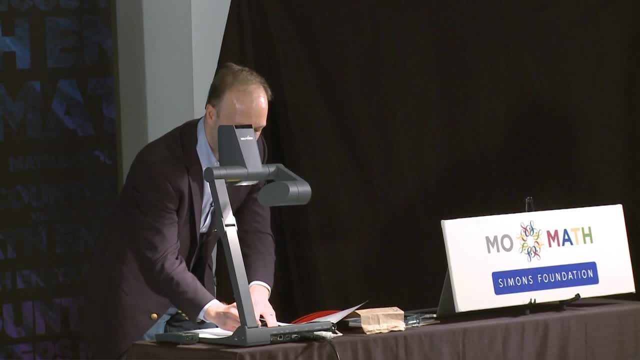 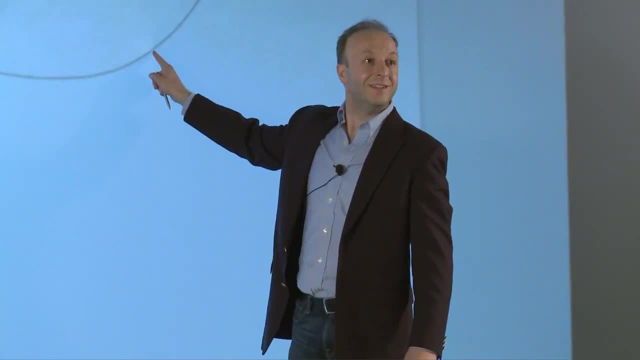 He picked tangent circles and he picked one point of tangency and made a circle, And the question was: how did he determine the radius of this circle? The answer is: he didn't. Any circle works. It doesn't matter how you reflect, because all you're 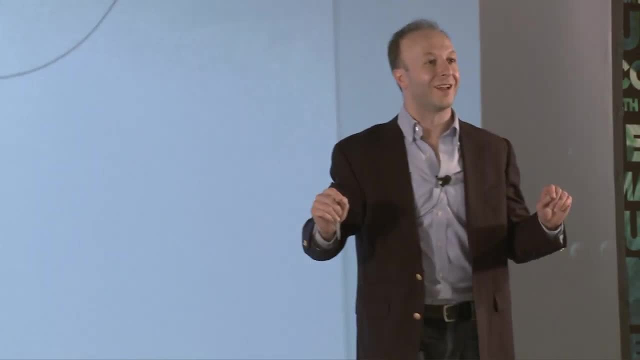 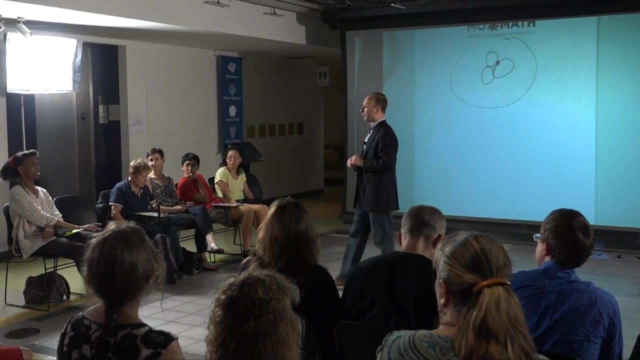 going to do is reflect back and undo any difference in the radii. Excellent question. Excellent question. Other questions: Yes, ma'am, When you started off, you said it has to be perfect too. Yes, I am very interested in what made it perfect for this. 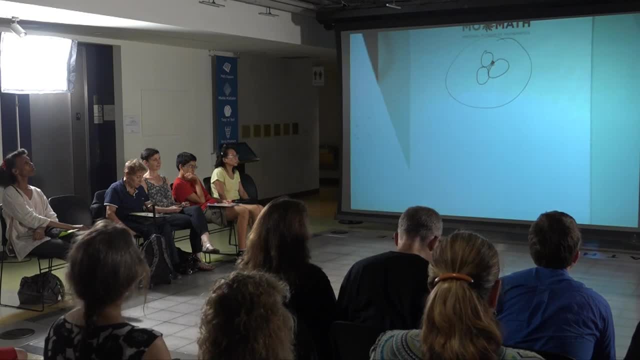 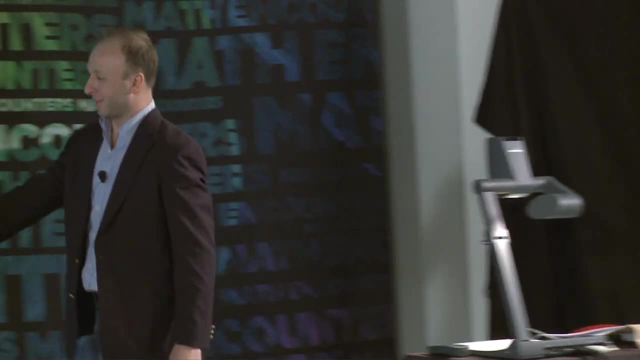 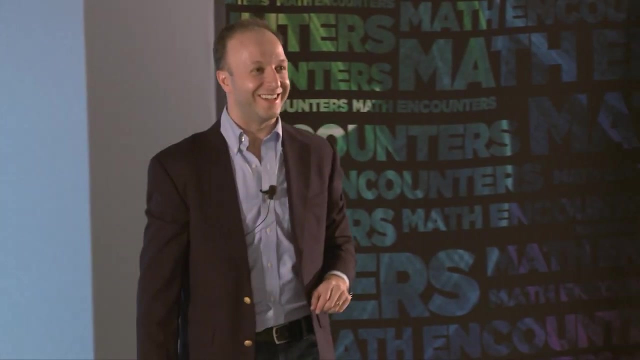 So we know that they Yes, that they're exactly tangent, that there's no. Well, that's what this tells us. There's only one solution, Or is there? Thank you, Somebody saw it. There's something wrong, Or maybe there's not something wrong, right? 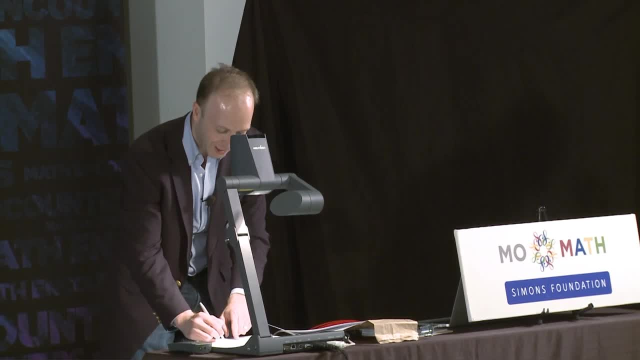 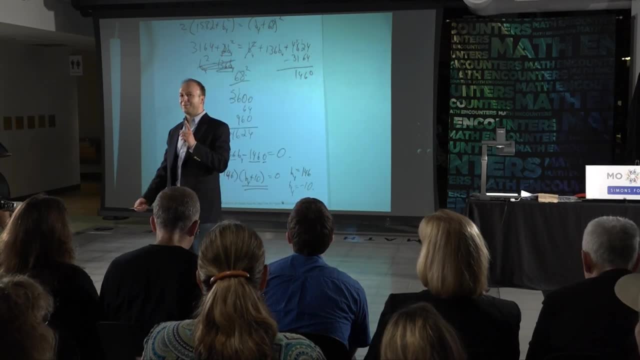 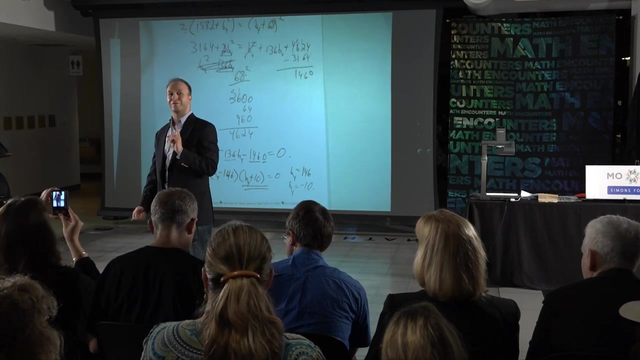 We have another solution. B4 is also equal to negative 10.. Well, that's obviously nonsense, right? How can you have a negative radius? Sometimes math answers questions that you haven't asked yet. You should always take all the information math gives you and 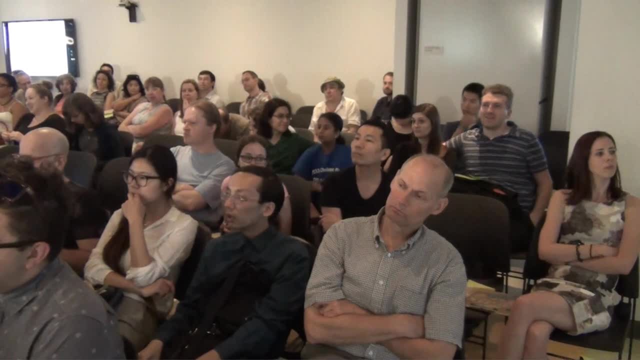 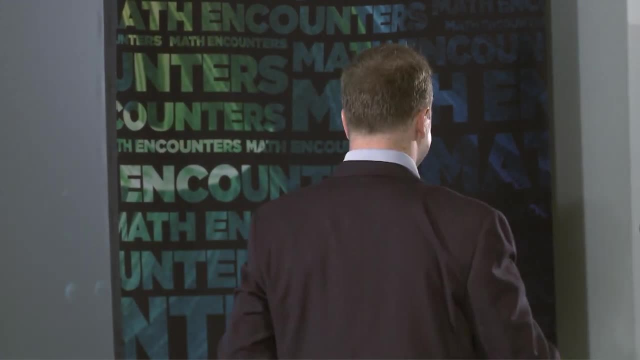 try to figure out what it means. There was a question back there, sir, I was just going to answer it, that you draw the circle around. Excellent, Excellent. The answer was: what does this negative 10 have to do with anything? 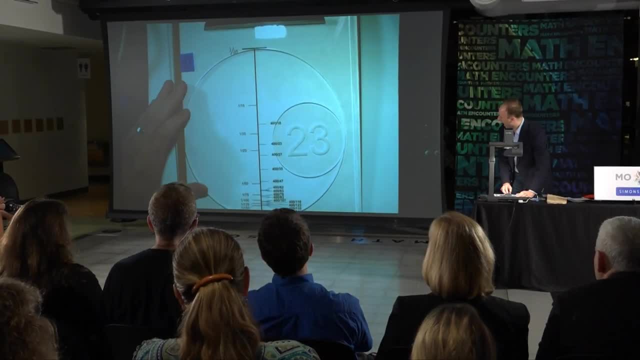 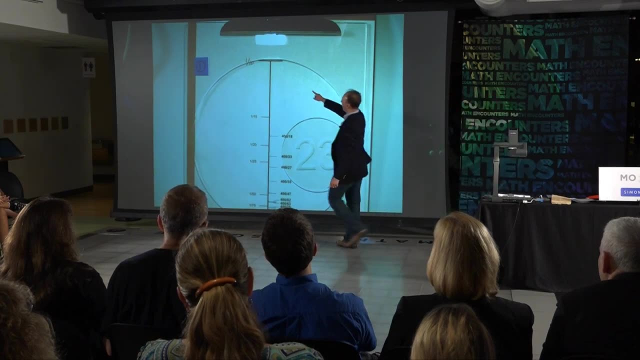 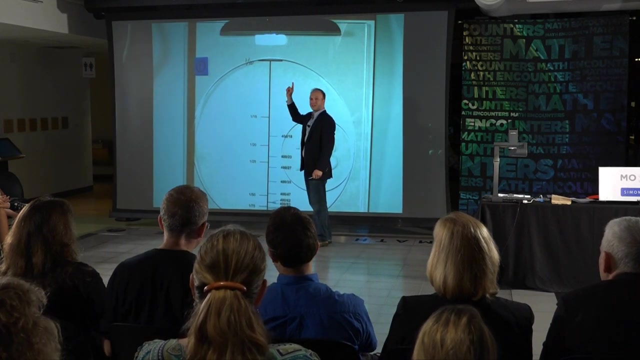 This gentleman noticed That the outermost disk, which is a hole, has mommath curvature 10, because that's a 1 over 10 mommath. So the bend of this outermost circle is 10.. What's with the minus sign? 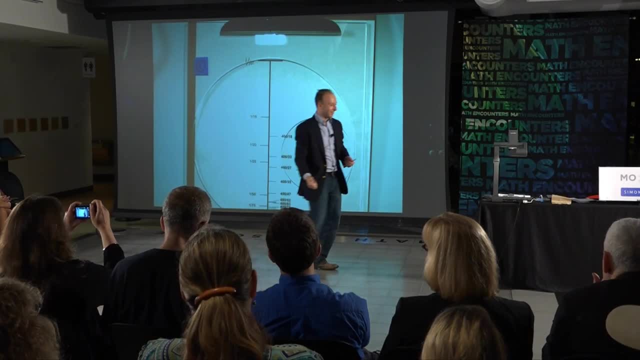 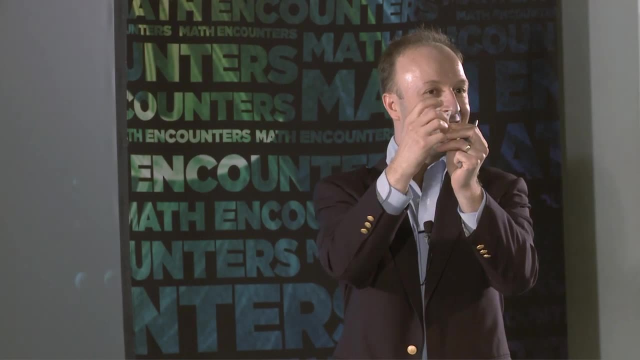 The material is on the outside. You see all of these circles. well, they're not circles, They're disks. They have material And the material is on the inside. The orientation of this one circle is backwards. The material is on the outside. 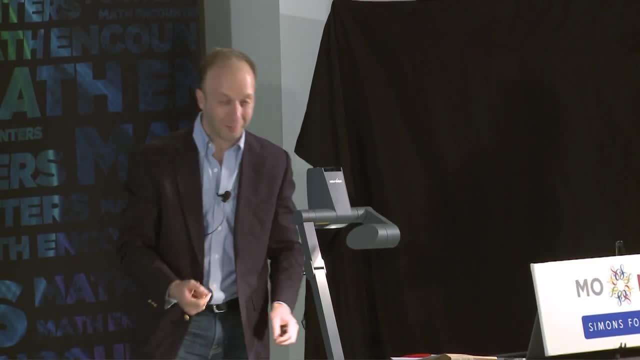 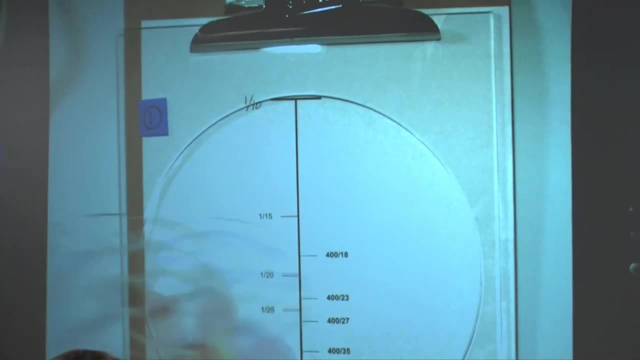 That's what the minus sign is about. The minus sign is to remember the orientation. And let's look again When we took our 18 and 23 and 27 circles and everybody was thinking about: well, how do we get that? 1. 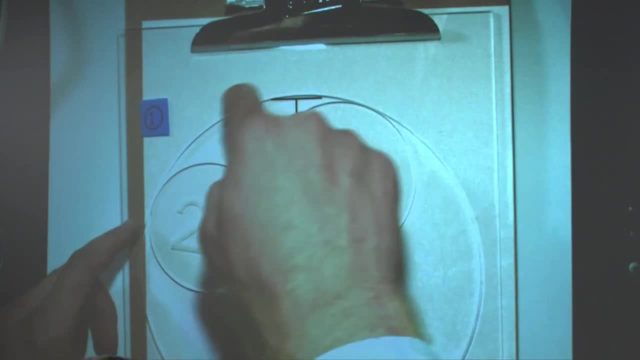 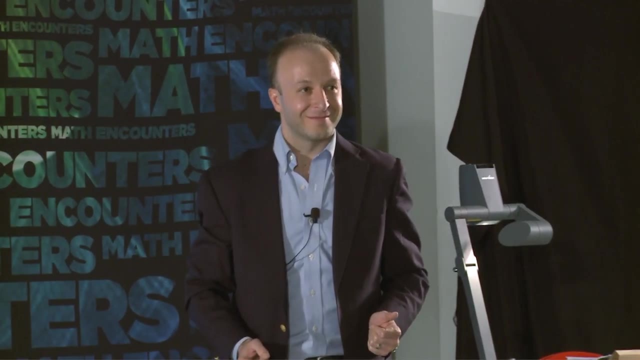 and 46 on the inside. Actually, there's another solution to the Apollonian problem, which is the one around, And that's what Descartes finds algebraically. So never throw away an answer. Always try to understand what it means. 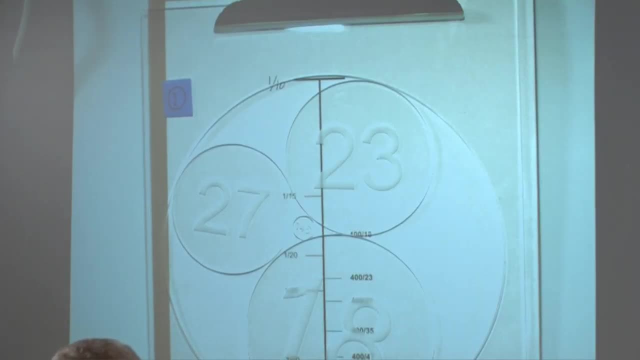 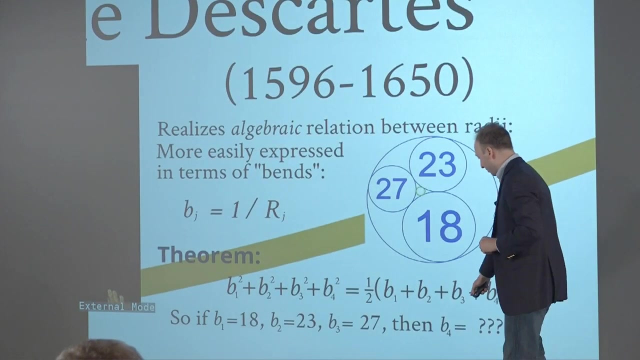 OK, so that's what our perfect curvatures look like. So that tells us the answer to what b4 is. It's 146.. But there are two b4's b4's and the other one is negative 10 because of the. 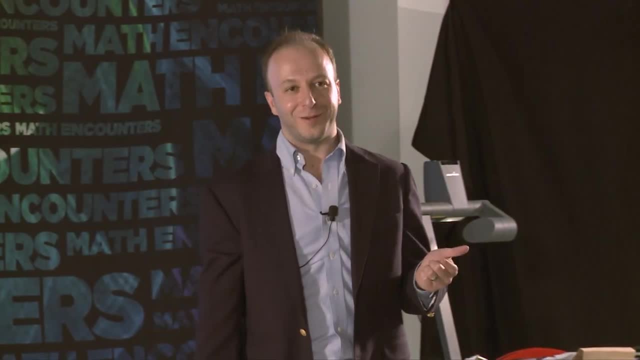 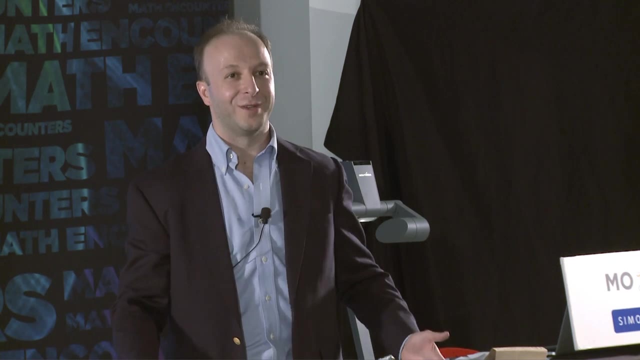 orientation. It reminds me of this joke: There's an engineer, a physicist and a mathematician and they're given 15 feet of fencing And they're told: enclose as large an area as you can. And so the engineer makes a 17-gon, and that's really. 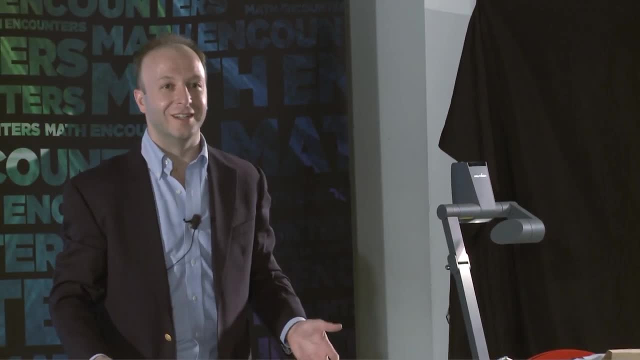 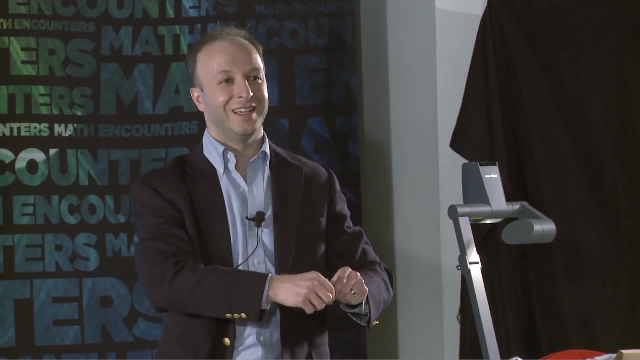 quite good. That encloses almost all the area you possibly could. And then the physicist computes. well, actually you can show by variation of calculus- it's even easier than that- that the circle is the thing that will enclose the most area. 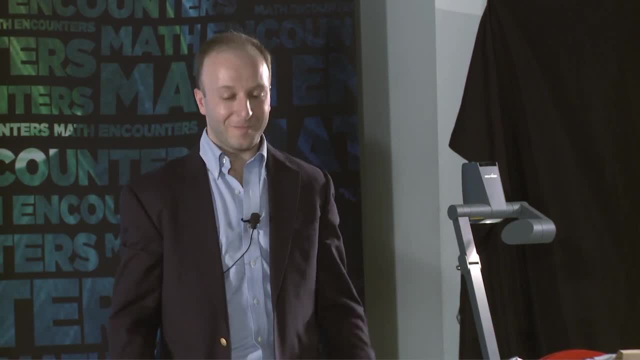 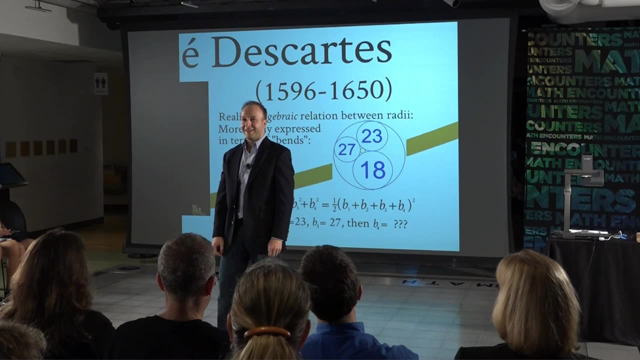 So he uses all 15 feet on the circumference of a circle and says: there, I've done it. And the mathematician just takes three little pieces of fencing and encloses a tiny little thing like that And the physicist and engineer what the 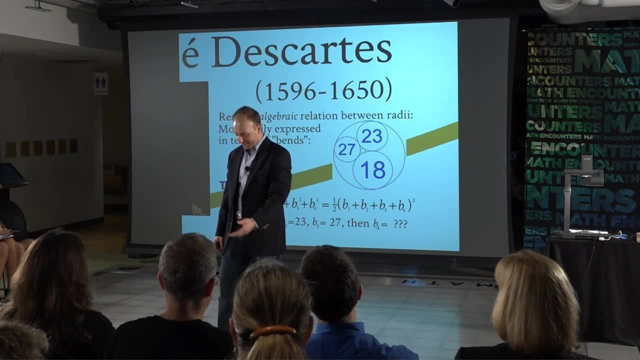 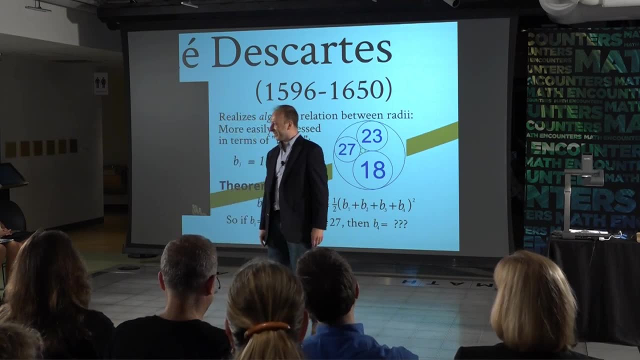 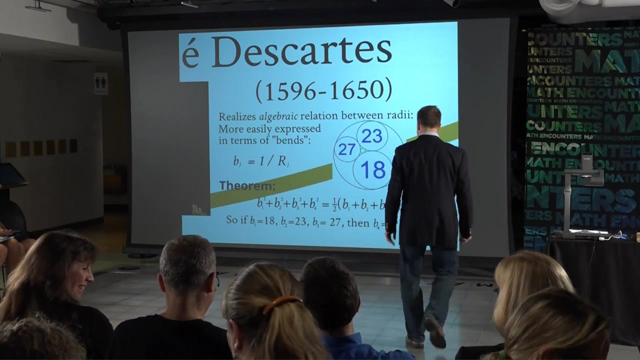 heck, what are you doing? You missed the point of the game. The mathematician says: no, that's the outside Orientation. It takes a Wednesday night crowd that'll go to a math museum to understand that joke. All right, You guys got it. 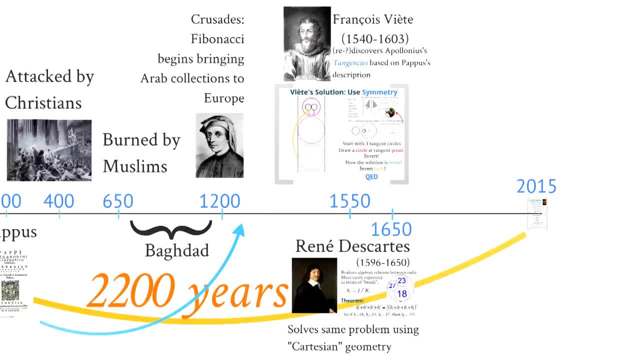 I'm impressed. OK, So that's what we learned from Descartes: The algebraic relation as opposed to the geometric relation. the story doesn't end there. Our next laureate is Leibniz Wilhelm von Leibniz. 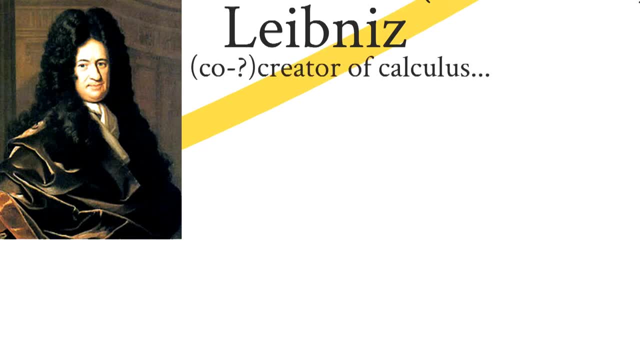 If you're German, maybe he's the creator of calculus. If you're British, he's a lying thief. Another story for another time. In fact, it's the topic of one of the encounters that you should go to YouTube And see. 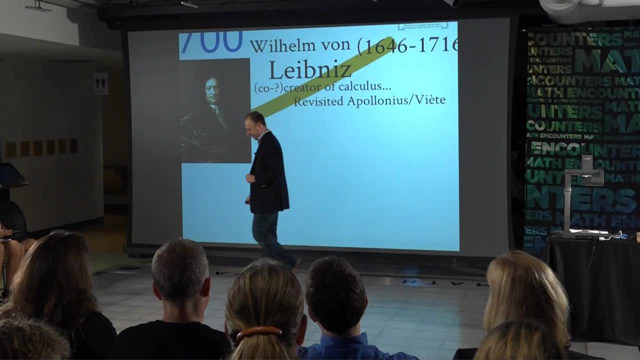 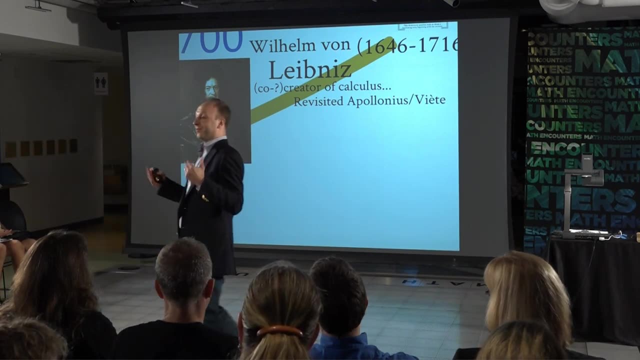 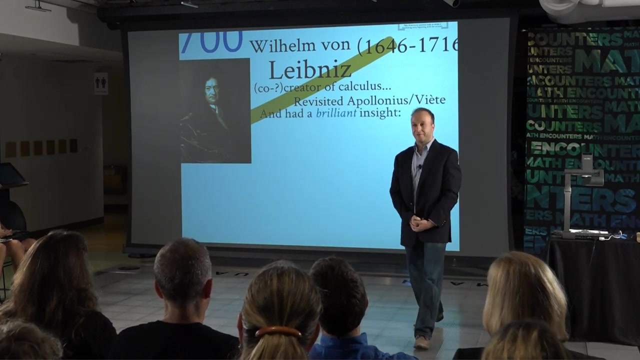 Like all the other mathematicians and scientists before him, he revisits geometry and all this- just every mathematical piece of information known before that time, including Apollonius and Biet's construction, And he has yet another brilliant insight that everyone else missed. 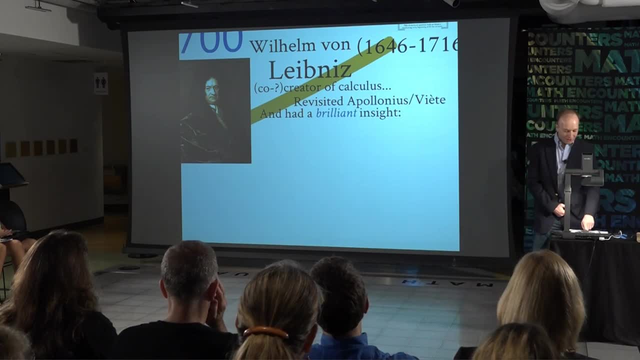 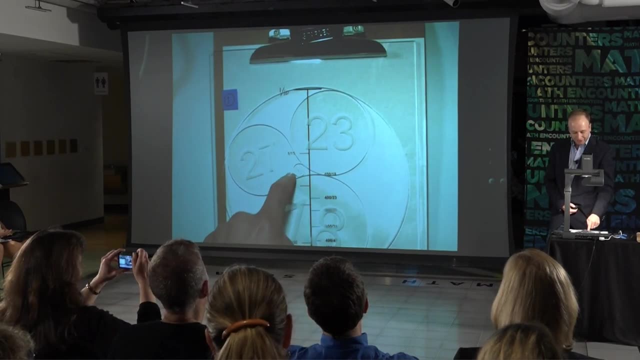 Once you've put in one circle, what's stopping you from putting in Once you've put in this one guy? well, what have you really done With straight-edging compass? you've constructed, you've inscribed a circle in this curvy linear triangle. 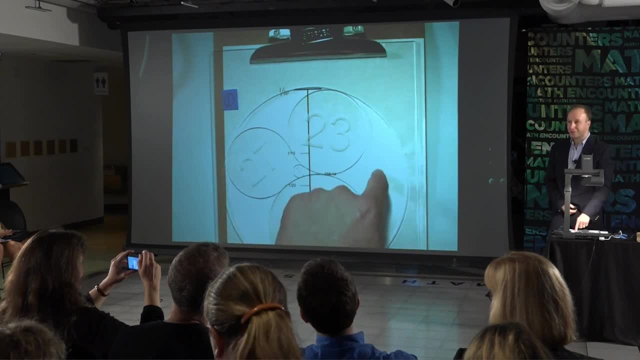 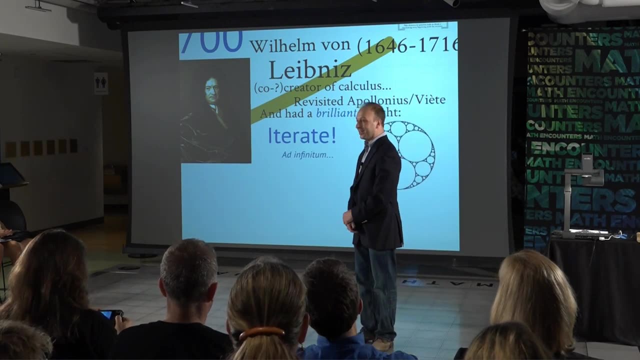 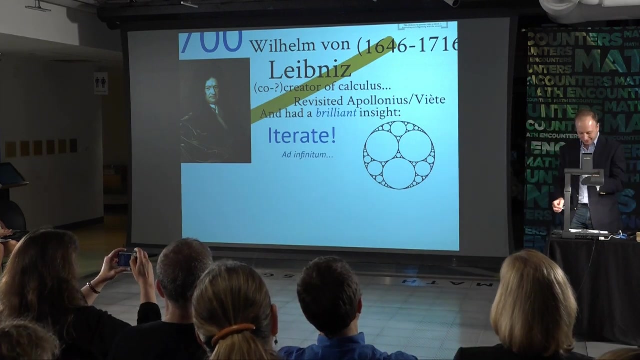 What about this curvy linear triangle? What about that triangle? What we should do is we should iterate forever, And what we'll see is a beautiful fractal. So I invite you now. all of these disks are actually disks that will fit somewhere in the picture. 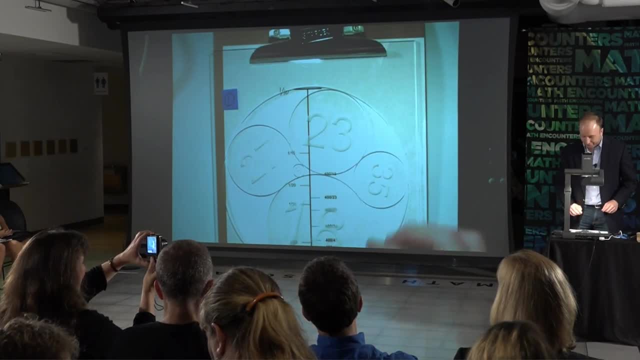 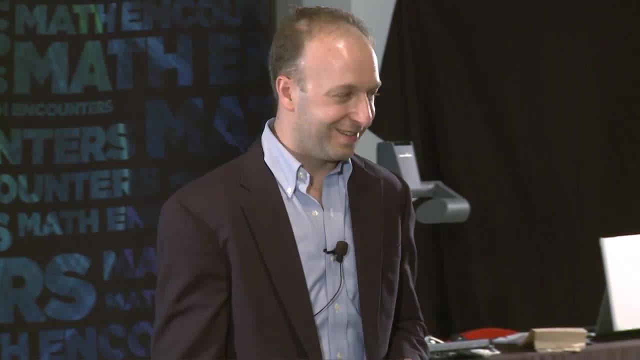 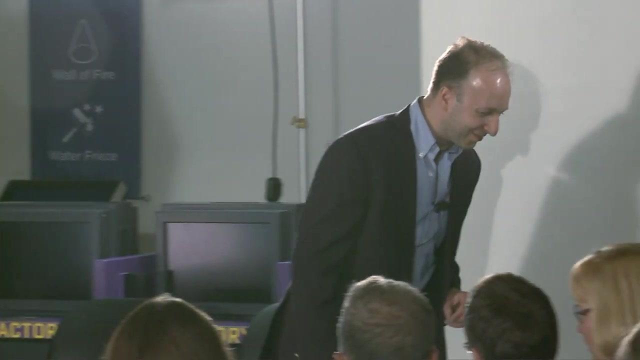 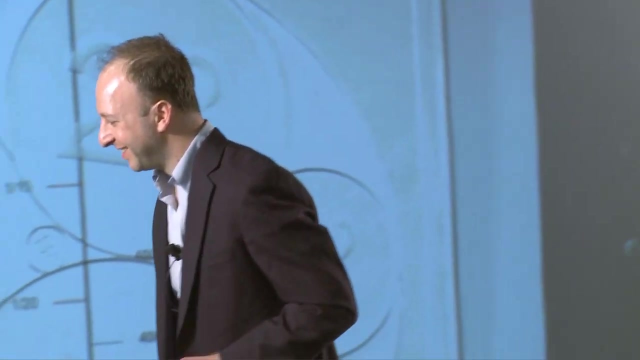 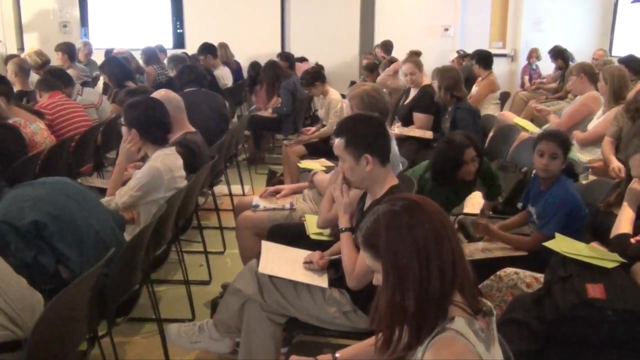 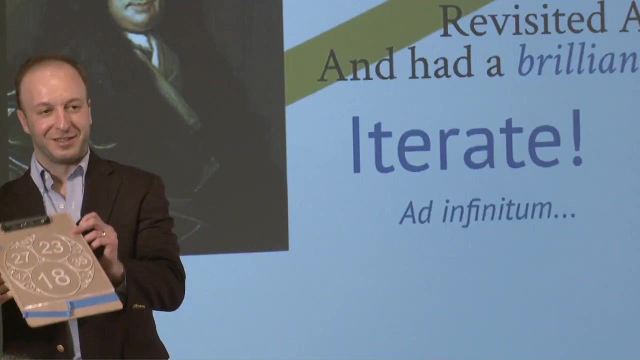 And you have to figure out where they go to perfectly lock in Use people next to you. You need your friend's help. Oh, you did it already. Yeah, looks good, You got them all. That was quick. Here's the finished product right here. 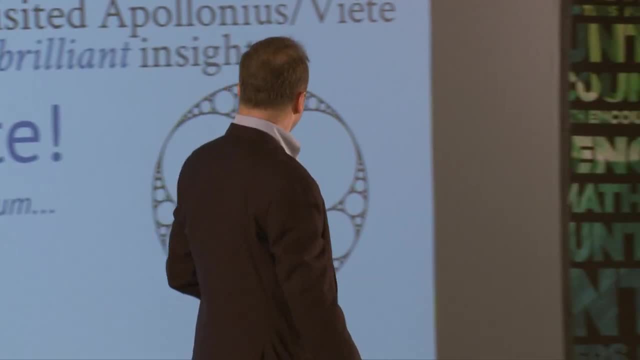 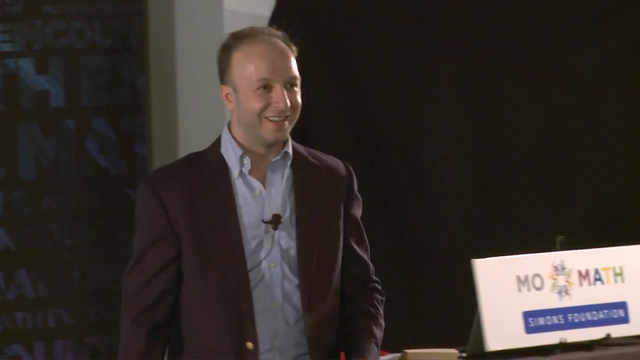 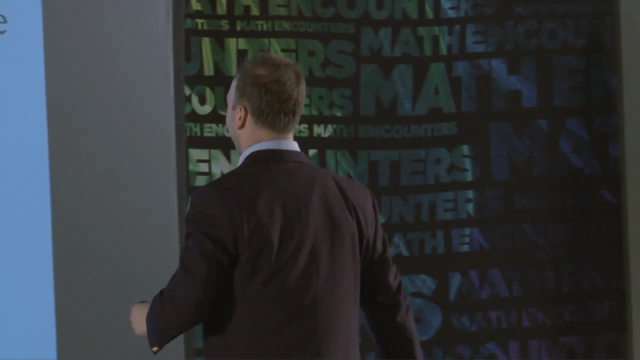 Well done, Well done. So you see, this is again. this is the ideal object. This is, if we had infinitely many hands and infinitely much time, if we were sitting in Dorian's cave for years and years and years and for eternity, putting in circles. 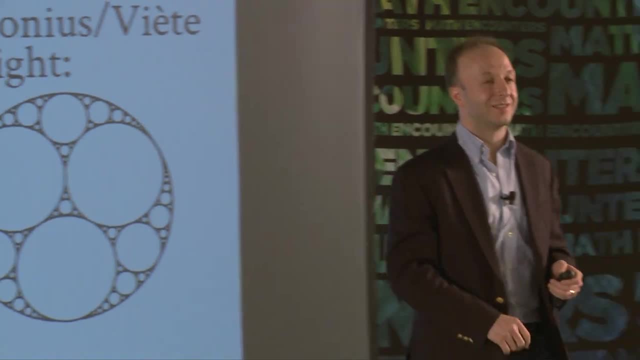 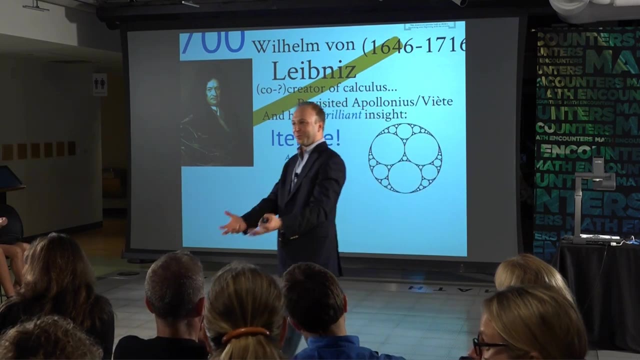 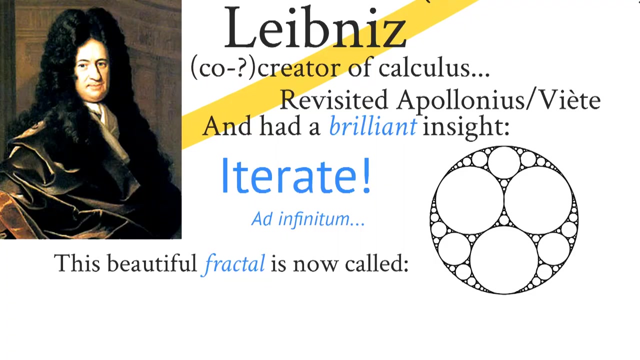 forever, We would get this ideal object And this beautiful object. so you have a finite piece of it. We're in the physical world, We're not in this ideal platonic world. But this beautiful object is a fractal, as I'll explain in a second. 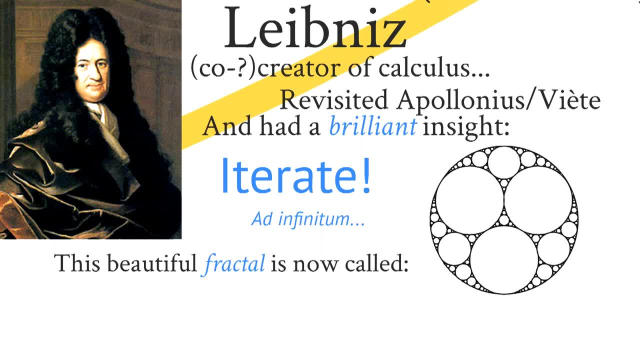 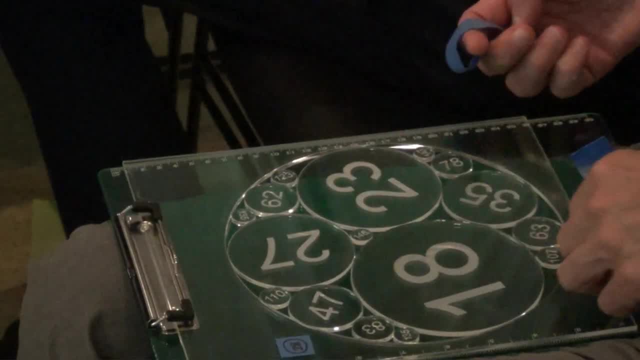 And what is this thing called A Leibniz circle packing? What are the numbers? The numbers are the bends. So it's one over the radius, Yeah, OK. So it's a Leibniz, Oh no. 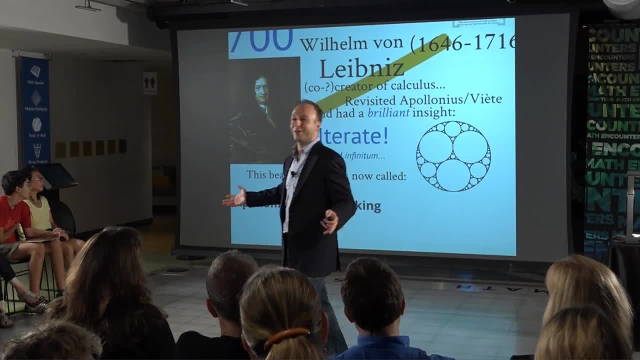 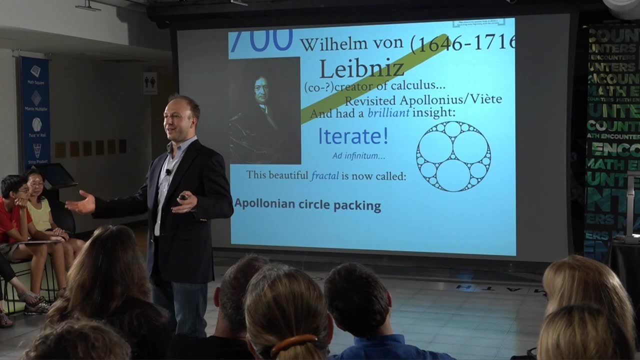 Sorry, It's not a Leibniz circle packing, It's called an Apollonian circle packing. OK, So this is an inverse axiom. You know, in math there's nothing. What's the guy's theorem? That in math there's nothing named after the person that? 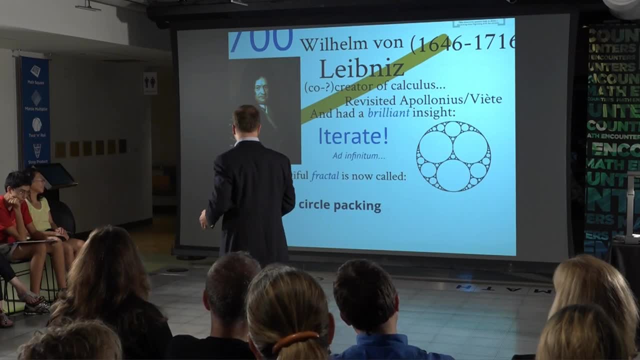 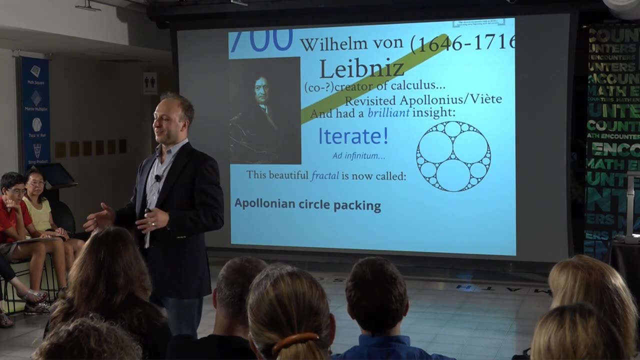 actually discovered it. So this name- the Apollonian circle packing- is actually a name from the 1950s. So somehow people realized that things weren't being named for the person. It's always someone like 100 years after the actual discoverer. 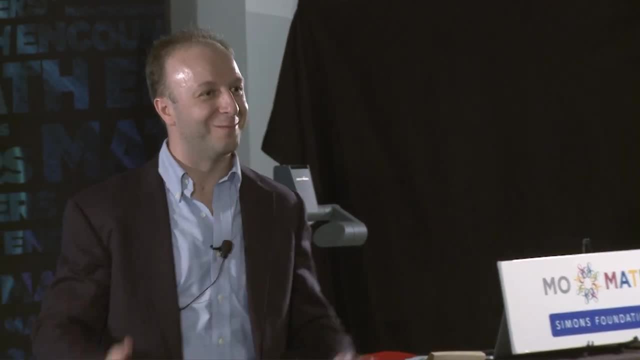 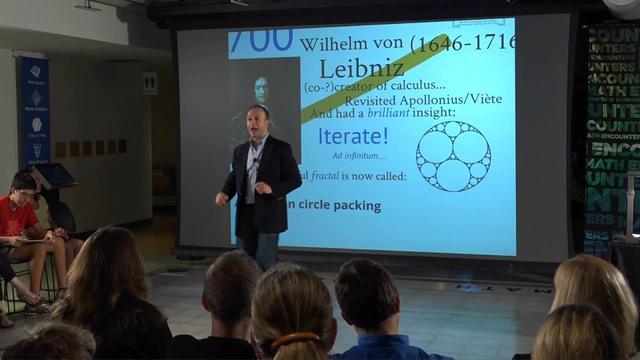 So this time they went 1,000 years before the actual discoverer to give the name Should have gone to Leibniz for some reason. OK, Apollonian needs his credit, So it's called an Apollonian packing. 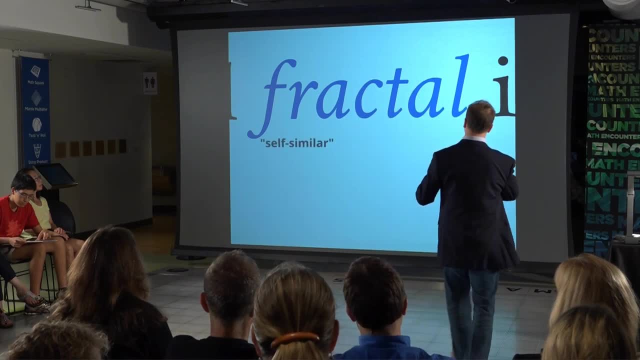 Now, why fractal? So what do I mean by fractal? Well, first, let me give you a very simple thing. It's something that's very self-similar. So here's one way to tell that this thing's a fractal. 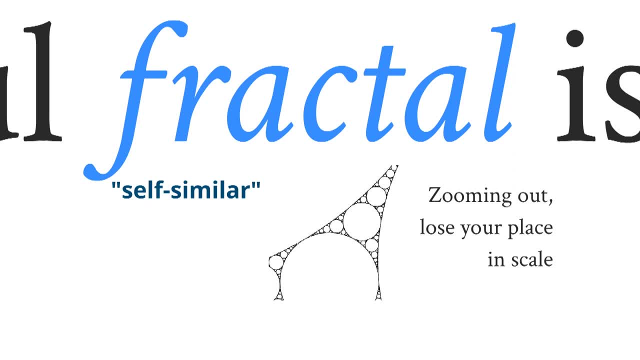 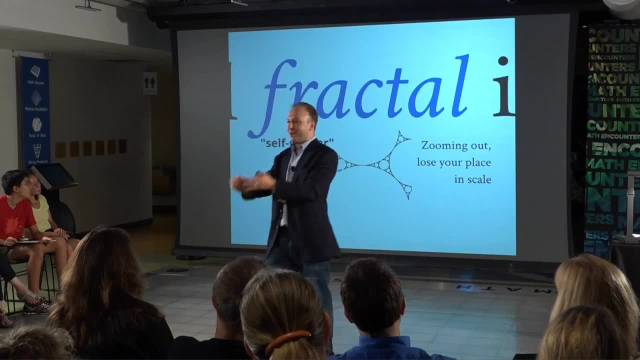 If I zoom way in and I start zooming out, it's impossible to tell what scale am I on. Am I on a level of nanometers, millimeters? Am I on a macro scale? Everything looks the same until you get to the very end. 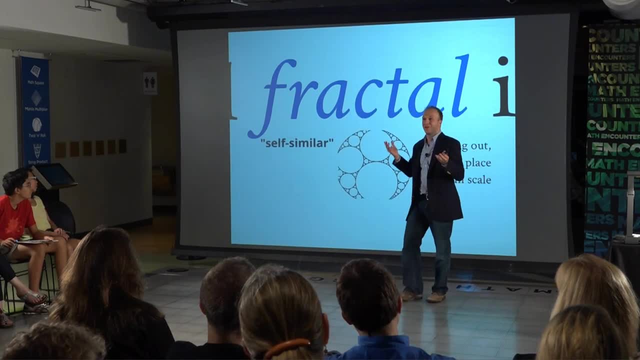 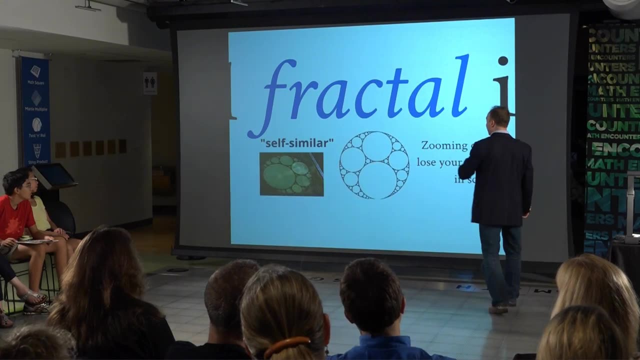 And then you say, oh OK, here I am, But all the way inside there's no way to tell where you are, And so when you zoom out you lose your place in the scale, And in fact aliens were so interested in this. 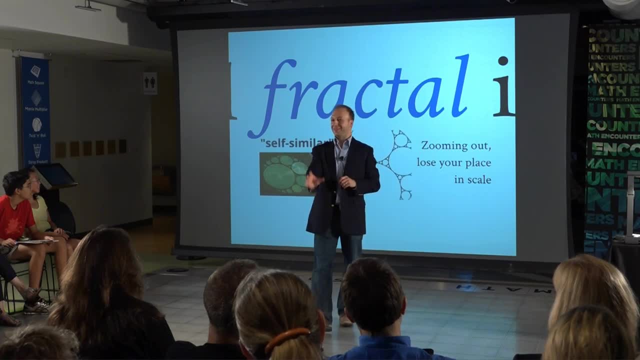 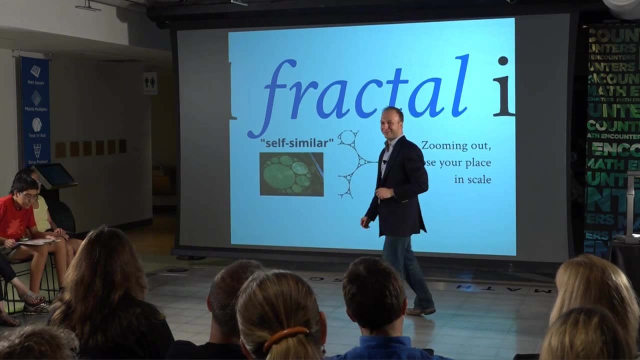 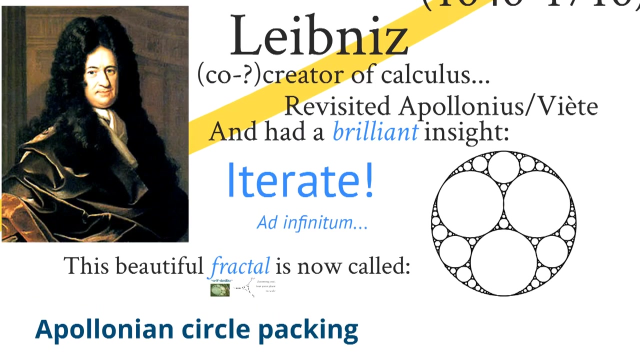 they built spaceships and landed them in England, cornfields. It's actually from a BBC special on crop circles. OK, so that's our self-similar fractal. Now it's more than self-similar. This picture has a beautiful symmetry. 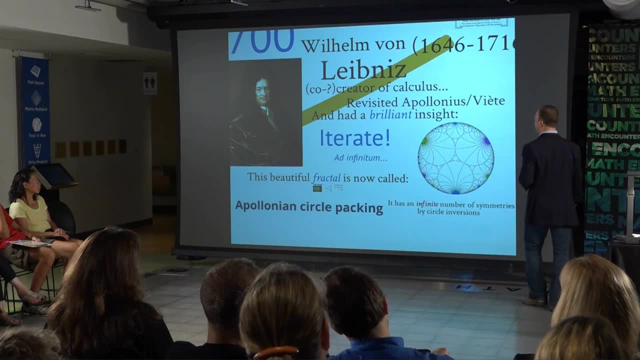 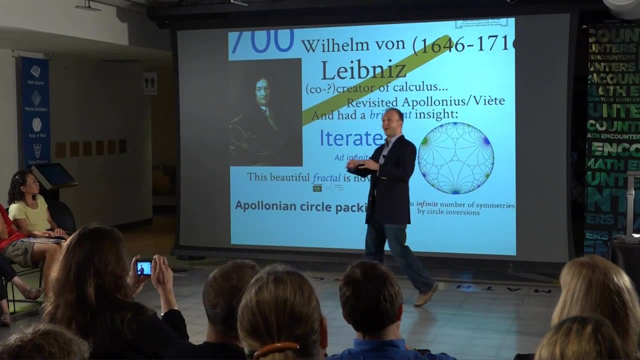 In fact it has infinitely many symmetries, And the symmetries are by circle inversions, So let me show you just one of them. It doesn't work for any finite set. You need the entire infinite fractal. So let's take this little circular arc. 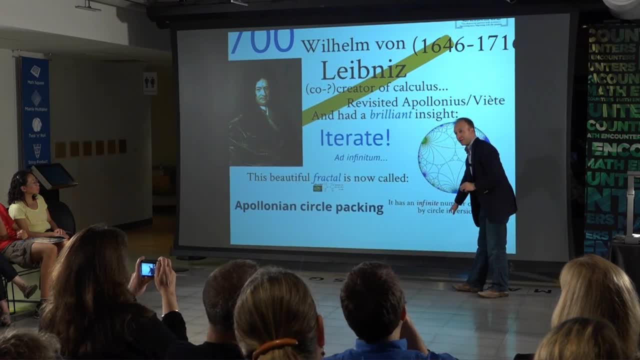 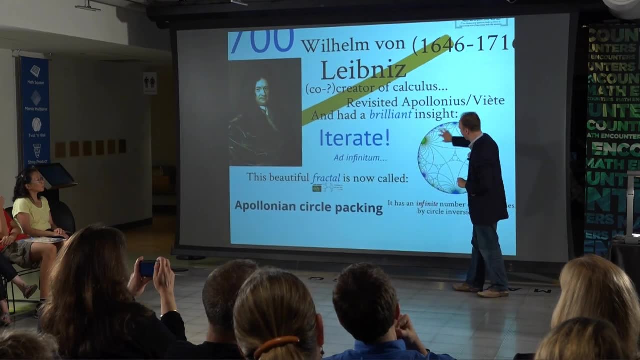 which represents a circle, And we'll invert everything through this circle. Now, remember, circles go to circles, So this circle under inversion reappears right there, And that circle reappears right there, And that circle reappears right there. 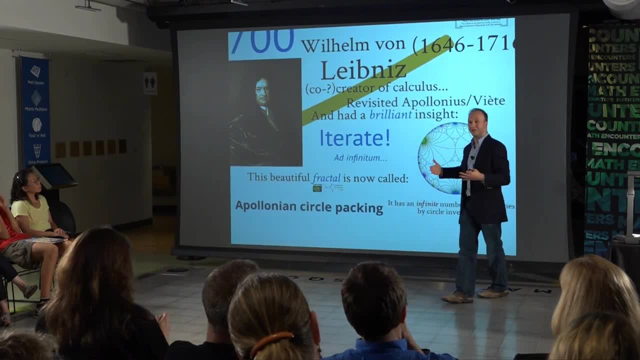 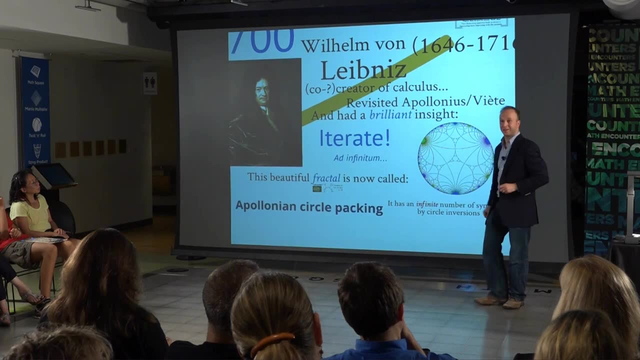 And everything is fixed and vice versa. So the entire image is unchanged, under this reflection and also under this inversion, and also under this inversion and many more than I'm showing you. And those symmetries are the symmetries of the hyperbolic disk, as you heard from Dorian. 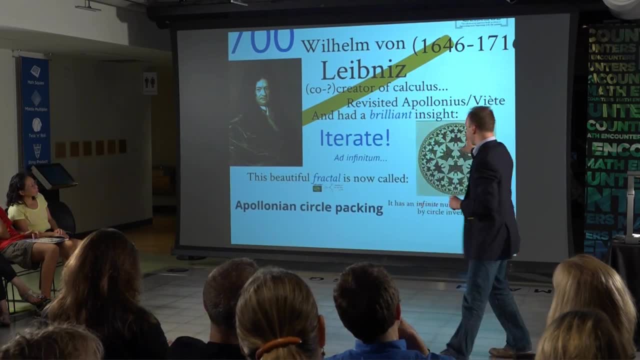 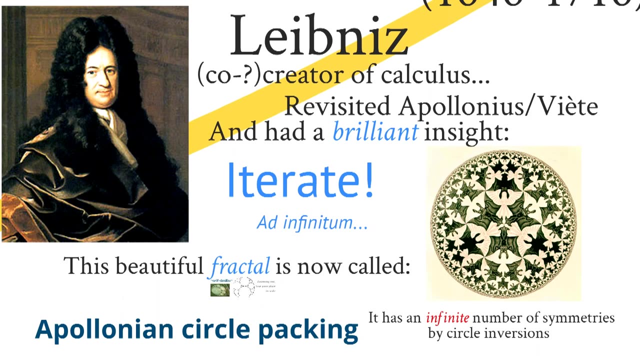 There's some non-Euclidean geometry. We won't go into it at all, except I'll mention this Escher sketch and many others that employ exactly the same symmetries. So that's the symmetry. Now let's look at this picture. 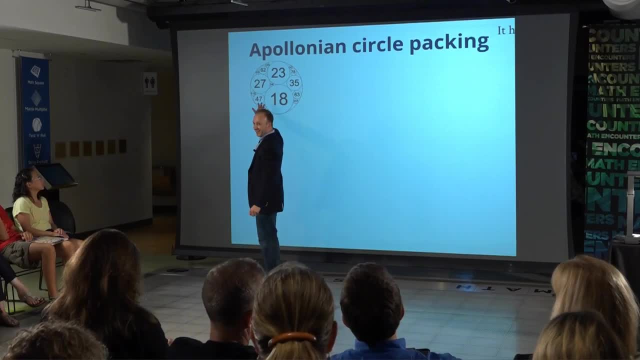 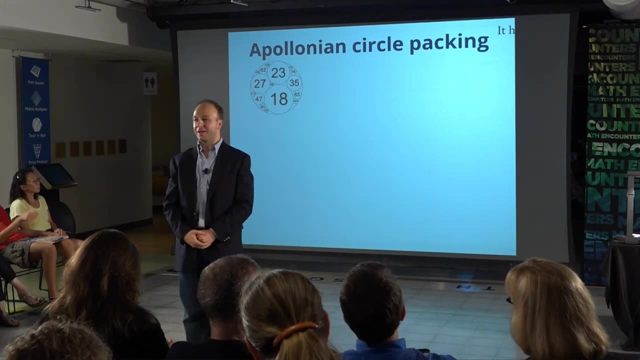 So I hope everybody got it to look like this at some point. Again, there could be some physics interfering and some numbers may be misplaced, But roughly that's what you've looked at. How many disks are there Inside or outside? 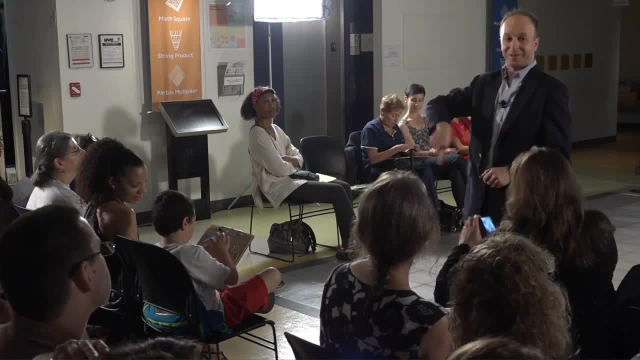 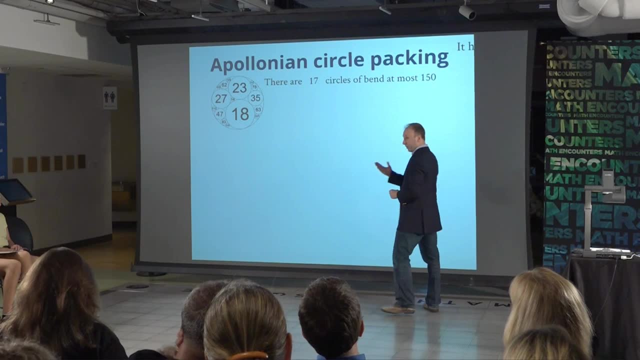 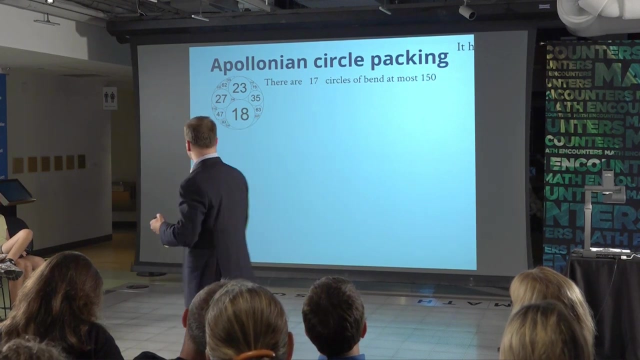 16. And the outside ones. So there are 17 total. So there are 17 circles in this packing of curvature of bend, at most 150.. Now if you give yourself more circles, it'll take you a long time. 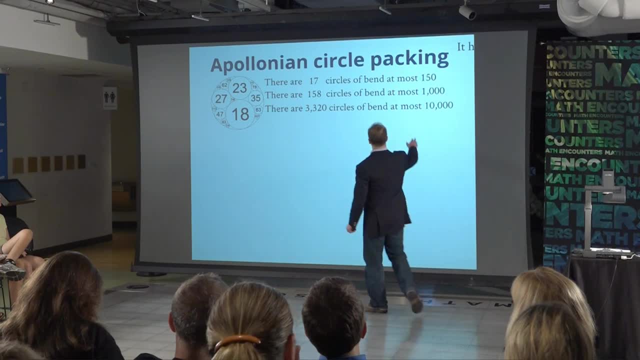 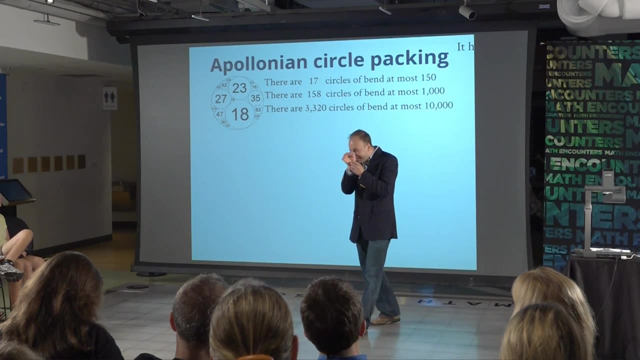 But if you go all the way out to 1,000 circles or 10,000, well, if you take all the circles in this packing of bend, at most 1,000. So it's radius 1 over 1,000, these tiny, microscopic things. 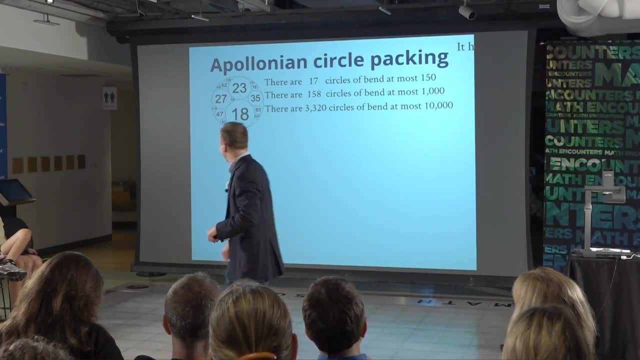 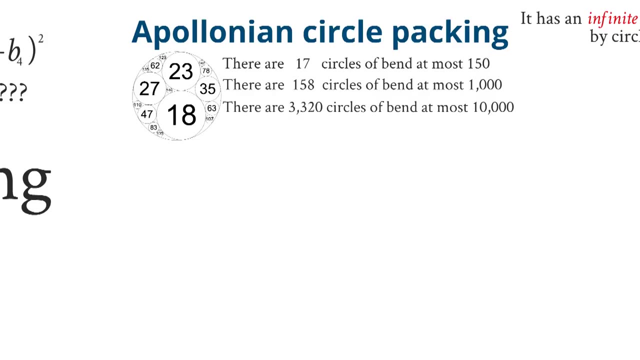 You need pliers- diamond guys are putting them in- You'll get 158 circles And if you go out to 10,000, now it's really nanobots are putting them in- You need 3,320 circles. Is there some pattern? 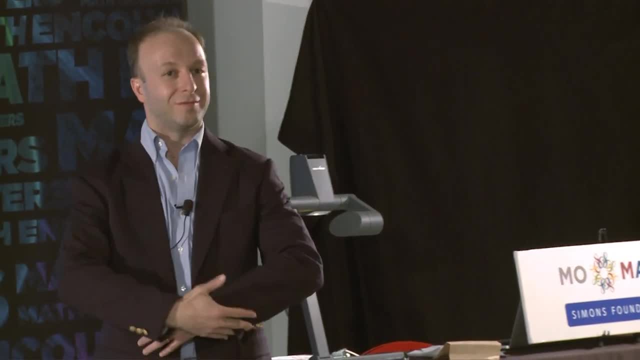 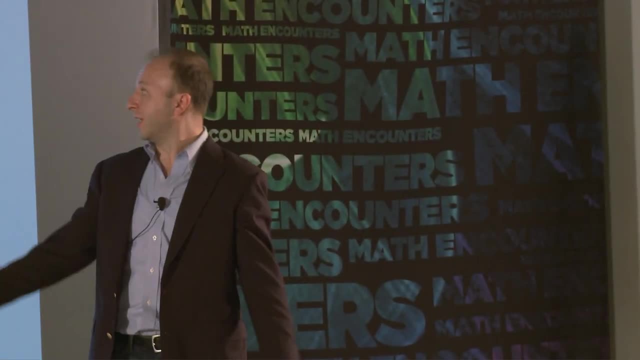 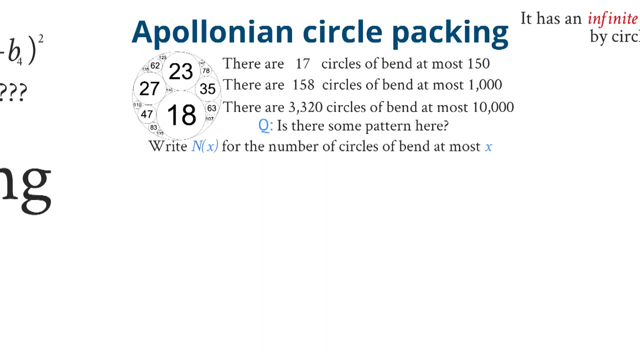 Can you predict how many circles you'll need to sieve to include all of the circles of bend? at most a million or something. Well, let's look at the data. So let's sorry for the math notation. So if n of x is the number of circles of bend, at most x, 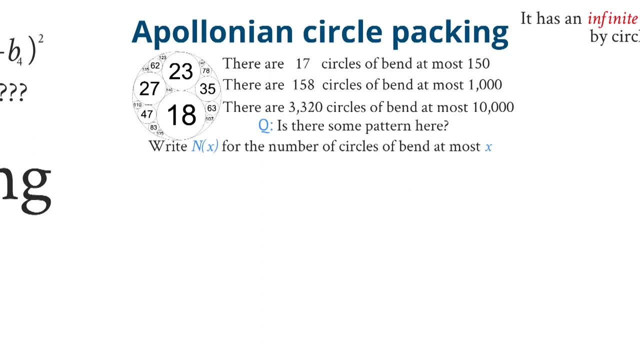 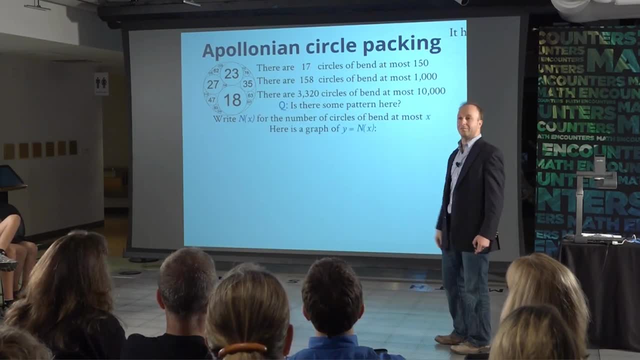 In other words, n of 150 is 17, and n of 1,000 is 158, and n of 10,000 is 3,000, whatever. Let's look at a graph of that function, And here it is. 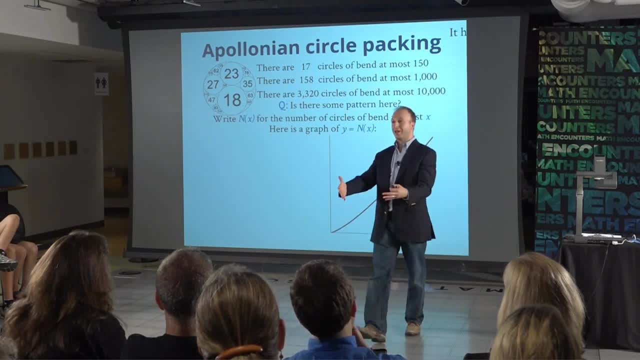 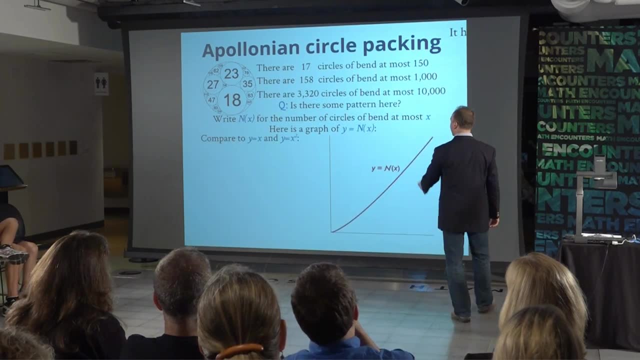 It's this pretty little curve, And maybe that curve will help us understand how many circles you'll need with bend: at most a million. Well, it's hard to see what's really going on. Let's compare it to the graph of y equals x, which is a straight line. 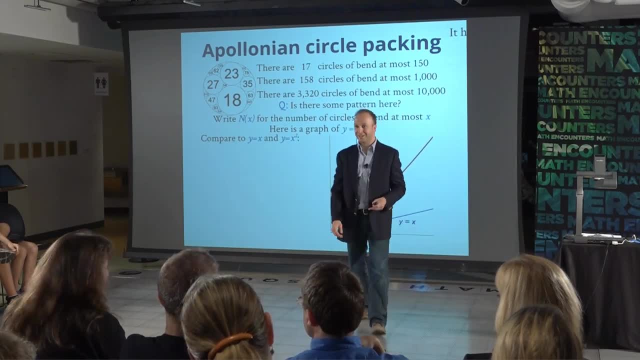 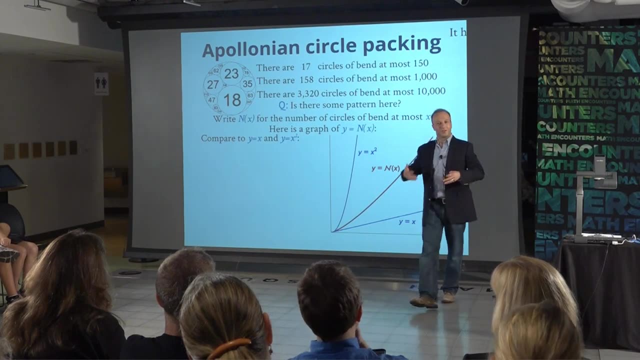 And y equals x, squared our parabola, our conic cross-section parabola, And you see the curve is going quite a bit faster than linear, quite a bit slower than quadratic. So what does it mean? How is it growing? 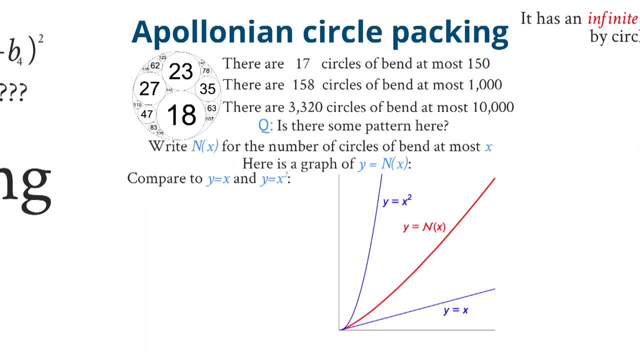 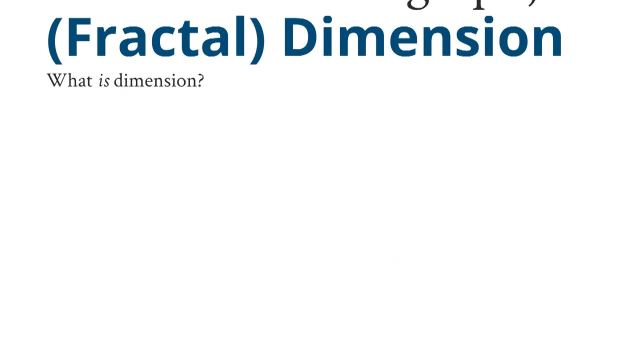 How is this function growing, Turns out. bless you that to understand this, we need a notion of fractal dimension. And before we have a notion of fractal dimension, we need a notion of dimension. So, what is dimension? Well, OK, what do we know? 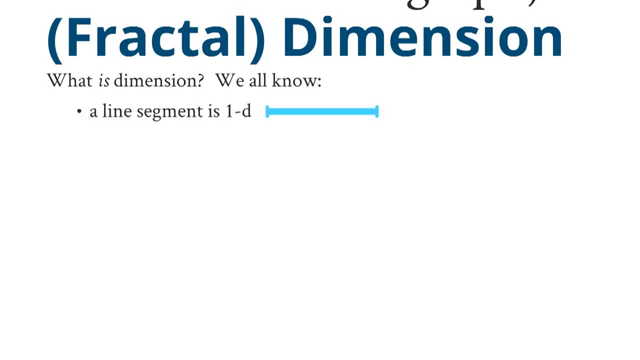 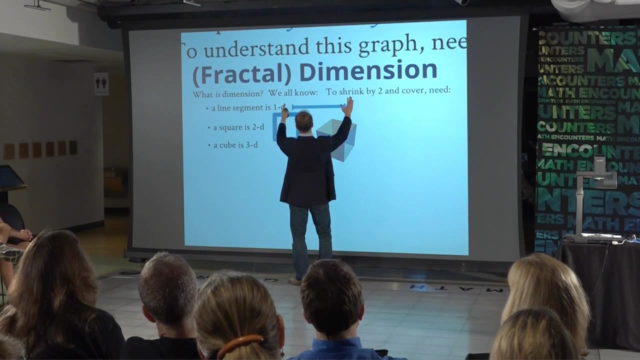 A line segment is one-dimensional, A square is two-dimensional And a cube is three-dimensional. How can we try to understand what dimension means just by studying these three objects? Well, what we can do is we can take this line segment and we can shrink it by a factor of 2,. 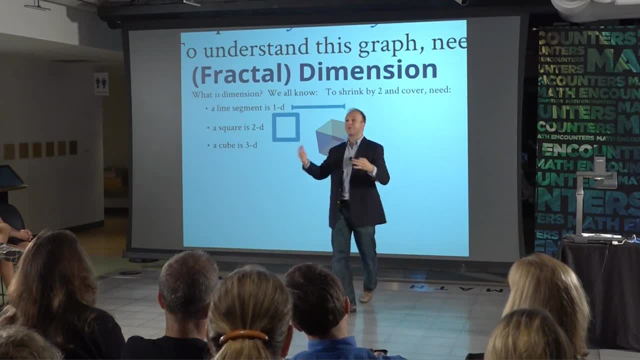 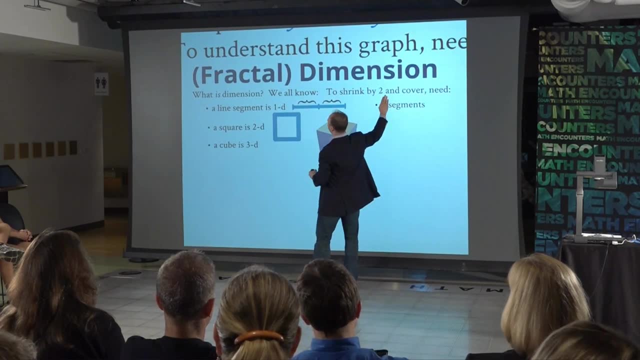 and then say how many copies of that shrink do we need to make up the original line segment? OK, So how many Half segments do we need to Don't look How many half segments do we need to make up the whole segment? 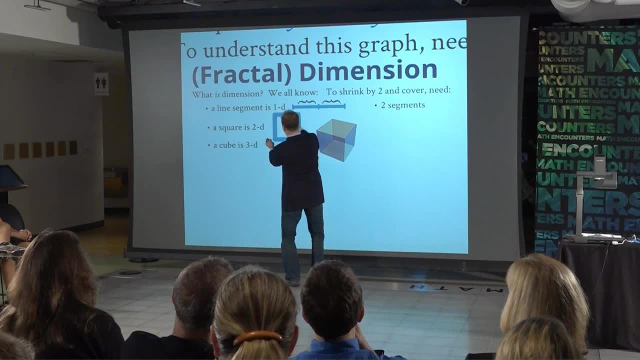 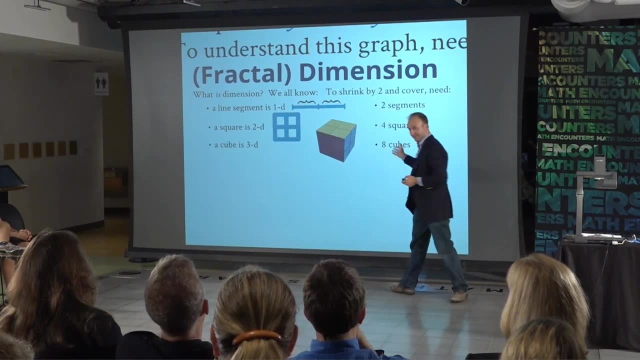 Two, OK, And if I take this square and I shrink it by a factor of 2,, how many will we need? Four, Four, right, We need four of these squares. And how many cubes? Eight, Eight, OK. 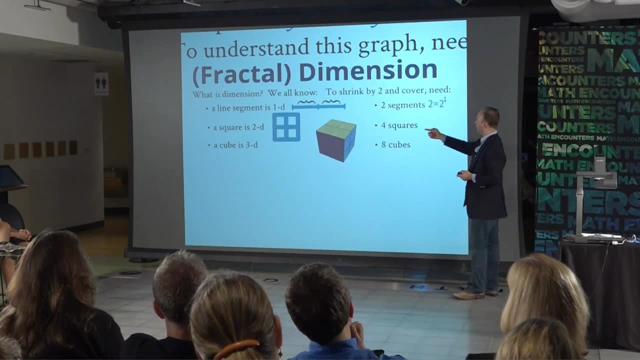 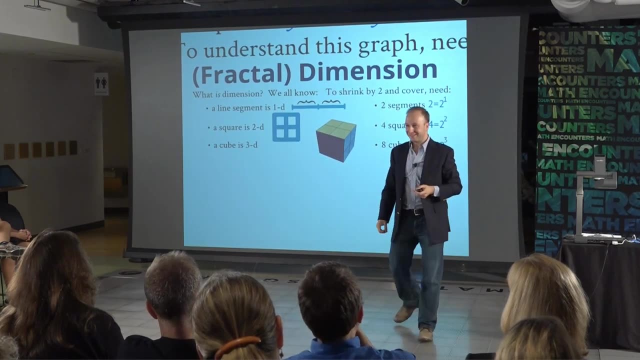 And then we notice that 2 is actually 2 to the first and 4 is 2 squared and 8 is 2.. That's why it's called squared and cubed right. It's exactly for that reason. Everybody see that. 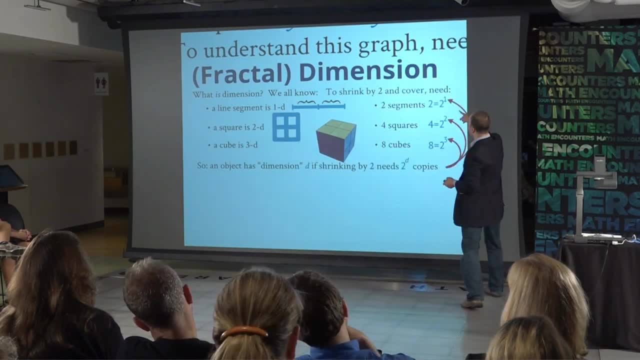 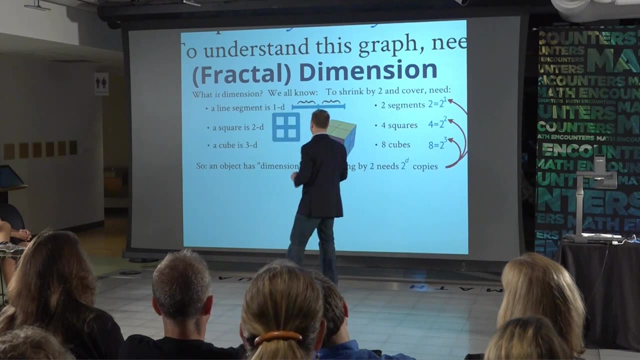 And so what's the dimension? The dimension is this number hidden in the exponent. So one very vague, very naive, and they're much more complicated notions of dimension. For us it suffices to just understand. some notion is: if we shrink our object by 2, then we 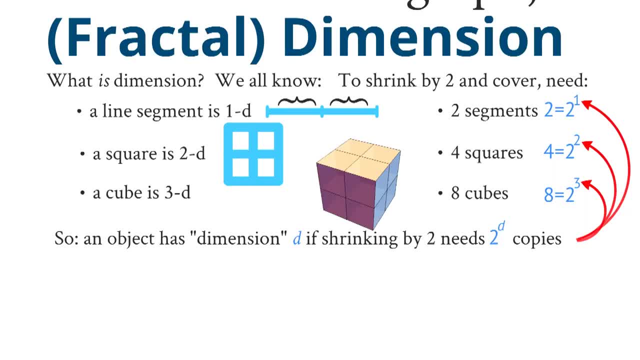 need 2 to the d copies of that same object to cover the original, And d is the dimension. So that's our understanding of dimension. OK, So let's test it out. What about our Sierpinski gasket? OK, so this is a picture where you take out. 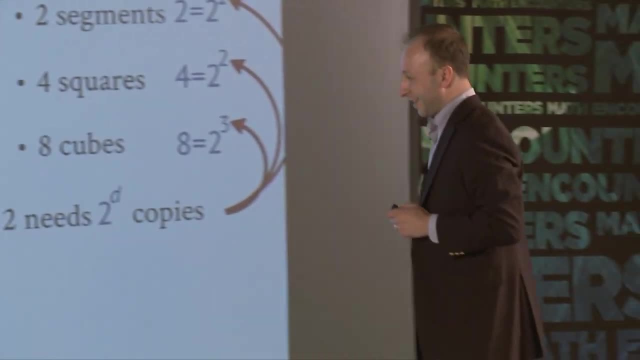 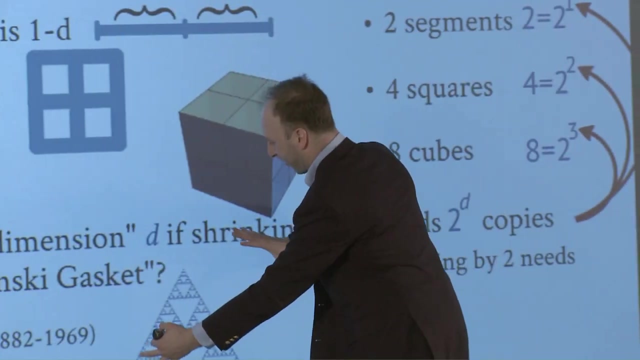 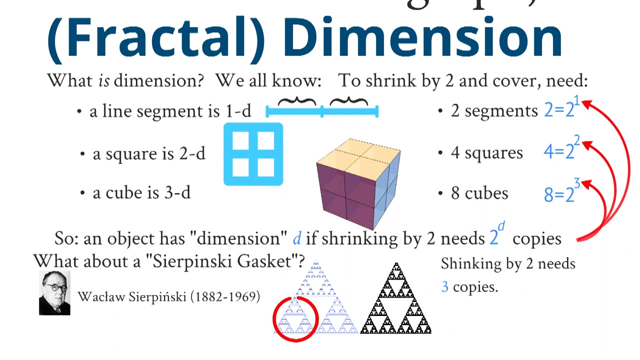 all the middles of all the triangles. So if you shrink it by 2, what do you get? If I shrink this by a factor of 2, I just get this little corner. This little corner is a factor of 2 smaller than the original thing. 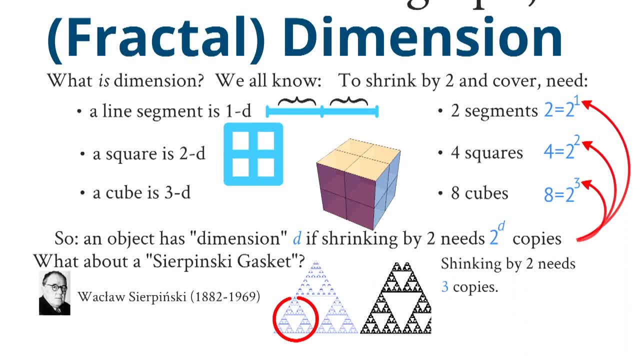 So how many copies of it do I need to make up the original 3.. Does everybody see that? So you need 3 copies. And here's the self-similarity of this fractal. As you zoom out, it's just the same thing over and over again. 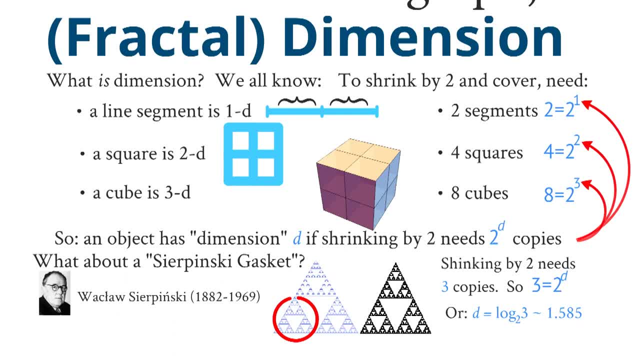 So 3 is supposed to be 2 to the number of copies is 2 to the dimension. That gives us an equation for d. So 3 is 2 to the d. Your mom will help you with logs, Don't worry about it. 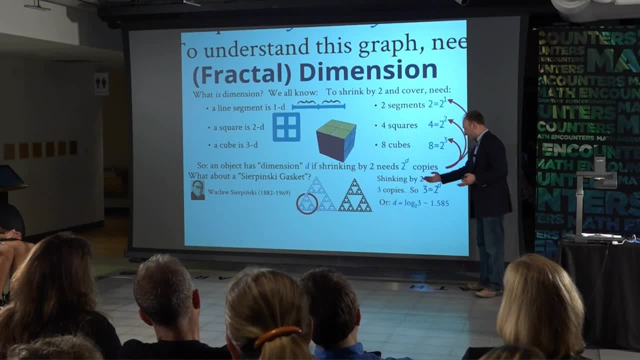 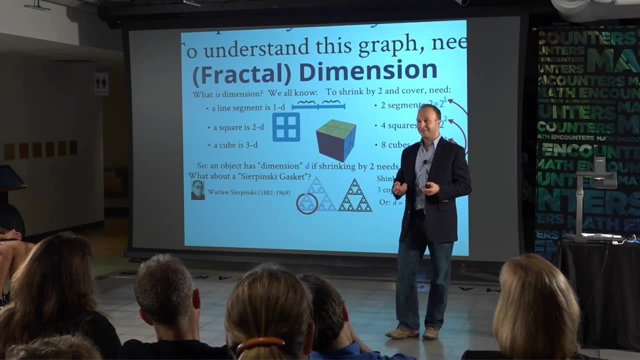 So you need to solve this equation. And the solution? well, it's log base 2 of 3.. It's just some number, 1.5, something. So that's the dimension. It's not one-dimensional, It's not two-dimensional. It's 1.58 dimensional. The Sierpinski fractal is 1.58 dimensional. It's not an integer dimension. That's what we mean by something that's not an integer dimension, And so that's called fractional dimension or a fractal. 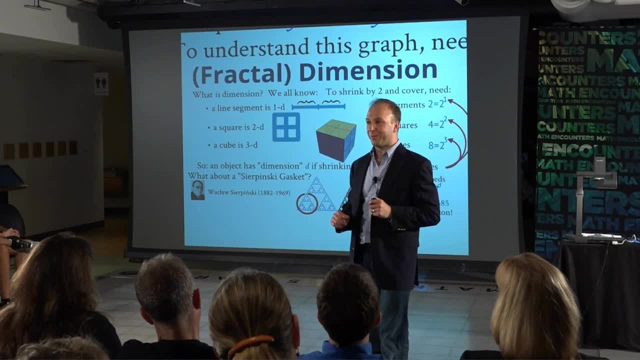 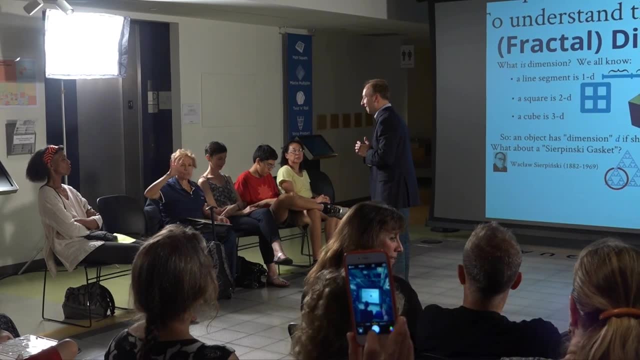 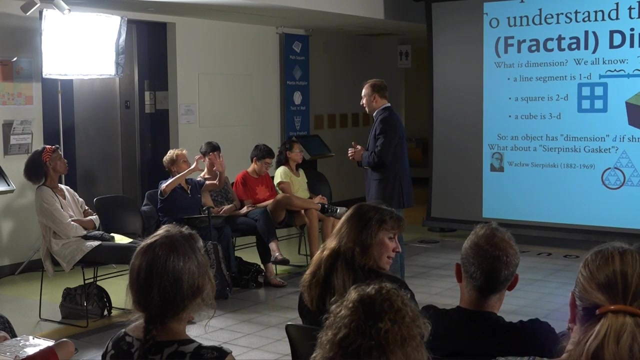 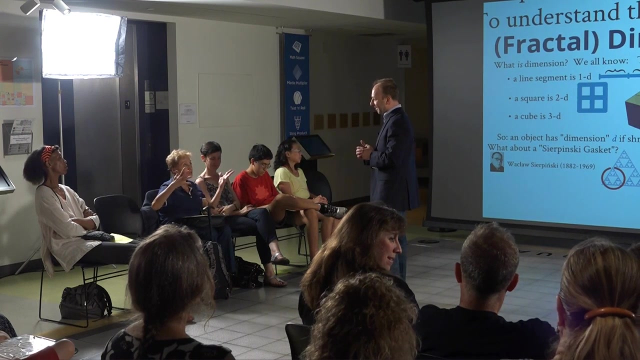 OK, Does everyone understand what I mean by dimension? I wasn't there, But yeah, Do you remember how to do the designs of the wall when they do the scores to design the floor and everything? Uh-huh, It's more or less similar. 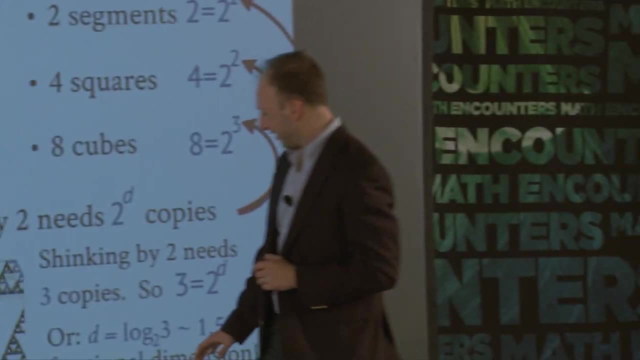 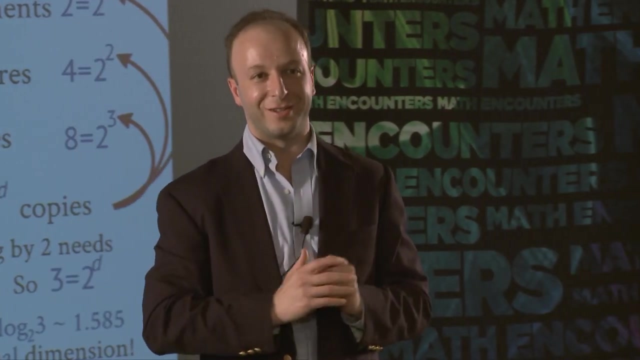 Yeah, yeah, self-similarity and structure: Yeah, exactly. So this is just some notion of dimension for us. OK, There are lots of others and there are lots of other examples. OK, so that's fractal dimension. 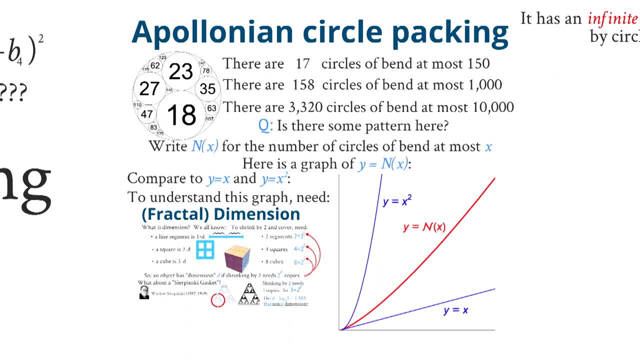 Now, when we go to our circle packing and we go to this infinite object- not our finite object- it has some dimension And that dimension can be computed and it's something like 1.3, something OK. So now you're going to learn your first- maybe not your first. 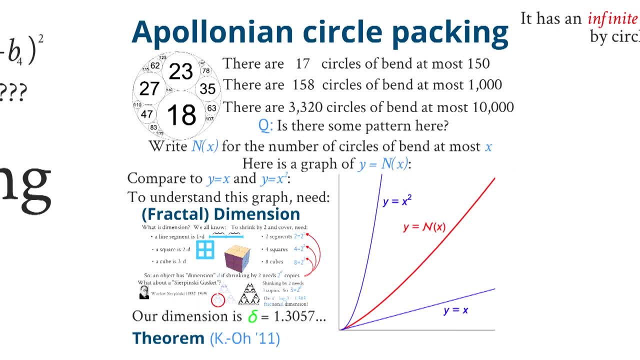 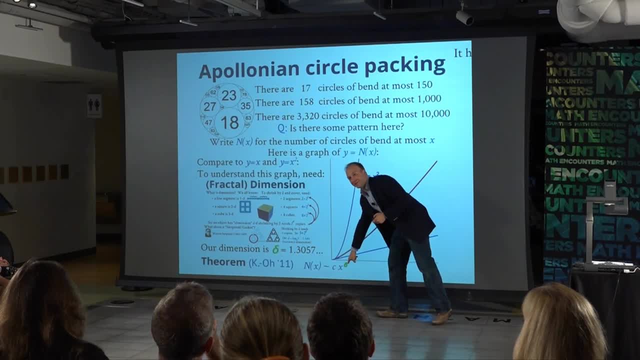 of the night- 21st century's theorems. This is joint work with from a few years ago. We show that this curve is asymptotic to some constant, sometimes x to that dimension, And that dimension is between 1 and 2,. 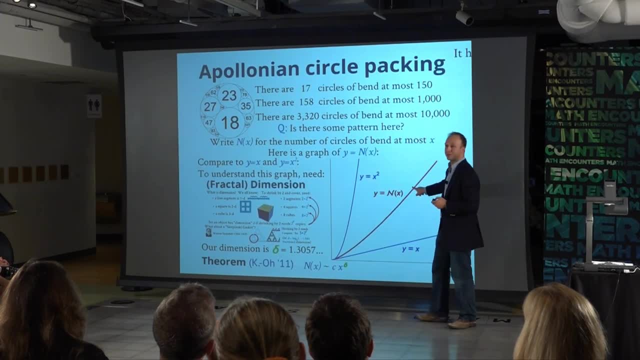 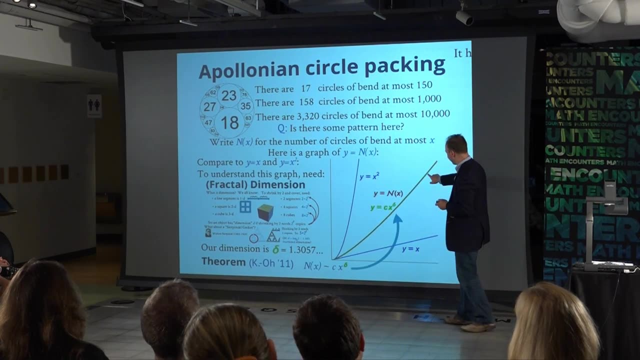 so the curve grows faster than x, but slower than x squared. So that explains this curve. I'm going to graph the curve. Ready Watch it. Did you see it? It's in green as opposed to the original curve is in red. 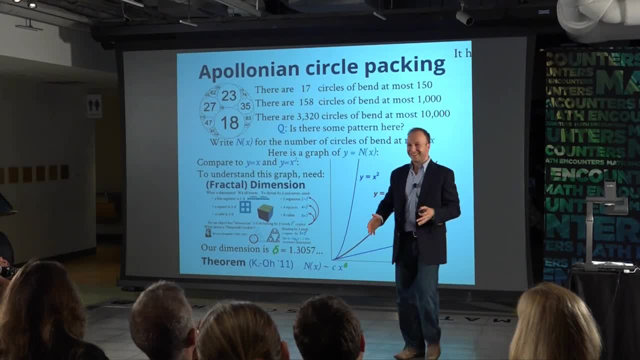 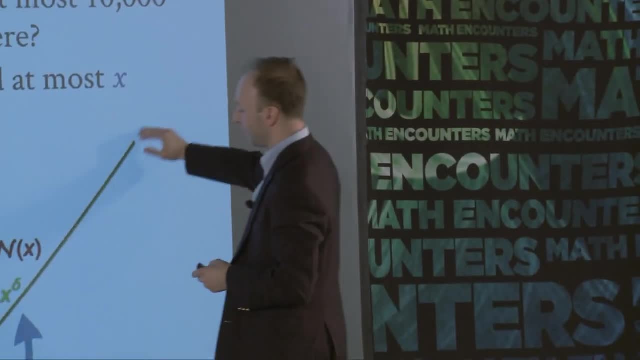 Now I could have just drawn the same curve twice. You have to believe me that I'm not cheating you. I really did compute n of x and drew that curve, And the theorem says that these two are very close. OK, So asymptotically you can't tell the difference. 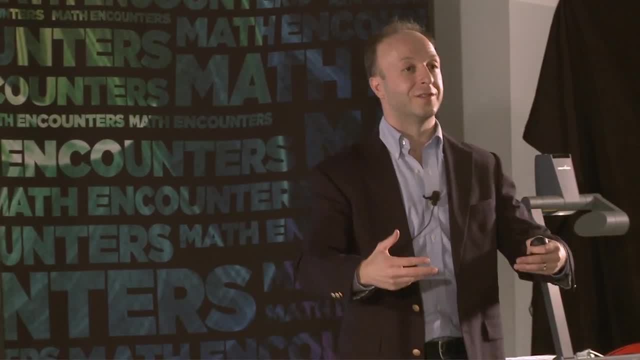 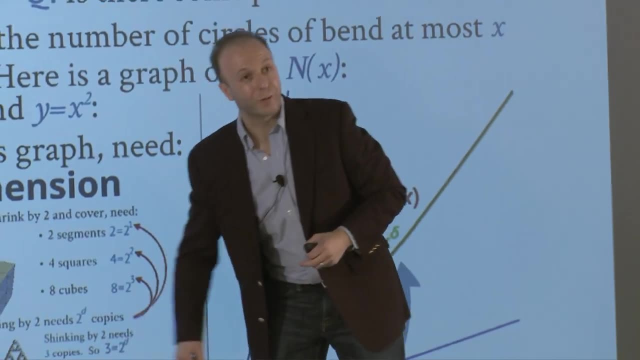 between one and the other. So that's the growth rate. So if you want to know how many curvatures there'll be with bend, at most a million- you take a million and you raise it to the 1.3, and that'll. 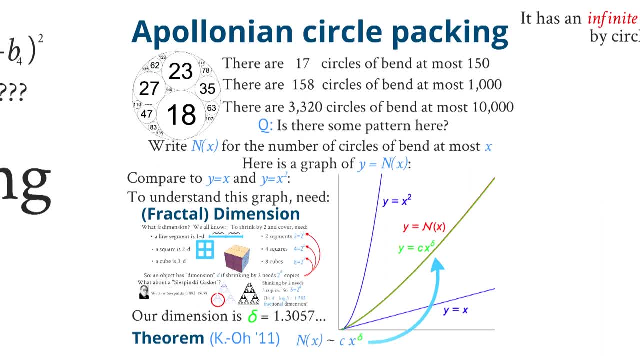 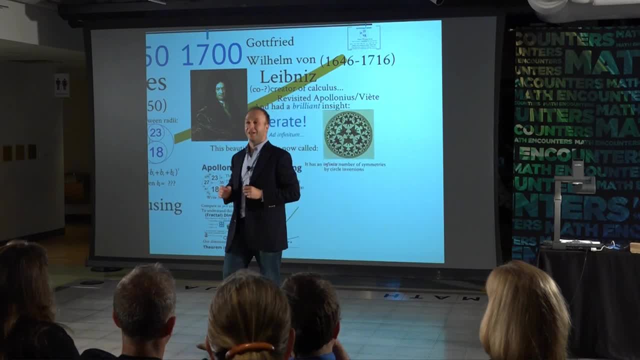 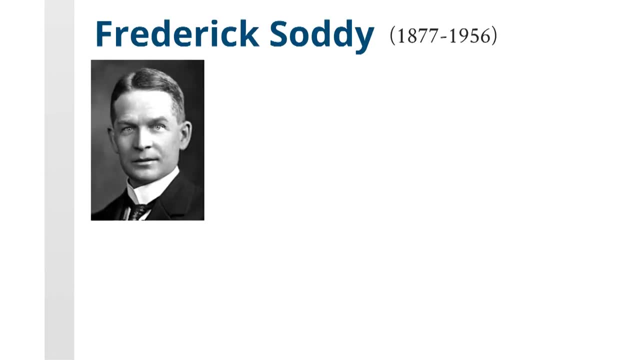 approximate how to extrapolate that curve. OK, So that's the fractal, the infinite fractal that you get from iterating this process infinitely. There's one more person we have to meet, And that is Frederick Soddy. So Soddy is not a mathematician. 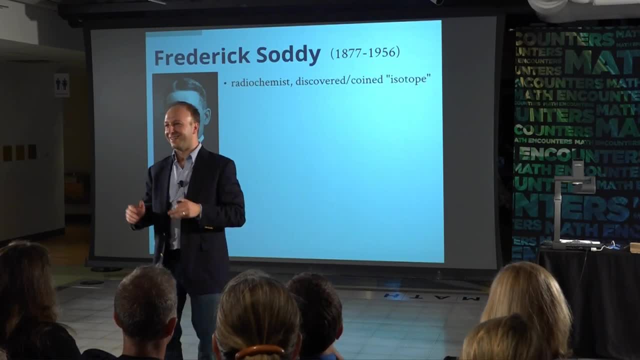 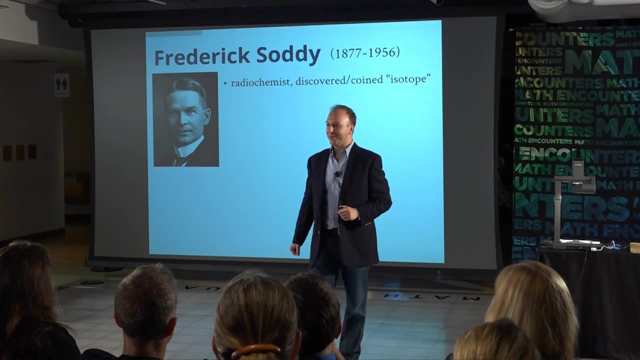 He's the only person. Well, Descartes is a philosopher, Anyway, he's a radiochemist. He's really not a mathematician. I mean, he is a mathematician Professionally. he's a radiochemist. His most famous thing is discovering isotopes. 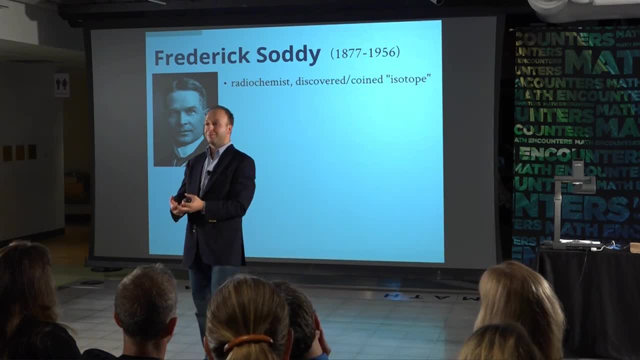 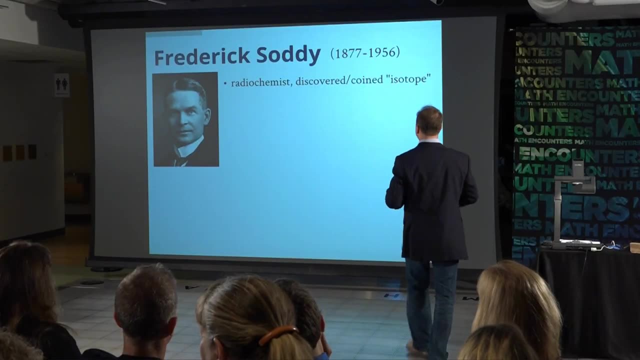 that you can have the same different atomic weight while having the same. What grade do you get to chemistry? Not yet right, OK, Don't worry. So isotopes is something. He discovers, these things called isotopes, And for that he's rewarded with a Nobel Prize. 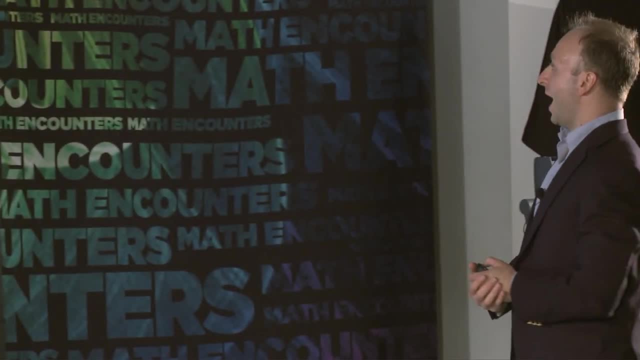 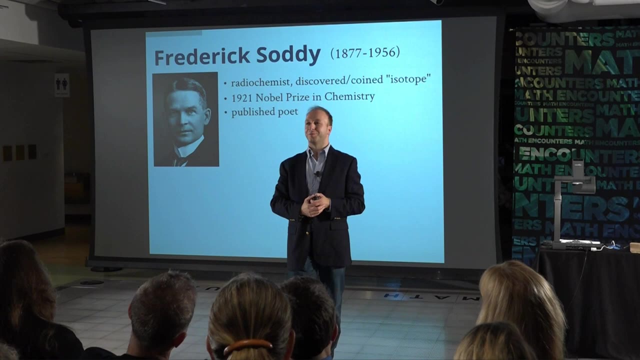 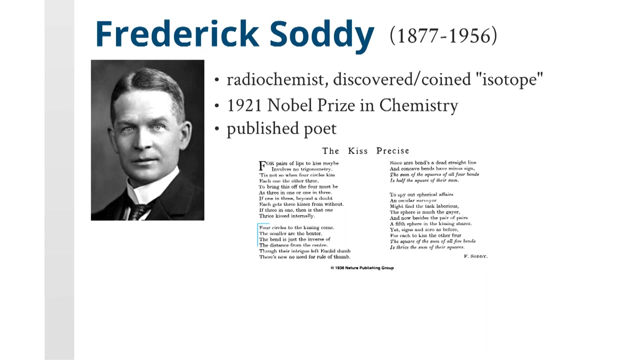 in chemistry in 1921. And he's also accomplished in many areas, including poetry. He publishes his poems in unusual places for poets. He publishes them in the journal Nature. I guess if you're a Nobel laureate you can put your papers in Nature. 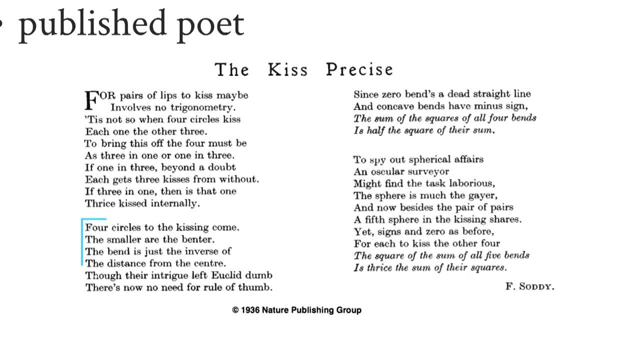 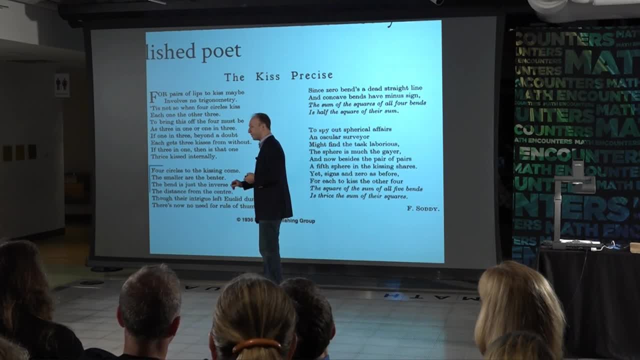 So let me just read you a piece of this poem. Four circles to the kissing come. The smaller are the benter. The bend is just the inverse of the distance from the center. The bend is 1 over the radius, Though their intrigue left Euclid dumb. 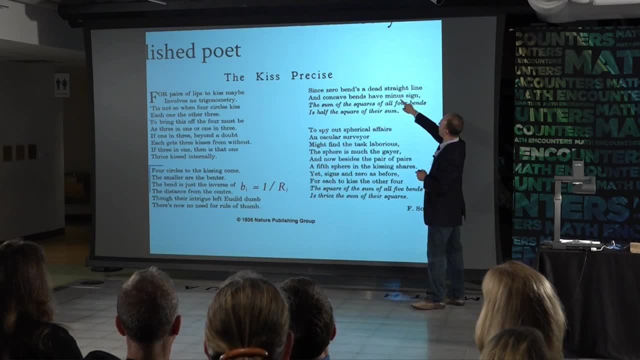 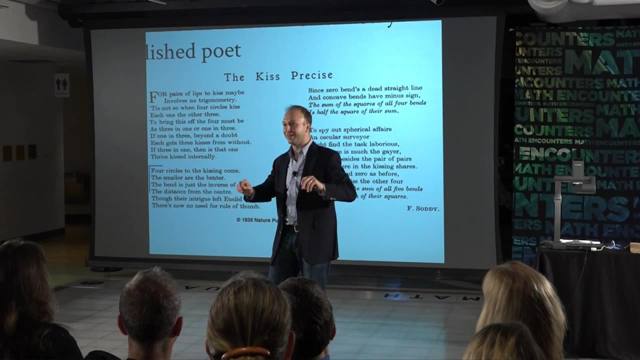 there's now no need for rule of thumb, just poetry, Since 0 bends a dead straight line. so what if the bend is 0? That means the radius is 1 over 0, which is infinity sort of. So what's a circle of infinite radius? 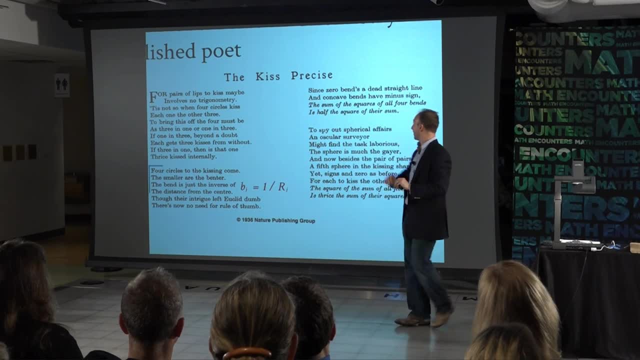 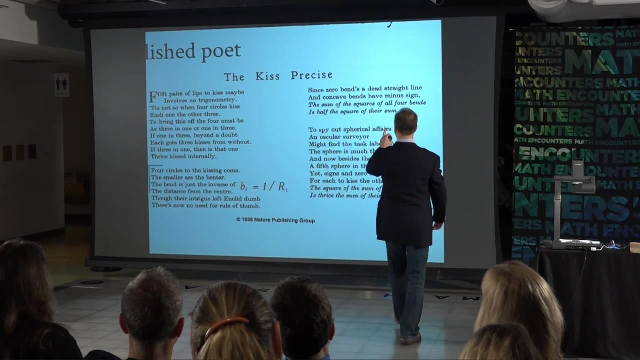 A straight line. OK, So curvature 0, bend 0 is a dead straight line And concave bends have minus sign, just like we know about orientation. The sum of the squares of all four bends is half the square of their sum. 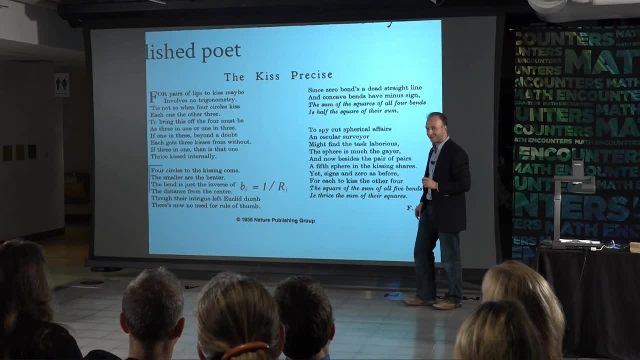 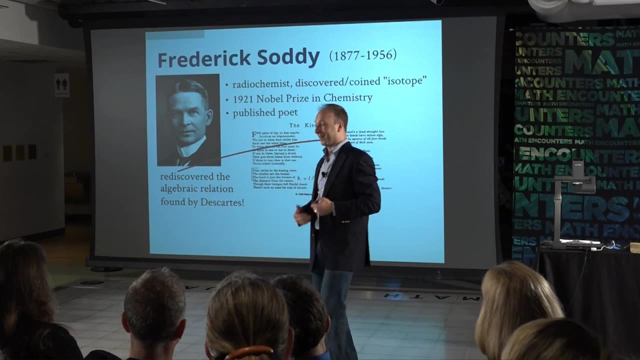 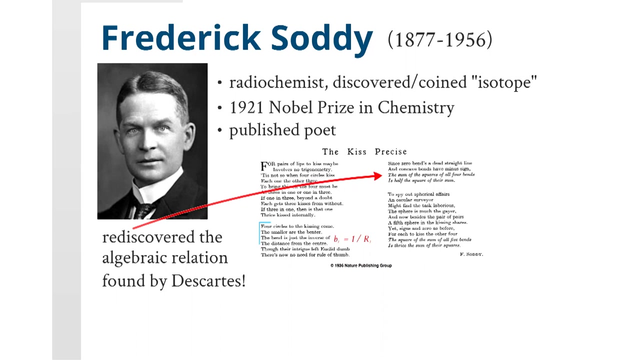 That's familiar. That's the formula Descartes had discovered 300 years before. He didn't know about Descartes' work. so he rediscovers this amazing formula, And then he observes something That Apollonius missed. 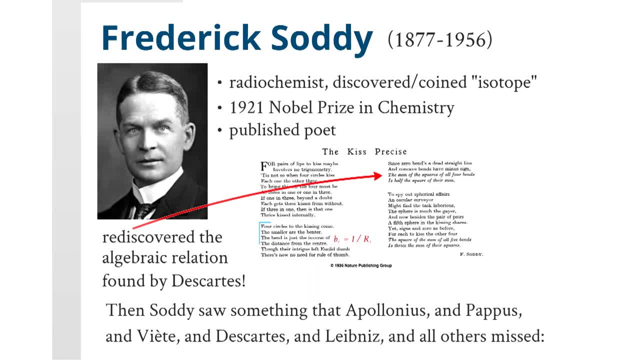 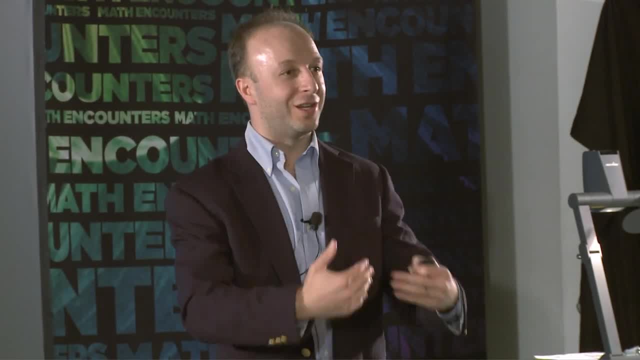 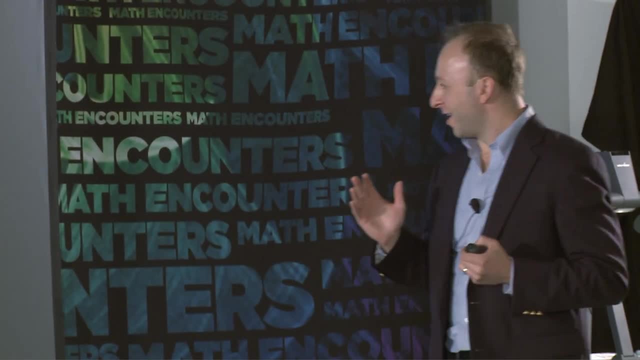 That Pappus missed, That Viet Descartes, Leibniz, Newton, every single mathematician that came before him studied these beautiful pictures, studied these properties, and they all missed it. What is it? The integrality of these circle packings. 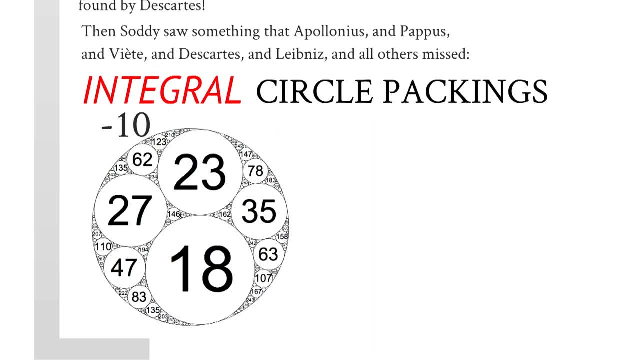 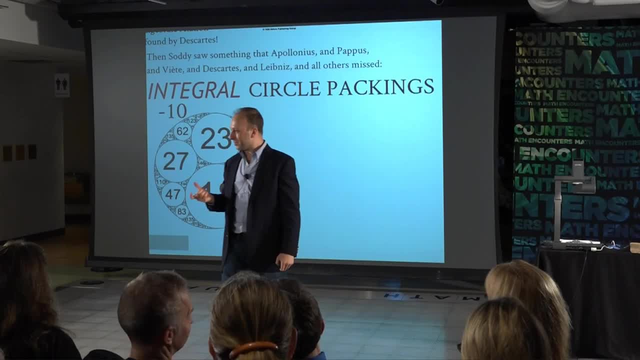 Let's go back to our picture. So here's the picture with more. Here's your exact thing, except now I've put in 100.. 100 more circles, The curvatures, the bends. this is a circle of radius 1 over 18.. 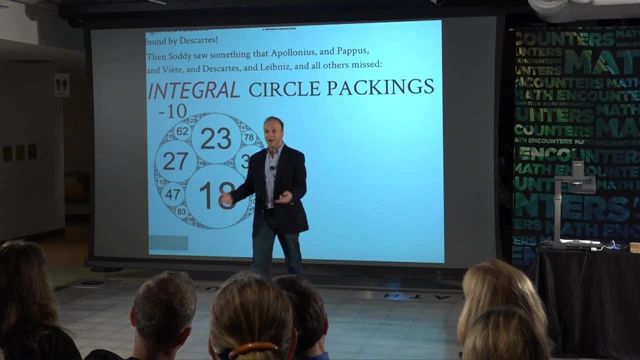 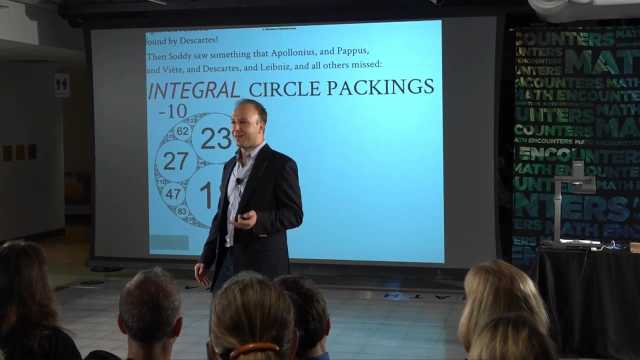 This is a circle of radius 1 over 242, 1 over 282.. Why are these integers? Where is the square root of 2?? Where is the e or the pi, Something? Why are these numbers all integers? It's very bizarre, right. 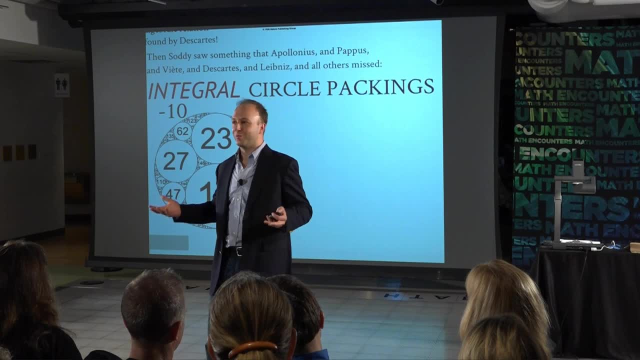 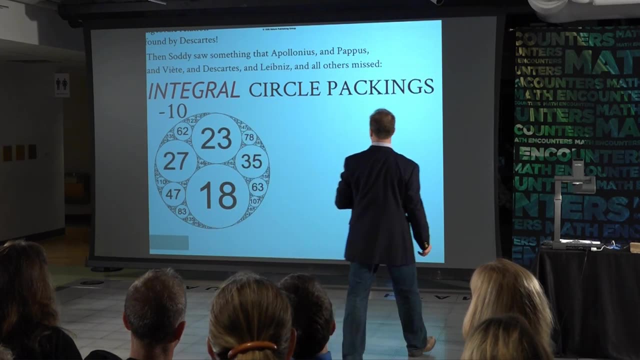 You're doing some very geometric, straight-edge and compass construction to get more and more circles. Something must be driving this integration. Why are these bends all integers? And he figures out what it is. He first of all observes this integrality for the first time. 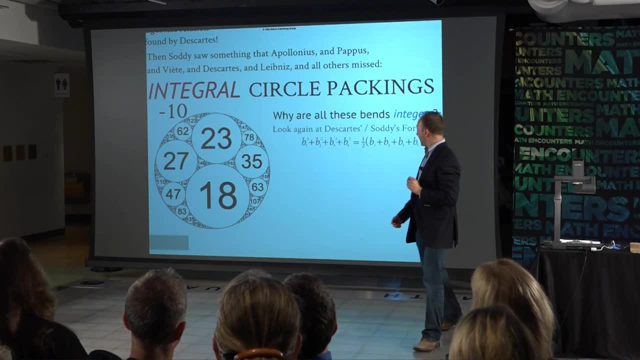 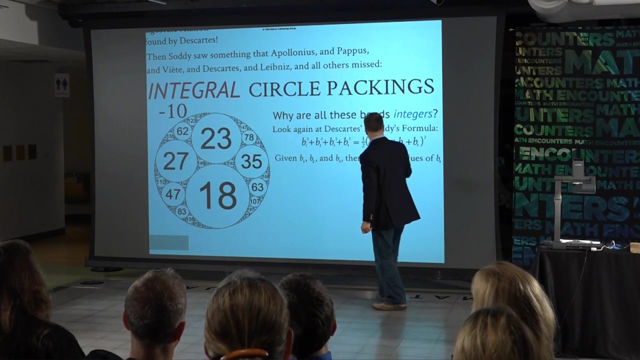 And he answers the question: why are these bends all integers? And it goes back to again the Descartes formula, which Saudi independently discovers: The sum of the square of all four bends is half the square of their sum. So again, if you give me b1,, b2, and b3,, 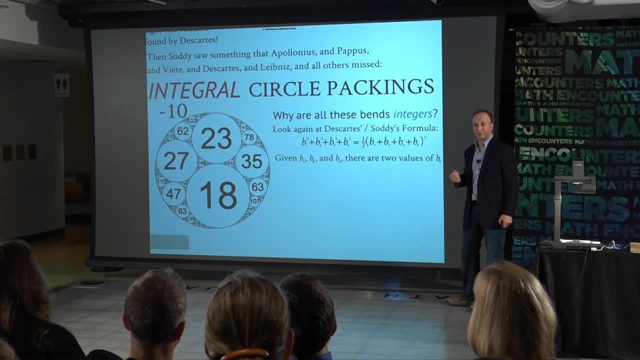 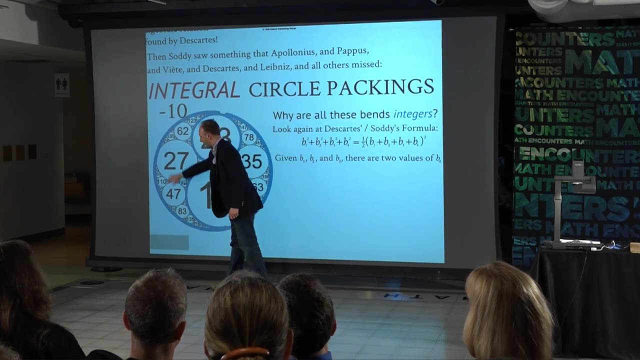 then there's a quadratic equation for b4, which we solve, and we find two solutions. What does that mean? So let's pick the 18,, the 23, and the negative 10 as our b's. So those are three circles. 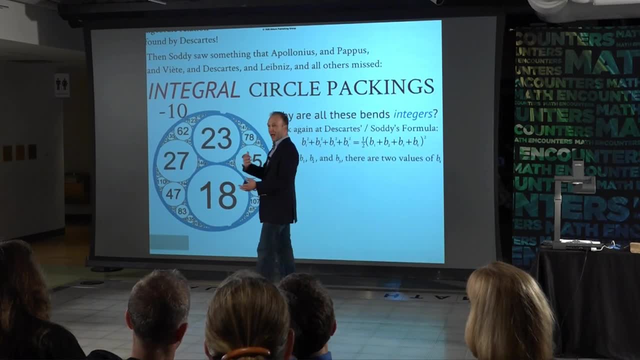 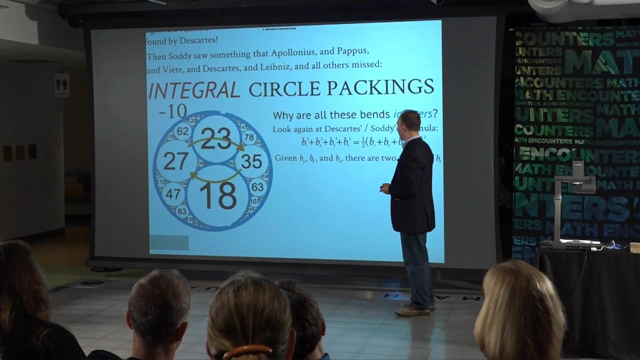 And there are two values of b4, which means there are two solutions to the Apollonian problem. So what are the two circles that are exactly tangent to just those three, The 27 and the 35.. So it's a simple exercise from this formula that how do you get from one to the other? 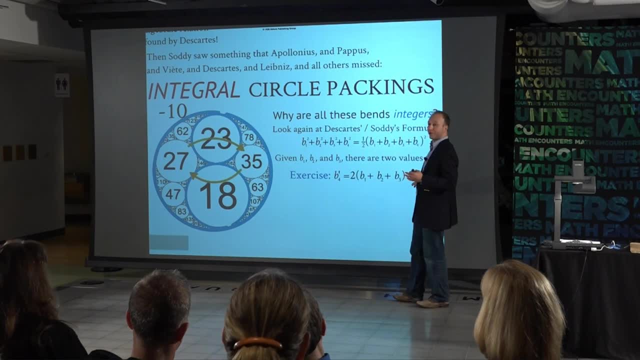 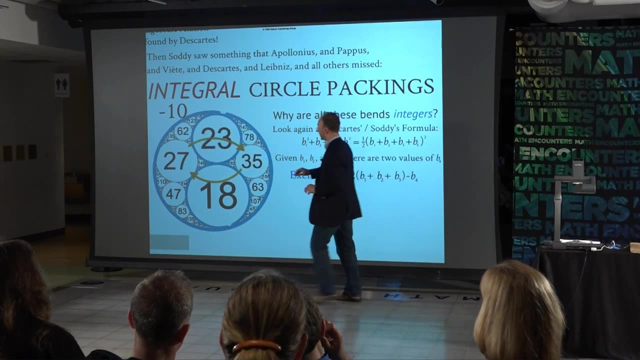 Well, you get from b4 and b4 prime are the two solutions you get from one to the other by adding the three b's, multiplying by two and subtracting. So let's do our example. So if our three b's are negative, 10,, 18, and 23,- so what's their sum? 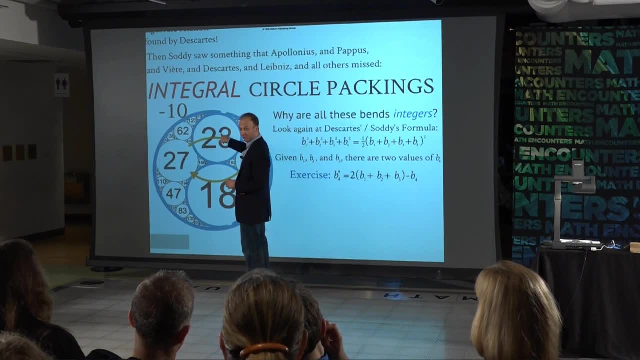 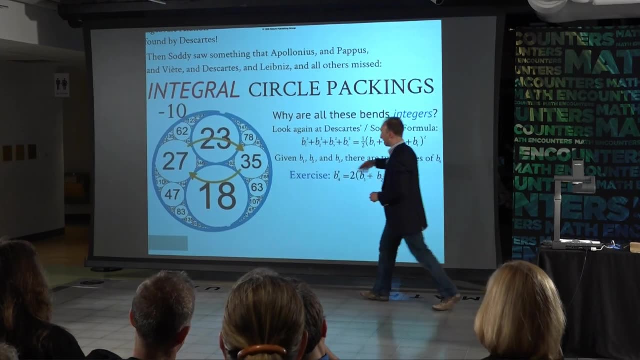 So negative 10 and 18 is 8, 8 and 23, 31. So that's 31.. If I double 31, I get a 62. And if I let's say b4 is 27.. 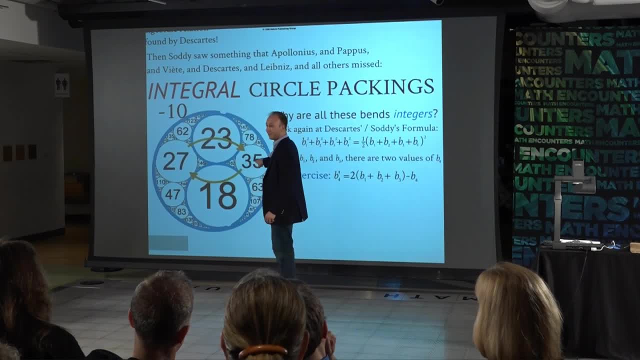 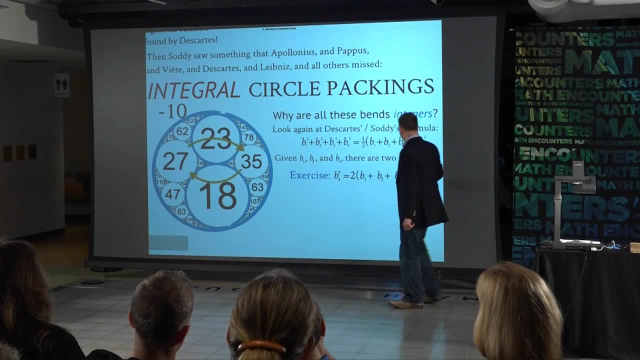 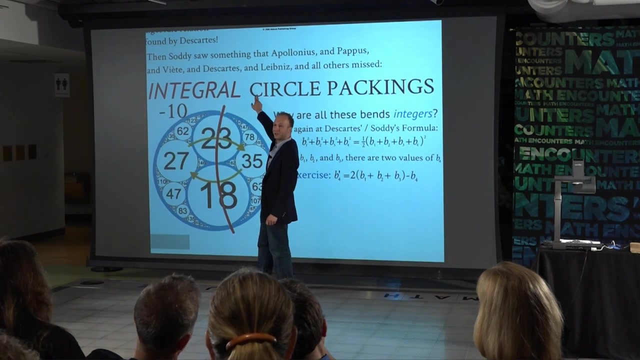 So what's 62 minus 27? 35.. And what's 62 minus 35? 27.. OK, So this simple algebraic relation is what you get when you apply the inversion, this symmetry- Remember there are infinitely many symmetries- through circle reflections. 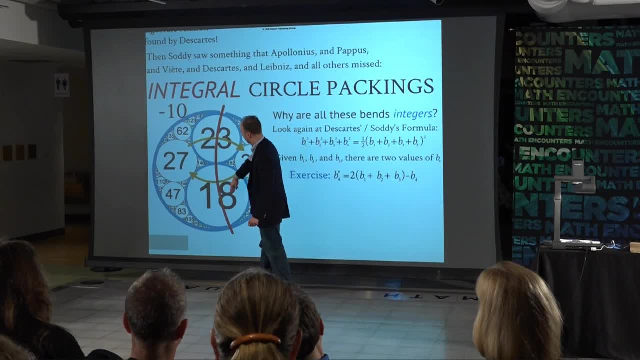 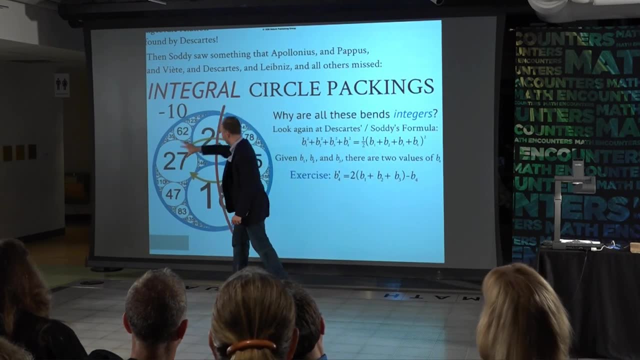 When you do a circle reflection, through exactly this circle, this reflection, this inversion which fixes the negative 10, the 18 and the 23 circles, the 27 circle is sent to 35, and 35 is sent to 27.. 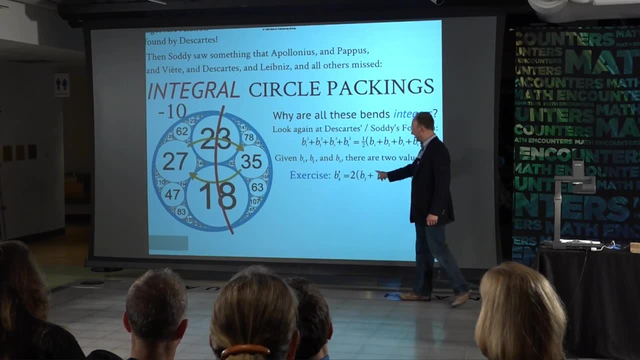 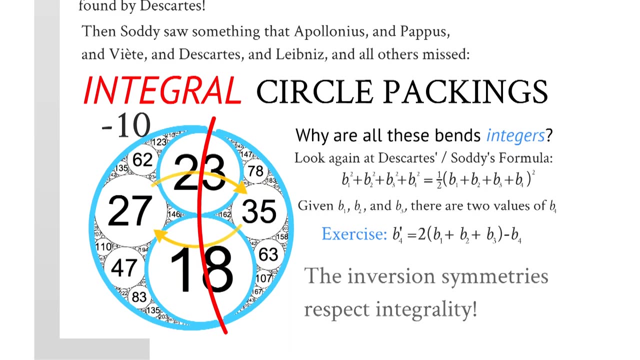 And look at what operation we did on the bends: We added, we multiplied and we subtracted. When you add integers and multiply integers and subtract integers, but not divide, no square roots, no raise to the 1.3 or anything. 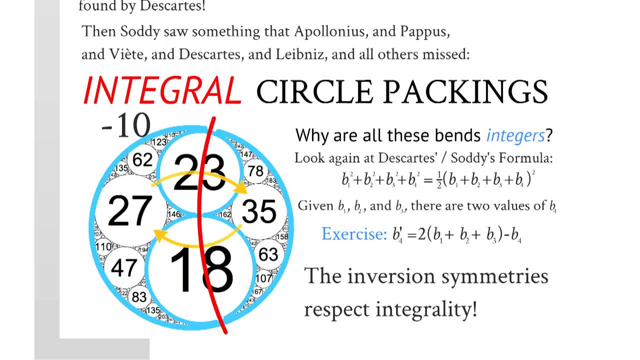 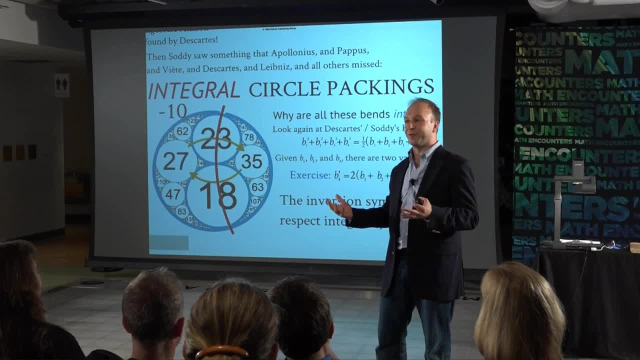 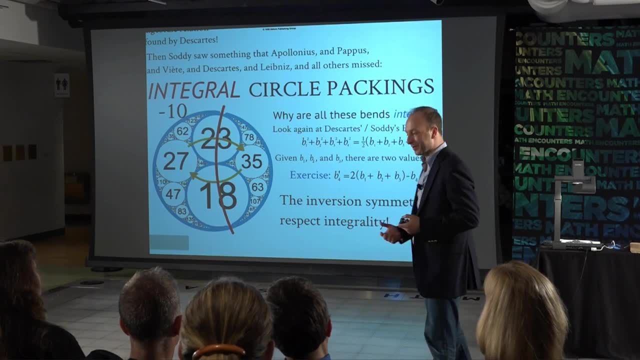 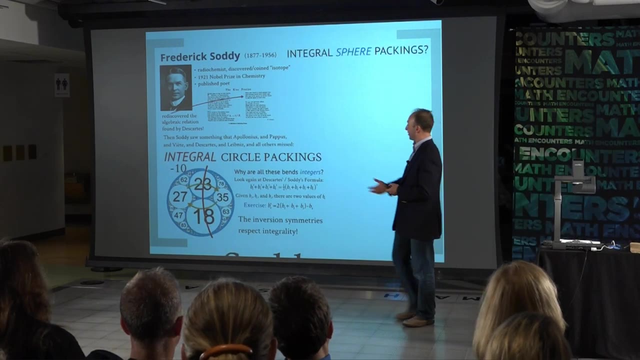 It's just addition, multiplication, subtraction. Those symmetries, as acting on the bends themselves, preserve integrality. That's why there exist configurations with integer bends. He saw it, Everybody else missed it. Very bizarre. All right, Let's finish with some sphere packings, because why only circles, right? 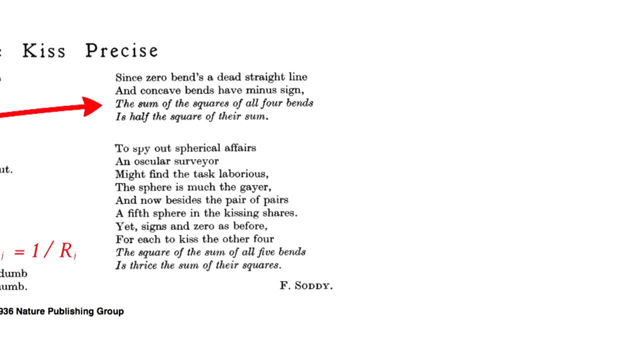 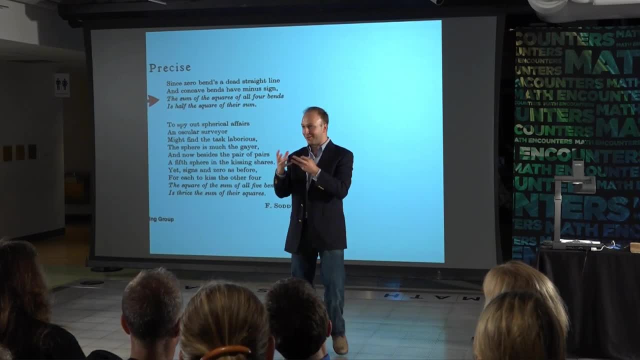 Let's see what happens in higher dimensions. What do we know about sphere packings? Well, actually, he continues his poem To spy out spherical, Spherical affairs. An oscular surveyor, Oscular, the mouth Kissing. 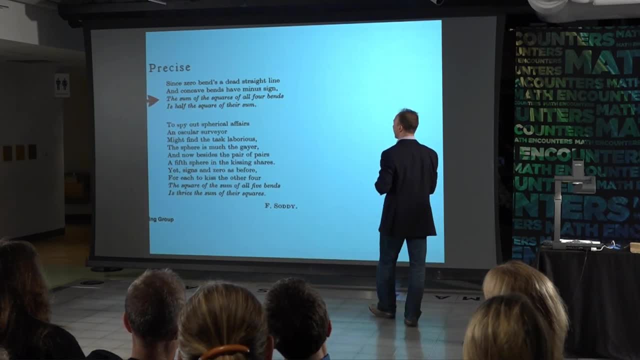 You want to know about kissing spheres Might find the task laborious. the sphere is much the gayer And now, besides the pair of pairs, instead of four circles, a fifth sphere in the kissing shares. So you need five spheres that are all tangent to each other. 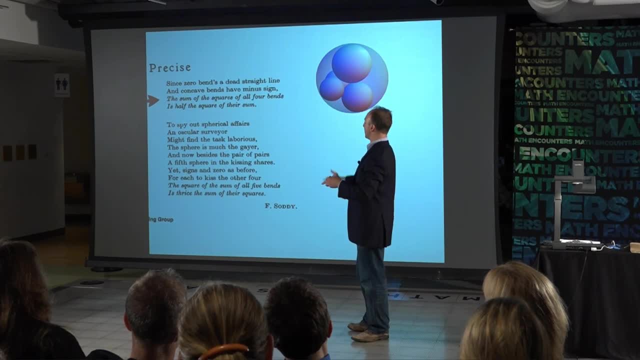 And yet, sines and zero, as before, for each to kiss the other four, the square of the sum of all five bends is thrice the sum of their squares. So that's some other algebraic relation on the bends of five mutually tangent. 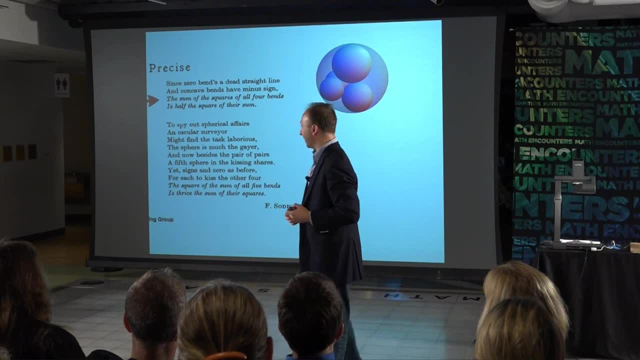 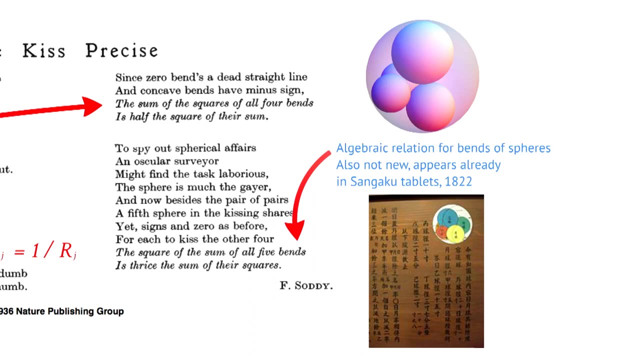 All right, Thank you. So that's the algebraic relation on the bends of five mutually tangent spheres. This time he's only a hundred years too late. That algebraic relation was discovered by the Japanese, And these appear in Sengaku tablets early 1800s. 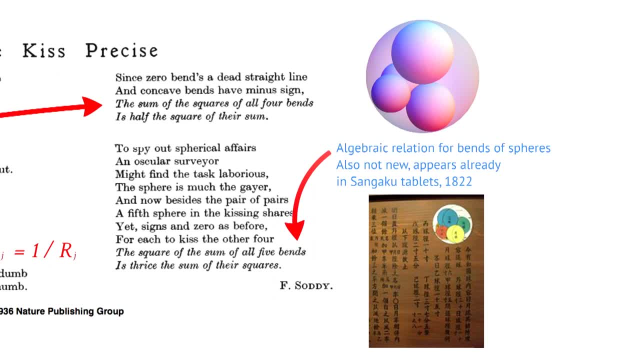 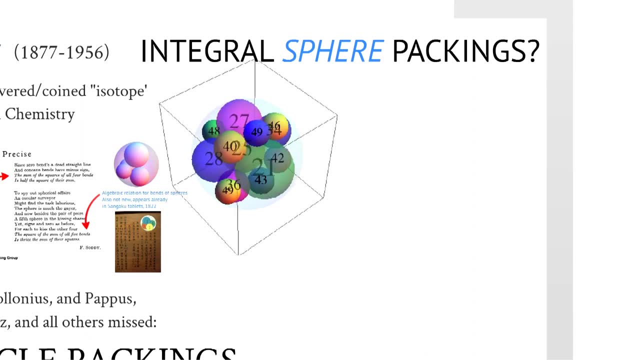 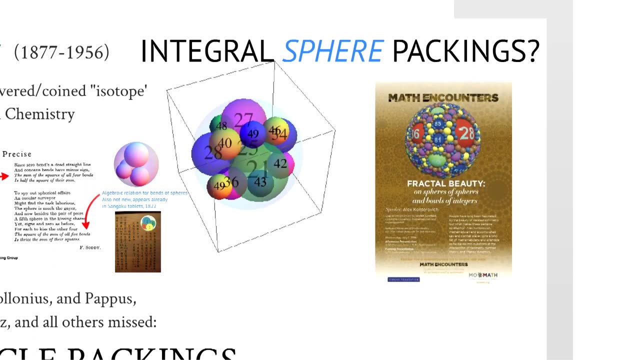 But nevertheless, he's again the first to realize the integrality properties that arise as a result of this algebraic relation. So here is an integral sphere packing, And in fact that's what's on this poster. Okay, sphere packing, which has so 28, is a sphere of radius 1. 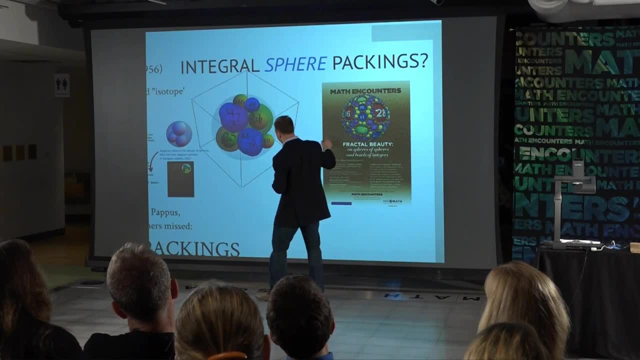 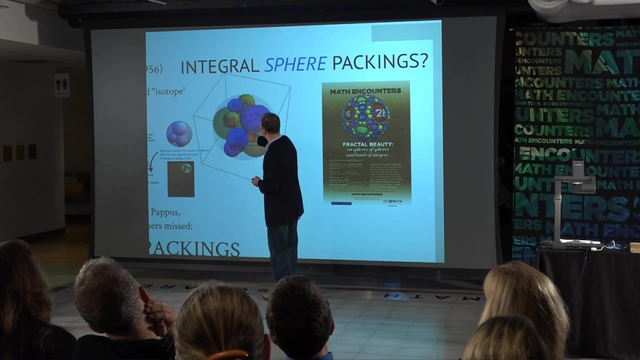 over 28.. That's spinning around here. There's a 49 here, There it is going around, And a 36, wherever it is. Anybody see it? There it is. There's the 36 sphere going around. 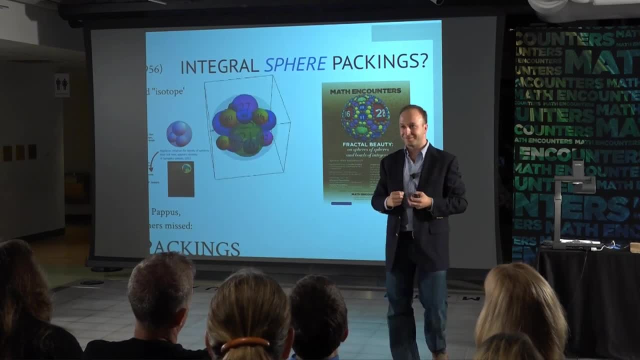 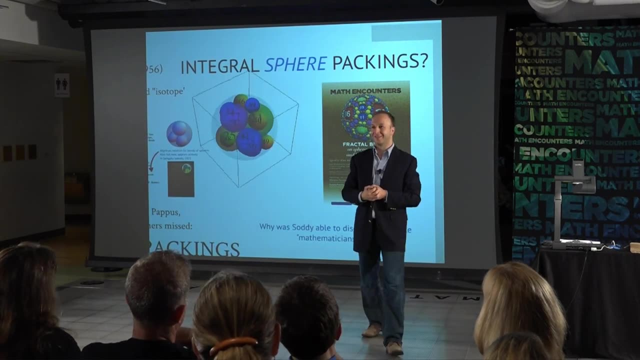 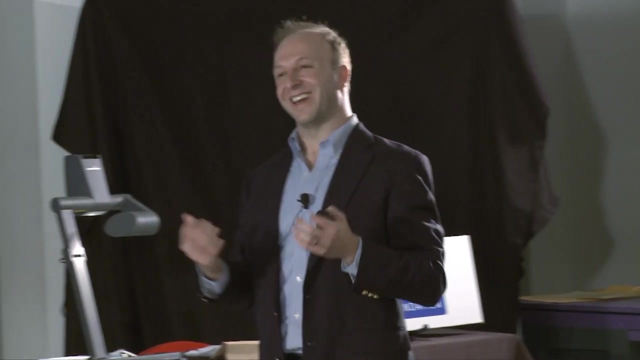 So this is a sphere packing with all integer bends. Why did Soddy see this when no mathematician saw it? How come he got it? He's a chemist. OK, I don't know what about being a chemist makes you. 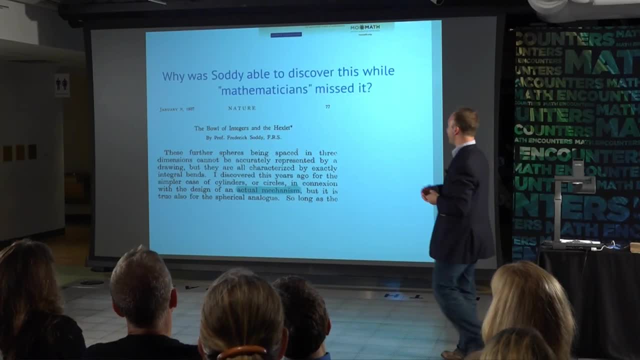 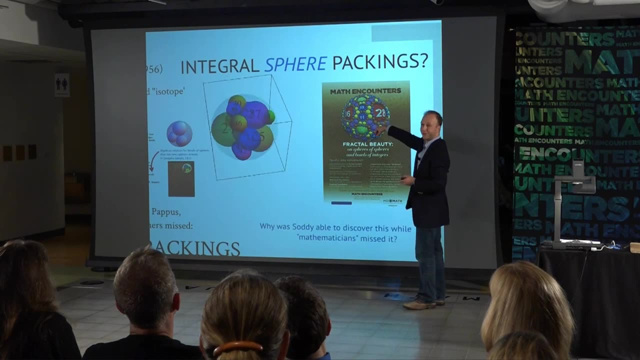 Let's see. Let's see what he himself writes about this. So a year later, he publishes another article in Nature. Now it's called The Bowl of Integers, which, by the way, that's what this sphere of spheres and bowl of integers. 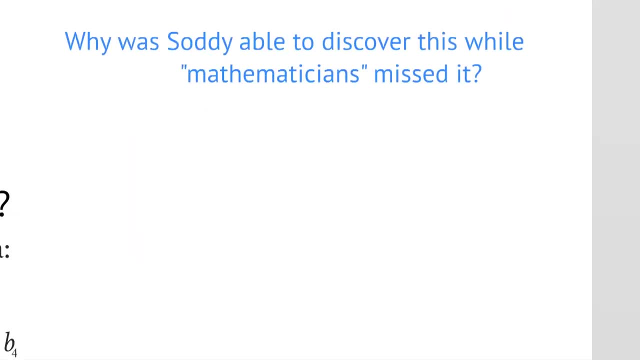 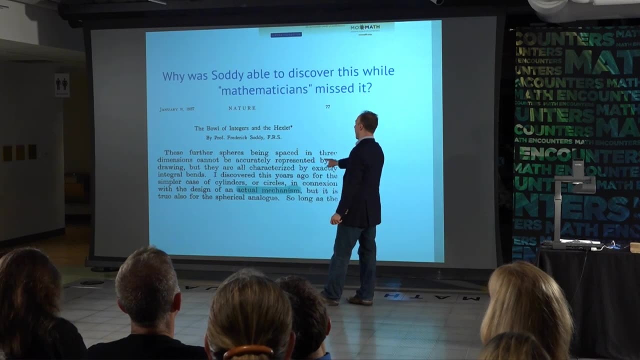 Now you see what that's referring to. So he writes an article called The Bowl of Integers, The Bowl of Integers and the Hexlet. These further spheres being spaced in three dimensions cannot be accurately represented by a drawing. That's why I had to spin the spheres so you could see where. 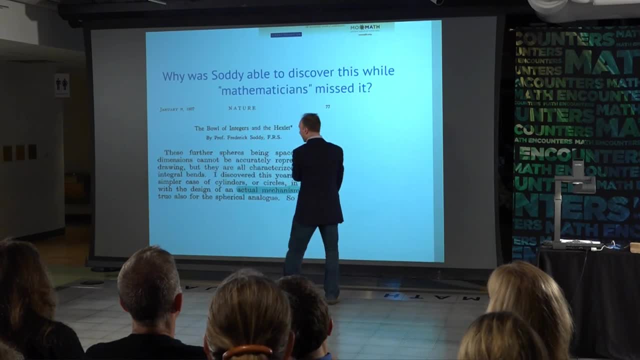 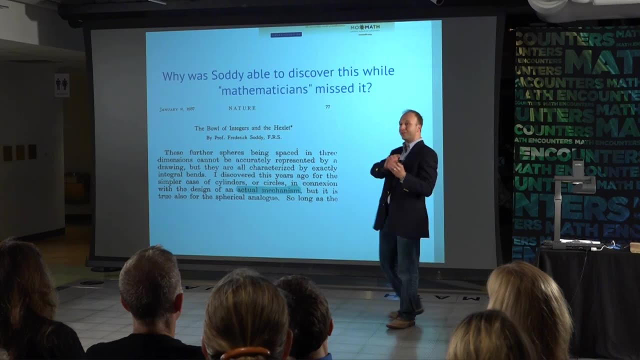 they all are, But they are all characterized by exactly integral bends. This he saw, that nobody else saw. I discovered this years ago for the simpler case of cylinders. So if you have a bunch of cylinders that you're running and you want them to be tightly packed around each other, 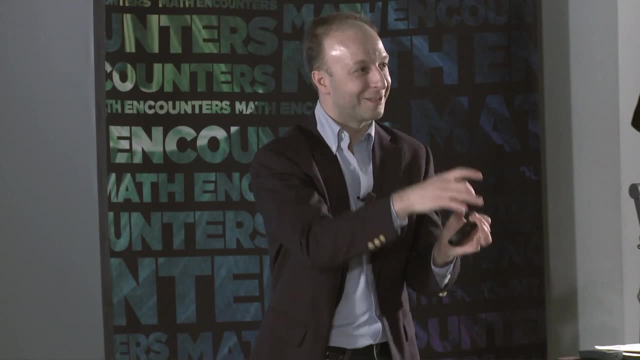 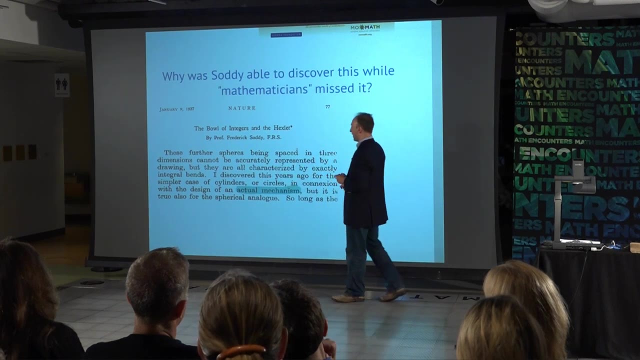 well, what's the cross section of a bunch of cylinders, Cylinders, Cylinders? It's a bunch of tangent circles, a bunch of kissing circles. I discovered this years ago, for the simpler case of cylinders or circles, in connection with the design. 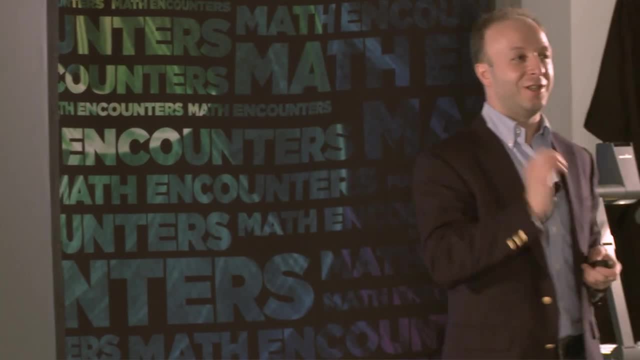 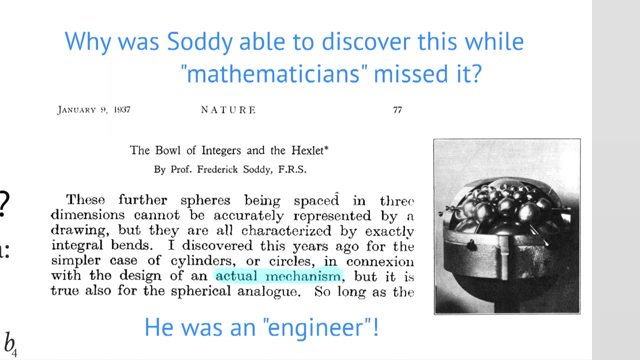 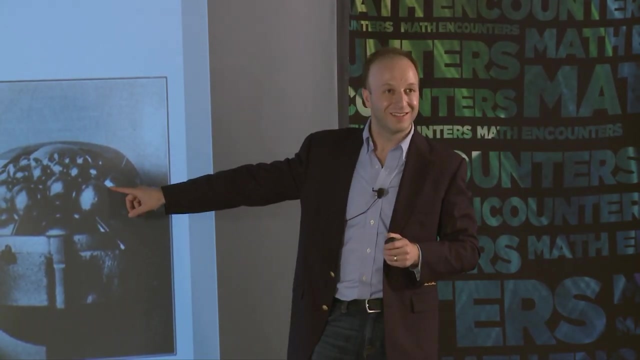 of an actual mechanism. That's the difference between Soddy and mathematicians. He was an engineer. This was not a Photoshopped image. in 1937 Nature. This is the picture of something that he actually built to get the sphere packing- exactly right. 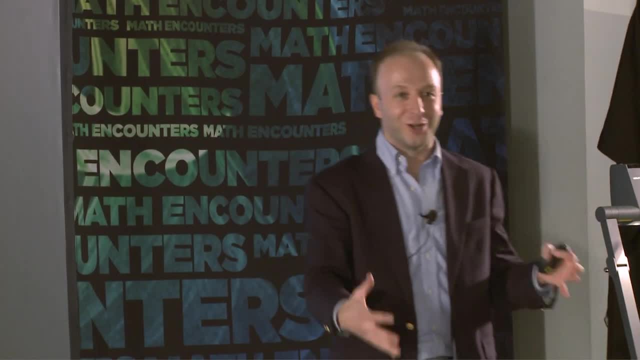 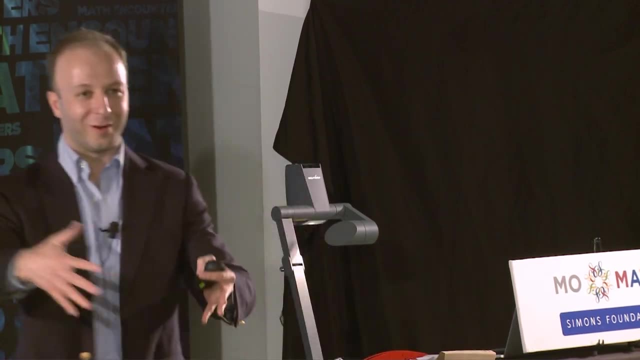 And if you actually build it, you need to know what curvature, what the radius is. And when he built this thing he said: wait a second. I took a sphere of radius 1 half and another sphere of radius 1 half and put it inside a sphere of radius 1.. 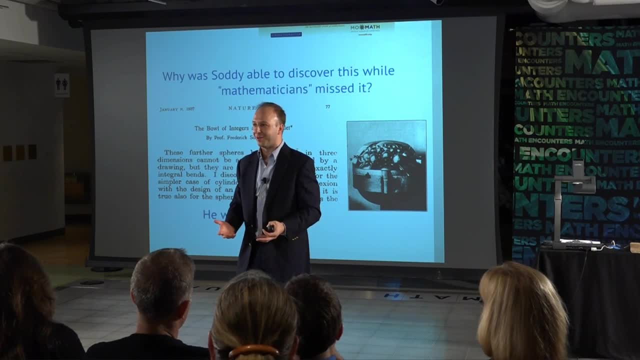 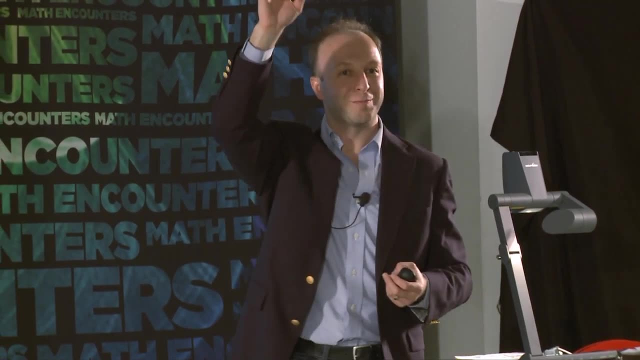 And I got a sphere of radius 1. third, Why are all these numbers 1 over an integer? And he dug deeper And he realized the answer. So sometimes it's not so good to be up in the sky of this perfect, pretend heaven world. 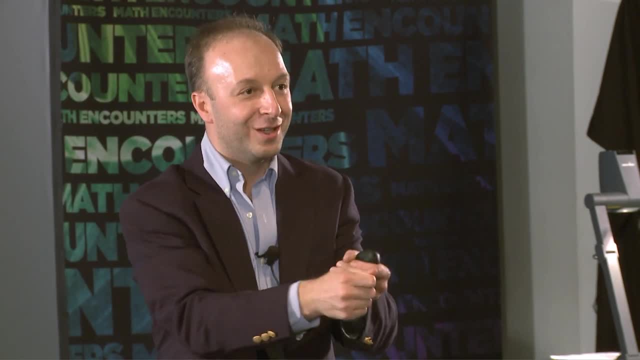 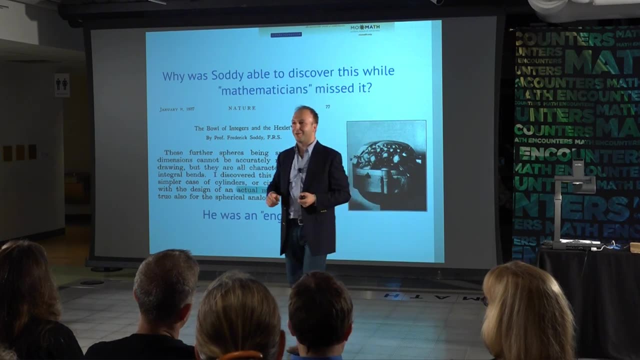 Sometimes you need to come down to the ground and do a physical, physical calculation and move some disks around so that you can discover things that you can't see when you're up in heaven. He was an engineer, not a mathematician. That's why he was able to make this breakthrough. 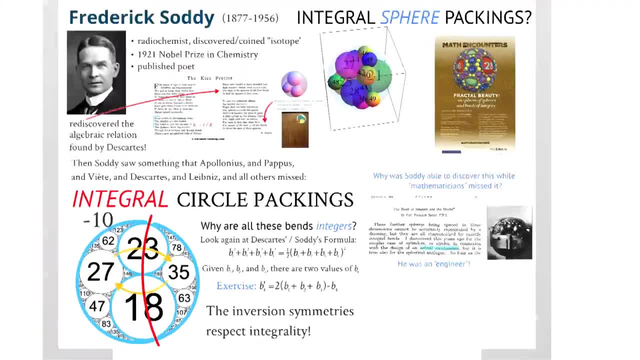 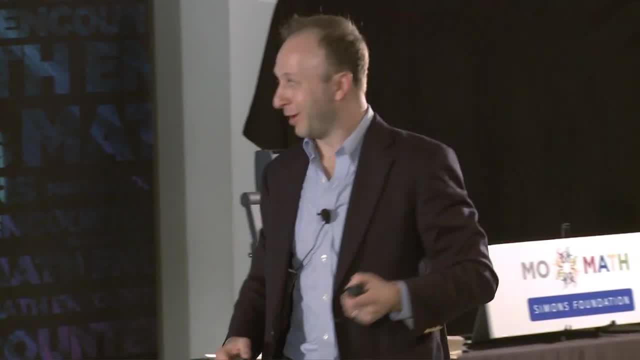 that mathematicians could not. One final question: I'm a number theorist, Dorian's a student. He's a number theorist. He taught me so much about these things. One final question is: which integers? So you're given a sequence. 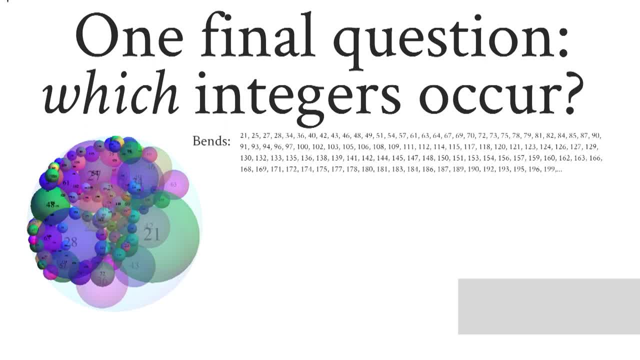 You're given a set of integers. So here's the packing with lots more spheres filled in. I'm sure you can't see. So here are some of the bends. There's a: 21,, 25,, 27,, 28,, 34.. 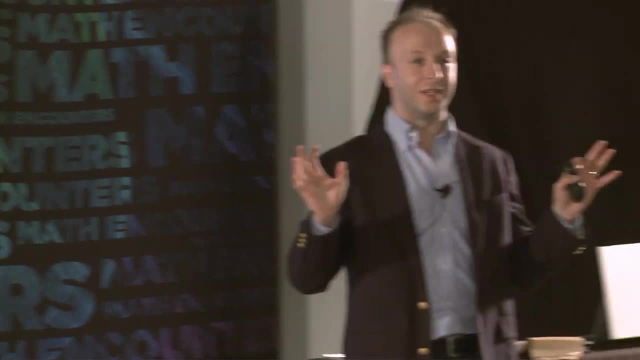 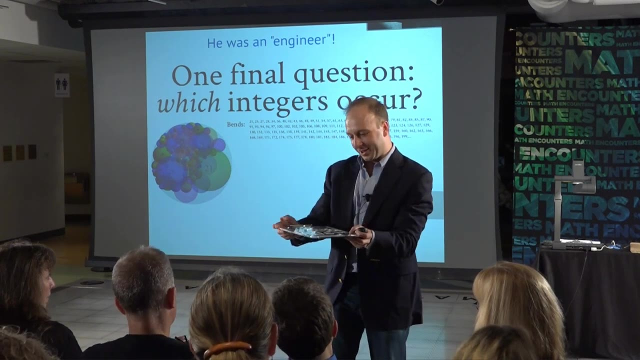 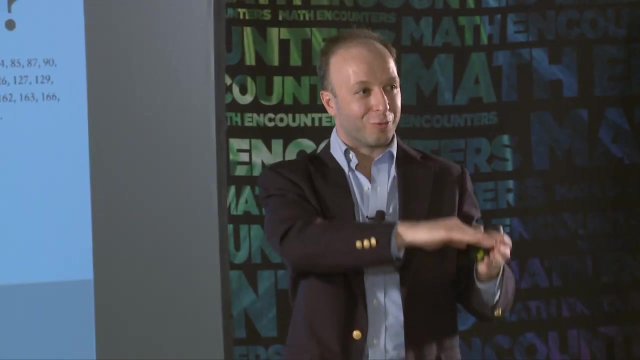 This is a long string of integers. These are all the bends that arise. I'm taking out multiplicities. You see, even in your disk there are two 135s. So there are some multiplicities. There have to be multiplicities because the rate at which the curve is growing. 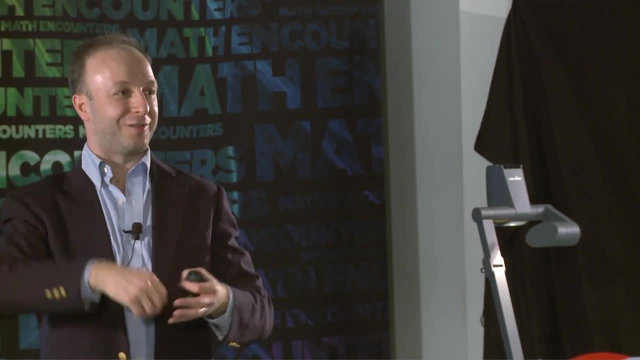 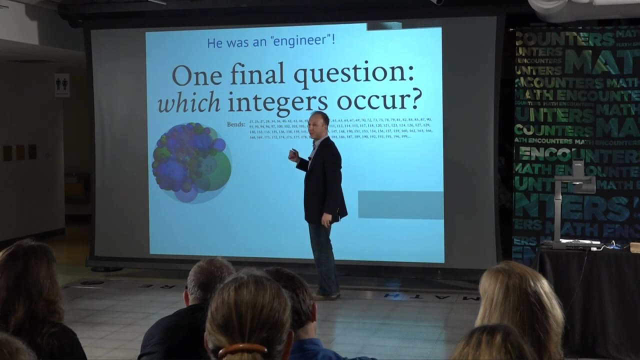 the number of circles is faster than the number of integers, So there are going to be multiplicities. So if we take away the multiplicity, if you just say which integers will you see in this list? Well, you stare at these numbers for a while. 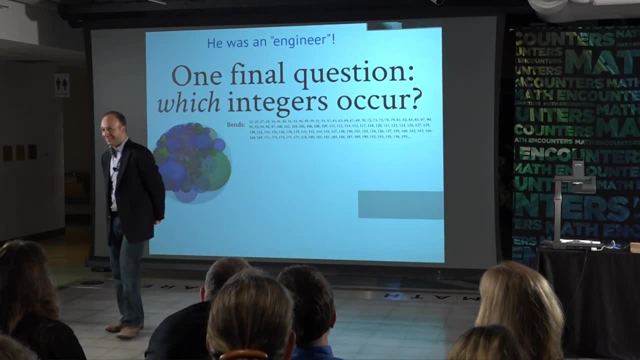 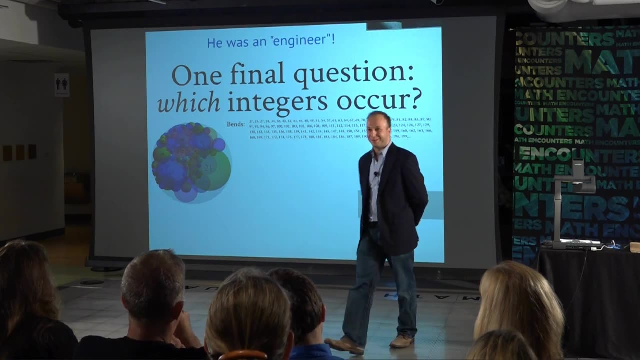 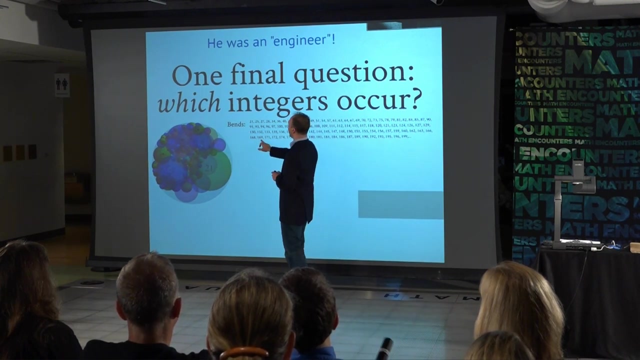 Take a walk, You have some coffee. You see any patterns. This time we won't wait 350 years, It's almost. you see, you go from 168 to 169, and then 171, and then 172,, 174,, 175,. 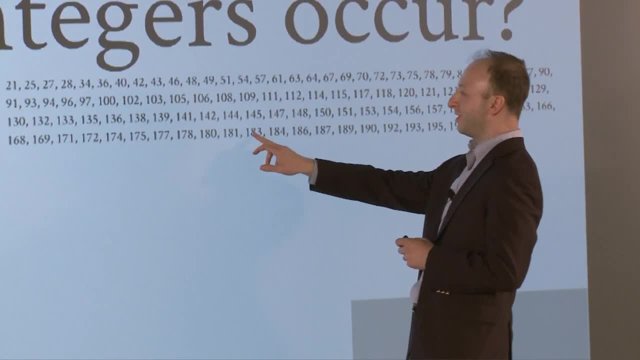 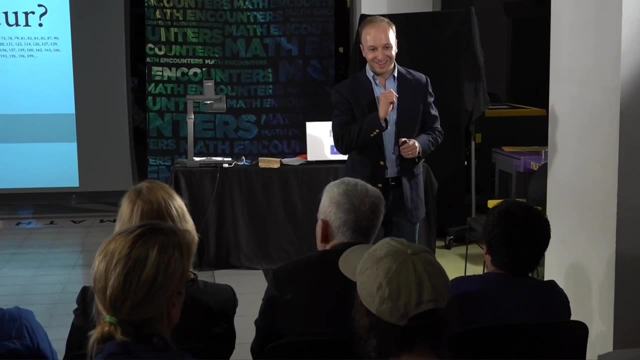 177.. You skip by one, you skip by two, You skip by one, you skip by two. So one way of just: yes, sir, They're all multiple of three except for one, Perfect, Perfect. So the observation this gentleman just made. 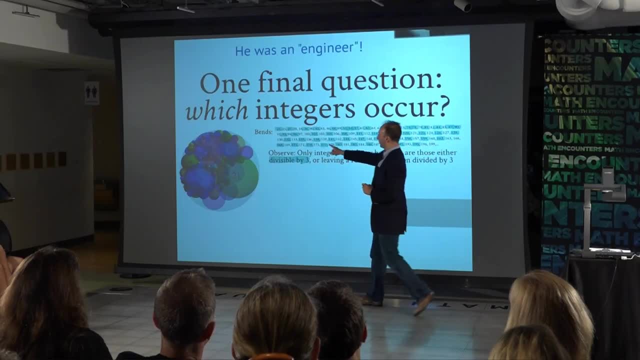 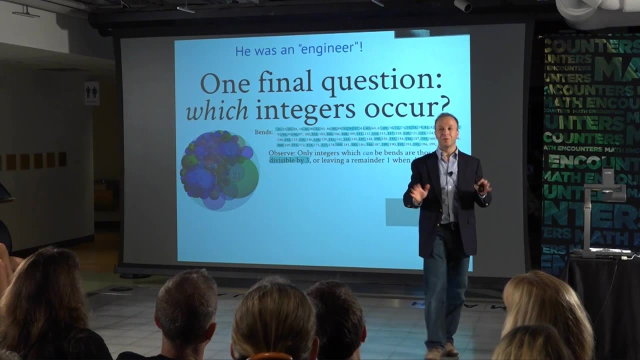 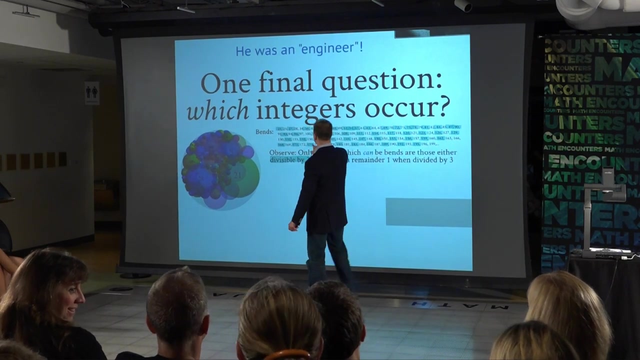 is that the integers that arise are all either multiples of three- those are the ones that are colored- or one more than multiples of three. You do not see any numbers that are two more than multiples of three, So that's why you're seeing this skip by one, skip by two, skip by one. 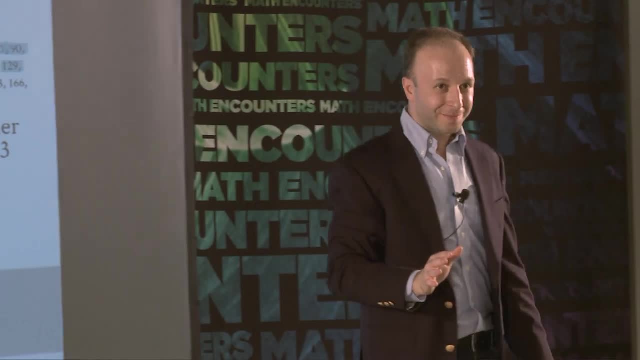 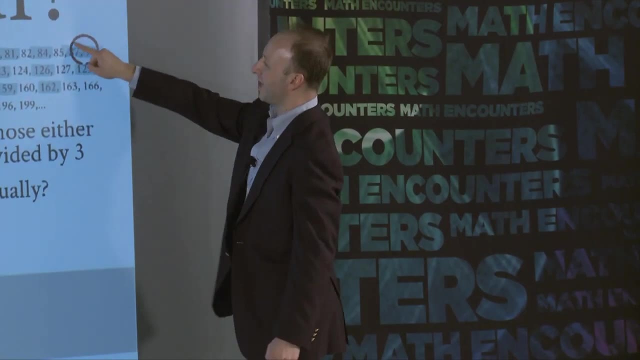 skip by two, skip by one, skip by two. pattern. Except that's not exactly what's going on. There are some gaps. Between 87 and 90, we're missing 88.. Between 163 and 166, we're missing 165.. 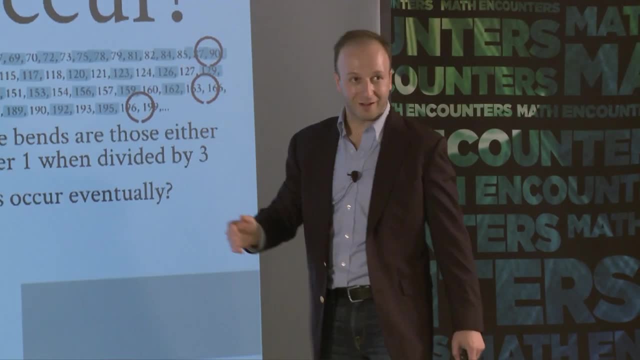 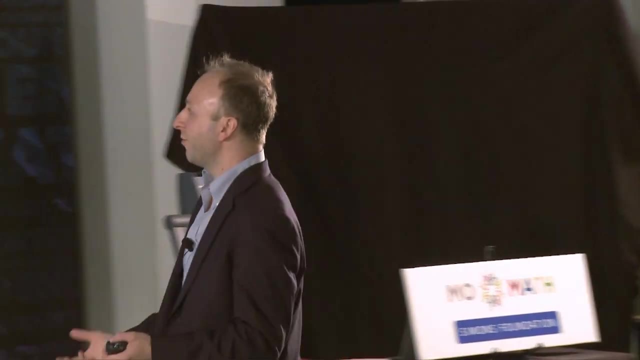 It should be there And here's another one. There's another gap and there are others. Do these gaps continue happening? Maybe the gaps are just some low. You see, there have to be gaps. The number 18 is a multiple of three. 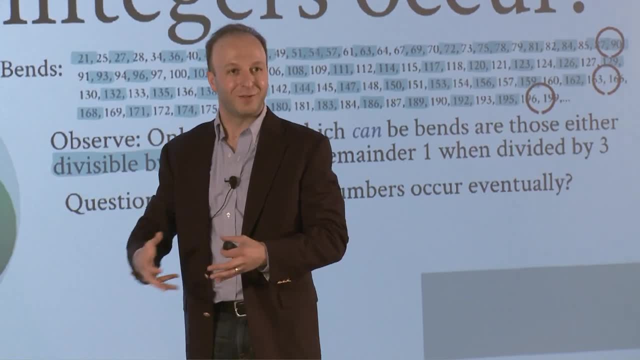 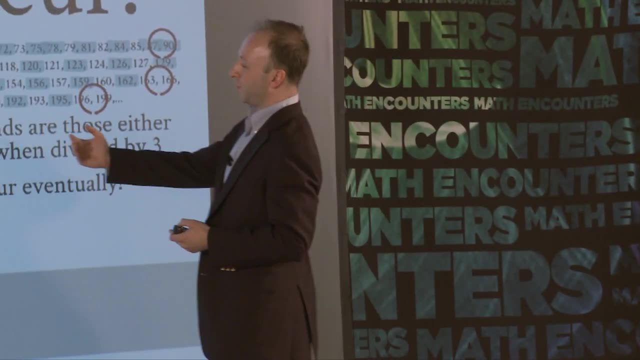 but it doesn't appear, because a sphere of radius 1 over 18 is too big to fit in this packet, So it's not clear what happens, But maybe all numbers which are either multiples of three or one more than multiples of three after some point. 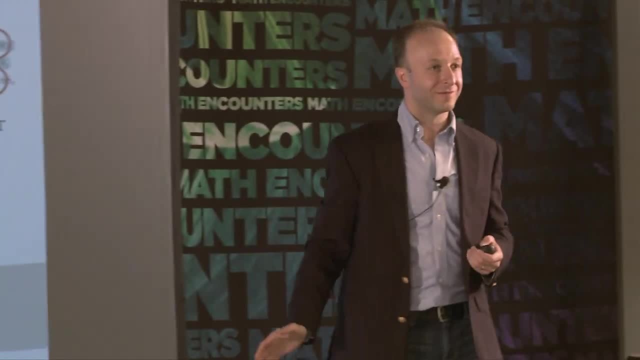 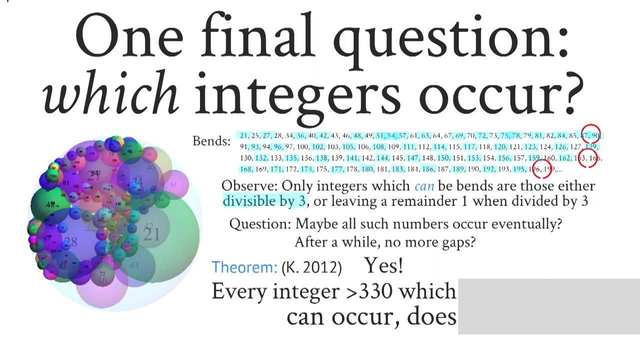 arise. Maybe eventually there are no more gaps, And indeed that's the case. So this is a theorem from just a few years ago. Once you get beyond 330, every number that's a multiple of three, or one more than a multiple of three. 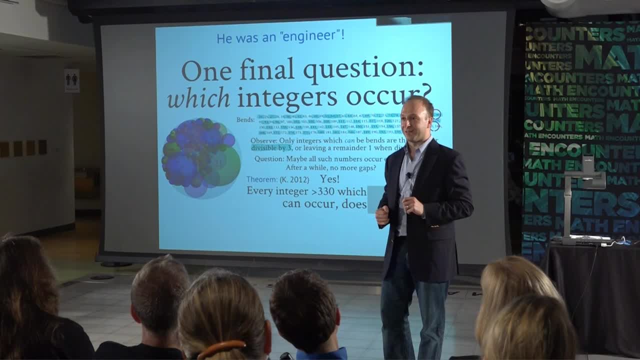 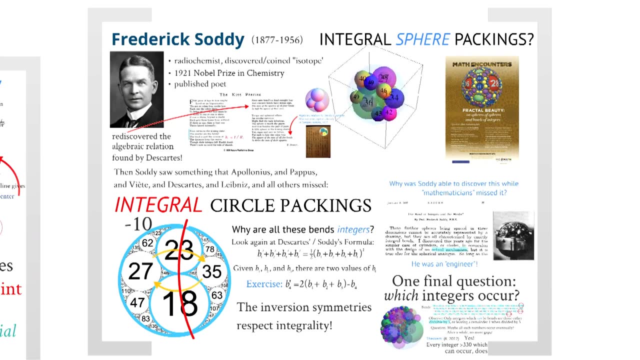 does arise. So there's no mystery in the integers which arise in these packets for the sphere case. All right, I think that is all the time we have today. I want to just thank Hiroko Takano. Hiroko, Hiroko Takano, if you could come up so that people 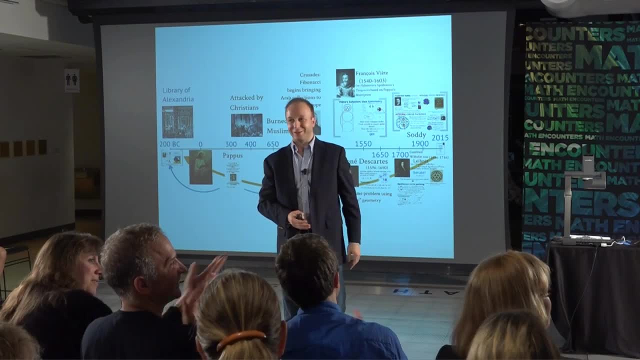 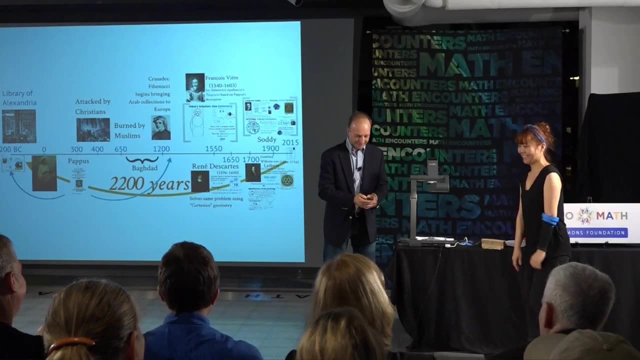 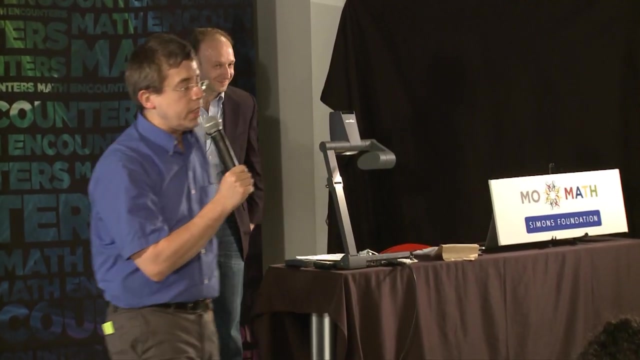 can see who you are. Hiroko made all of these beautiful disks. Take a bow, And that's all the time we have. Thank you, OK. So fortunately, we do have time for a few questions. So if your brain is not fully packed, 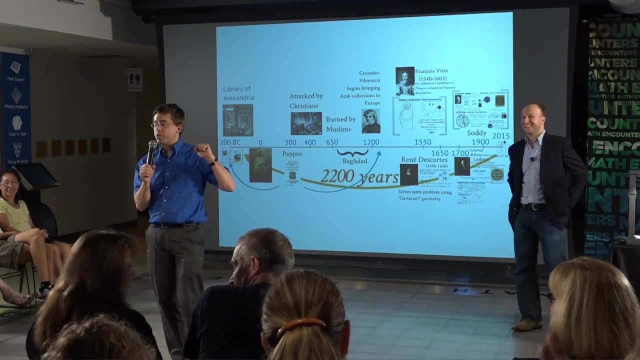 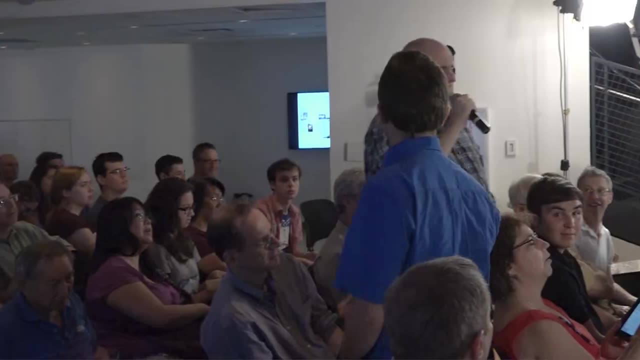 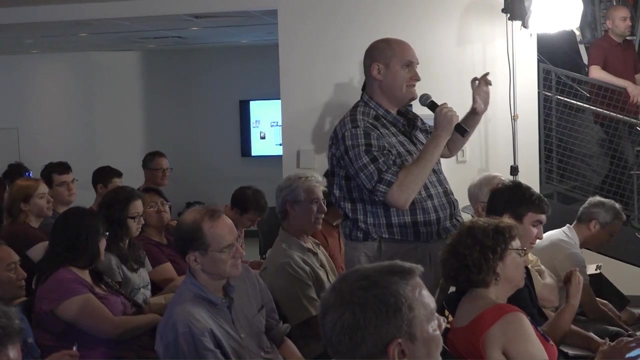 with spheres of knowledge. then you can get a question Or two, either for our mathematician or our wonderful circle fabricator. So we'll start right here. Fantastic lecture. first of all, I want to say So. I had a question about your choice of the initial circle. 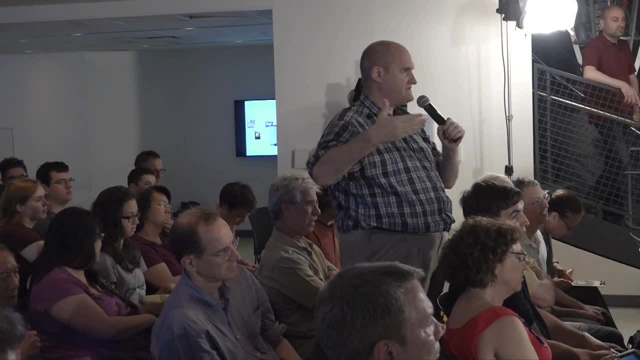 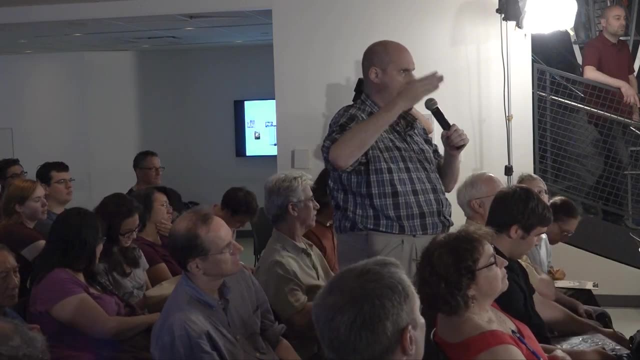 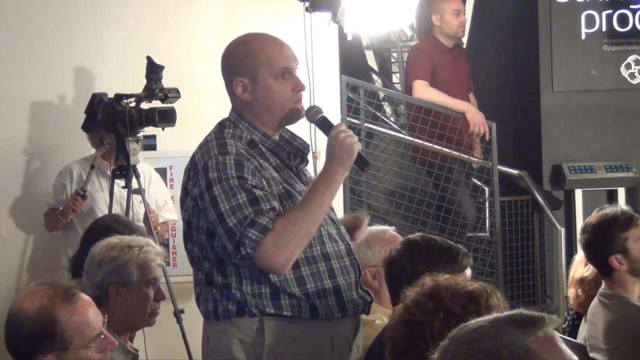 being 18.. Yes, And how that affects all the other things that you talked about, specifically how many circles you can get in under a certain threshold, as well as no remainder of 2.. So you could have started with 20, and then there would be one that didn't fit the pattern. 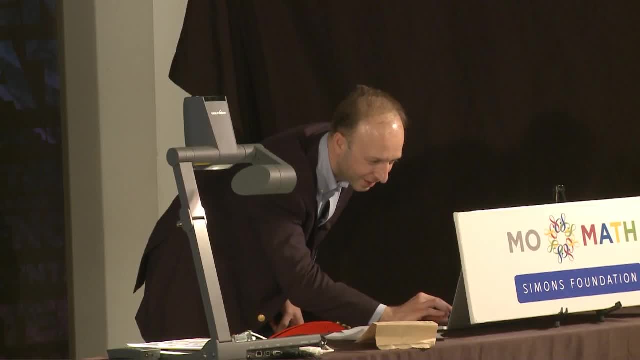 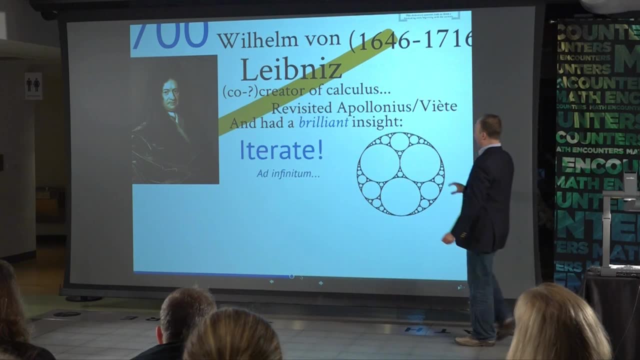 And then how would that affect all the other circles that came after it? Excellent question. Let's go back to Leibniz. So this was Leibniz's actual packing that he started with, And what he started with was three circles. 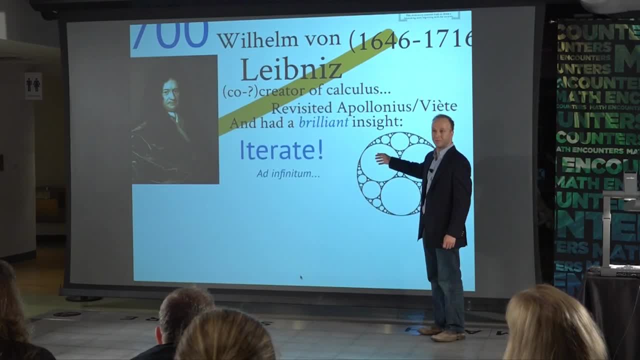 of exactly the same radius, So we may as well call it 1.. And when you solve the Descartes formula, this inner- So if you started with 3 equal, This inner circle- has curvature like root 3 or something: root 3 plus 2.. It's not an integer. You would expect the square root right, Constructing something with straight edge and compass. why should there be square root? So it's a very happy accident that there at all exist any configurations which lead to integer curvature. 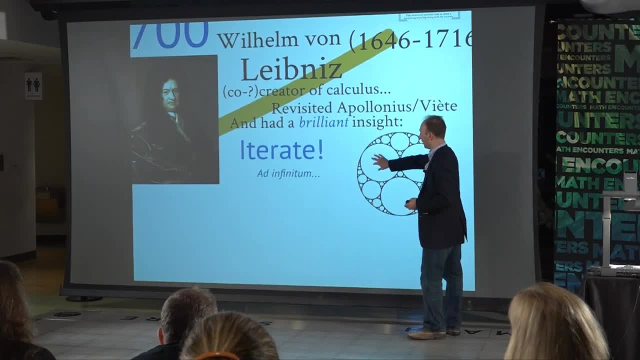 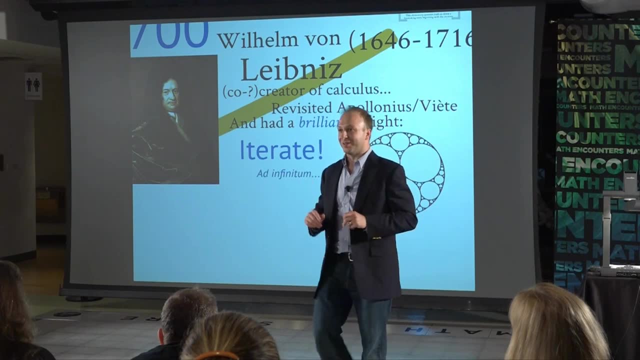 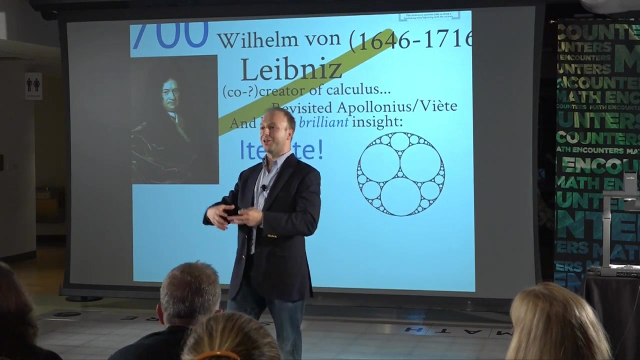 So you can have, as in this case, three circles, all of whose curvatures are integers, but then the rest are, all You know, some quadratic numbers or something, Square roots. they're all messed up. So the 18 was just one out of infinitely many configurations. 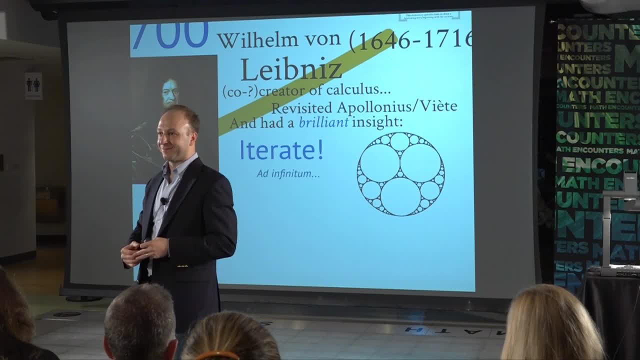 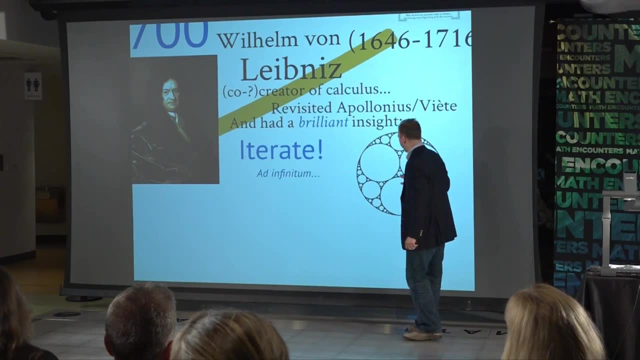 which have integral circle packing. So the 18 was arbitrary, but not that arbitrary. Had Leibniz started with a circle of radius 1 half and a circle of radius 1 half, sitting inside a circle of radius 1, he would. 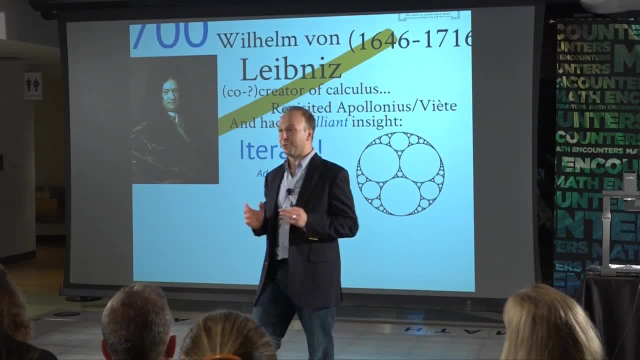 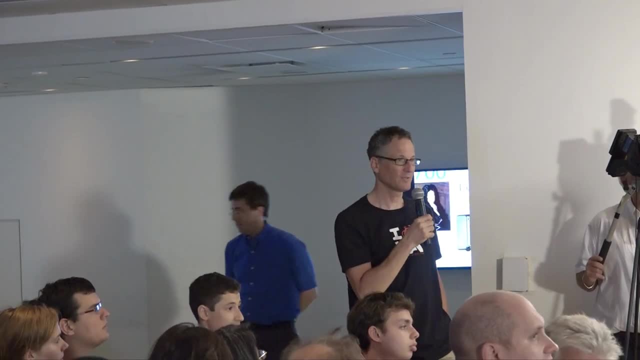 have found the smallest bounded integral packing And he would have realized this integrality, But he didn't. I was wondering what the how one predicts the location of the next circle. There doesn't seem to be a clear. I thought at first it might be a spiral pattern. 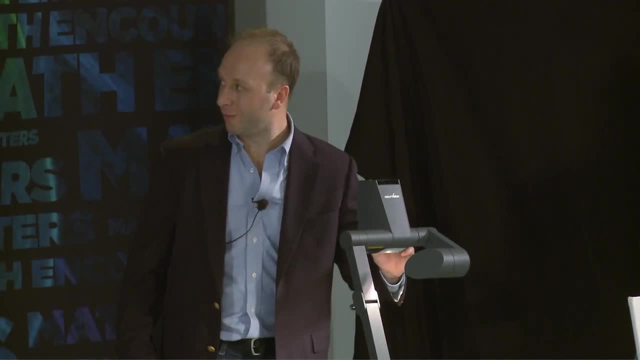 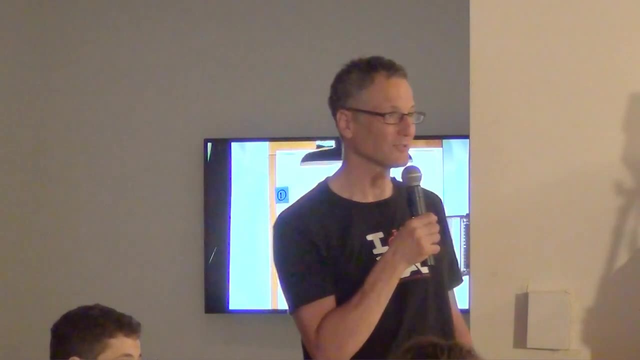 but that doesn't seem to necessarily hold. So what do you mean by location? Because every place, Yeah, the placement. So, especially when you have multiple options and when the integers get closer and closer together, is there a formula for the actual placement? 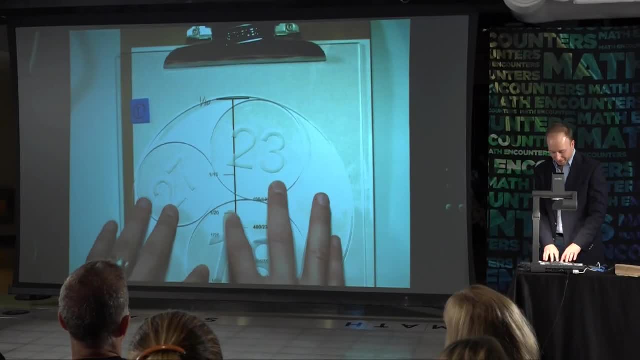 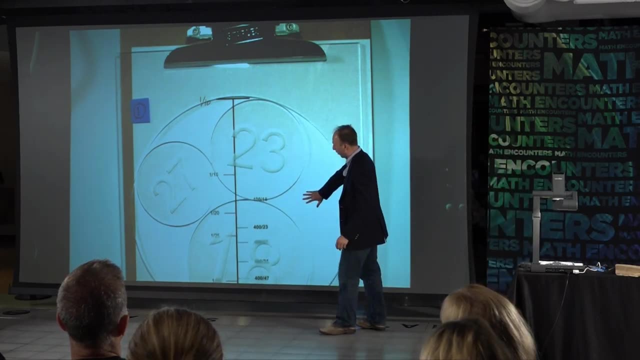 of the next integer in question. So let's start with the original configuration, which is these three circles. Very good question. What we'll notice? we can do this by generation. What we'll notice is we have one, two, three, four gaps. 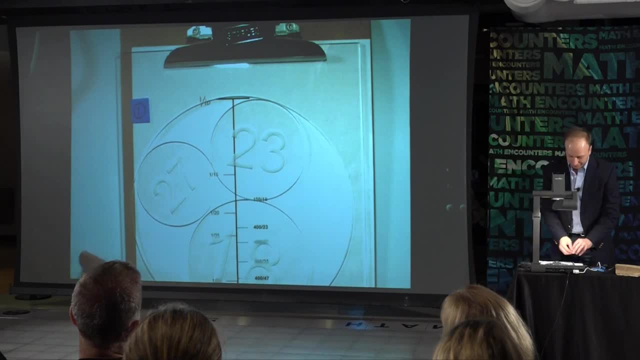 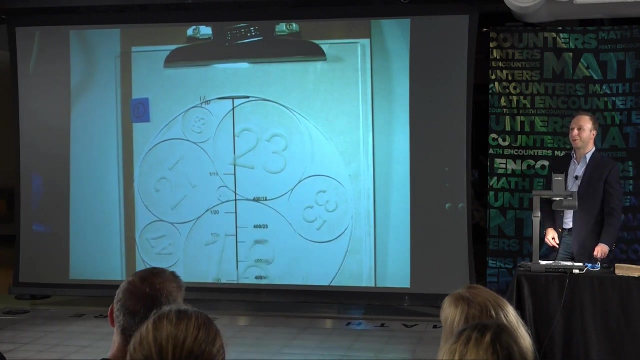 So all we're going to do is fill each of those gaps. So we fill this gap, then we fill this gap, then we fill this gap, and one more, is that 146.. And then we stop and say: OK, now what gaps do we have to fill? 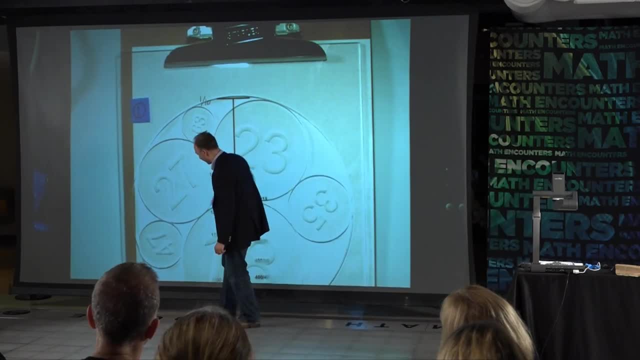 We have to fill 1,, 2,, 3,, 4,, 5,, 6,, 7,, 8,, 9,, 10,, 11,, 12 gaps, And then we fill in those. So if you do it by generation, then you just 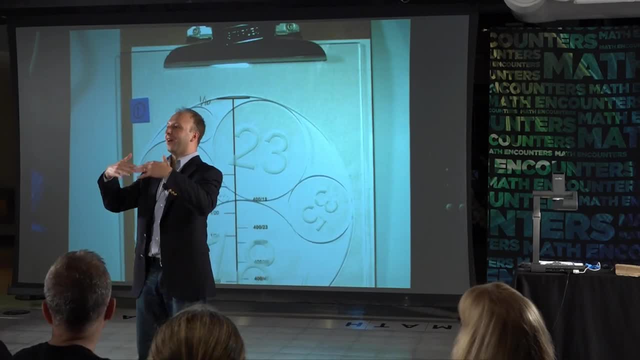 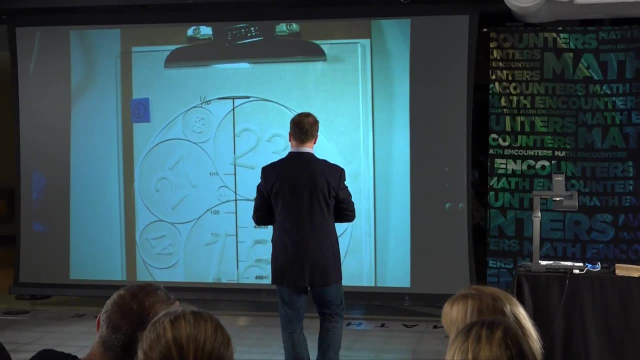 fill the gaps in the date on which they're born, And is there a geometric? Does that generate a geometric? Is there any sort of underlying pattern that that generates? So if you count the circles by what date they're born, then the number of circles you're putting in 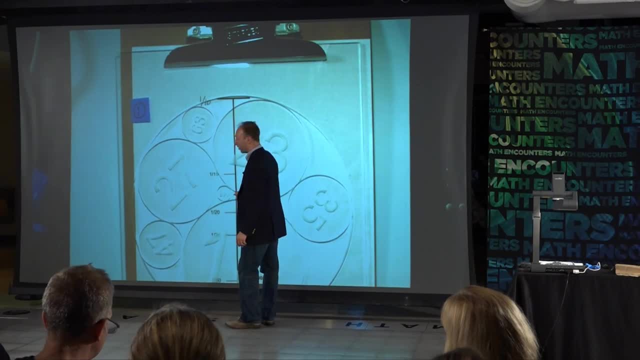 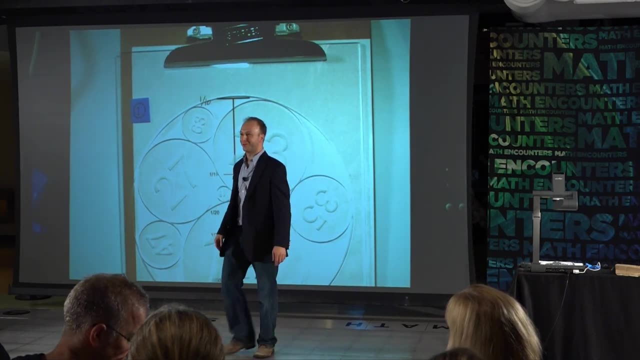 is very simple. It's just: every time you put in a circle you create three more gaps, Right? So it's 3 to the n, where n is the number of days times 4, because the first time you do it there's four of them. 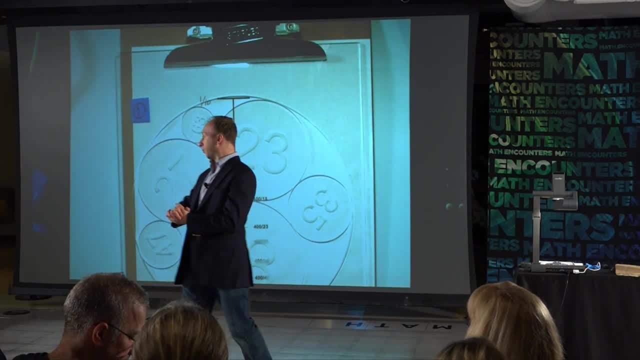 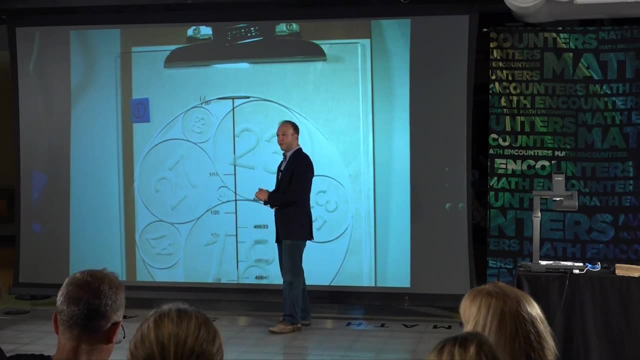 So that's something very, very rigid. On the other hand, if what you do is something completely different, if you say, I'm going to put in all the circles of radius at least 1 over 150. So you put all of those in at once. 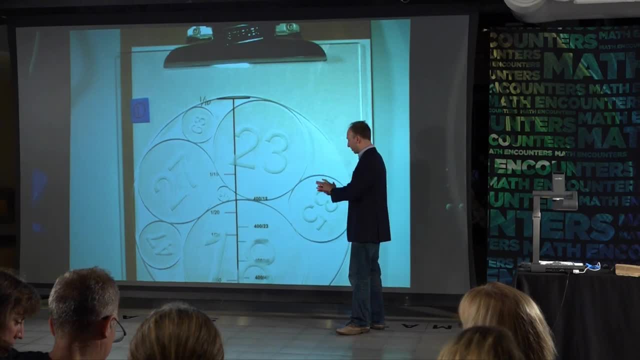 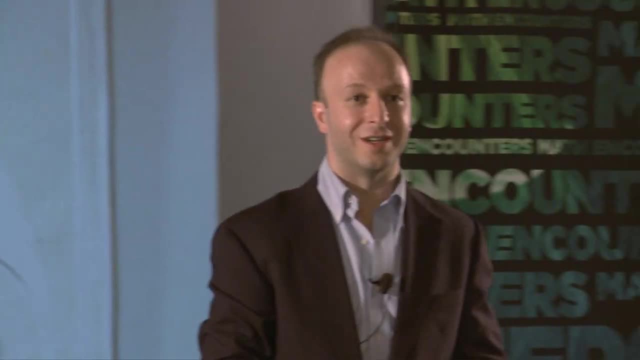 Or you just say: what's the next smallest circle that I can put in? So you put in circles by when the next smallest one comes. Then you get this other asymptotic growth rate where the fractal dimension enters the conversation. OK, And if you do put them in a numerical order. 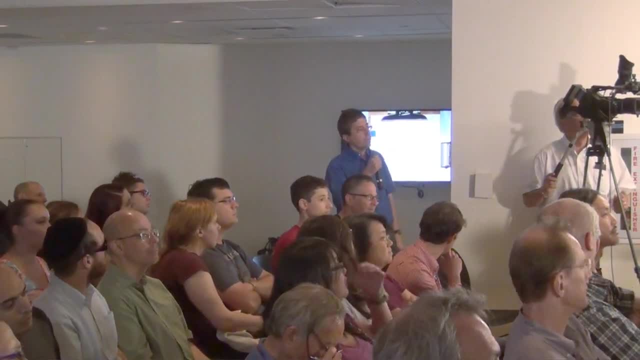 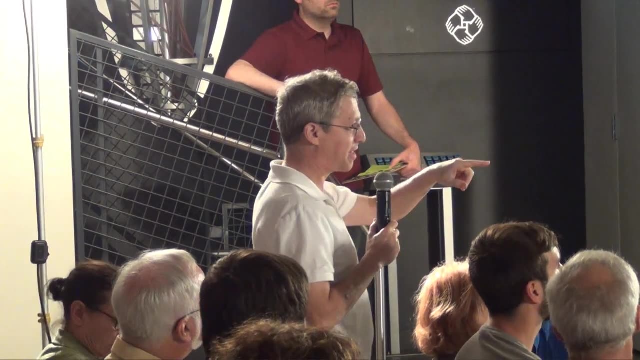 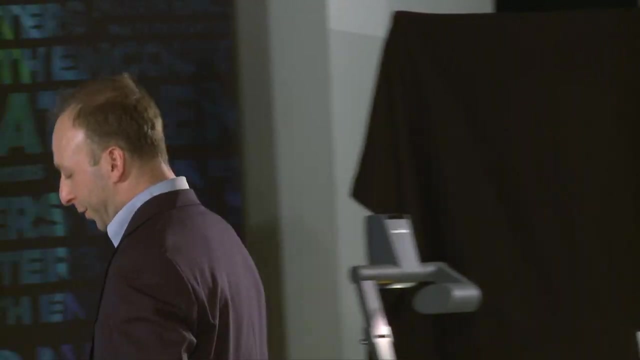 they just appear sort of in random spots At random. Yeah, Again, wonderful lecture. In the last theorem that you mentioned, how did the number 330 depend on the number? what was it? 21 or something? So the theorem actually says that for any integral, 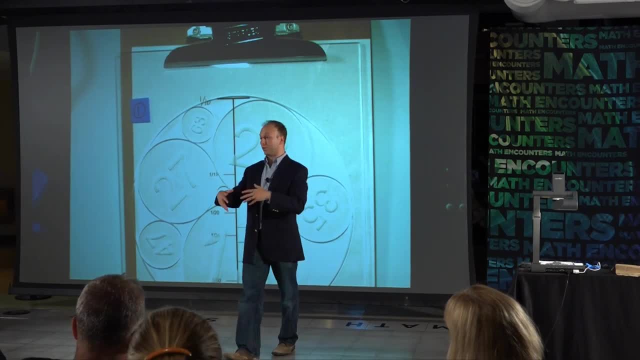 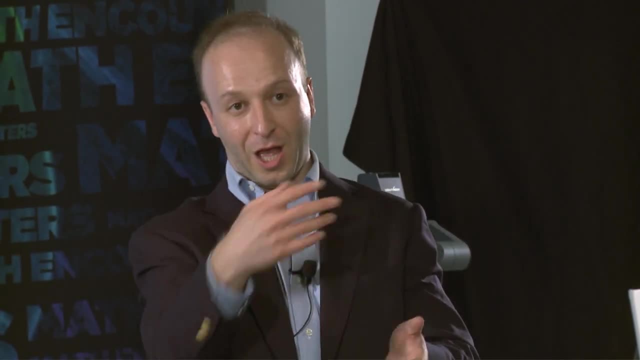 configuration. there are some. these are so-called local obstructions. There's some. In fact, they're all mod 3.. So you'll either have numbers that are multiples of 3 and one more than multiples of 3.. Or you'll have numbers that are multiples of 3 and two. 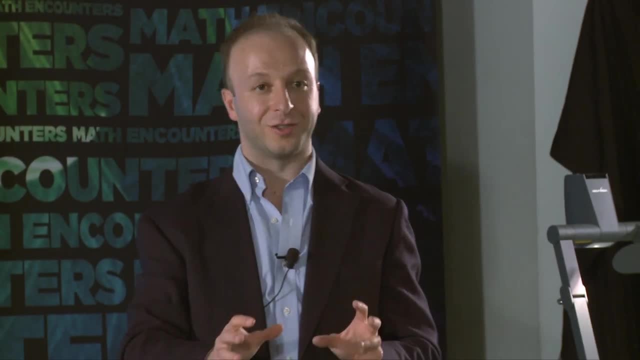 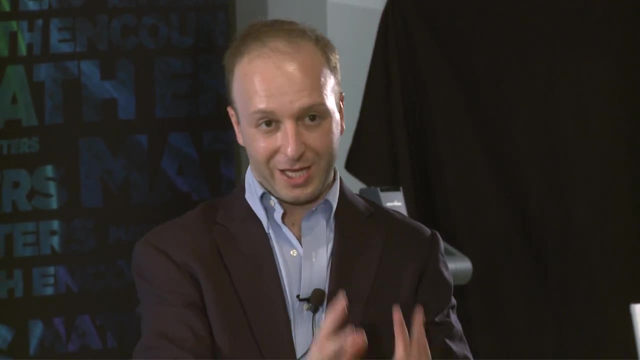 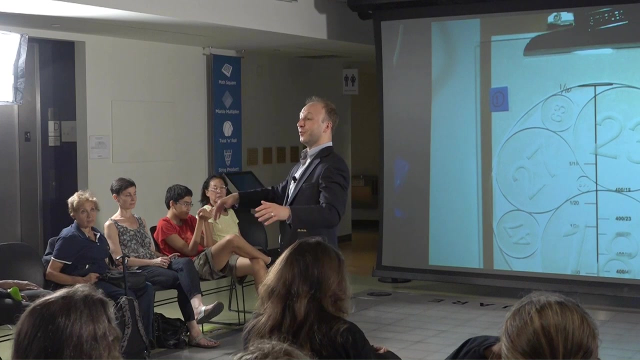 more than multiples of 3.. So there's always some obstruction for integers to arise. You probably grabbed the 330 answer And the theorem says: beyond those obstructions, for any given configuration there's a number beyond which the pattern repeats itself exactly. 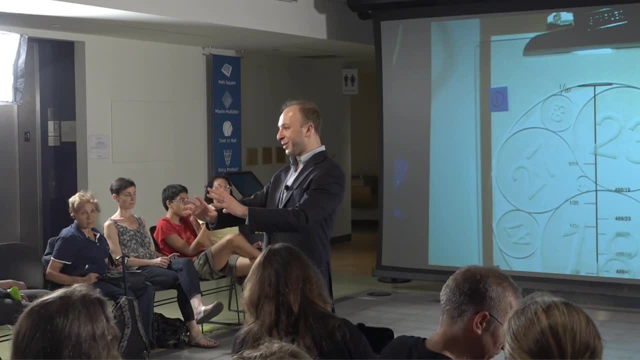 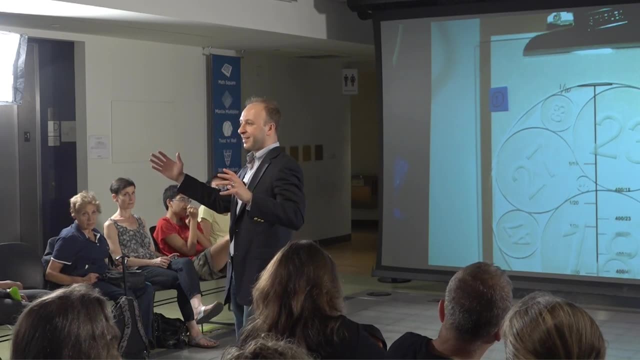 So it just so happens, for the 18,, 23,, 20, 27 configuration or whatever that was the circle packing, We're talking about sphere packing. For the sphere packing it kicks in at 330.. Do you have a bound on? 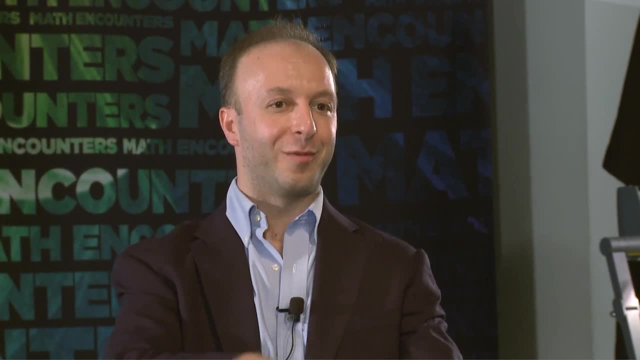 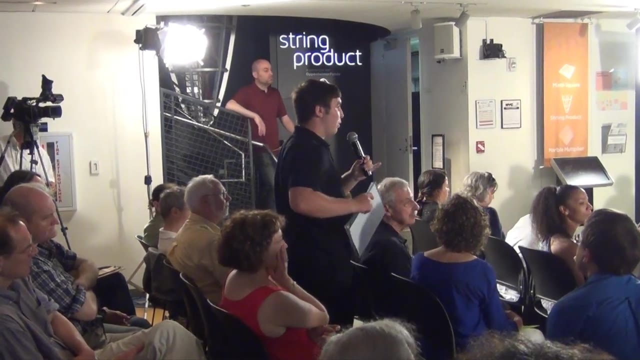 There is some bound, given the initial data. There's a complicated formula, given the initial data, to figure out when the theorem kicks in. Hi, I was just wondering if you have that picture where you're showing that inversion from the 27 to the 35.. 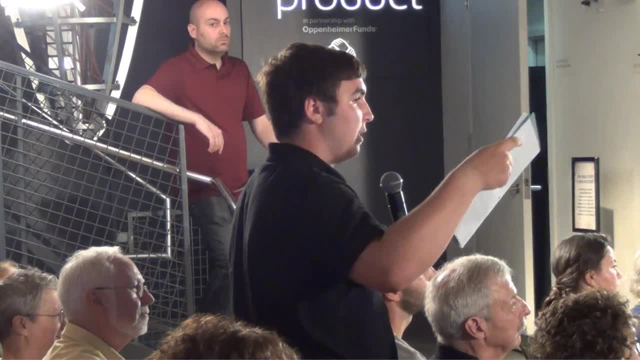 Yes, If that arc is the- I don't know- 27 to the 35,, is that the same as the 27 to the 35?? Yes, The arc that connects the three centers of the circles in question, and if there's any connection. 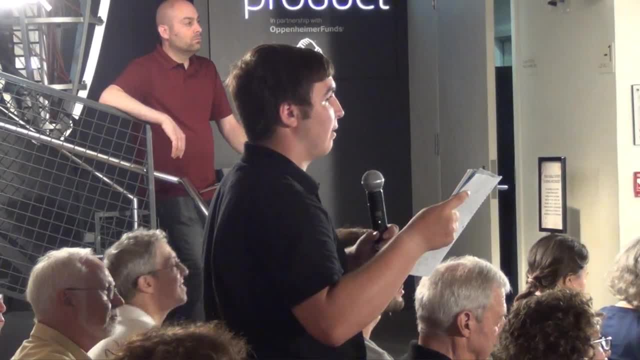 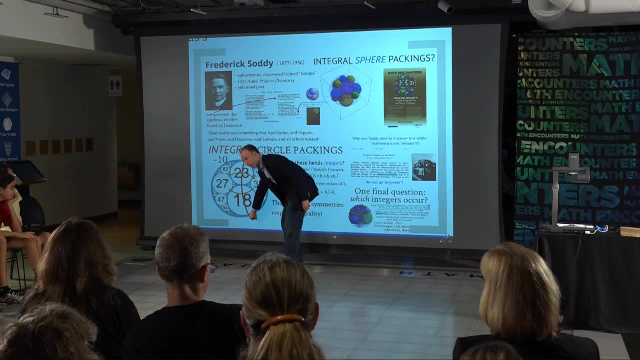 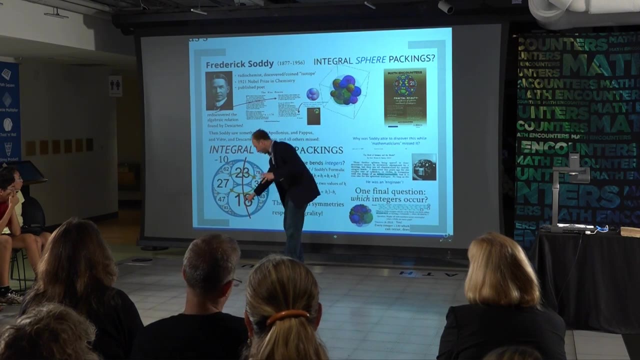 between connecting those circles and making and solving that Very good question. The way this arc is constructed is you take the three points of tangency, not the centers of the circles, but you take the three points where the circles kiss. Three points determine a circle. 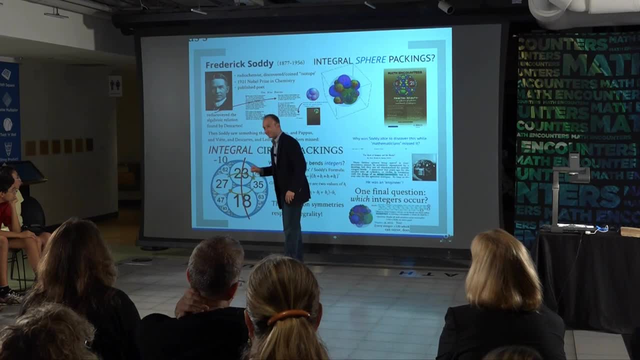 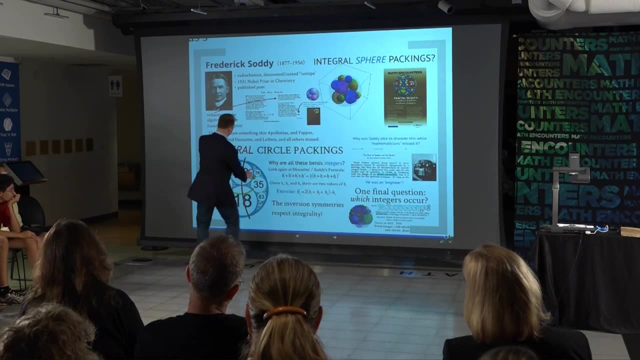 That's what that arc is. It does not go through the centers, in fact. And just to clarify what happens to that 23 circle under inversion in that red arc. So if you just look at the circle itself, it's completely fixed. 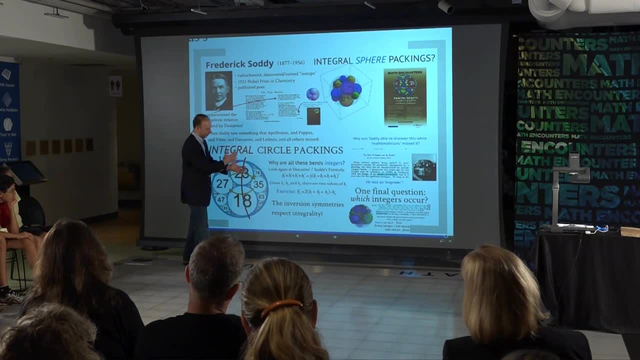 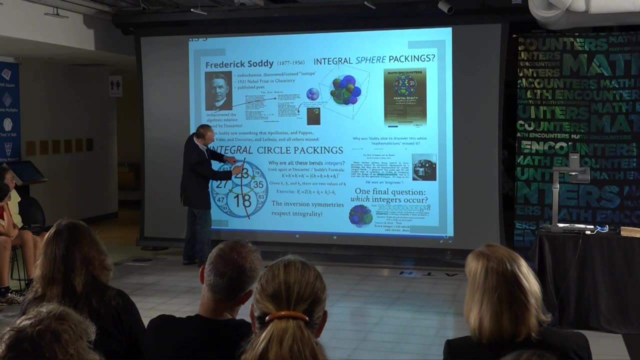 So this piece of it turns into that piece and vice versa. It just flips on itself. Now, if you put equally spaced points and you do the flipping, they're no longer equally spaced, But the reflection you see, these meet at a right angle in the two places where they meet. 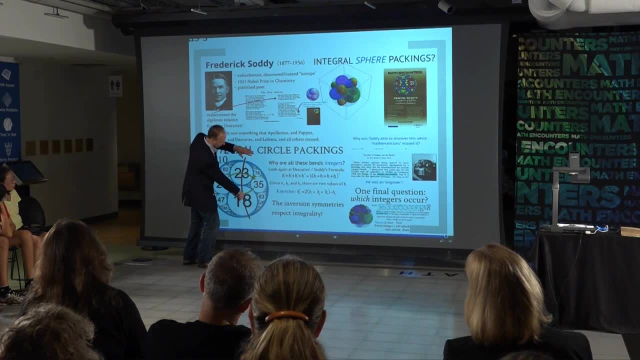 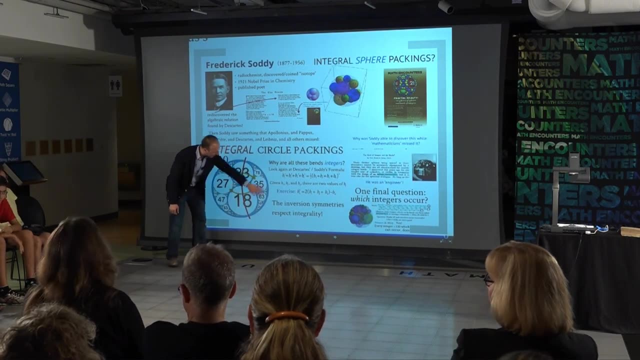 So if two circles are orthogonal and you reflect one through the other, it preserves the picture. It's fixed. So 23 is fixed, 18 is fixed and negative 10 is fixed And everything else is flipped over from one side to the other.